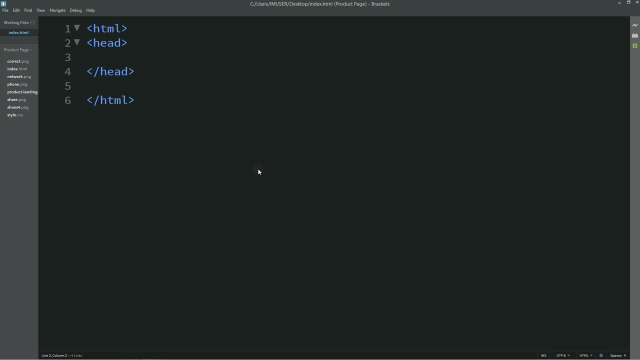 like meta description, meta title and other meta tags of this webpage. after head tag we will write body, open and closing tag. so whatever content we will write in this body, that will be displayed on our webpage. so the maximum things we will write in this body. so let's see how we can add title in our 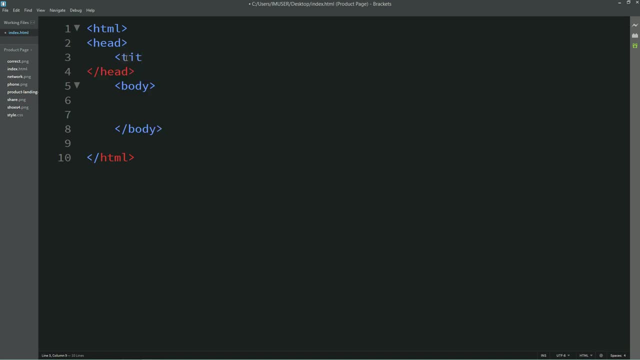 head tag to add one title. we need to write title- open and closing tag- and in between that we will write any text that will be our title for our web page. so this is our website title. let me save this page and now let's see how we can preview this. 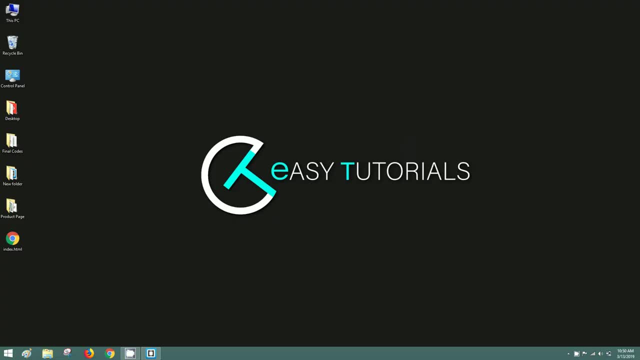 webpage for that. come back to the folder where you have saved the file i have saved on my desktop. so here it is: indexhtml file. i will open with my google chrome. if your html file do not open with my default, then you can right click over here, then select open with and select the google chrome. 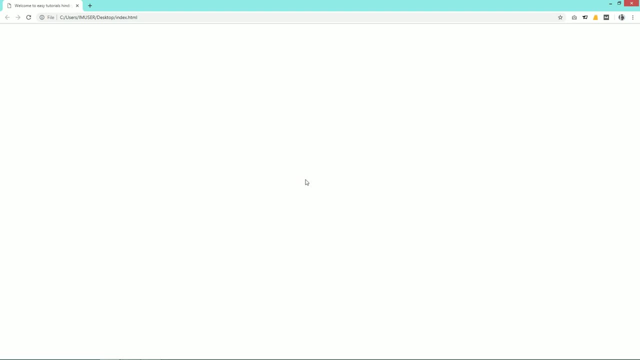 so now you can see this web page on this web browser and right now this web page is blank because we have not written any code in body tag. but you can see one title on tab which we have added the title in body tag title. but you can see one title on tab which we have added the title in. 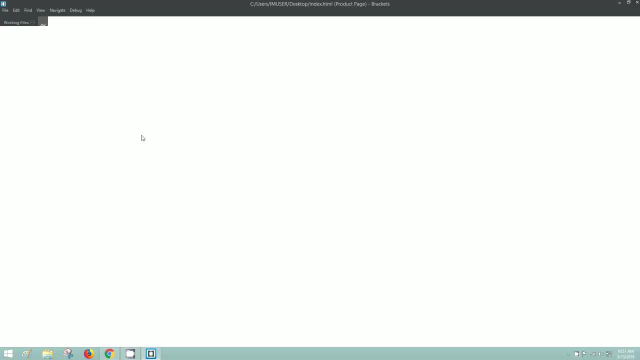 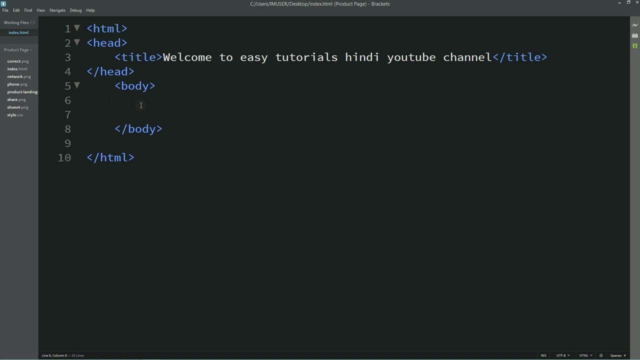 head tag. so let's come back in the html file and we will see what we can write in the body tag. so let's see what type of headings we can add in html pages. so let me write the h1. it is the heading tag. h1- open and close. let me write one text here. 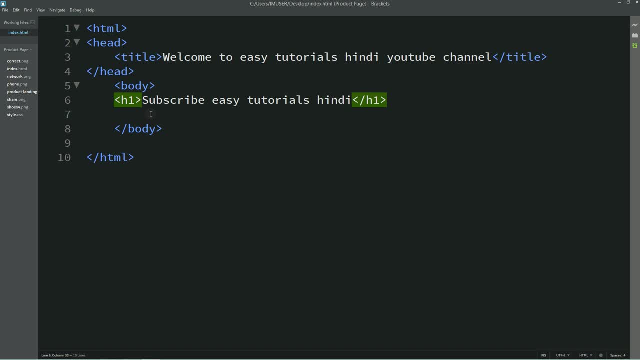 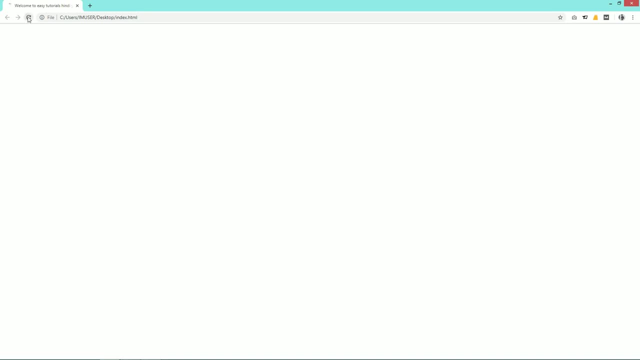 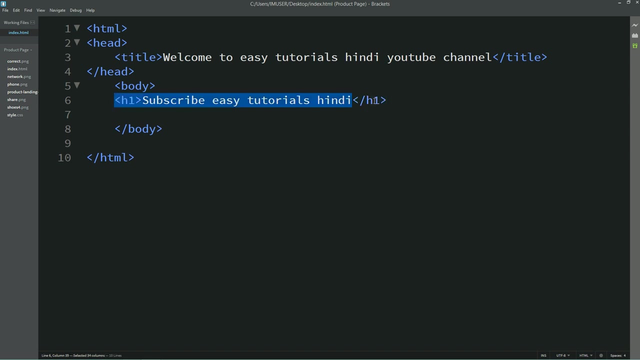 save this web page and again refresh the web page. now you can see the text on this web page that we have added in h1 tag. now let's see the other heading tags. so let me write it again. i will select and copy and you, if you are using brackets editor, then you can click here and press ctrl D. this is how you can. 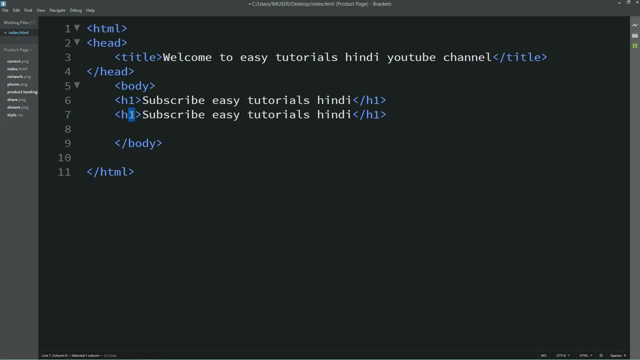 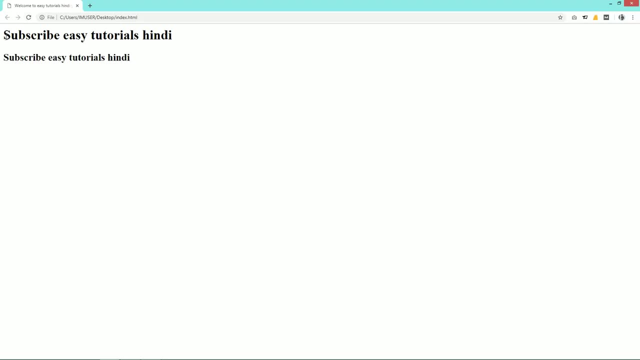 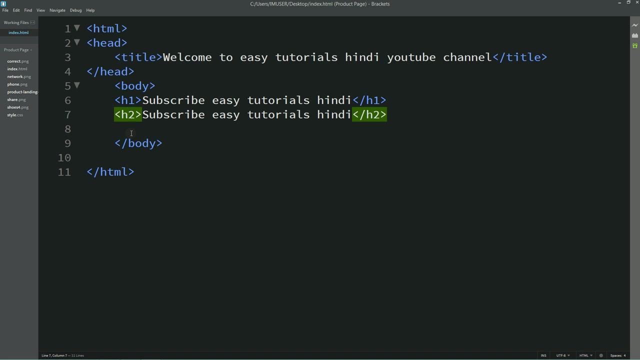 duplicate the content, so let me change it to h2, and this is the another title. let's refresh the web page and you can see there is one more title on this web page and the size is different. let's come back in the html file. now i will duplicate this h2 and will change the head tag. here it will. 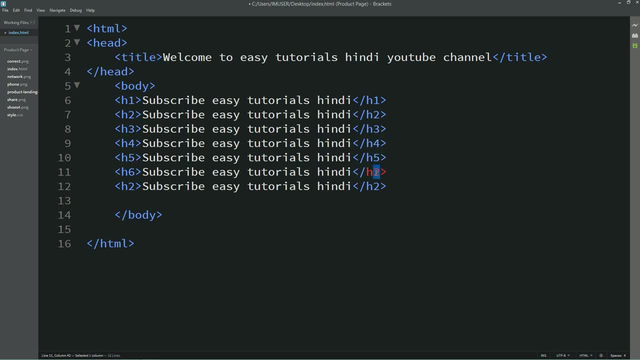 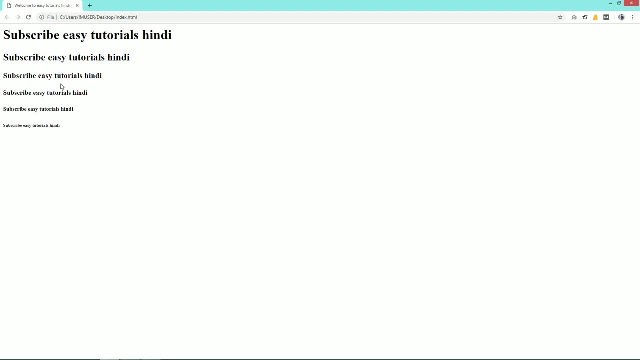 be h3, h4, h5 and h6. i will remove the last one. refresh the web page again, and now you can see all the heading tags on this web page and all sizes are different. so this is how you can add different size of text on your web page. and let's see how we can add simple text on our web page. 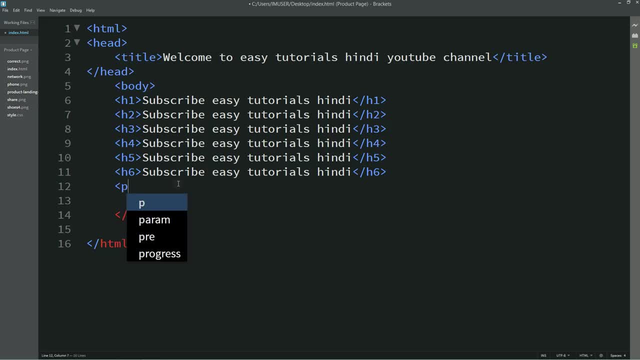 for that we will use paragraph text that we denote using p tag you. so in this p tag we will write whatever text that will be displayed as a normal text. so let me copy this text. i will add it in this p tag. i will duplicate it to increase the content length. 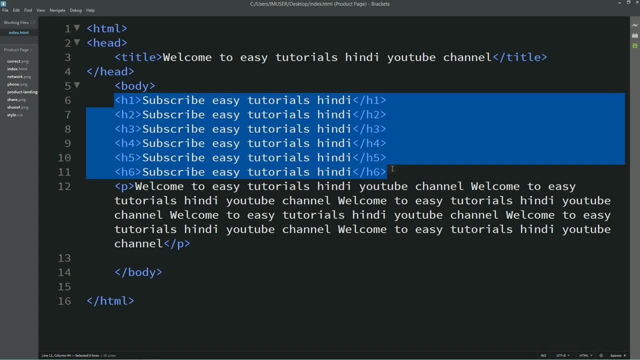 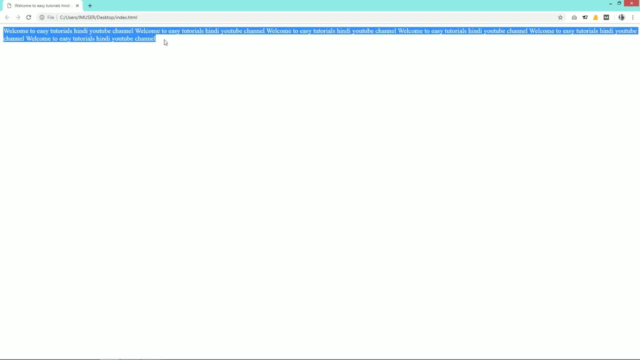 and let's remove this heading tag. refresh the web page and you can see all the text are in the small font. it is a normal font which is in paragraph tag. so mostly we will use this p tag in our web page everywhere. now we will learn how we can add links in our web page. for that we will use anchor tag that. 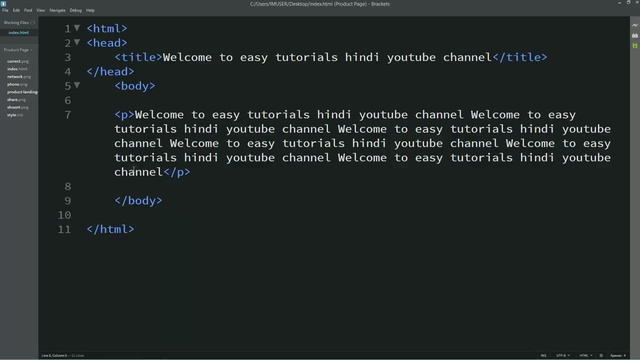 we denote using a tag. just remember whatever content i am writing here to display on web page that i am writing in the body tag. so to create a link, we are using a tag with href and href you can add a link on which link you want to redirect the user after clicking on that link. 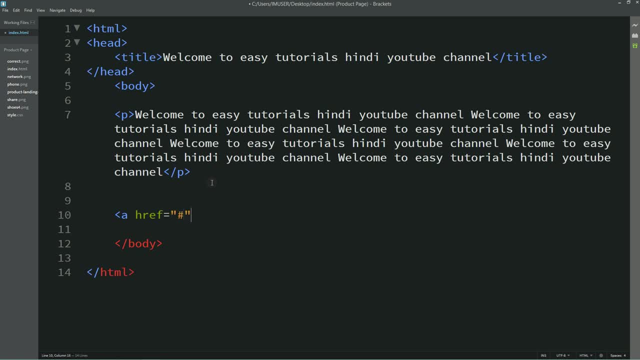 and if you want to redirect to the other page, then you can write the page name, like if you have another page called about dot html that you can add here. so let me write one link here. i will write googlecom. so this is how you can add a link in this href and: 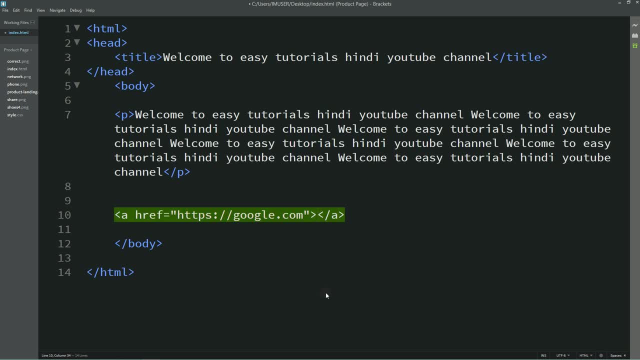 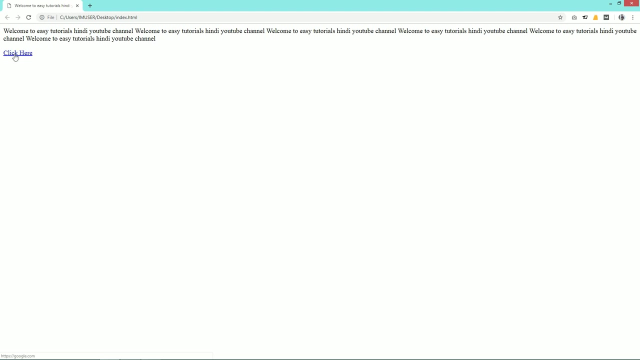 i will close this a tag and here we will write the text that will be our anchor text. so let me write one text here i will write: click here, reload the web page and you can see this link on this web page. as i will click on this link, it will open the. 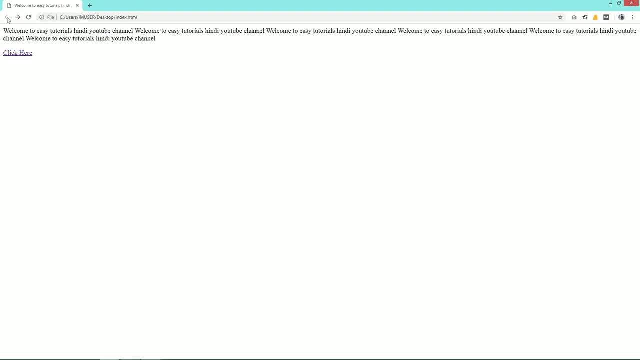 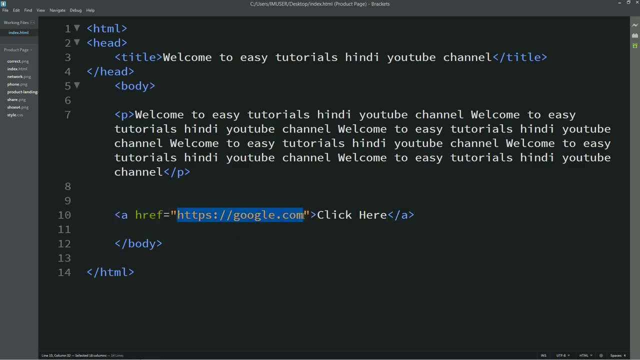 website googlecom. let me come back to our page. so this is how you can add a link text on your website using html. let me show you how you can add other pages link. for that i will remove this link here, and if we have another page called about dot html, then here we will write: slash about dot html. 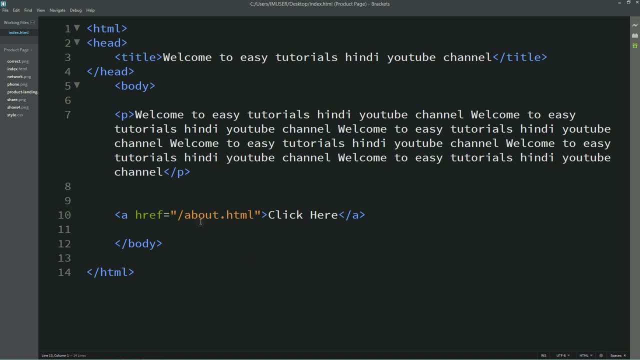 so if someone will click on this link, the people will be redirected to the another page, which is about dot html. so this is how our anchor link work. next we will discuss the tag small. it is very simple. let me write it here: small, open and close, and we'll write some text in this tag. so i am writing the text. this is a small text. 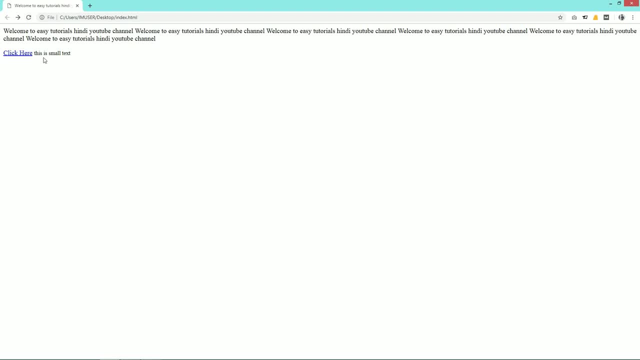 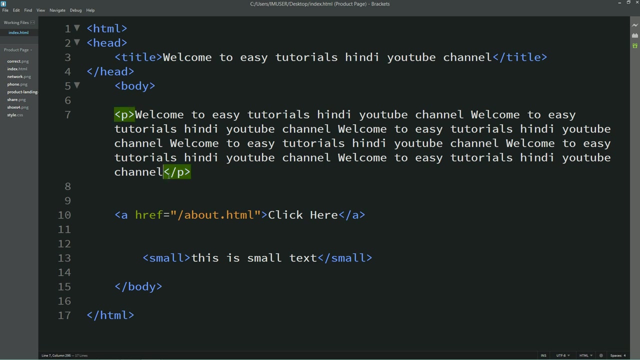 reload the web page and here you can see this text is very small, so its meaning is very simple. if you want to use a small text anywhere on your web page, then use this tag. next we will learn bold tag. so if we want to make the font bold, then we can add it in our web. 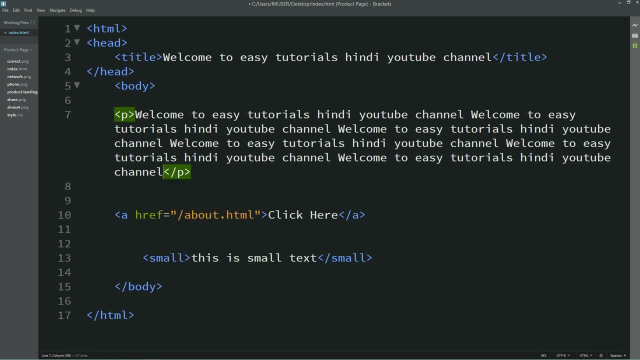 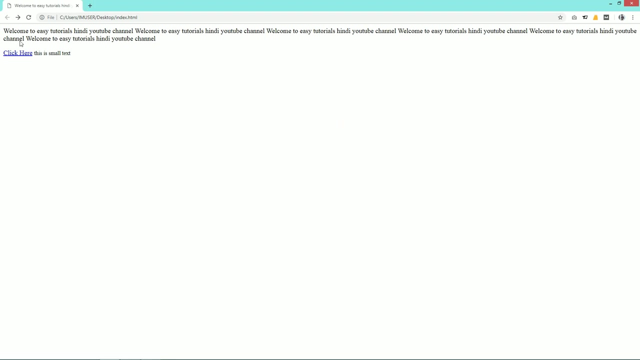 page. so suppose I want to increase the font width, so I'll write it here: be open and be closed tag. I will close it here so you can see I have opened the b tag here and closed it at this point. save these changes. reload the web page. 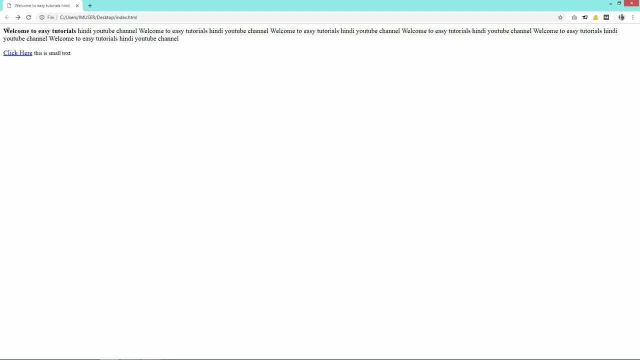 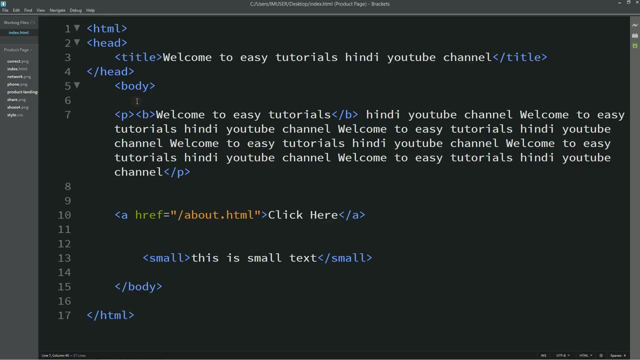 and now you can see other text are normal, but the first you can see- welcome to easy tutorials- is in the bold font weight. there is one more option to make your font bold. that is strong. let me write it here: instead of b, I will write a strong. 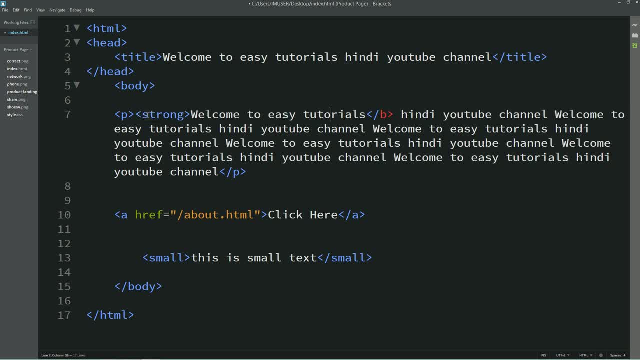 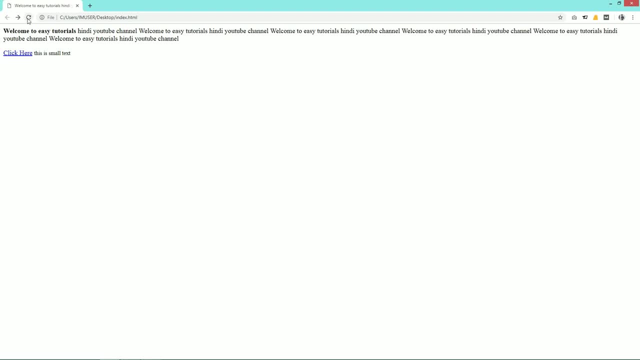 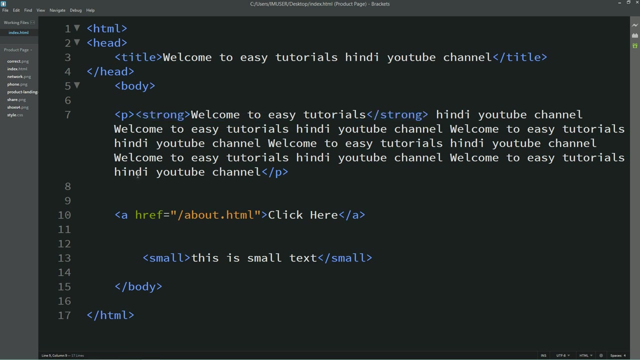 strong open, open and closing tag. reload the web page and you can see the same content here. first text which is welcome to easy tutorials. it is in bold and other is normal. now we'll see what is italic tag for that we use to write I, so you can see this text. the last text. 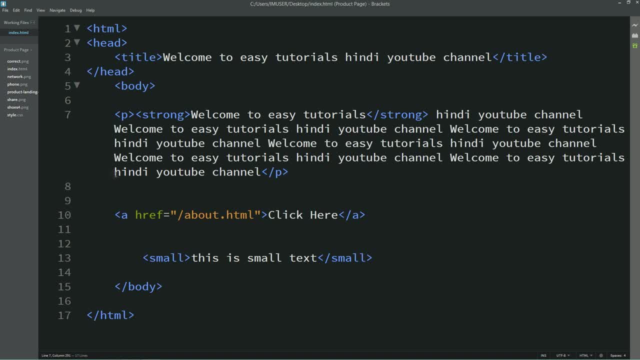 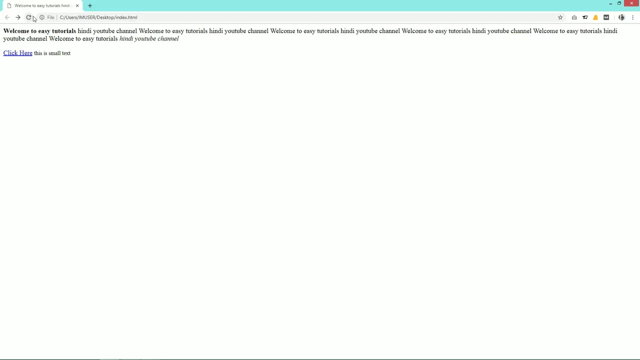 in the YouTube channel. so here I will write: I open and close and I will close it at the end. so I have added this. I tag from here to here. save these changes, reload the web page and you can see. other text are normal, but the last text which is in the YouTube channel, it is in italic font style. 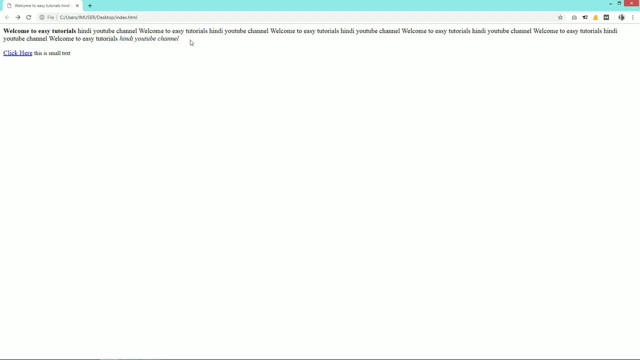 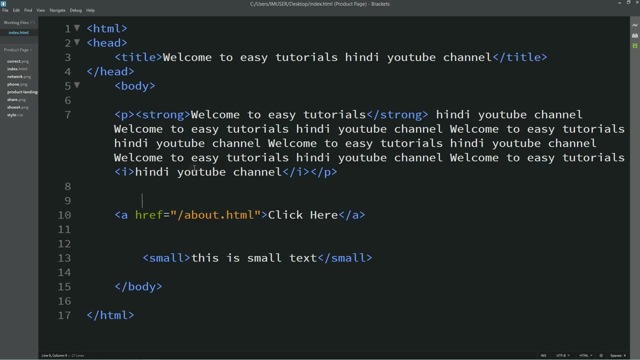 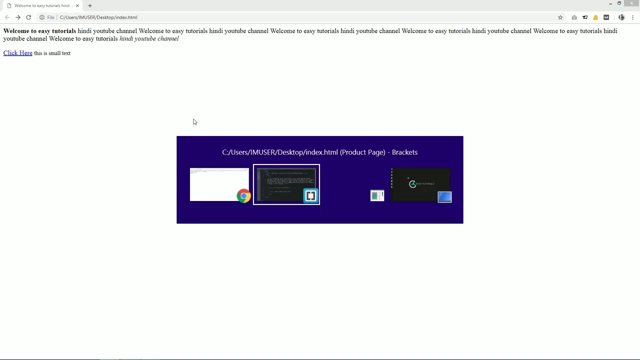 foreign is how I tag works. next we will see what is BR. so we used to write BR to change the line, to add a line break. suppose we have this text here and it is displaying in one paragraph like this, and if I want to change the line, so let me write BR. 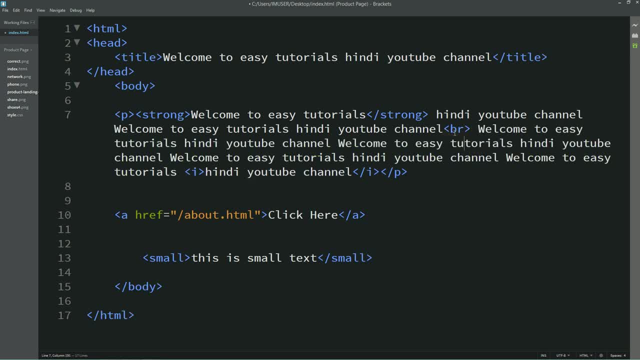 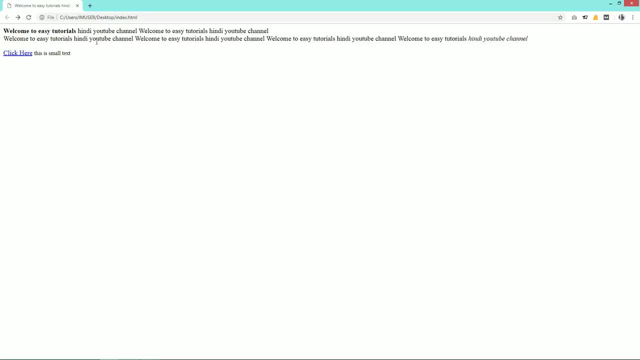 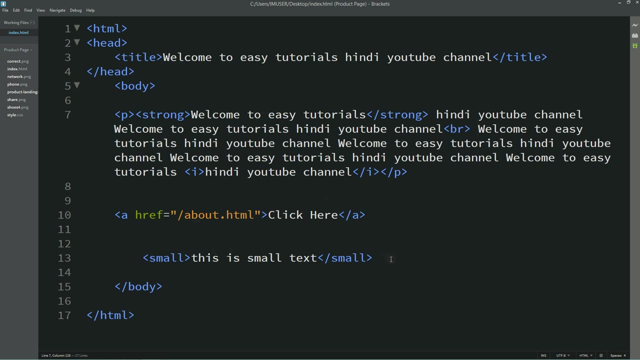 here. I have added BR at this point. save this changes and reload the web page. now you can see there is a line break where we have added BR. so this is how BR tag works. to change your line after BR, let's see what we can add- other things. so here: 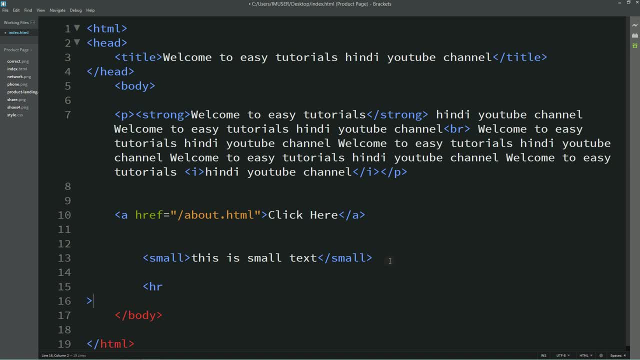 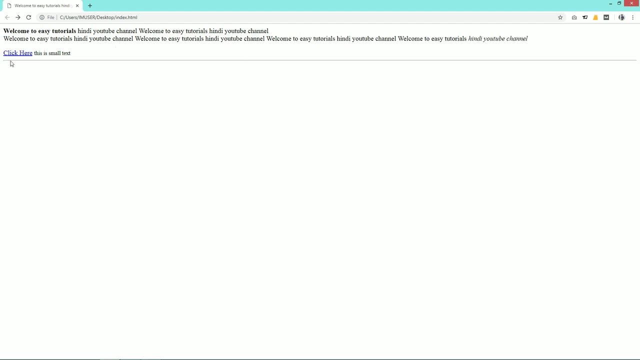 I am writing HR, so let me write it here first and we'll see what happens. simply, I'll write HR here and I will refresh the web page, and now you can see one horizontal line which is coming from left side to the right side. so this is how HR works it. 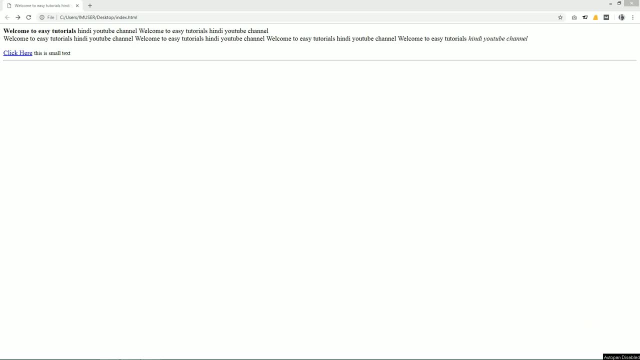 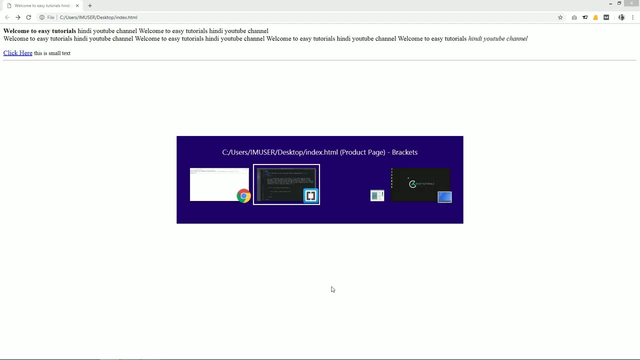 adds a horizontal line on your web page. now we'll see how we can create a form using HTML and what other things we can add in a form. so let me come back in the HTML file. I will remove everything. refresh the web page right now. you can see it is blank. 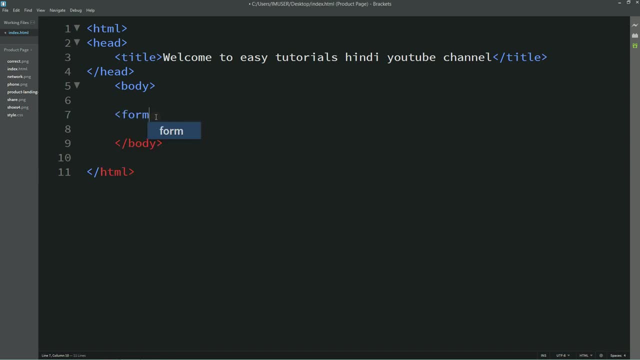 so first we will use one form to create a form. I'm not going to create form right now. first I am going to teach you what other things we can use in form. so in the form we use to add a input field like a text field and buttons. 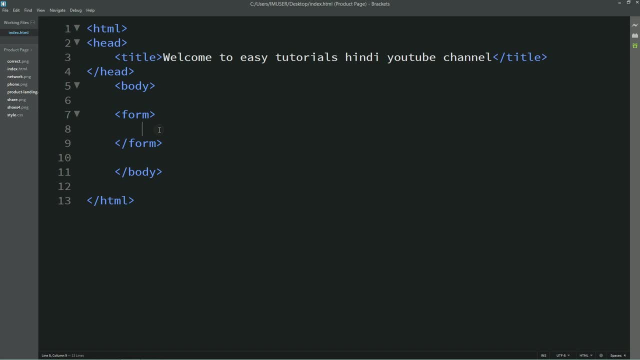 and select box like that. so let me write all the names here. one of them is input. we can use input tag to add some input fields: input field like username, input password, input email ID input fields. we can also add label to add a name of any field. that I will teach you with example later, when I will create a form. next, we can add a tag. 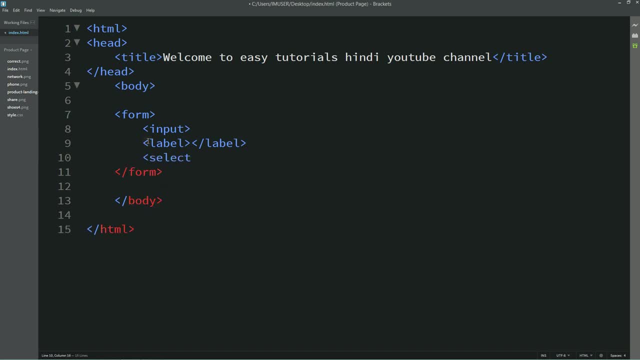 called select, and with this select we use to add one more thing, which is options, because we use this tag to create drop down in any form or anywhere. so in the drop down there will be some options as well. so that's why we use the select tag and options also. 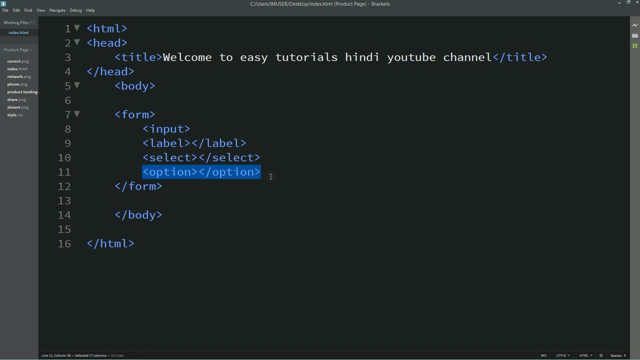 next we can use text area. suppose, if you want to add a field where people can enter a large text, a description text, then we will use this text area. and next we can use one button. you can easily understand its meaning. if you want to add something, to submit this text. 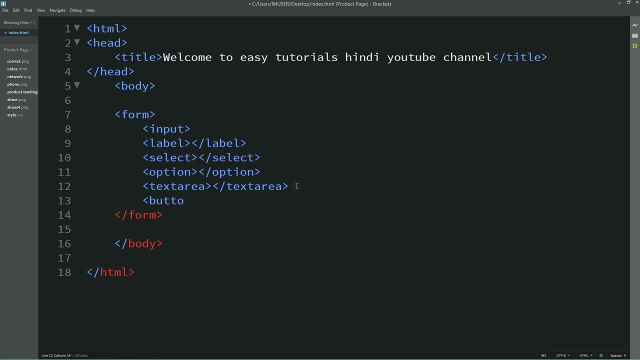 form, then we can use this button. so these are the tags that we will use mostly in our form, in our web page. so let me show you one example so that you can clear all your doubts how to create a form. so first I will start with input. 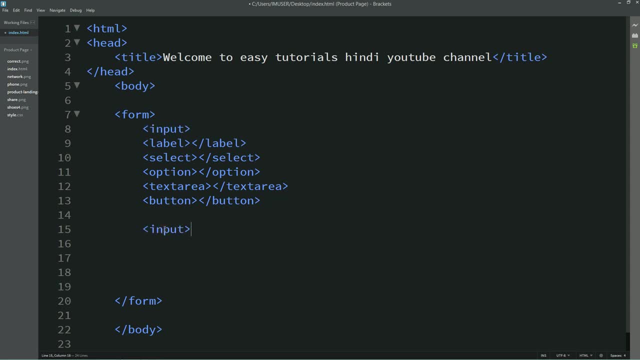 field. let me write it here. with this input field, we have to define the tag type, like what this input field will accept. it can be a button, it can be a checkbox, it can be a date, it can be a email id- like that. it can be a file also. 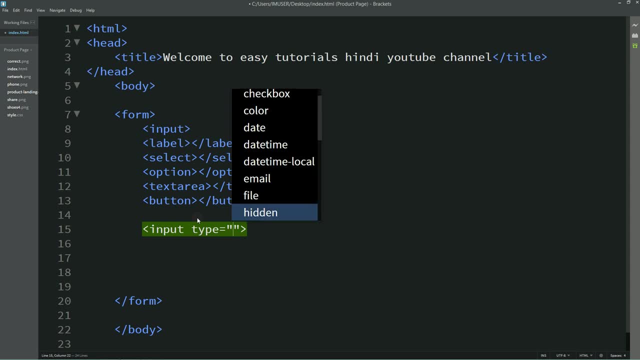 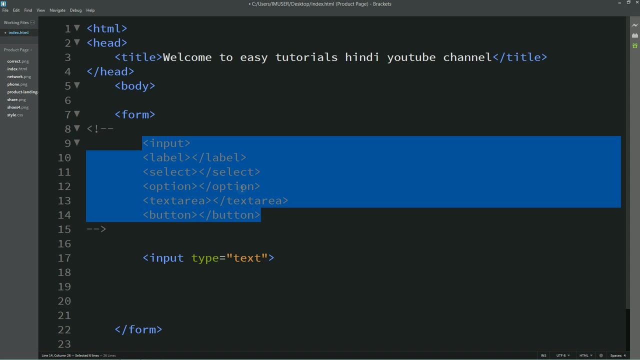 and password or number or anything. there's so many things here, so let me write a normal thing which is text, because we will create one username input field. that's why I am using input type will be text. let me comment all these things from here. to add a comment, you have to write: 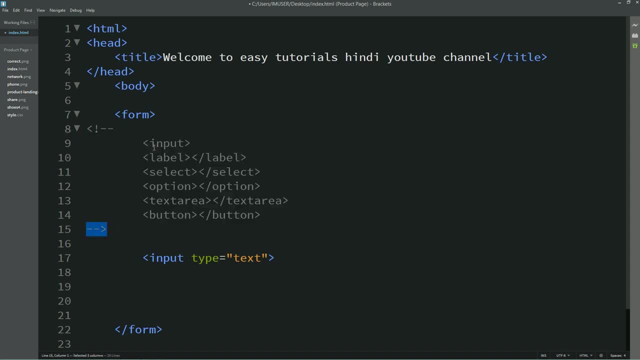 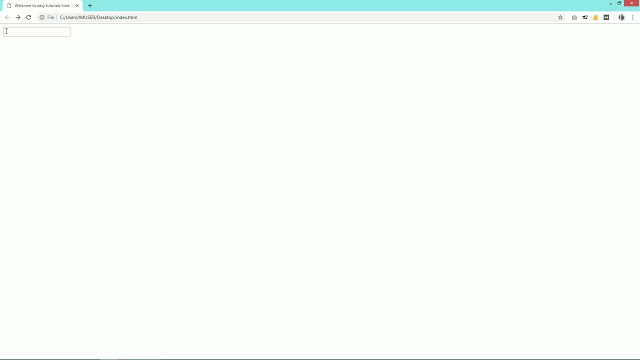 like this from a start to end. if you will write like this, the entire content will go into comment. with this code, we are displaying one input field, so let me refresh the web page and here you can say this input field. and this input field is blank right now. 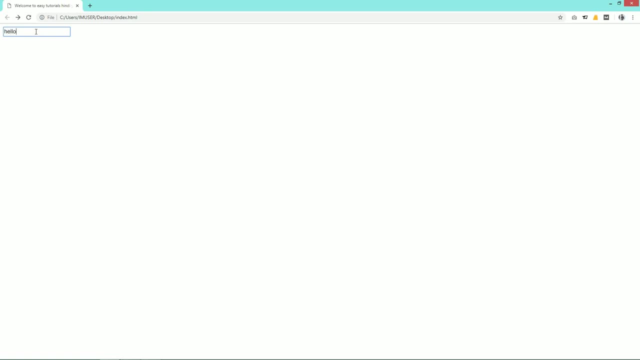 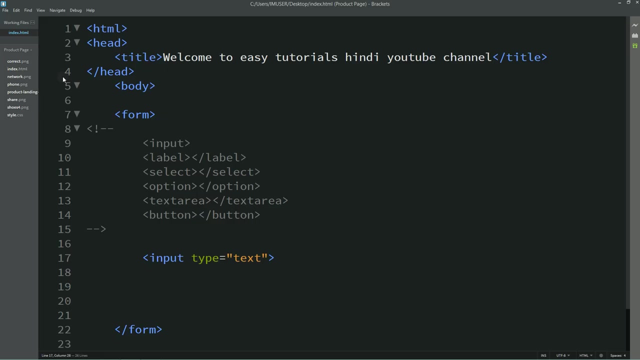 and you can type it in this input field. so this is how you can create one input field on your web page. let's come back to our HTML file and let's see what we can add here in this input field. so we can add placeholder. so placeholder will be displayed on our input field. so 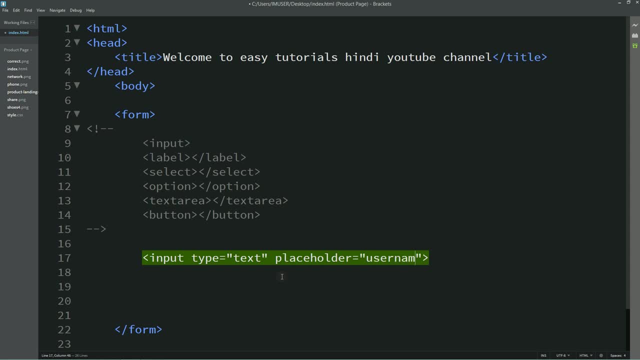 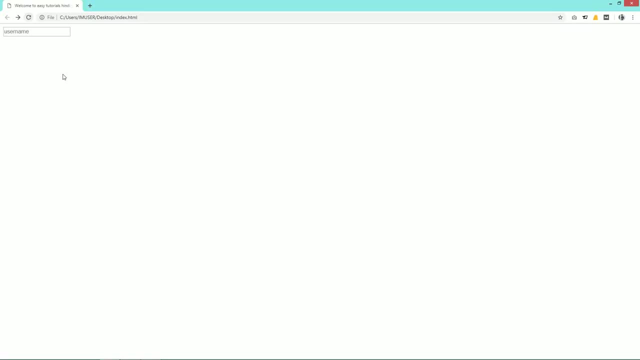 let me write one message here. I am writing username and reload the web page and you can see by default one username is written inside this input box. when we will start writing anything in this input field, the default thing will be invisible, like if I am writing anything here. you can see the username gone and 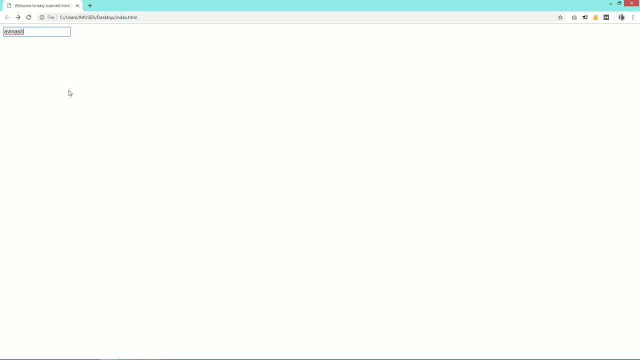 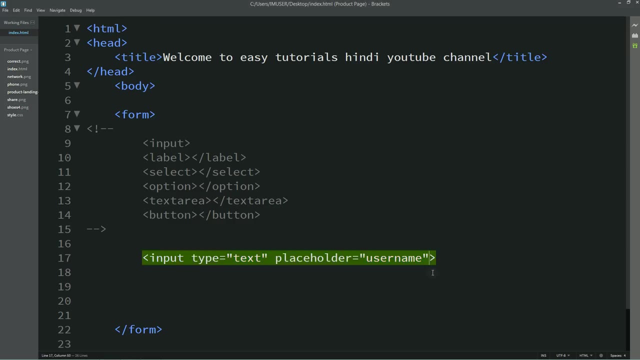 so this is how you can use the placeholder to add some text in the input field and let's see what we can add here. we can add required, so if I am writing this, required, so this input field will become mandatory to submit this form. if I will not write anything, and I will. 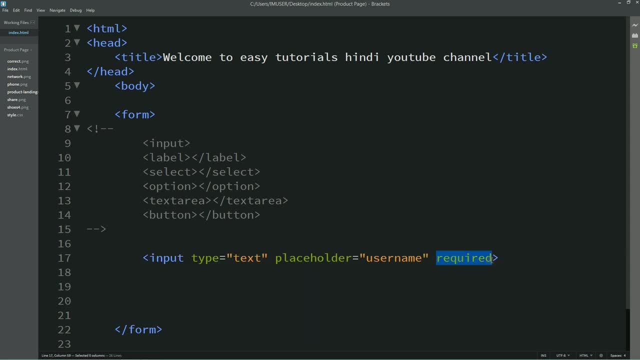 try to submit the form. then it will display a warning pop-up, like you have to enter something here- username field to create another field. I will simply duplicate it and input will be same, and instead of this type text I will write type email, because this is I. 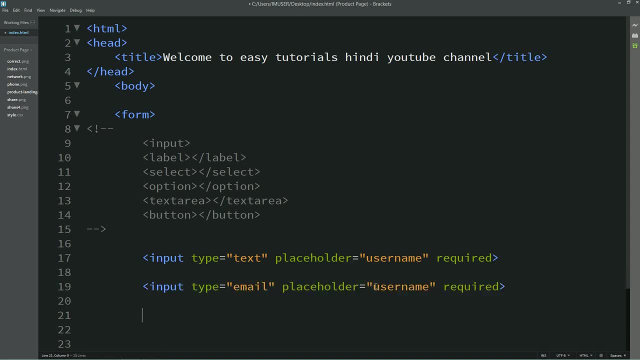 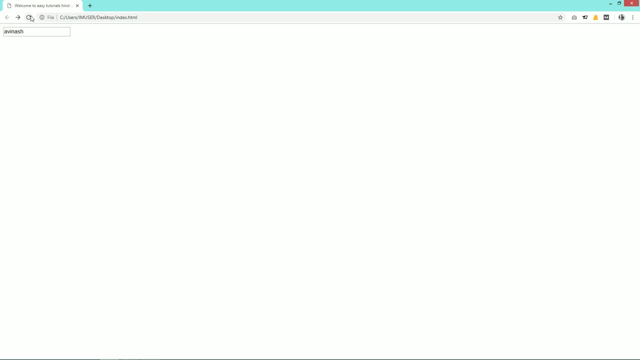 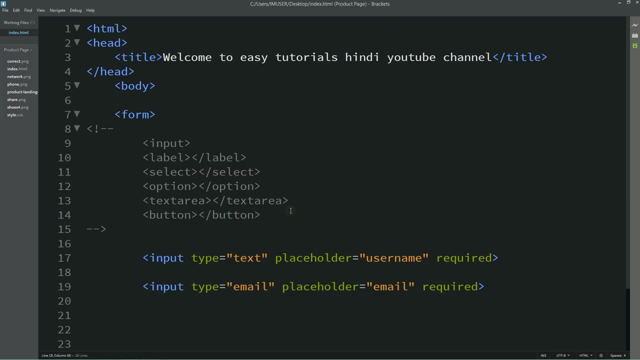 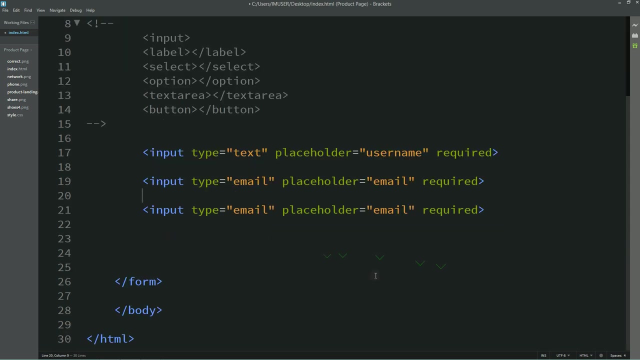 am creating email ID input field and the placeholder will be email. reload the web page and you can see two input fields on this web page, which is username and email. let's come back to the HTML file and let me duplicate it again and I will change the type: password and placeholder also password. 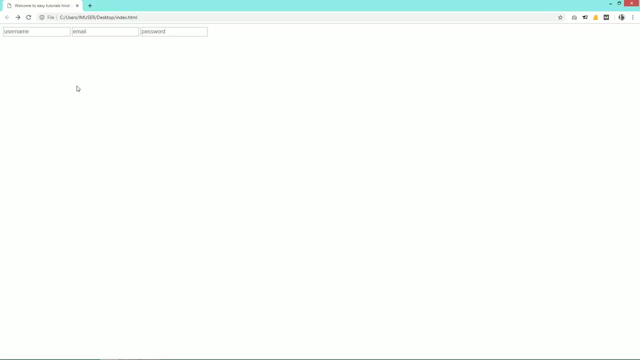 let's refresh the web page again. now you can see three input fields on the web page and three input fields on the web page and three input fields on the web page, which is username, email and password. in the username we use to write normal text in email. we will write email and the password you can see if I am writing. 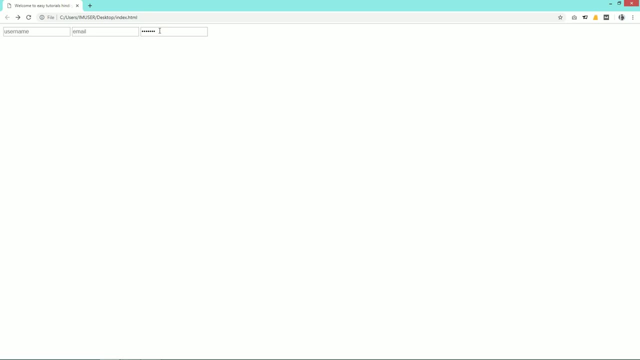 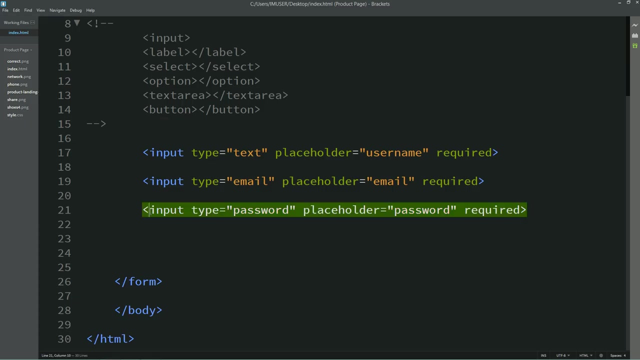 anything, it becomes invisible, as you can see in all the password field, because we are using the type password. so let me use the BR tag that we have already seen that that is used to add a password to the web page. so let me use the BR tag that we have already seen that that is used to add. 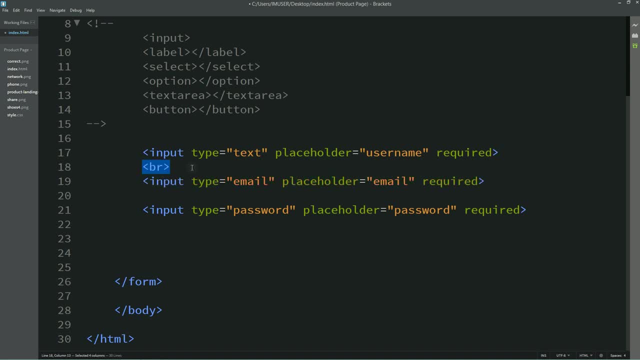 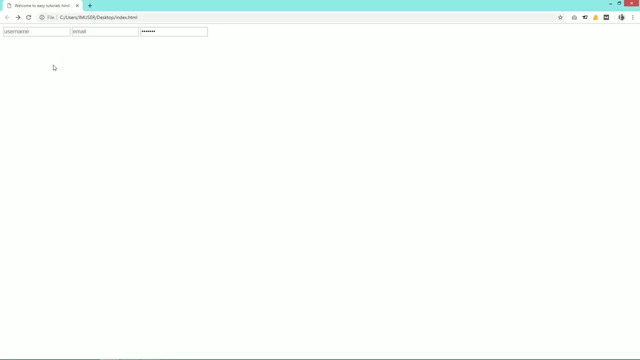 a line break. I will add it here and here. also reload the web page and you can see everything in different line. I told you we can add label also, so let me add it here and in this label I'll add one name. I'm adding username and I will add the C. 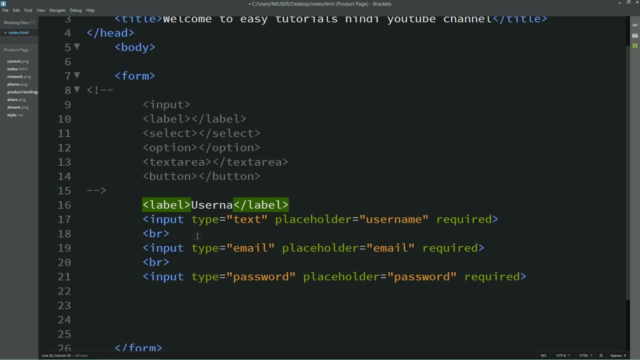 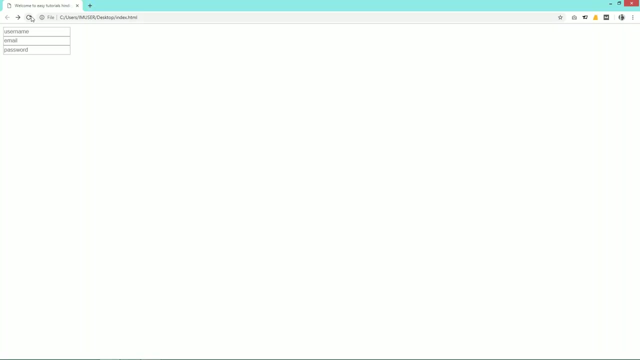 and in this label I'll add one name. I am adding username. I'll copy and paste it here. for this one I am writing email and for the third one it will be password. Deload the web page and you can see username, email and password and input fields also. so this is you how you can use the labels. let me. 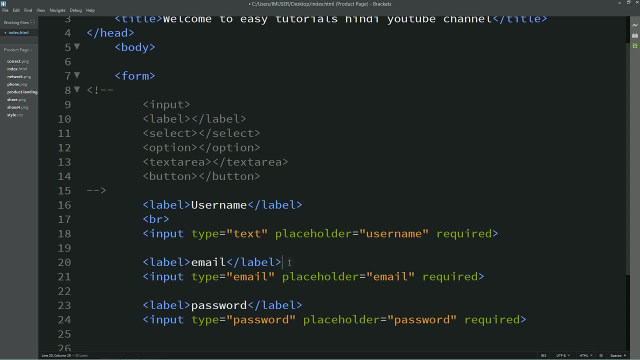 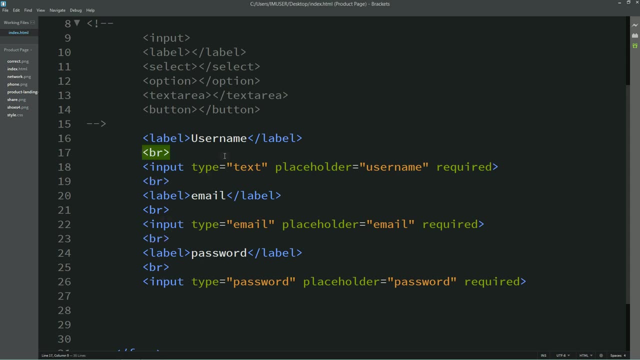 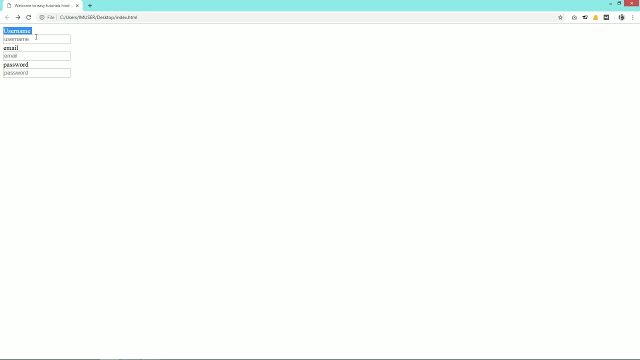 remove this BR. I will add it here. we'll add this BR after this input field. also after every content, I am adding one BR to change the line. let me refresh the web page and now it looks good. there is username, then username input field and email- email input field. and. 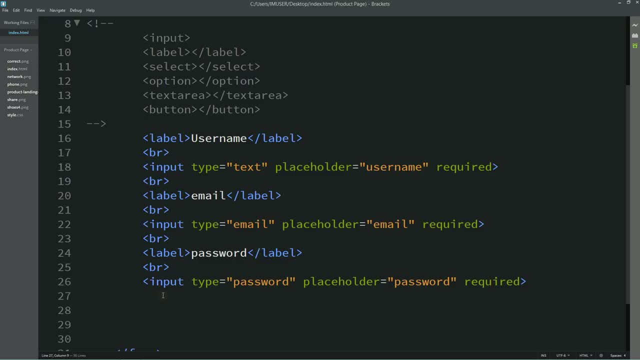 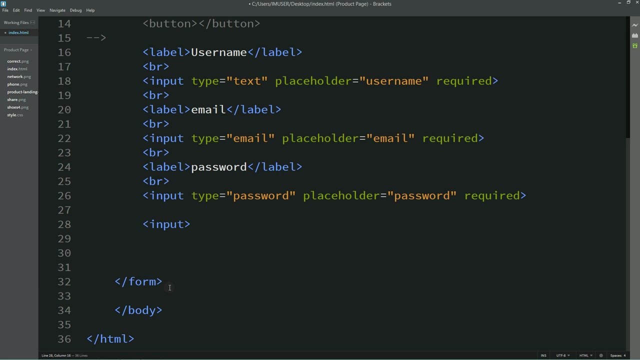 password and password input field. next we'll learn how we can add one radio buttons. suppose we want to add a general input field for that. we will use two options. so for this one also we will use the same thing: input. so I will write input, but the type it will be different. so the type I'll write radio, that's it I will. 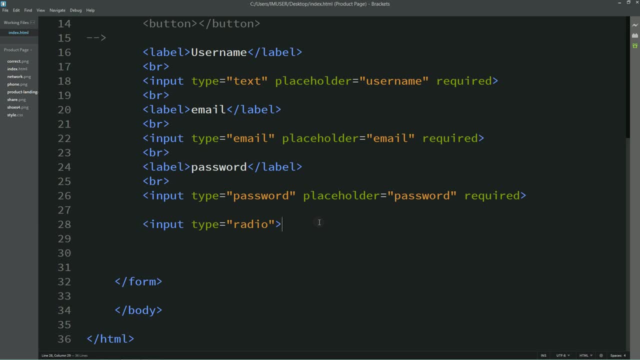 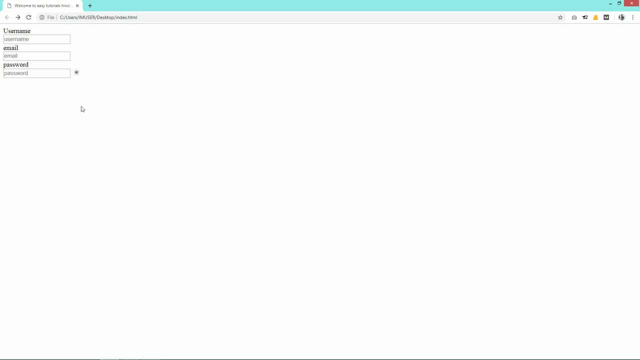 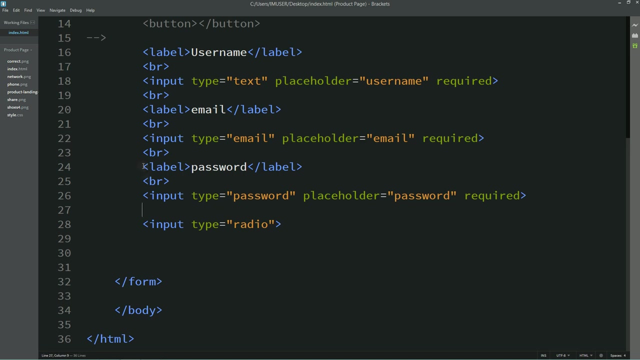 save these changes and let me refresh the web page. you can see one radio button here. you can click here to select this one. let me add one label also and set First. we'll add one BR to add a line break and let me change this label it. 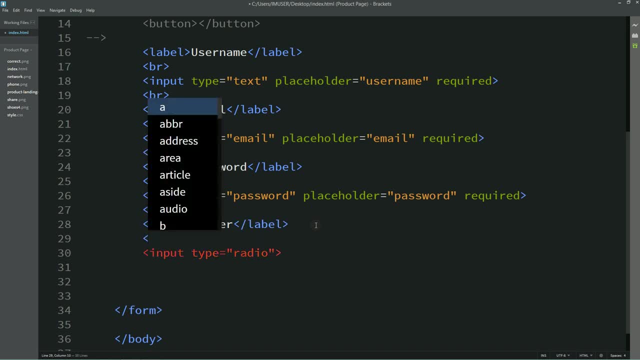 will be gender and again one BR. and like this, I will add two individualbot, then we will addize this one next time. and let me change this label. it will be gender and again one done. and let me go to lol world tab, before the button on the left, and you can see that the label and all the simply name and types unters Soldier, But Thirty curves which give you that. and like this table at our' settings, we'll also have take care of attention. and then we also have to- you also have to- 그러� Bianco and Diana session banner. that's in the description as frequency of the world too. first of all, I want to cartir series which are 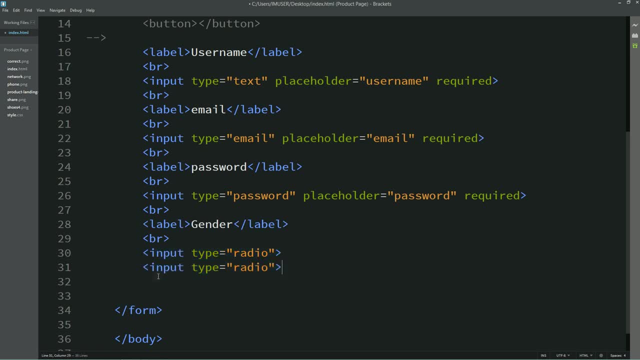 fields, So let me duplicate it. Next, you have to add one name in this input field, So let me write: one name equals gender, and the same thing I will add in the next input field. You have to write the same name in the both input field. You. 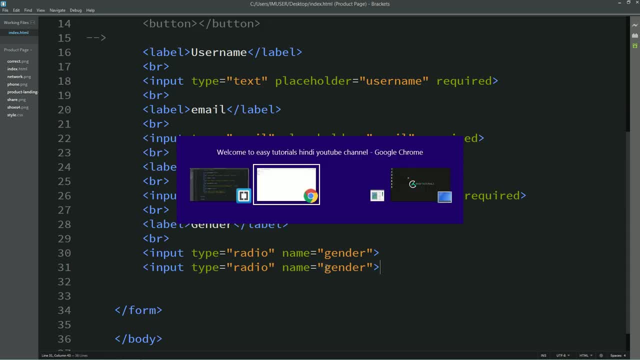 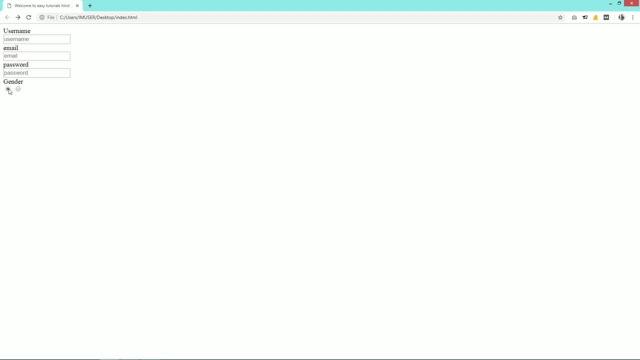 can see what will happen after using the same name. So let me refresh the web page and you can see we have two options. If I'll click here in the first one, it will get selected, and when I will click on the second one, it will get selected. 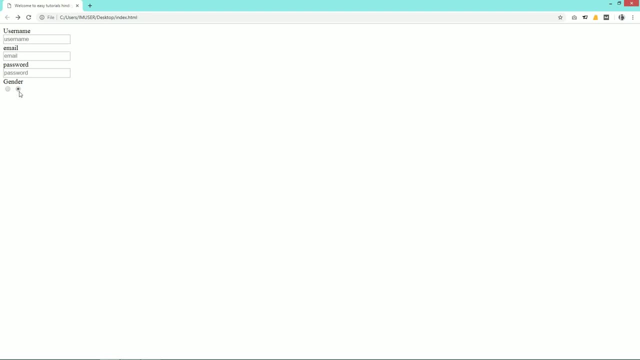 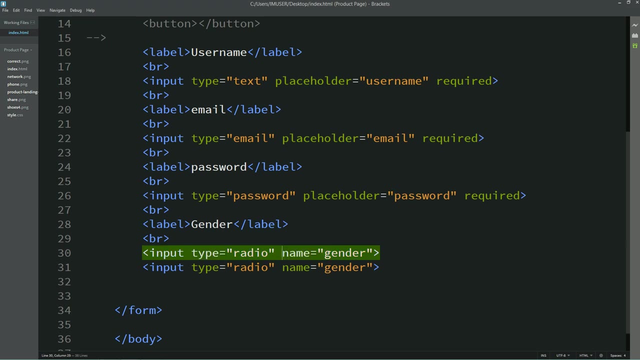 and first one will get unselected. This is happening because we are using the same name in both the input field, So only one will be enabled at once. As you can see, we we already written the same name for both the input field, So only 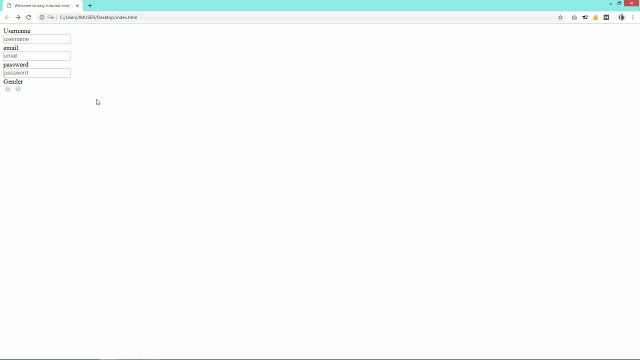 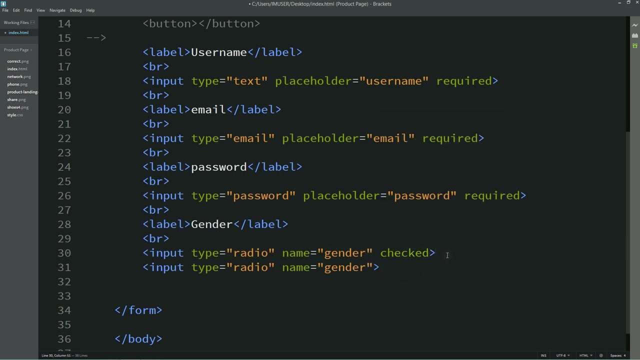 one input field is enabled for this: radio buttons, And first we'll refresh the web page. You can see the both things is blank, No one is selected. So here is one option Here: first I'll write checked and if I write checked here, refresh the web. 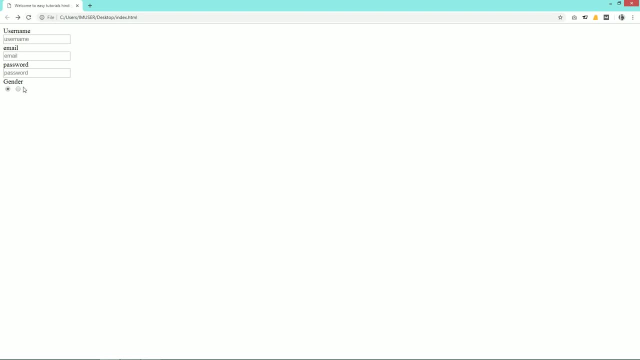 page and you can see: by default, the first one will be selected and the second one is unchecked. If I'll click on the second one, it will get checked and the first one will get unchecked. So this is how you can add radio buttons With this radio buttons, let me 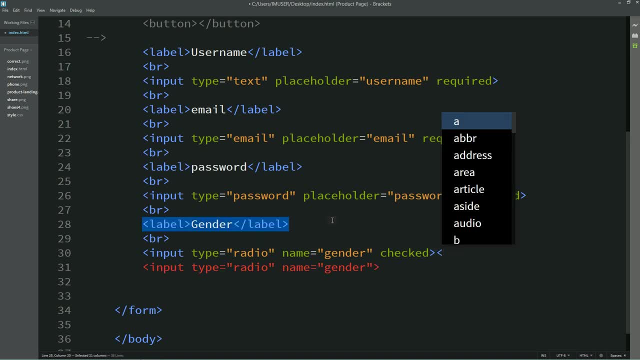 add some text here so that people can understand what this input field means. Let's come back in the HTML file. Here I'll add level and I'll write male and just duplicate it and add it into the second one. It will be female. 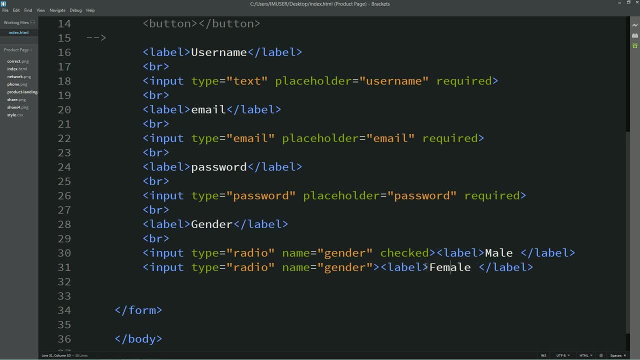 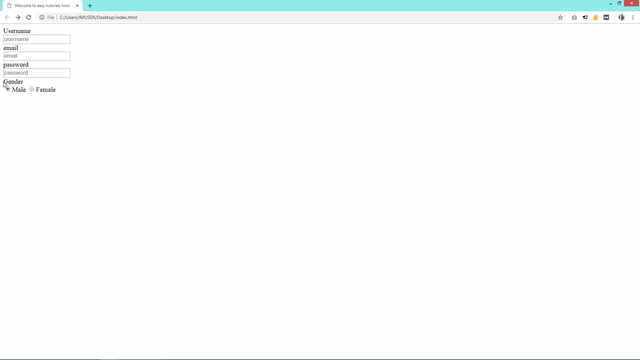 Refresh the web page and now it looks like this: Now it is meaningful, So in this case, definitely only one will be checked. Now let's see how we can add one checkbox. In most of the forms you see one checkbox. Most of the time it says: 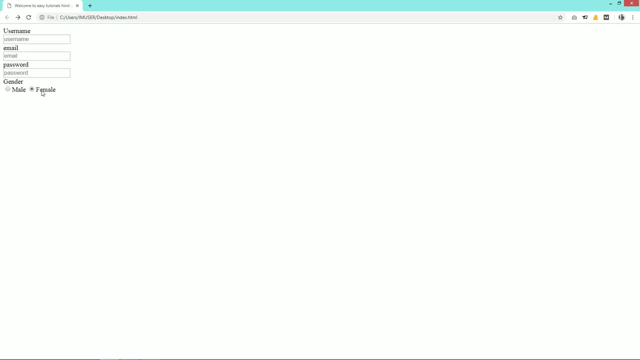 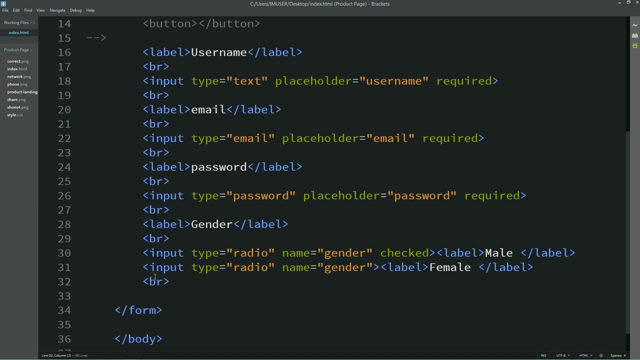 accept terms and condition like that. So let me create that one. Just come back in the HTML file and again we will use the same thing: one input field. So I will write input Before I'll write one BR to add one line break, and then I will write. 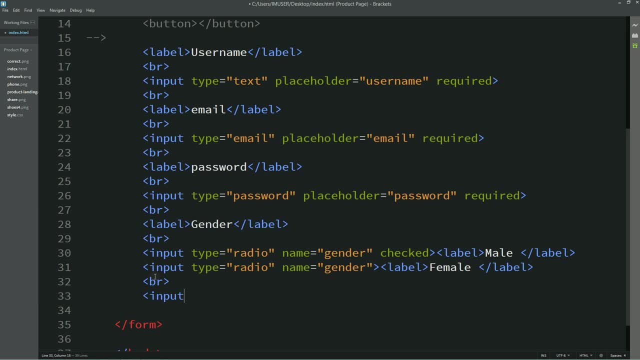 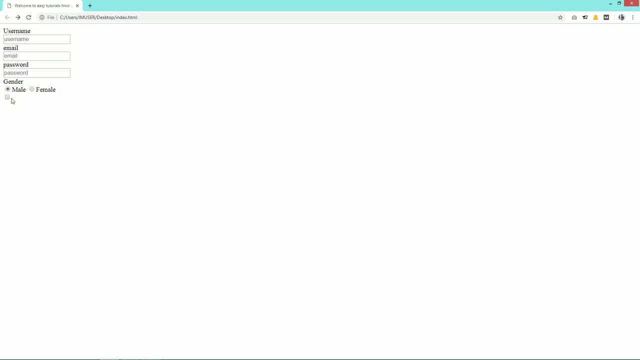 input field And this time type will be different. So here we will write the type: checkbox. So these are the attribute of this input fields. So the attribute is input type: checkbox. Refresh the web page So you can see one checkbox at this place. With this one we can add one. 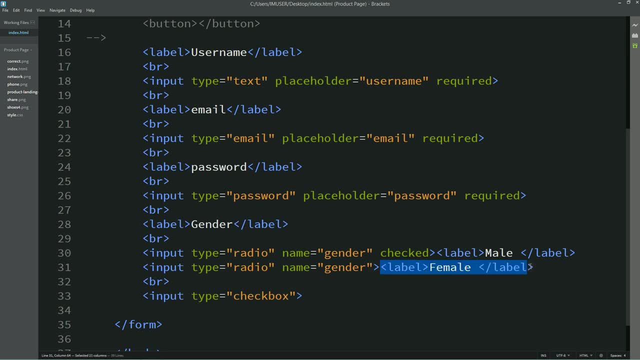 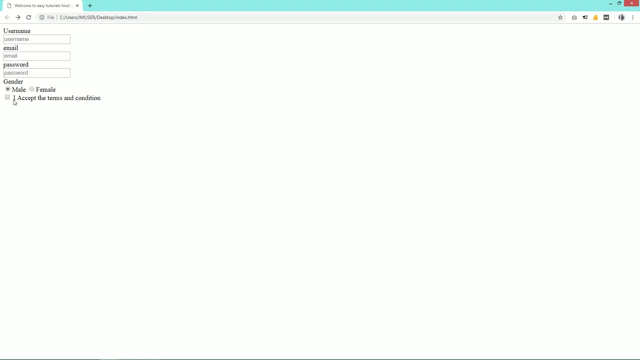 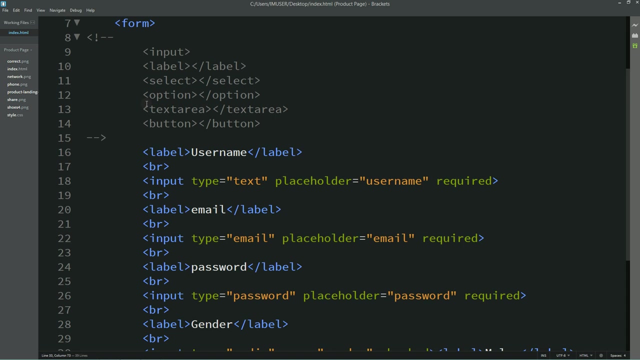 message also. So let's come back and let me copy it and paste it here. Here I will type one message. I accept the terms and condition. Reload the web page. So here we have message also and one checkbox. Next we will see text area. As I told you, we can use the text area to add a input field that will accept a long text. 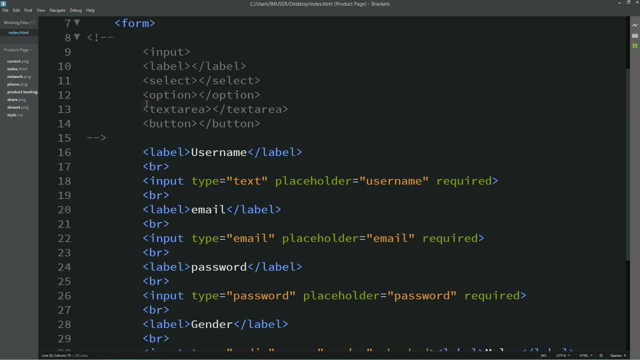 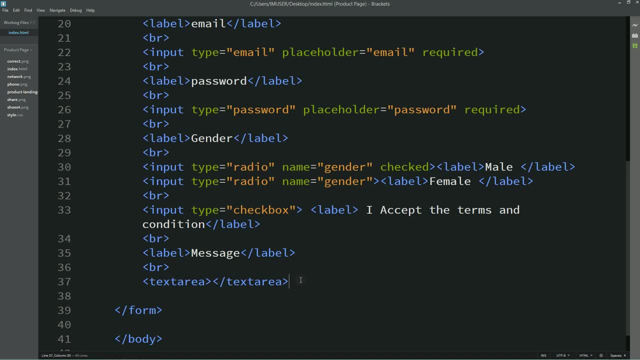 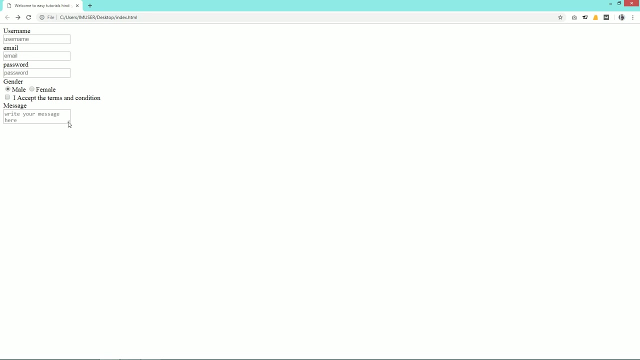 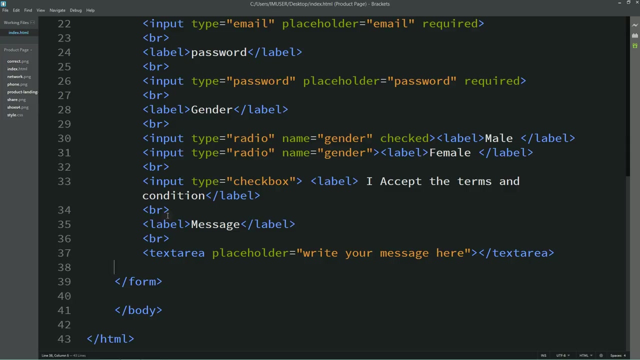 Next we will see text area. As I told you, we can use the text area to add a long text. Next, we will see text area. As I told you, we can use the text area to add a long text is a placeholder. so after this text area, let's see what we can use. we can use a: 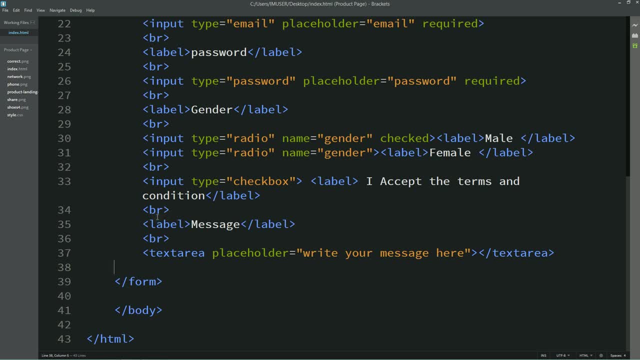 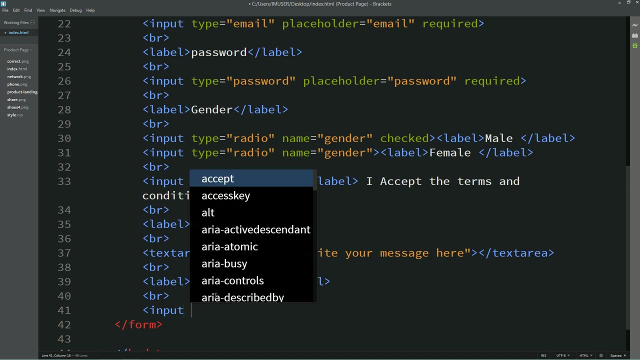 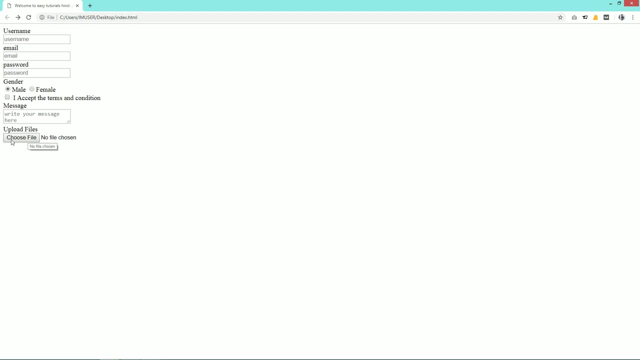 input field to upload a file. so let me write one message before that. so I'm writing one message- upload files- and after that we will write one input field and in this input type I will select file. that's it, save these changes and again refresh the web page and you can see one option to choose a file. so 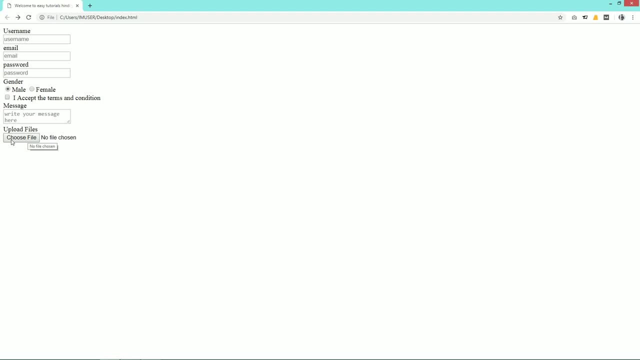 this is how people can select their file from their PC, from their computer, and upload it on this form. so you know how to create a input field for text and email: password, radio buttons, checkbox. next we will see how we can create a drop-down menu, as I told. 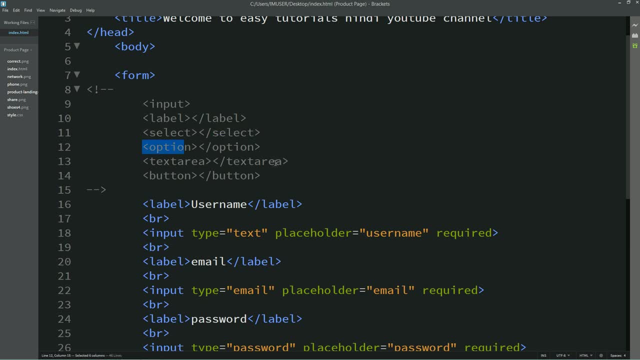 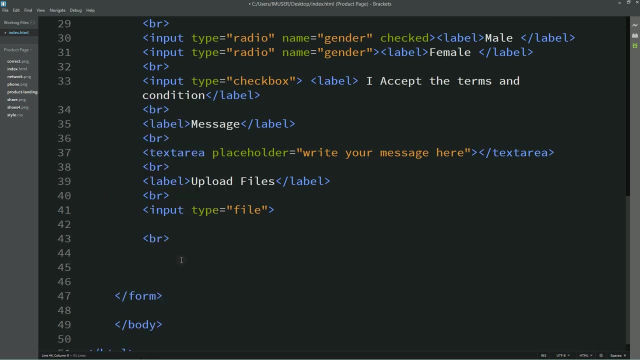 you so for that we will use the select option. first we will write one label. also I'll write BR to change the line. then we'll write label so that we can write one name for this field. so let me write the label. name will be select model. again I'm adding one BR to change the line. after that I'll write. 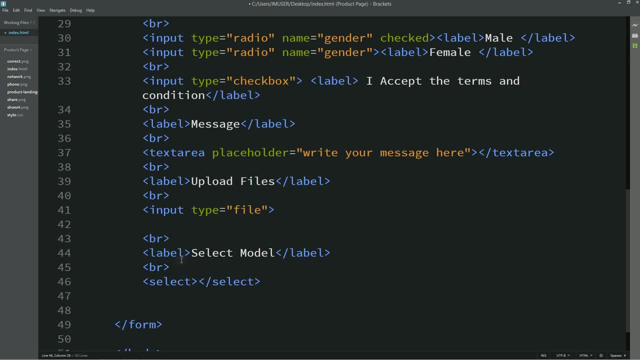 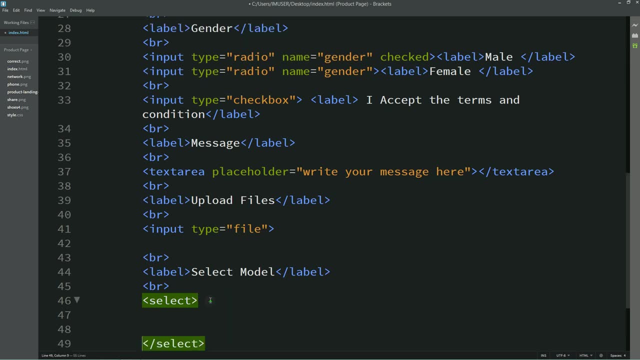 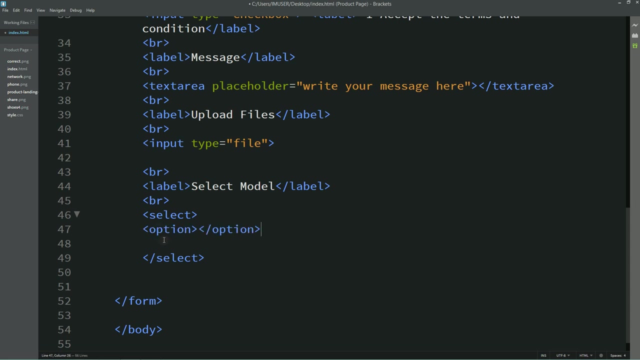 select open and closing tag and in this select tag we will add some options. so let me copy from here that I have written, let me add it here, and in this option we'll write one text. so I'll write one model here for mobile phone Redmi Note 4, duplicate this and write another message here. 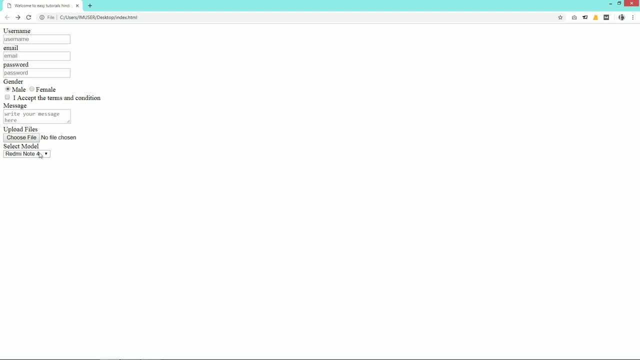 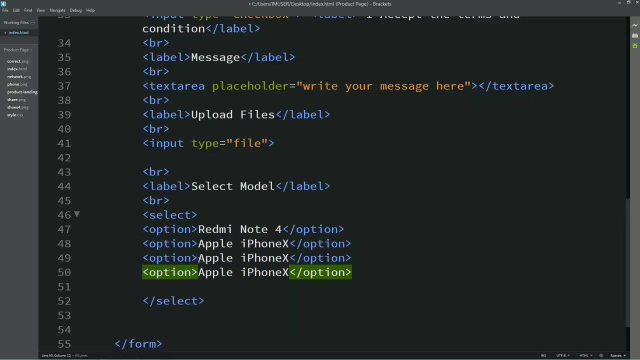 reload the web page and now you can see there is a drop-down option here you can, here you can, select any option. we have two options in this drop down. let me duplicate it again and we can add more options again. refresh the web page and now you can see four. 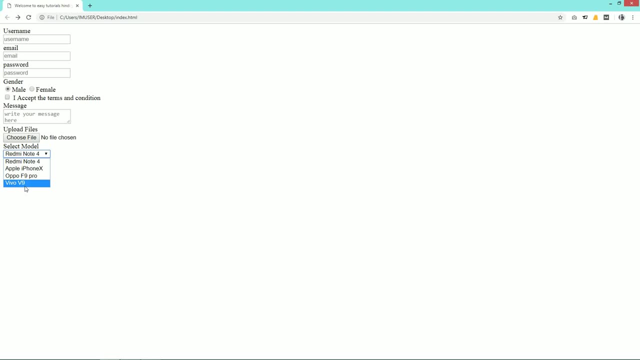 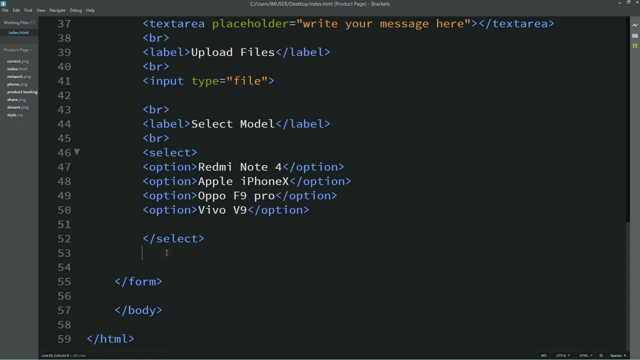 options in this select. so this is how you can create a drop-down select option using select tag and option tag. so after adding all these fields, let's see what we can add. next, we can add some button. for that we have two options. one is to use the input field and the second one is: 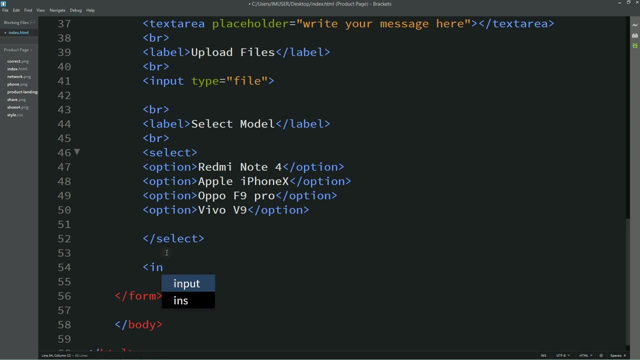 using button. so let me write the first option, which is input, and in this type we'll write submit, then we'll write value and this value will be displayed over this button as a button text. so in this value I am writing submit, then refresh the web page. 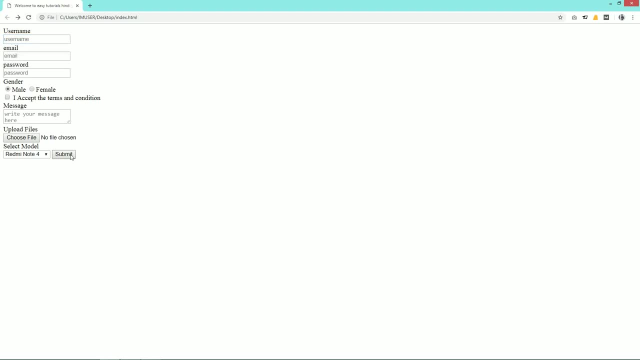 and you can see one submit button at the bottom and when I will click here you can see one message is coming. please fill out this field because I told you I have added required and if we add required, then this field will become mandatory. now we'll see the other option to. 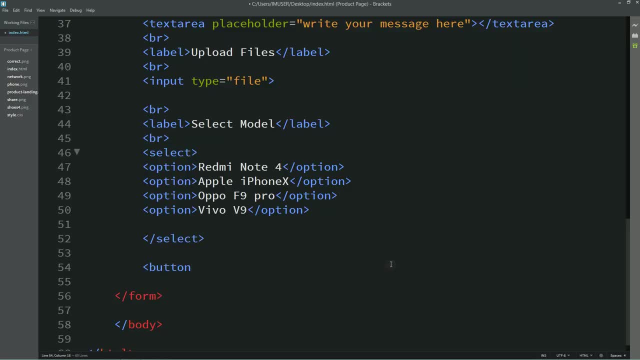 create button for that. we can use button and type. it will be submit, reset or button. it can be anything. so let me select submit and close it, and here we will write the text. that will be button text. so let me write the same thing: submit, let me duplicate it and I will change the button type: reset. so 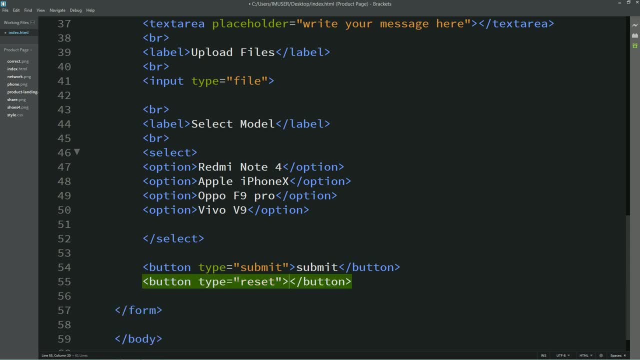 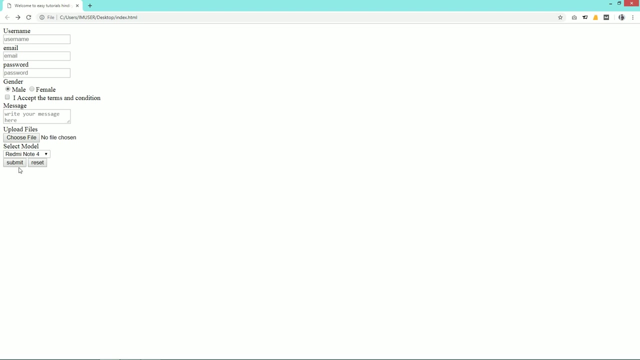 this button will reset the form. write this reset in this button text. let me add one beer to add one line. break again. refresh the web page and you can see one submit button and reset button. let me add some more space. now you can see some space above these buttons and this is the submit button and reset button. 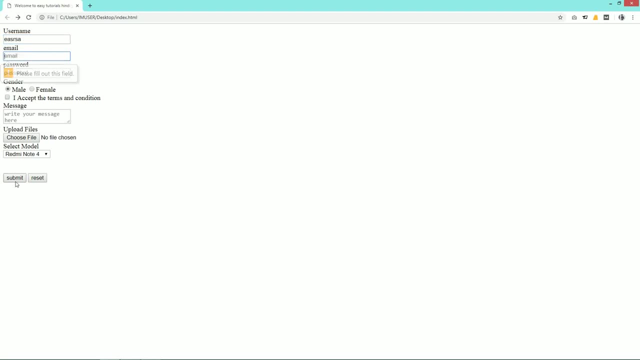 let me write something in this username and submit. you can see it is asking email field. if I'll write something in email field and submit button, then it is saying it is the wrong email format. so we have to write the correct email format. so it will be. 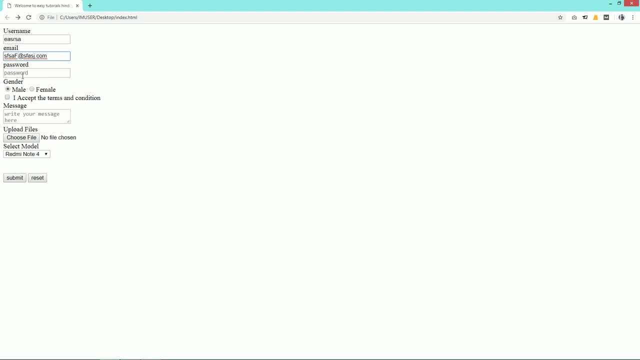 at the right something and domain name. let me click here: submit. it is asking the password. we can select the any radio button. we can select the check box. we can write the message in this field. we can upload the file or we can select because it is not required. it is also not required, so let me click on. 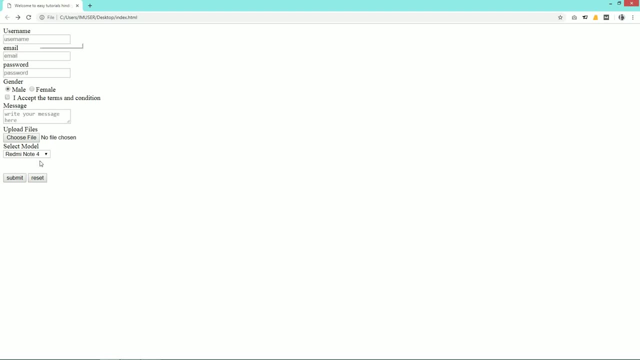 this one reset and you can see this field will become blank again because it is a reset button and when we will write something in this field and will write submit, it will submit the form. so this is the things to create a front-end form, because right now this form data will not go anywhere, because we are not. 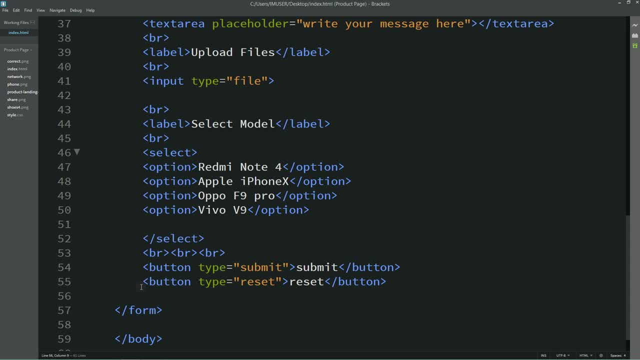 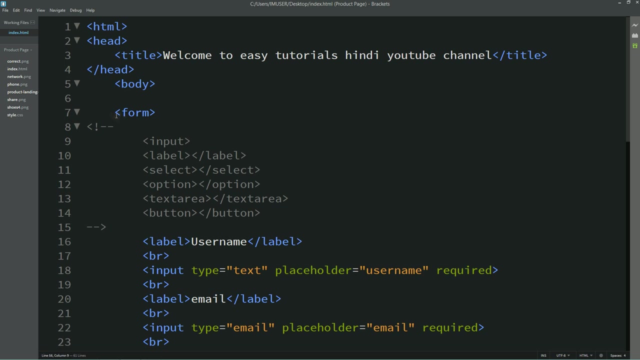 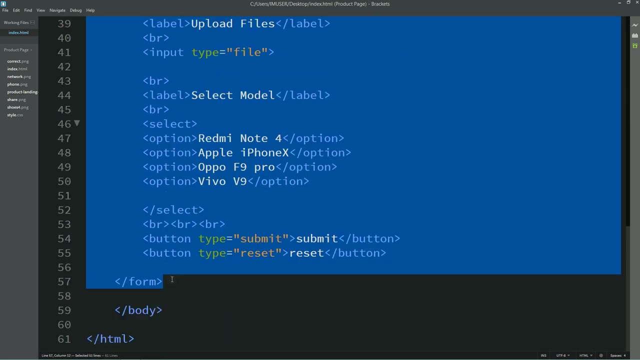 connecting it through database or we are not connecting it through any email. that's why. so this is just to create the front-end of this form. so now we know how we can create a form, how to use these input field and some other fields like text box, and we can add labels, we can add select and options. so 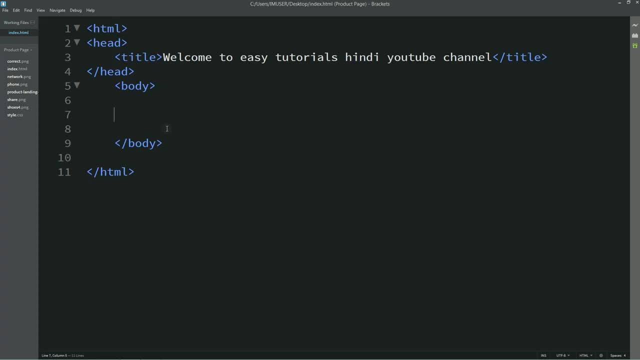 let's see how we can add list on our web page. I'll tell you two types of list and we have more options also, but frequently we use to add ordered list or unordered list. so that is only required for most of the web design. so here will. 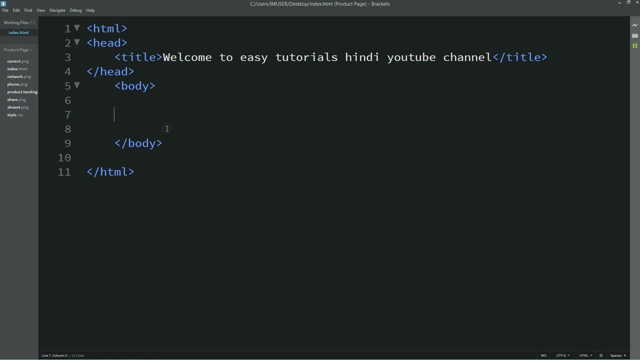 teach you ordered list and unordered list. so to create one unordered list will create a non-ordered list ul. it is unordered list tag and let's see how we can add different items in this list. for that we'll add li and in this li we can write our message. so first i'll write: welcome. 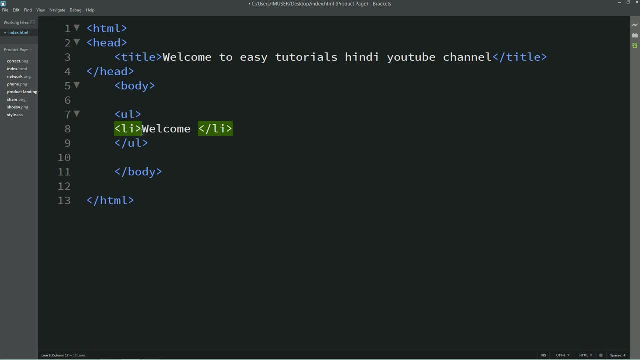 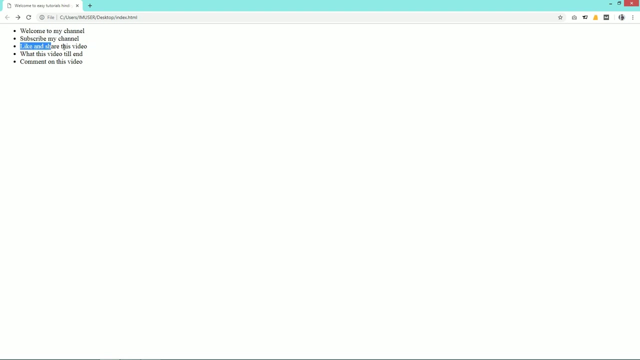 to my channel, duplicate it and change the message here. let's duplicate it again and write the third message. let's add it. one more message. so we have 4 items in this list. let me add one more. so we have five list here. now refresh the web page and see you can see all these items are coming in a list style. 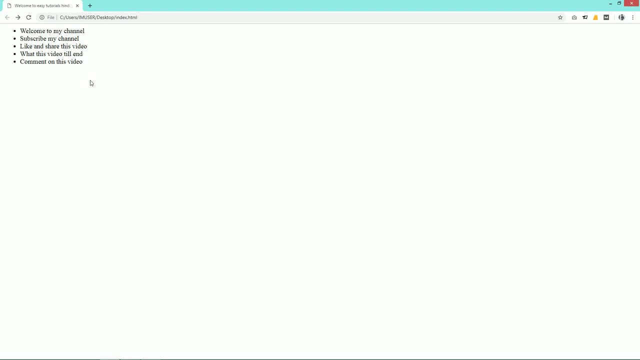 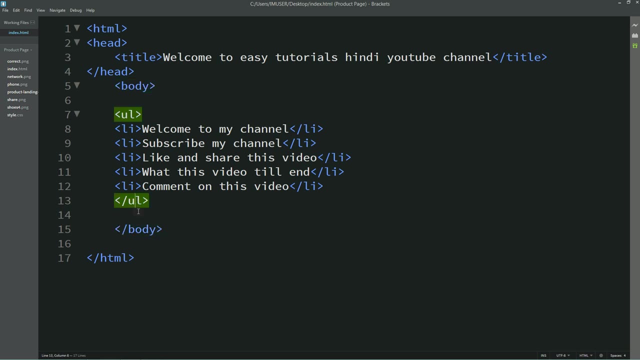 and you can see one bullet points at the beginning. so this is the unordered list. now i'll tell you how you can create an ordered list. for that we'll come back in the html file. in this tag, instead of ul, we will write ol and here also ol close. so this will be ordered. 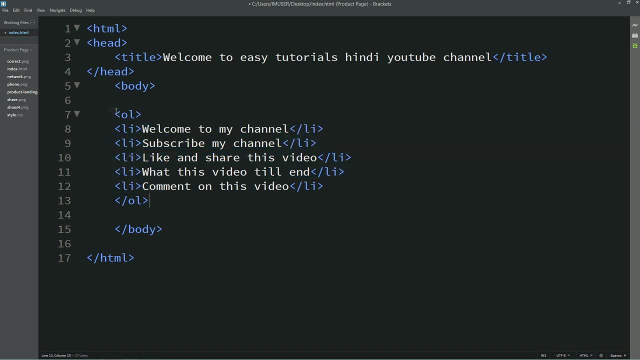 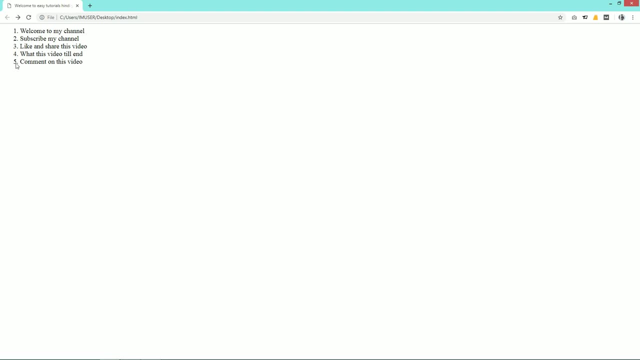 list. everything will be same. just change this one and save these changes again. refresh the web page and now you can see the order also, which is 1, 2, 3, 4 and 5. so this is the ordered list. this is how you can create two types of list on your web page using html. i will teach you more. 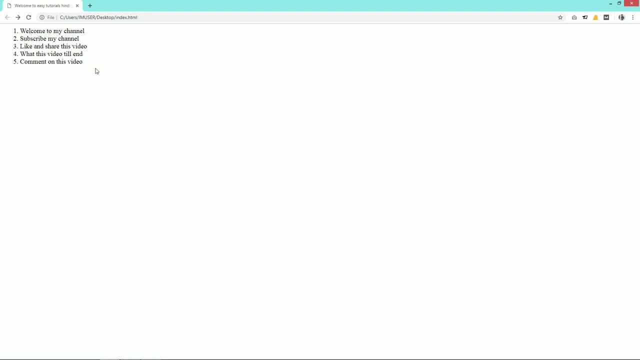 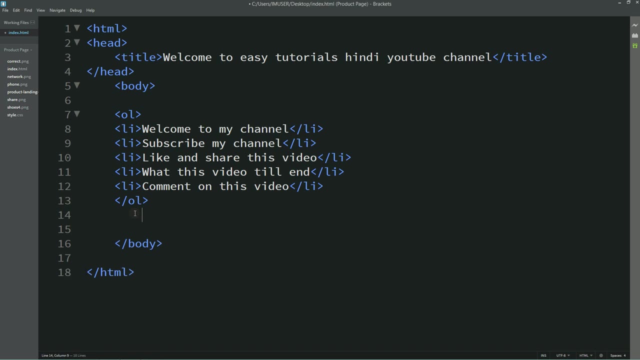 things like how you can create a list on your web page and how you can create a list on your web page and design these list when we will go for the template design next, we will see how to create a table on html page. so let me add some space here and here to add some line break, so to create a 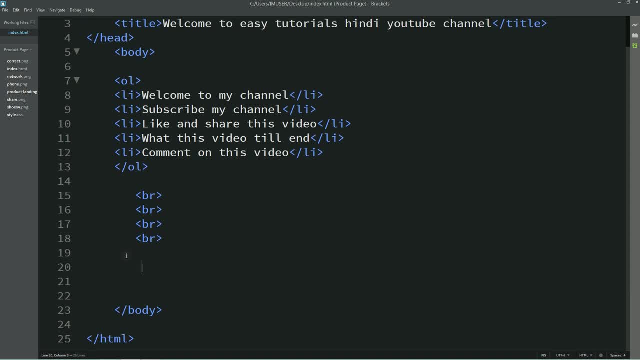 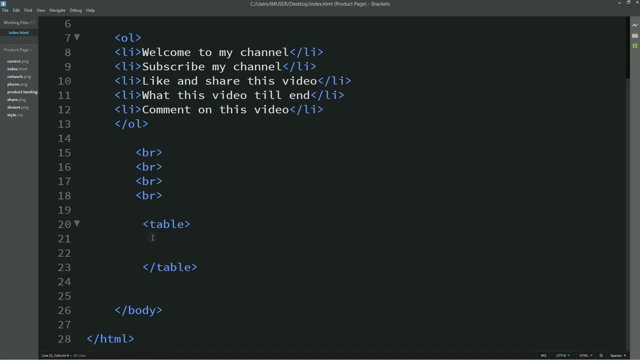 table. we will use one table tag, table open and closing tag. so in table usually we have some row and column, so we will discuss about table row and instead of column we will create table data. that will be table cell and in that table cell there will be. 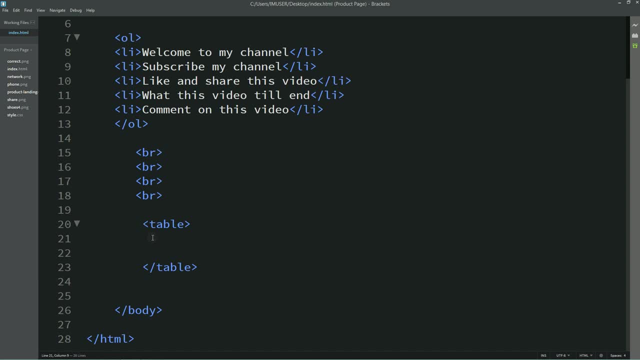 table data. so first we will create table row. for that we will use the tag tr, so this will add one row in the table. and after creating this row let's see how we can add data in this row. so for that we will use td and in this td i will write one message. it is hello, duplicate this and write some other message. 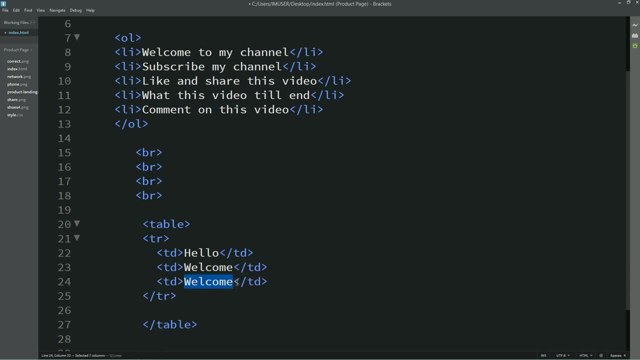 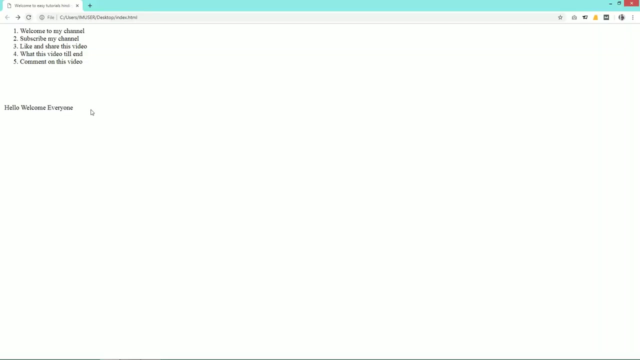 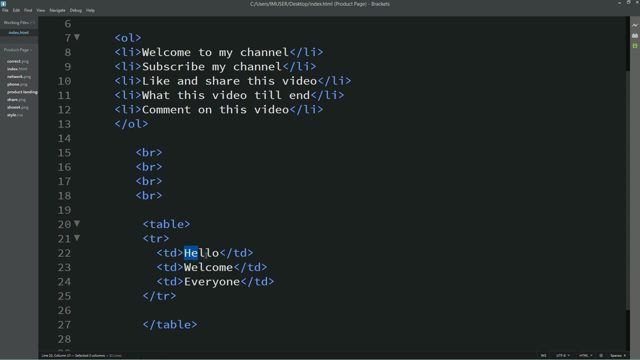 so let me duplicate it again and we'll add one more message here. let me refresh the webpage and you can see everything is coming in horizontal line. first one is hello, then welcome, then everyone. So let me remove this and I will write it here: number. and in the second place I will 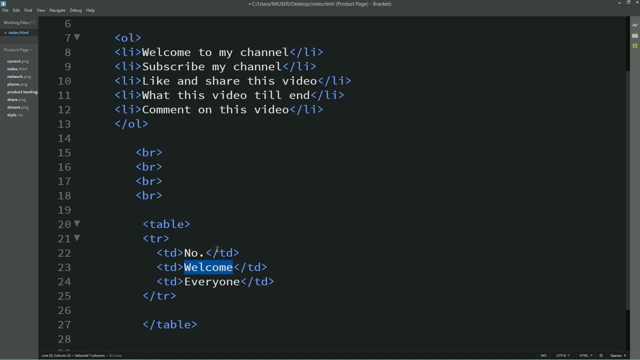 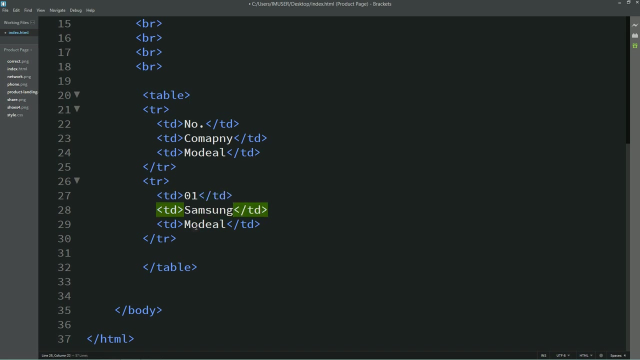 write company and next I will write model. Now we will duplicate this entire row, which is tr, so just select this and press control d, and here we will write number 01. here we will write the company name and model. Let me duplicate this row again, so this will be 02 and company name here and model. 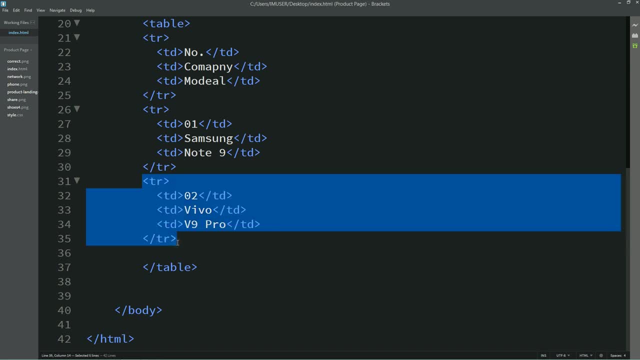 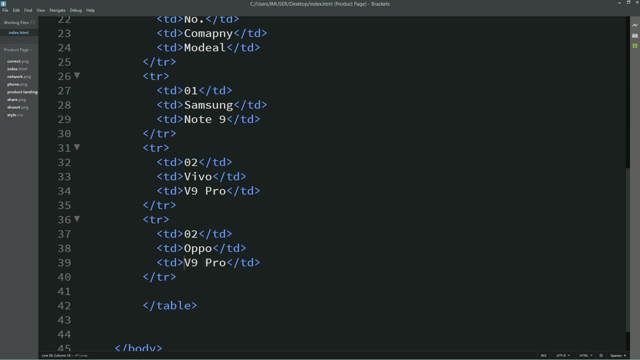 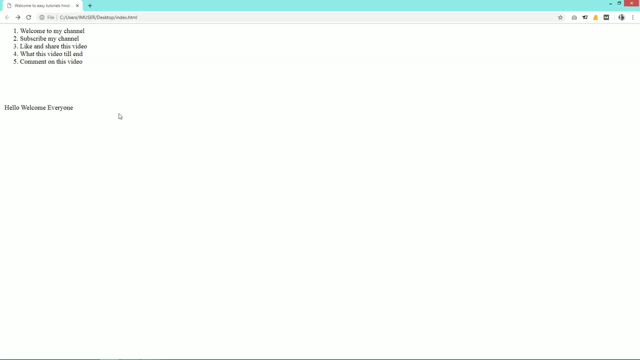 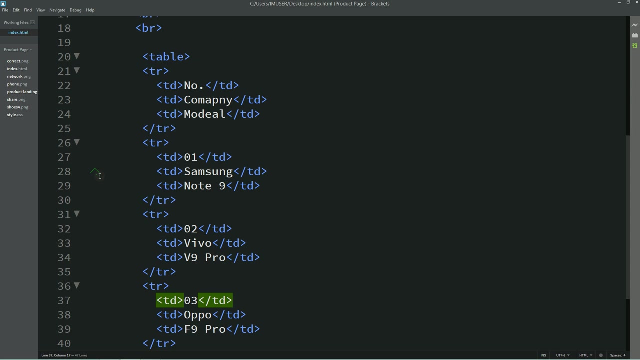 Let's create one more row and we will add some different data in this row. Let me refresh the web page again and you can see it is coming in a table format. There is different model for different company and this serial number. Now, if you want to display the first row as a heading for that, just come back here. 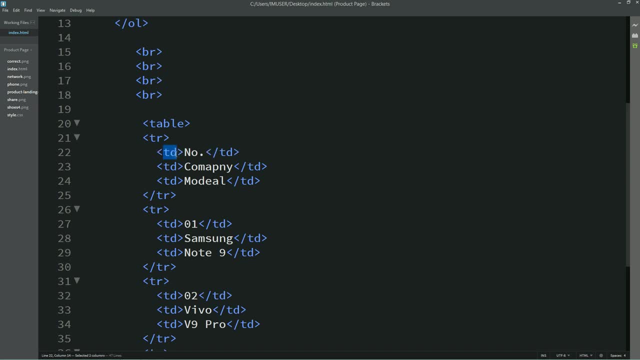 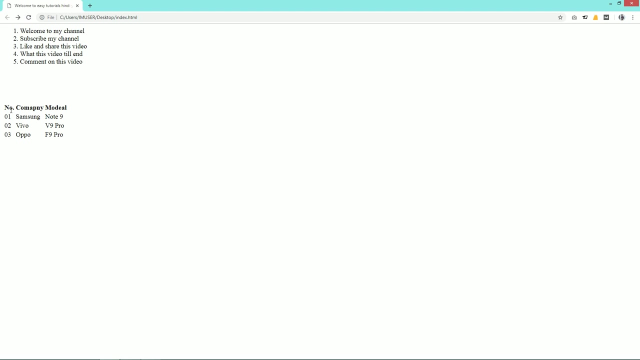 Here we have added td, so instead of td we will write th, So it will be table head. So for the first row we are adding th and for the other one it is td. table data. So the first row. you can see it is in bold. 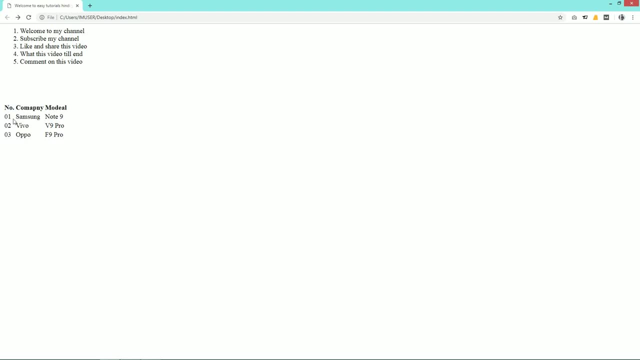 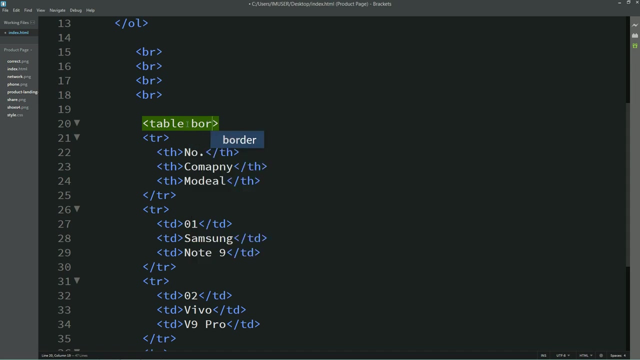 So that this table looks better. So now let's see how we can add border in this table. So here you can see the table tag that we have written here. So in this tag we will write: border equals 1.. Save these changes, refresh the web page and you can see border around every data in this. 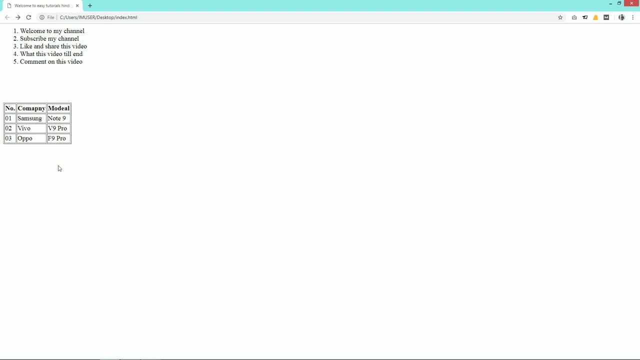 table. So this is how you can use the table data table head and tr and table to create a table on your html website. So here we have added th. So this is how you can use the table data table head and tr and table to create a table. 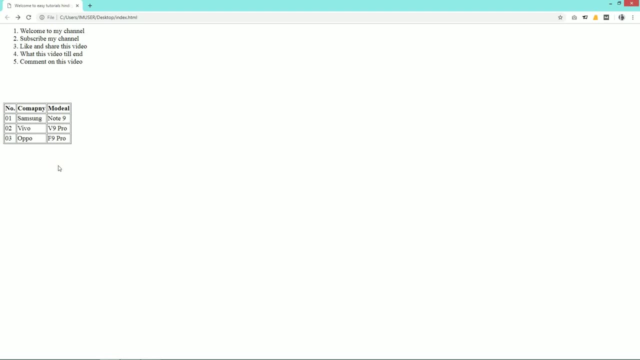 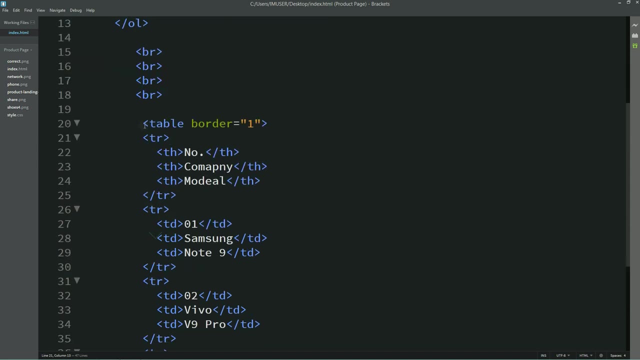 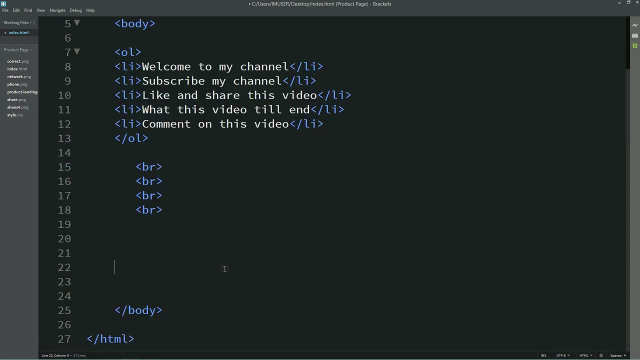 on your html website. Now let's see how we can add a image on the html website. That is very easy. So let me remove everything And to add one image we will use the tag img, and with this img we have to give the source. 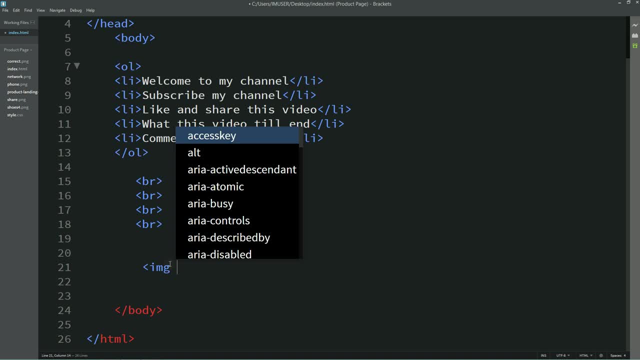 of image file. So for the source we will write: src equals. If your image file is on the same folder where you have kept your html file, then you can simply write the image file name, And if it is in some other place, then you have to write the complete file path, like if it. 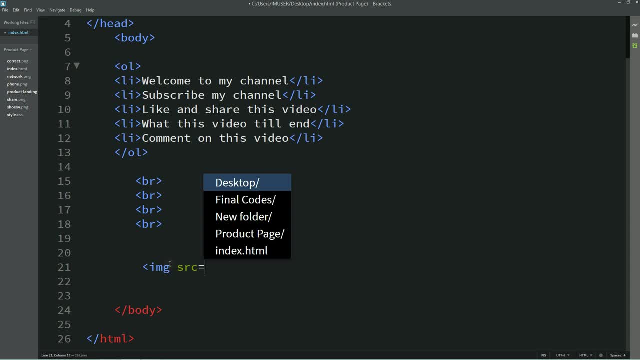 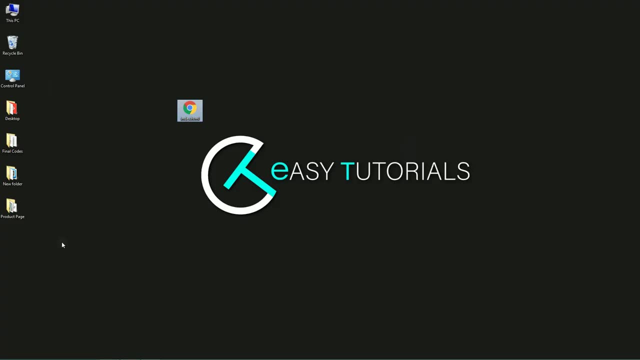 is in some folder after this folder, then you have to enter the folder name, then slash, and your image file name. So let me create a new image file name. So let me create a new image file name And let me come back and in this desktop you can see i have this html file here and i dont. 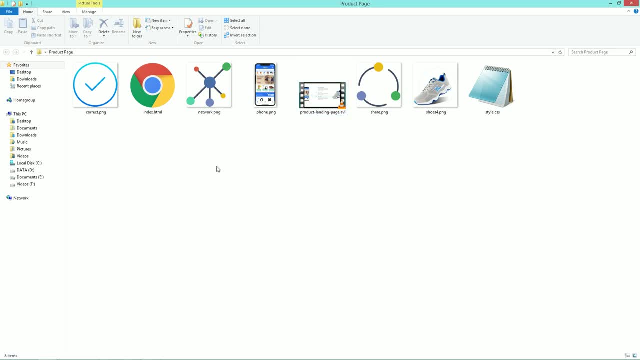 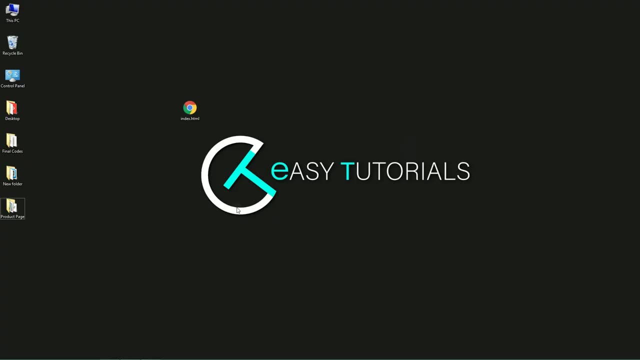 have any image here, So let me bring one image here. so i have this image. i will add it on this desktop So you can see. right now our html file and the image file are both on this desktop. It is in the same folder, right? 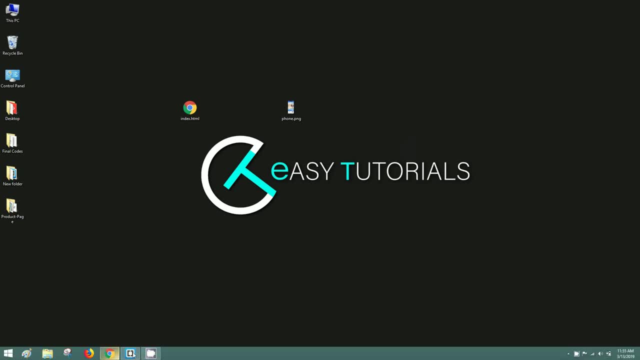 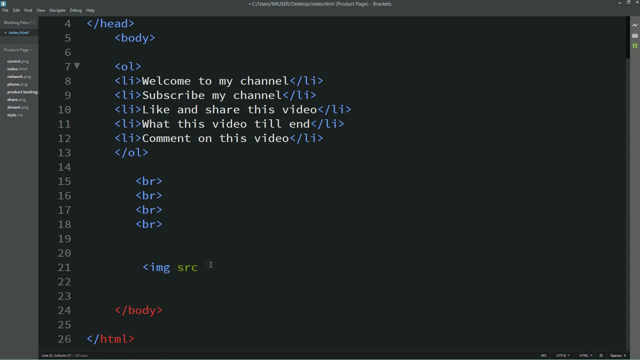 So that's why we can simply use the file name without writing any folder name. So the image file name is phone, So let me write it here: source equals phone dot png. This is our image name. Then close this tag and reload the webpage. 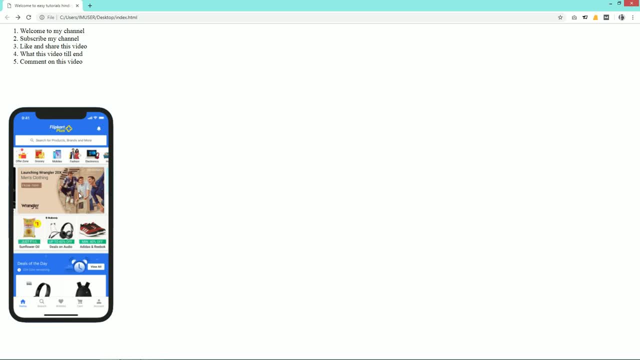 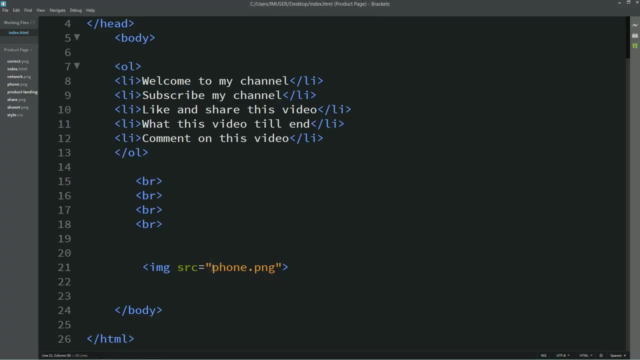 So you can see this image on this webpage. So this is how you can easily add image on your html file using image tag, I mean img tag. So suppose you have this image in other folder, So then you have to go to another folder. 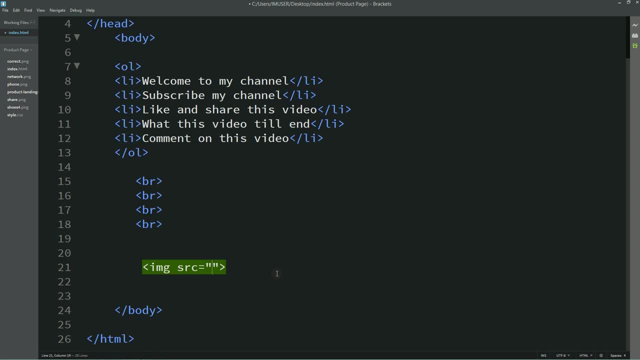 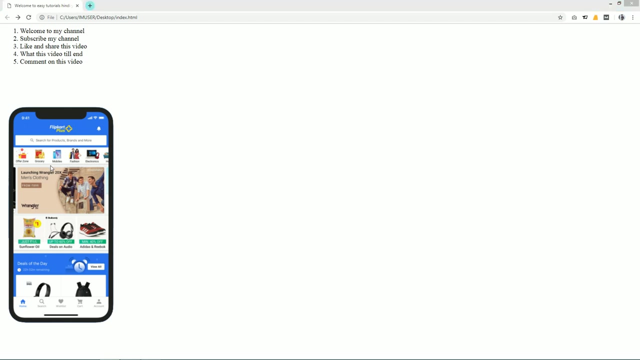 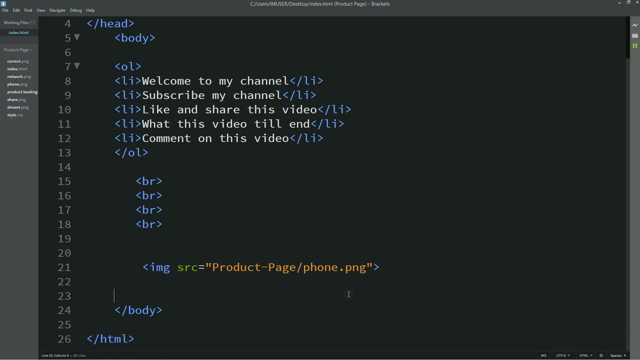 Like: if this image in one folder- This is the folder called product page- Then write the folder name, Then write slash, Then image name. Refresh the webpage and you can see it will be displayed on your webpage. So you have to enter the correct file of your image in this html file. 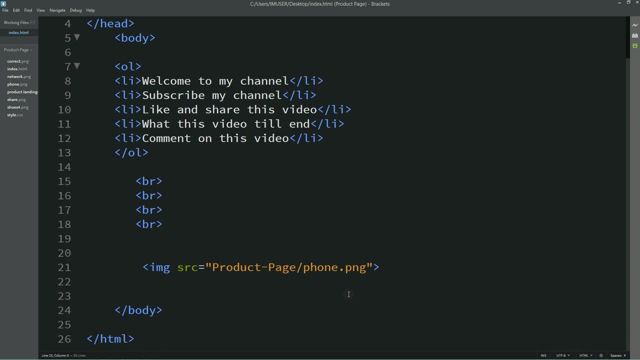 Till now, we discussed about html tags that will be used for creating webpage and creating website In further videos, But before that, we will learn more thing, which is css. We will use the css to design our webpage. What are the properties in css? 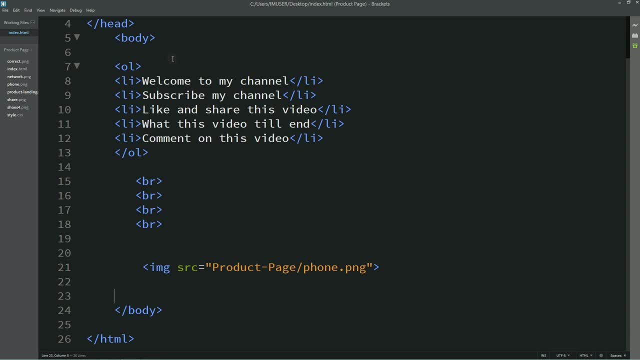 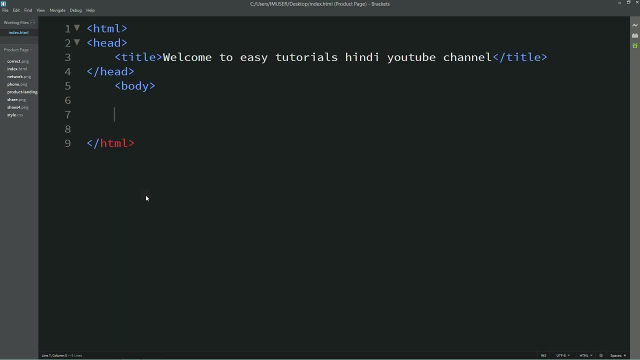 We will learn all those things. So first let me remove these things. I will remove all the content. Don't remove the body. We will write all things in the body tag. Let me refresh the webpage And you can see this page is blank right now. 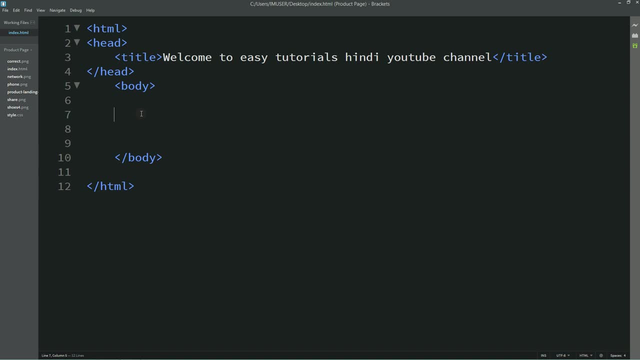 So you know css we use to add styling for our html elements. We need to design our webpage so that we need css. To add css, we have three options. First option is we can write the css inline. The second option is we can write the css as internal css. 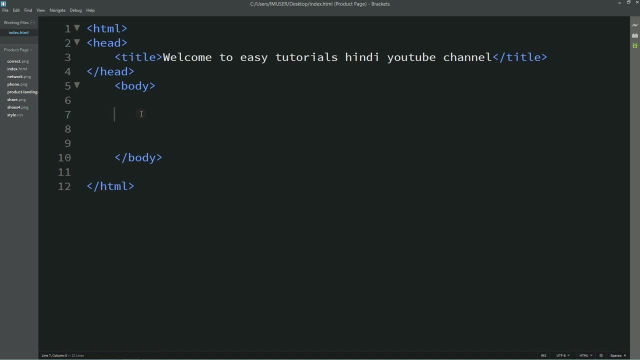 And the third one is external css. So what are all these inline css? I will show you everything with one example. So to show you, I will write one normal html code here. I will add one message in p tag. In this p I will write this text: 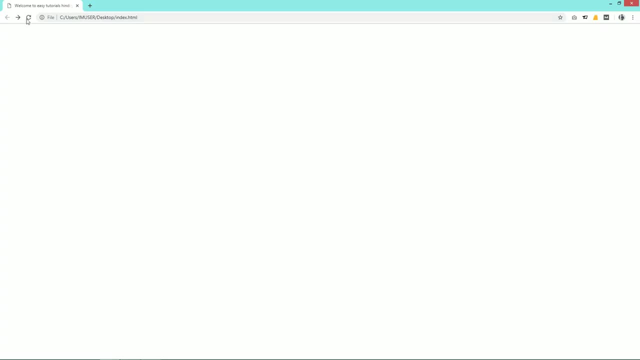 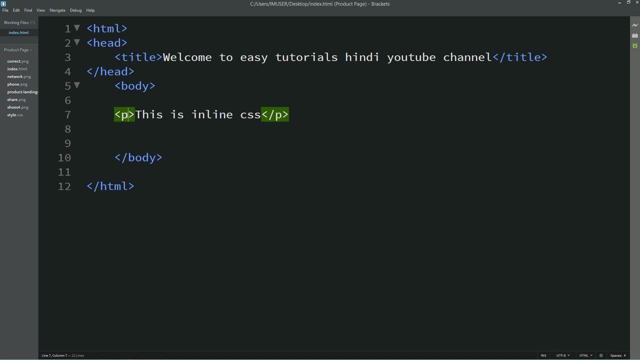 So it will be displayed as normal. You can see, this text is as a normal text on this webpage, Without any styling. So here we will add one inline css For that. in this particular p tag we will add one space and then we will write style. 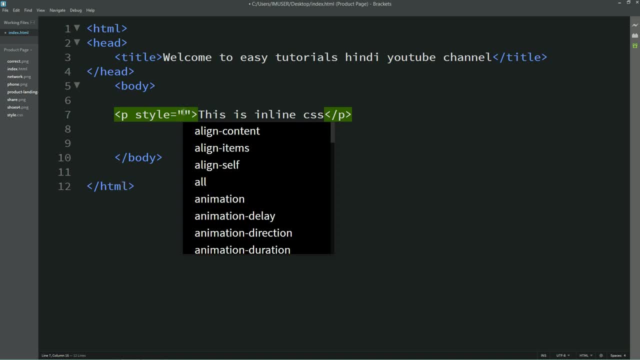 In this style we will write the css properties. So there are so many properties that I will discuss later, But I will take one small example here That we can use in css, Just like font size. So here I am adding font size. 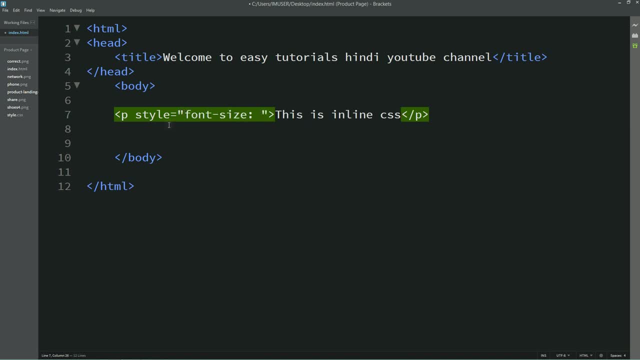 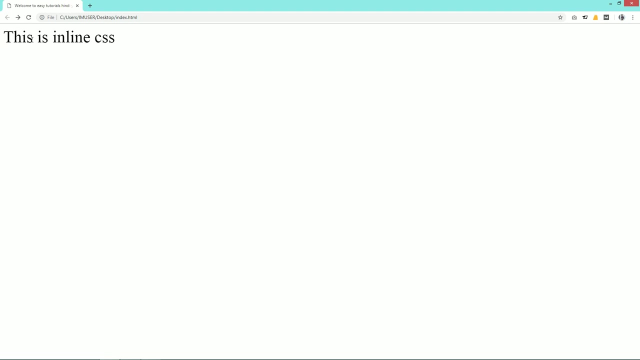 And I will increase the font size like 40px. So we have added 40px font size for this p text. For that I wrote: style equals font size 40px. So this is inline css. Let me preview this webpage. You can see this text. font size has been increased. 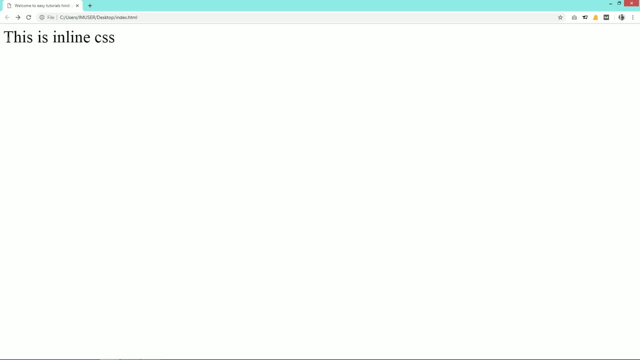 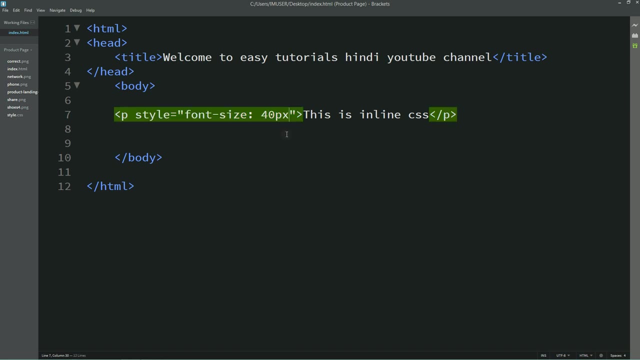 So this is how you can add Inline css in any html elements. Now we have second option, called internal css. We will write the css code at a particular section in a particular block, And we won't write this in the html element, But we will write it in the html page itself. 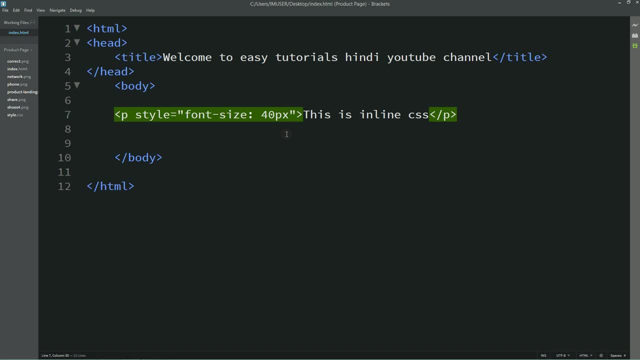 We will not create any new page, So for that we will write this internal css in the head tag. So in the head tag We will write style open and closing tag. So we have added this inline. Let me remove this. Save these changes. 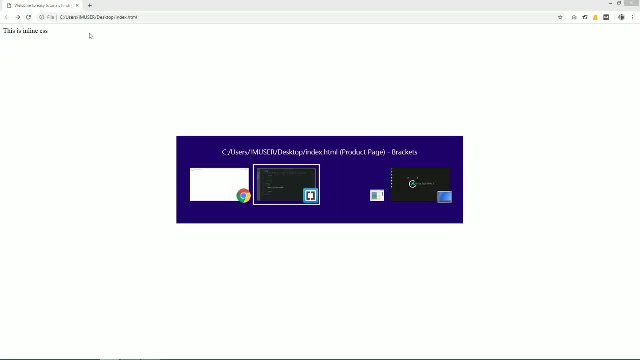 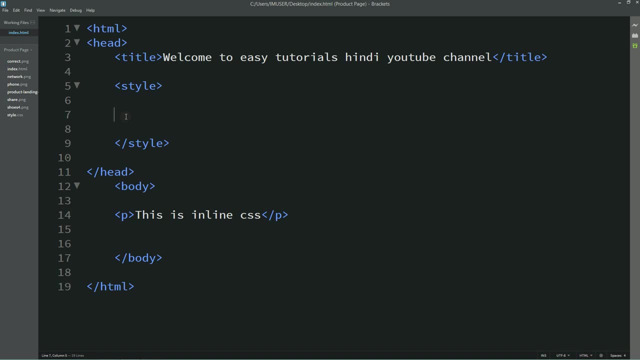 Reload the webpage And you can see it is again normal text without any css In this style tag. we will add some css. To use this css, we will apply this css code on this p tag. So later we will write this p in this style. 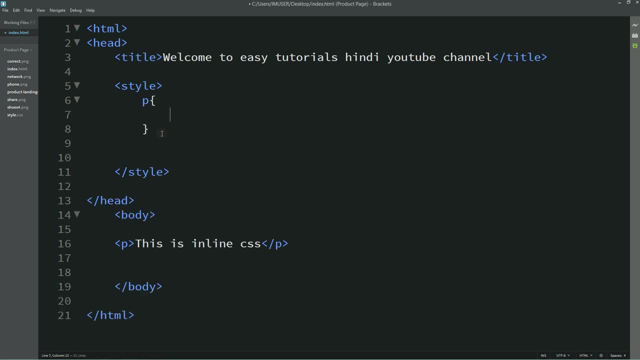 So here we will write p And for this paragraph text we will add font size 40px. So this is how you can add one internal css, And this is we are writing in the head tag Using the style open and closing tag. 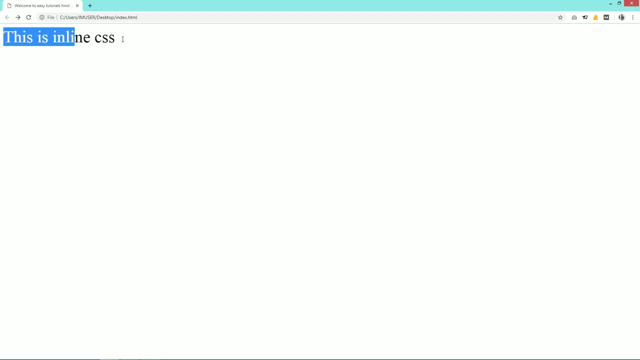 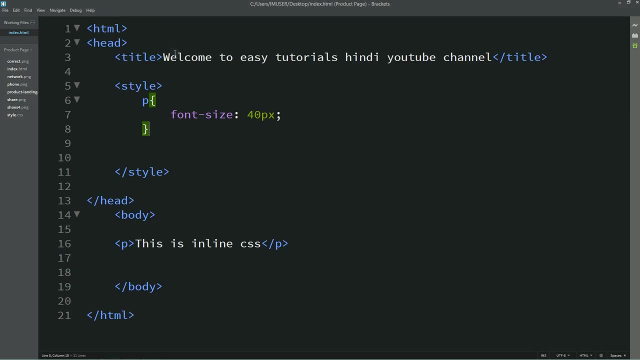 Let me refresh the webpage and you can see the font size has been increased. It means This property is applying on the particular html element. Let me add one more property of this p. Let me add font weight. I will write font weight volt. 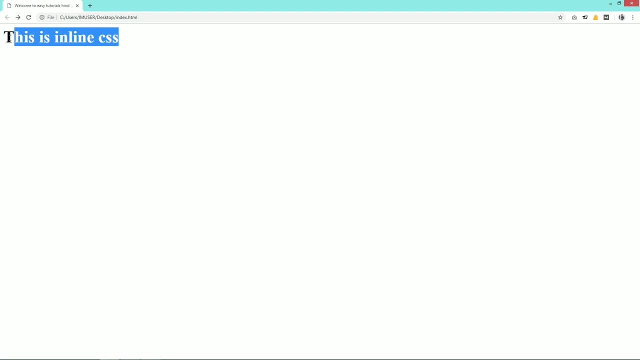 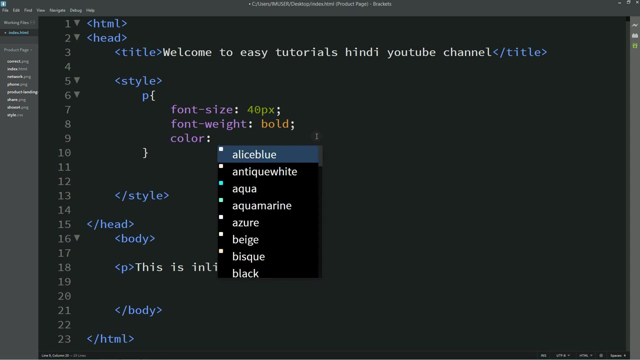 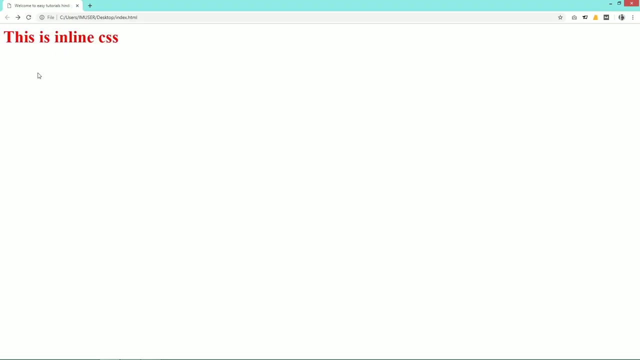 Let's refresh again. The font weight has been increased. Let's add one more property, which is color Color. we can write in three different ways That I will tell you later. For now, I am writing color red. Refresh the webpage and you can see this text in red color. 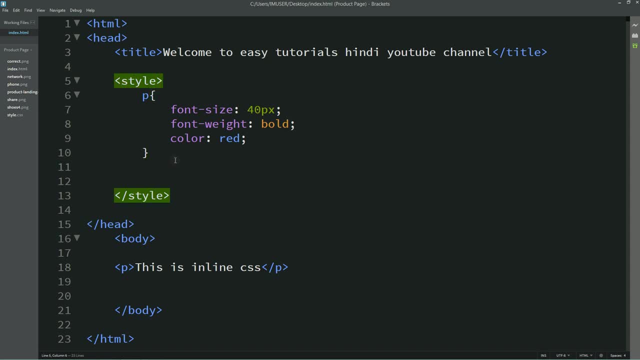 So this is how you can add internal css in the html file itself. Now we have the next option, which is external css. So if you have lots of html and we have to write large number of css, Then it's better to create a separate file for this css. 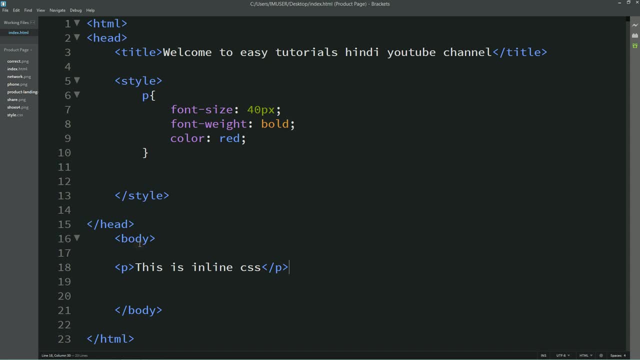 And we will connect this css file with the html file. So let me remove this. I will show you how external css works. To do this, we will create a new file again. So for this one, we created a file called indexhtml extension. 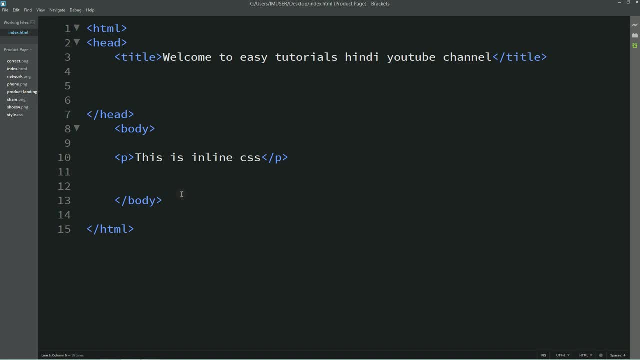 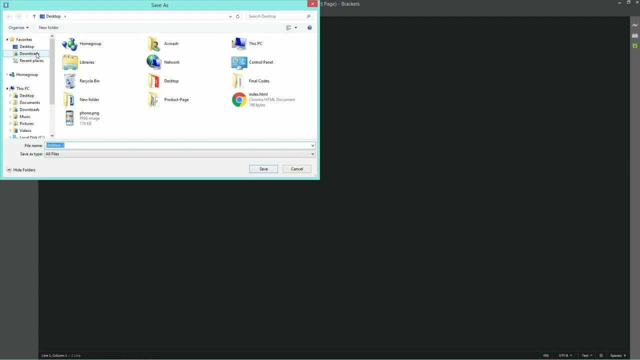 Extension was html, but for the css we will create a new file. Let me create a new file And Put this file on the same place, And let me write the file name: stylecss. Make sure the file name extension is css. 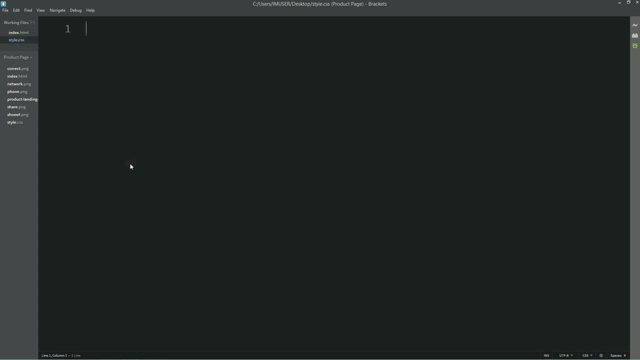 So this is how we have created the new file, which is stylecss, and it is blank. right now We have not written any code in this css file, So first we have to connect this html file with this css file. So In this html file we will write link. 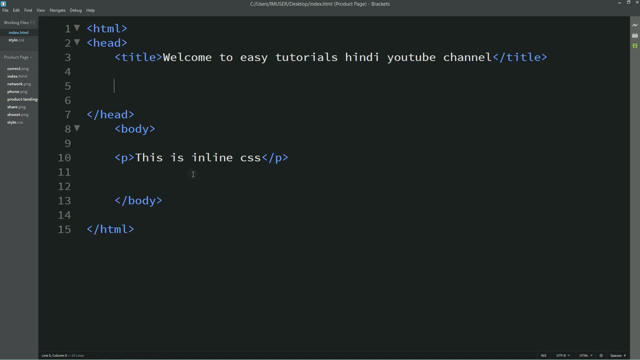 That will link our html file with the css. In this head tag I am writing link. Then we will write ariel rel equals. It will denote the relation with the next file. So it is a css file. So here we will select stylesheet. 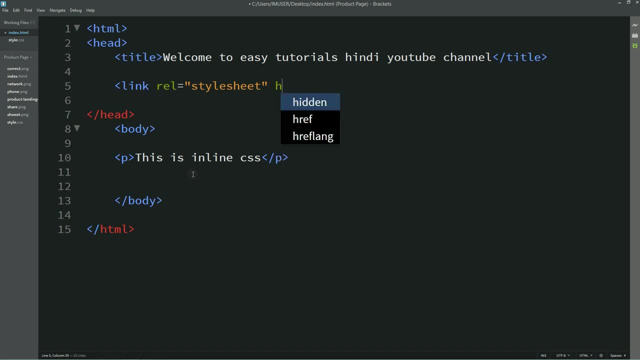 Then we will write href And href will be the file, Which one you want to connect with html file. So suppose this file is in the other folder. Then you have to write the folder name, Then slash and file name. But we have saved the css file on the same place in the same directory. 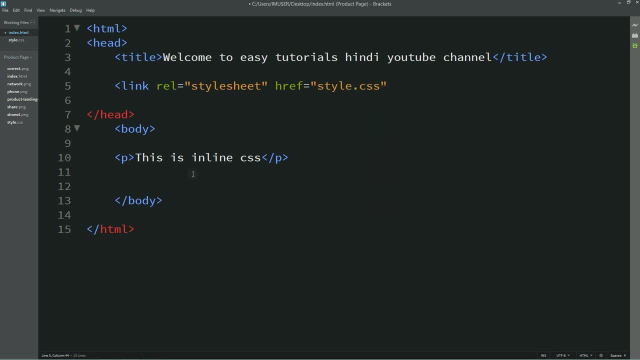 Then simply I can write the file name, which is stylecss, Because our html file and css file are in the same directory. So Let's go Go Then close it, And now it is connected. We can add one more thing. 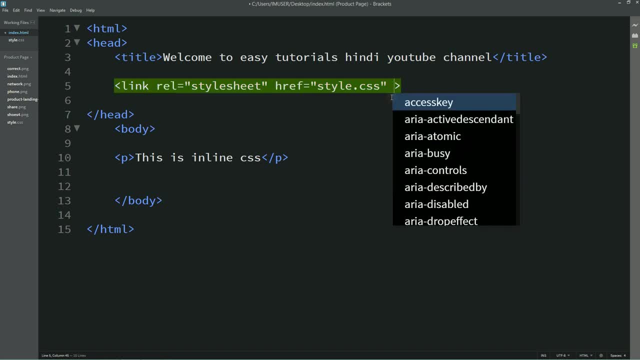 But this is optional. You can write, or you can also ignore it. So here I am writing: type text: slash css. So this is how our html file and css file is connected. So let's try one normal css code on this p, As we did earlier. 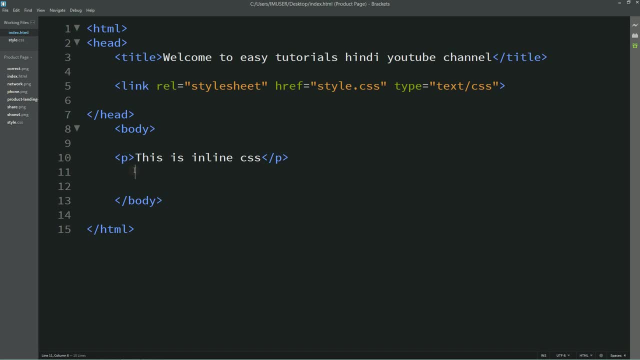 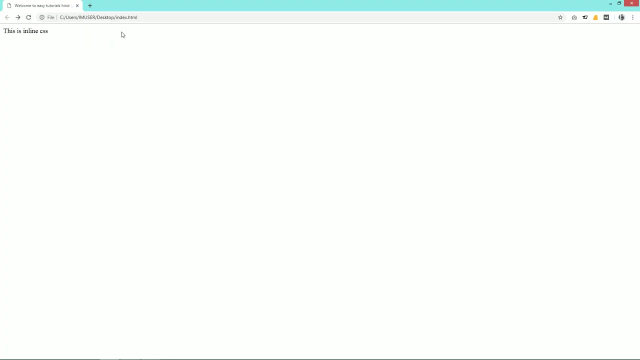 So Let me copy this p and we will come back in the css file, which is blank right now. So here we will write p tag because we want to apply css on this p tag. Let me refresh the web page and you can see right now it is a normal text. 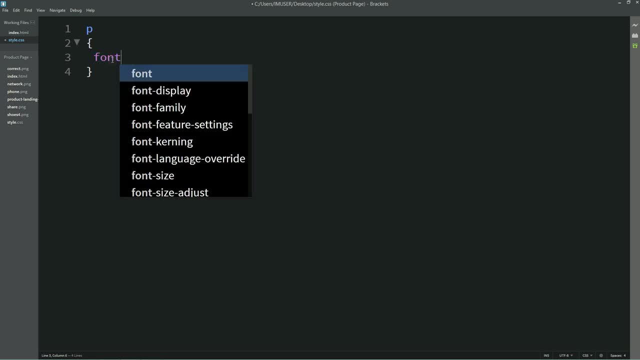 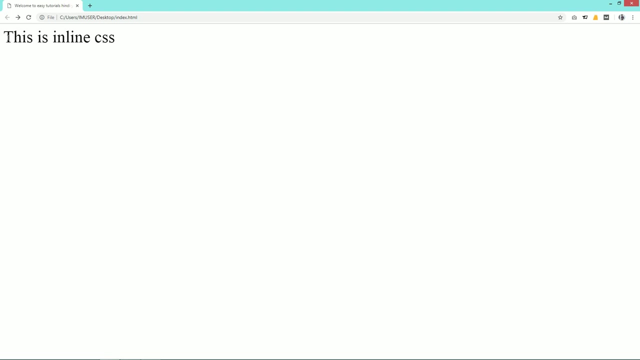 Let me write one css property in this css file. So here I will write font size: 40px. Reload the web page And you can see increased font size: 40px. You can see increased font size for this text. So we are writing this css in the separate file. 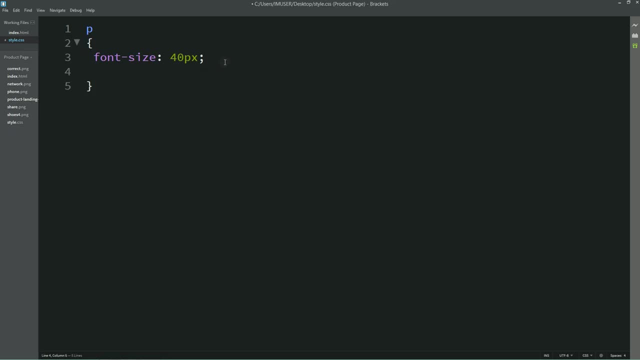 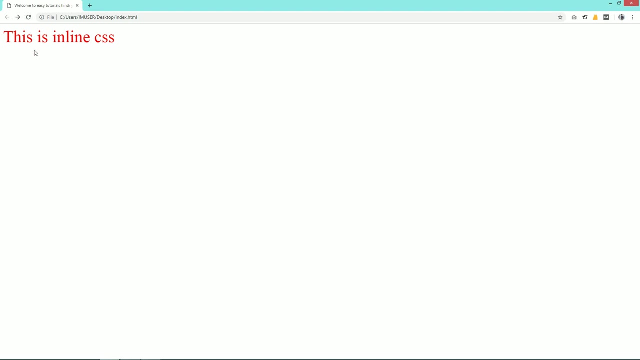 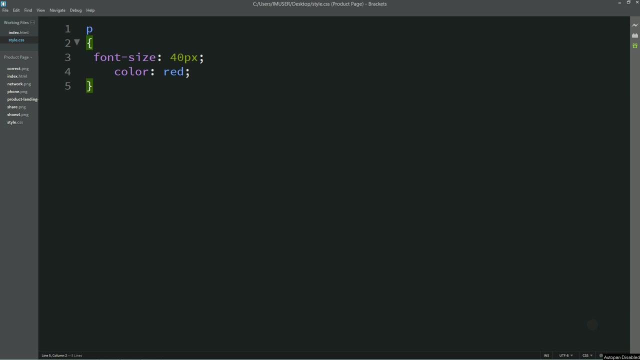 So this is how the external css works. Let me add one more property, which is color red, And now you can see this text in the red color. Now you know how to connect the external file for css And how to use the external css. 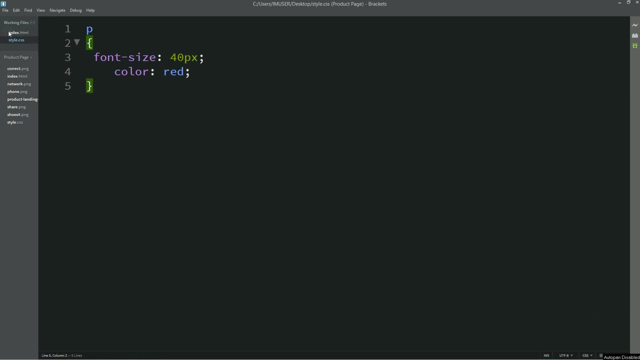 Now I will tell you how you can apply the css in other way. So right now we are using the same html tag, But we have another option. also: Instead of using this html tag, we can write the class name for the particular html element. 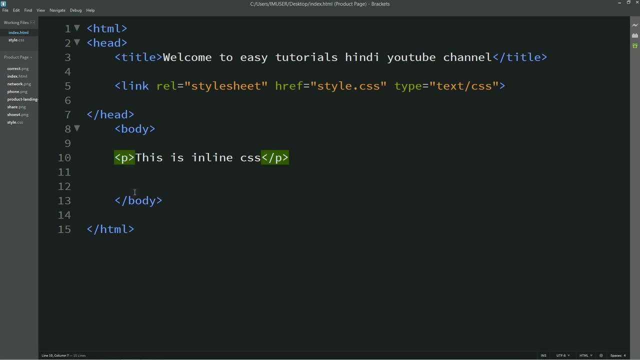 So in this p tag I will write one class equals and write the any class name. Let me write the class name title. So This is p tag, So this is the class name for this particular p tag. Let me copy this class name title. 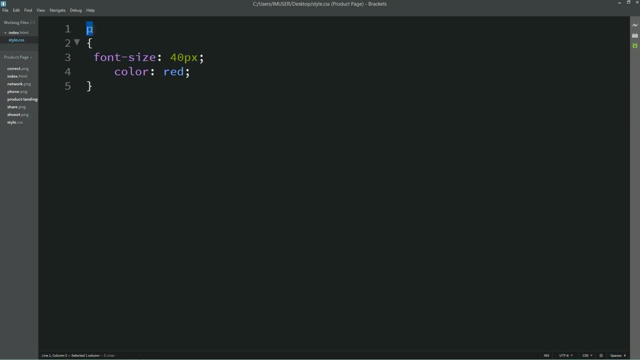 Come back to the css file. Here we are using the p, but instead of this p we will write class name. But when we are using any class name we use to add one dot also before the class name in the css file. So here we will write dot title, which is a class name. 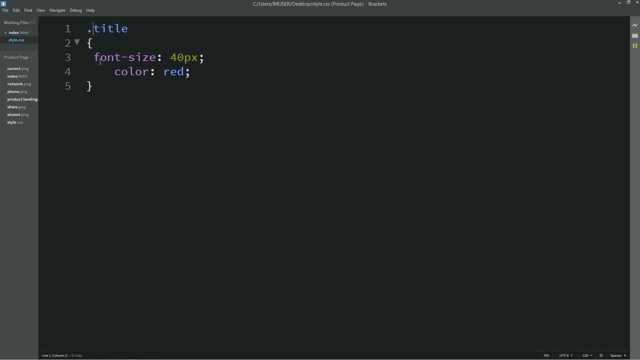 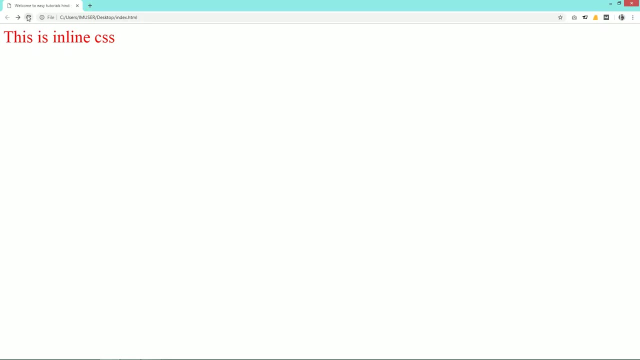 So Make sure You Remember this: when adding one class name in the css file, add one dot before the class name. Let's refresh the web page and you can see the same css property is again working with the class name also. So if we are using html tag, it is working. 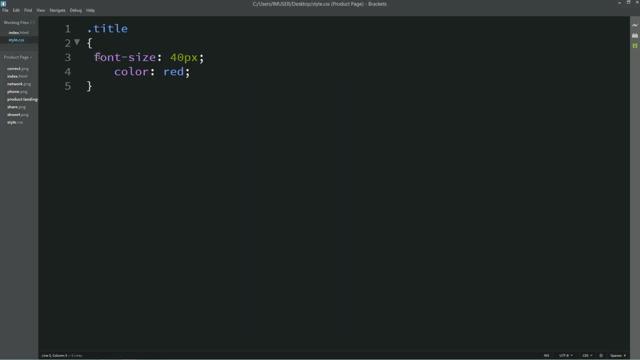 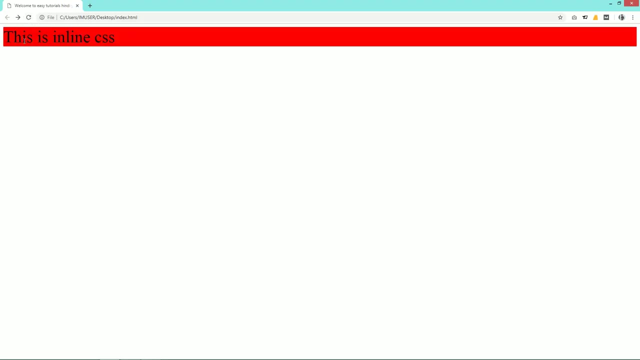 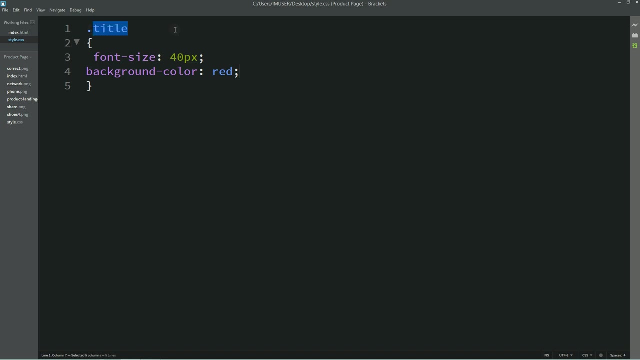 If we are using the class name. still it is working. Let me remove this color and I will add background color. I will write red. Refresh the web page and you can see the background color is red and the text is black by default. And let's come back in the html file. 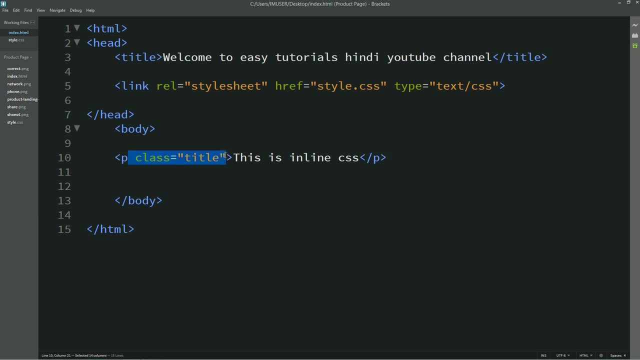 I will change it to p again And I will remove this class name from here. Suppose we have one more text after this p And the first one is h1.. This is h1- closing tag. Then we have p tag and some text in this p and let's create one more element. 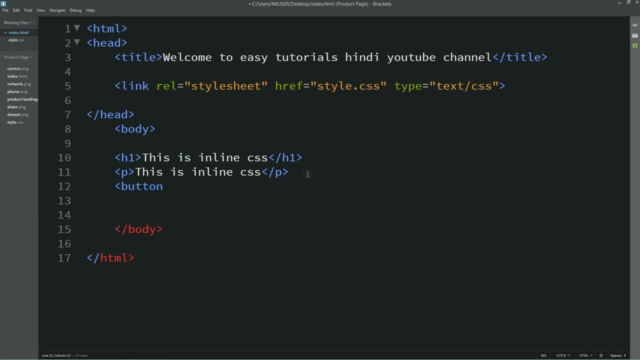 We know how to create buttons. So let me add one button here, But let's create another element. So In the button type I will write submit And button text here, Which is submit. So we have added one title in h1, then p tag, one button. 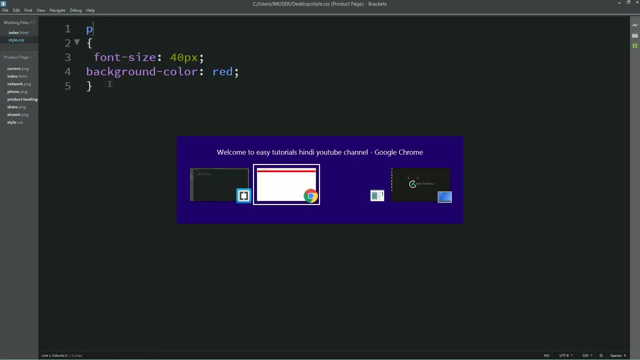 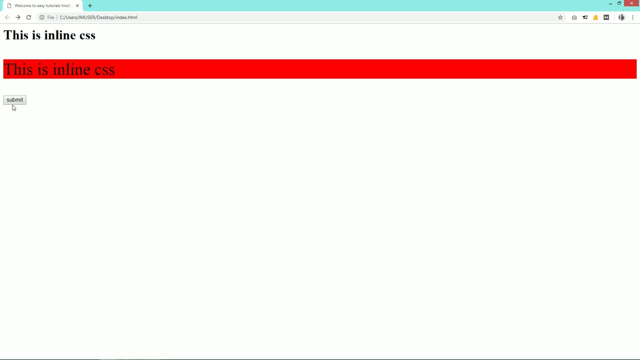 And in the css file you can see I have written the css only for p tag. Let's refresh the web page and you can see the first one is normal in h1. The second one has one background color And this button has no css style. 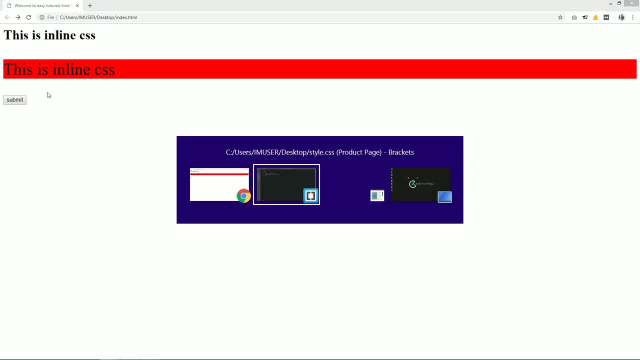 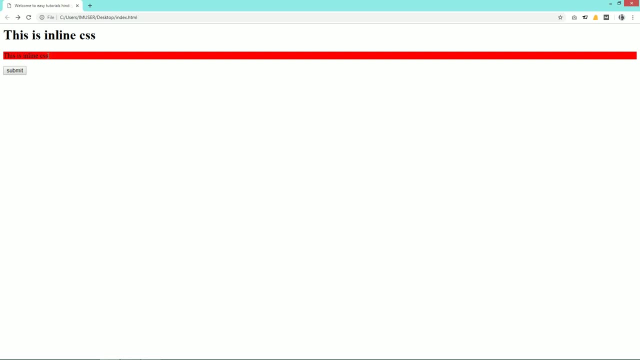 Now we want this background color for all these three elements, So let me remove this And you can see it is a normal text, It has only background color. And we want this background color for h1 also and for this button also, And we want to write the css for one time. 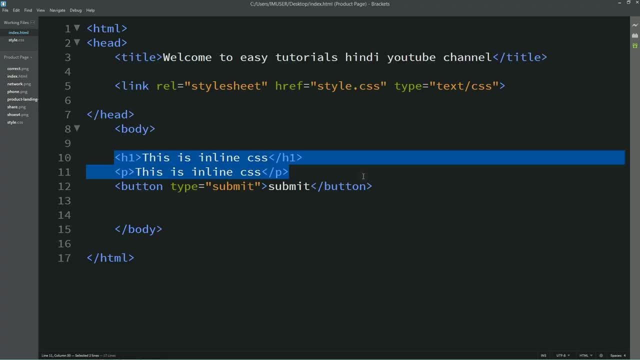 So let's come back in the html file And for this all three things, We will create a button, We will create one group, So later we will create one division, like we are creating a box and we are adding everything in that one. 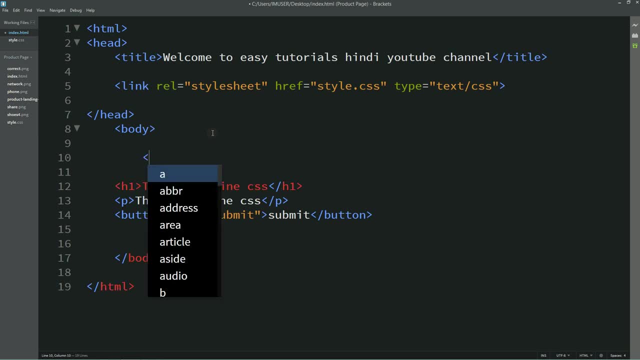 For that we will create one division And for that we use to create div. I will write one div And with this div we will create one class name also, so that we can apply a css property on it. We can directly apply on the div also. 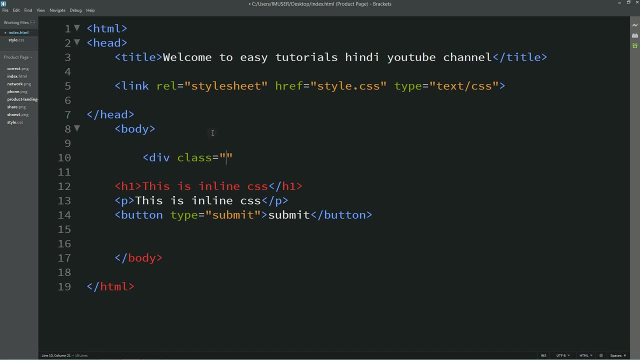 But we will use the div so many times on our page. That's why We will use a class name. So let me write the class name hello, And it will start here and close it after this three content. So you can see all the three contents are inside this div and this div's class name. 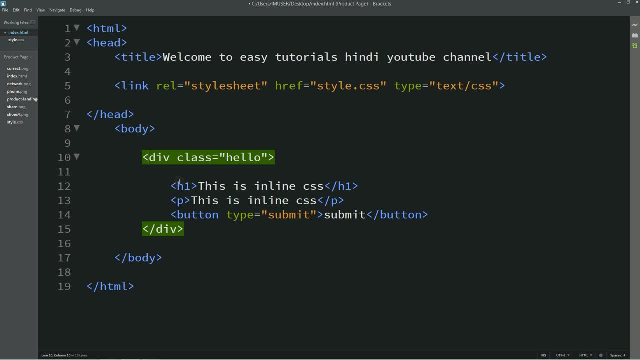 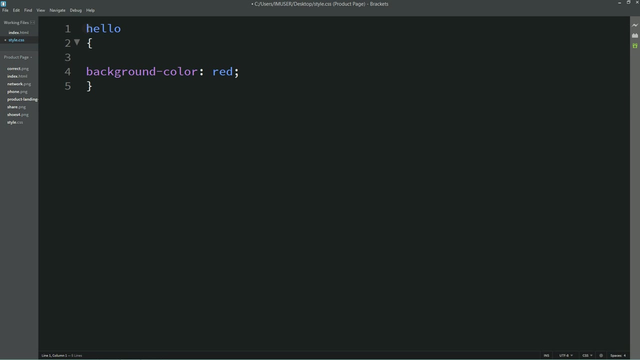 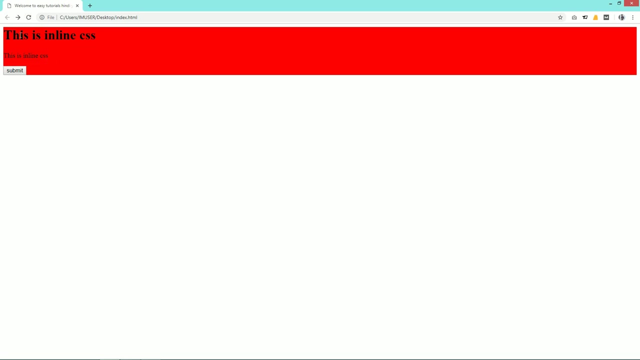 is hello. So now we can apply the css code on this. So let me copy this and add it into the css file. and background color: red. Here also we will write one dot, because it is the class name. That's it. Refresh the web page and you can see the background color is applicable for this entire content. 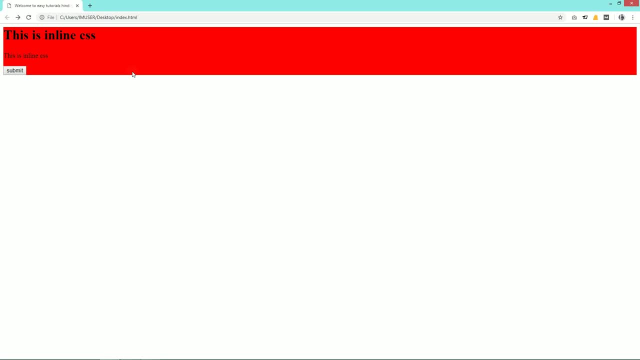 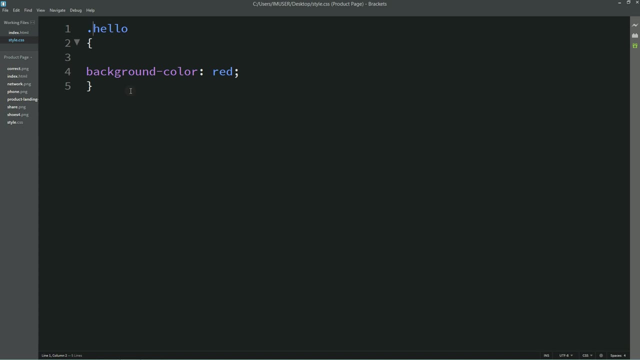 So this is how you can group some contents and apply css code for the parent element. How we will use the div, that I will teach you when we will go for the creating complete web pages. Now we will tell you more css properties that we will use mostly on our web page. 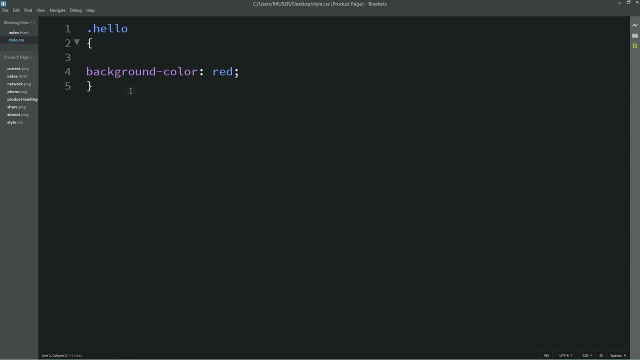 So first let's understand background, What are the background properties and what we write in the background property. So let me remove this, I'll write background. So, And for this background we can write one color. So, as we did earlier, red. 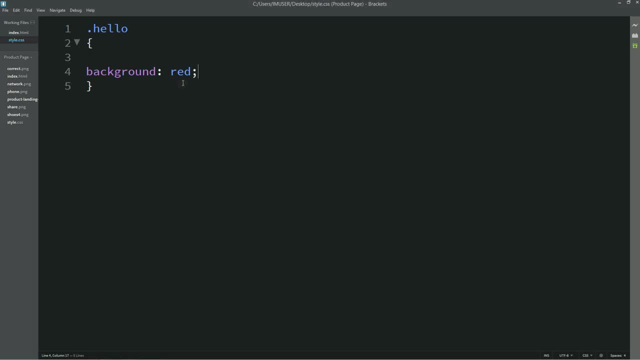 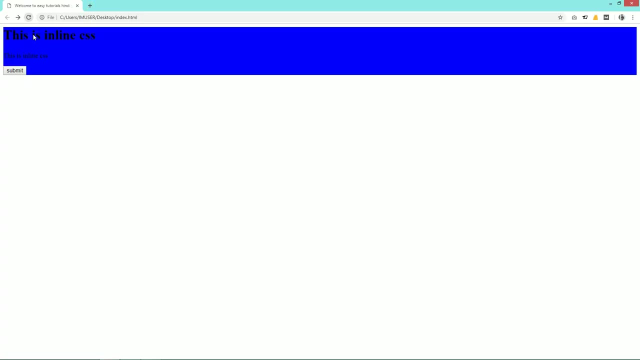 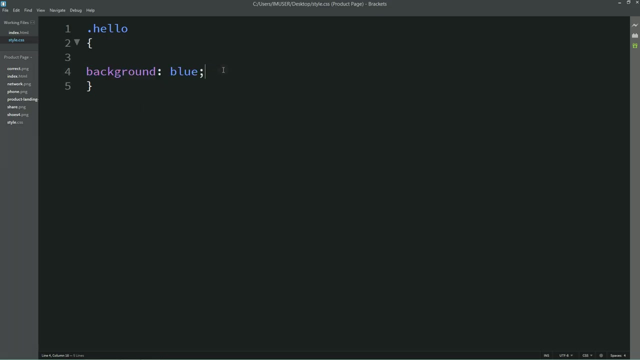 Right now you can see the background is red. Let me change it and here we'll write another color, blue, And you can see now blue color background. So this type you can add a background property. But before explaining other beg Property of a background, I will tell you how you can add different type of color. 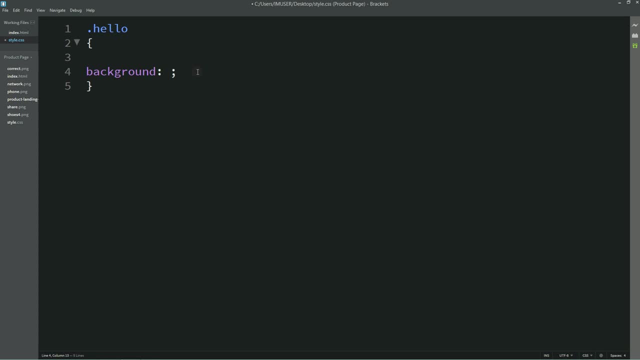 So you can add different name of the color here. Instead of that, we can write the code of the particular color. So every color has some code that I will teach you how you can get the code. So let me give you one example that I already know. 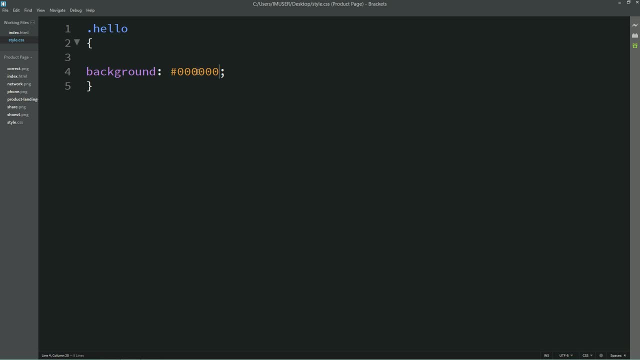 If you want to add a black color, you can use the zero, zero, zero. Refresh the web page and you can see the background is black right now. So this is the code for black color. Let me change it and here I will write this one: EFEFEF, and refresh the web page. 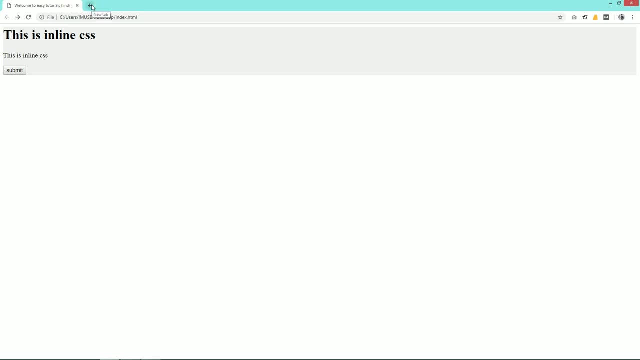 Now you can see some gray color on this web page. So this is how you can add different type of color, And if you want to know more about the codes of each color, then it's very simple. If you are on Google Chrome, then right click and select inspect, or there is one more option. 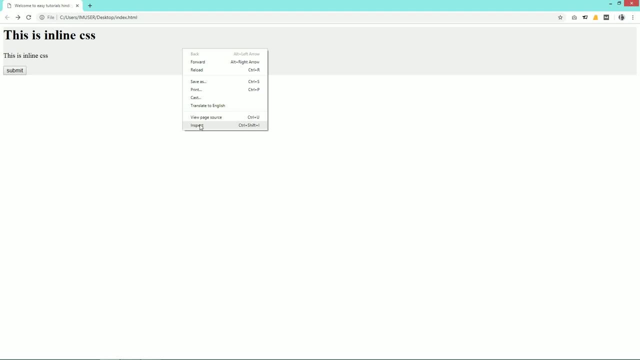 you can press F12 key on your keyboard and it will open a developer option. So let me right click here and I will select- inspect, Then select this pointer right here And select any content on web page where we have the color. So I will select here and in the right side in bottom you can see the class name is here: 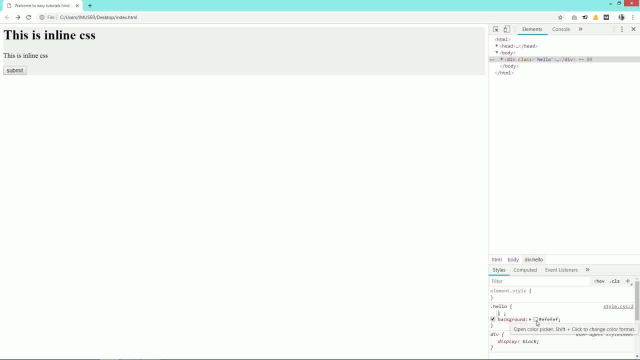 and then we have background, this color code. So let me click here and it will open a color box. In this box you can move the cursor to change the different color and you will get the color code for the particular color. Selecting the color, you can see the color code is also changing here. 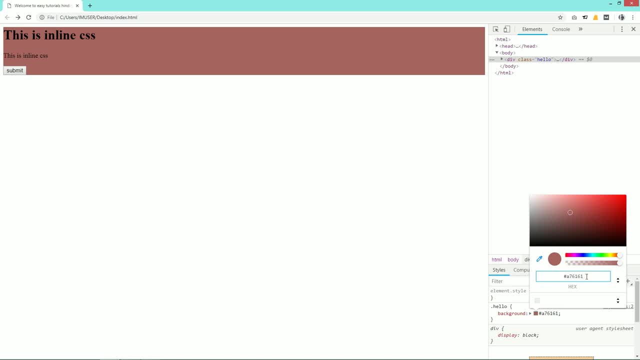 So like this, you can find your perfect code, which code color is working very good for your web page. If I click here in blue color, we can select the blue from light blue to dark blue, anything. I will click here on green. Now we can change the different version of green. 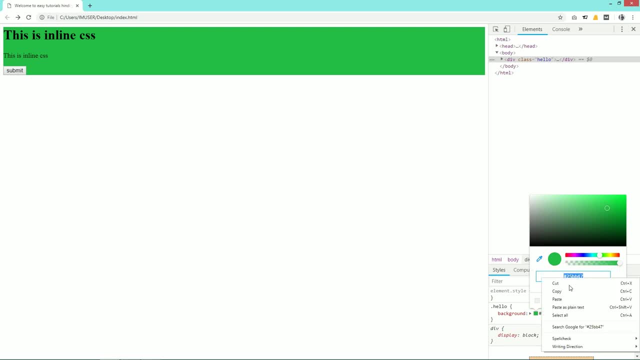 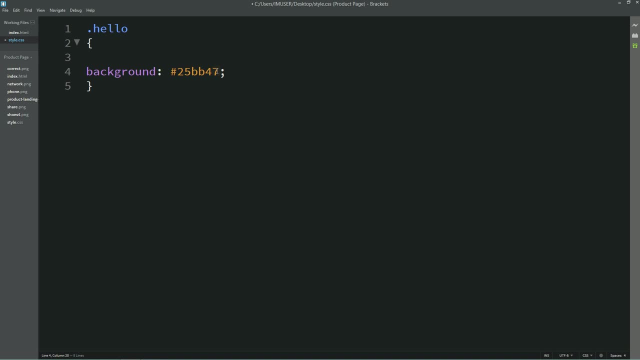 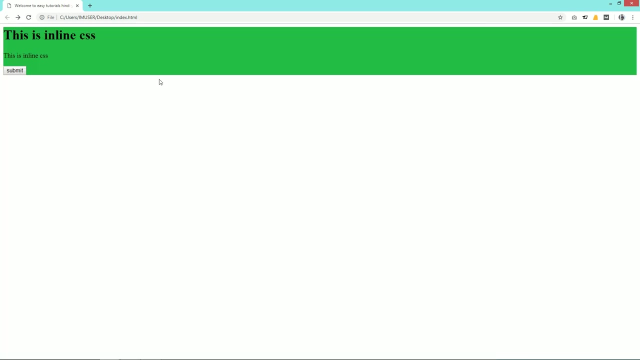 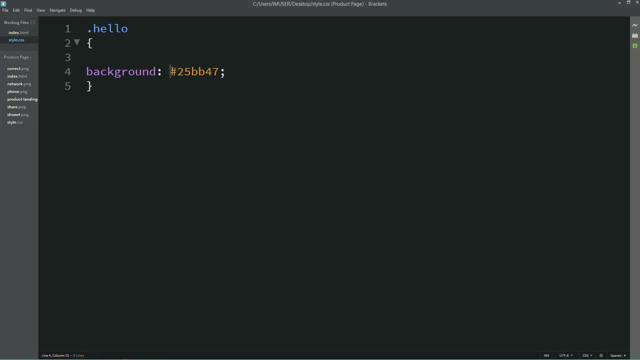 Suppose we want to use this one, Let me copy this code and come back in the CSS file and we will add this code here. Save this changes, reload the web page And now you can see this green color has been applied in background. So this was the second option to add color. 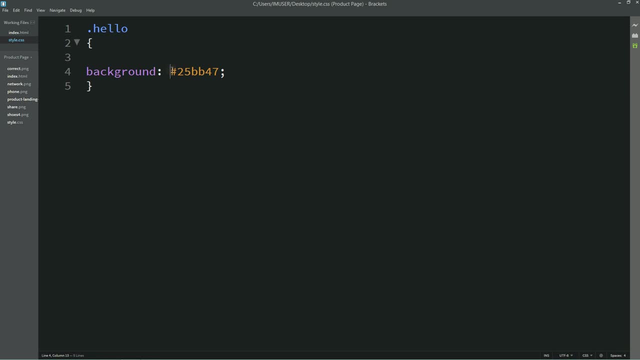 And first option was: we can directly write the color name and this was the color code. the second option. Next, I will tell you how you can add the color in the third format. For that we will write RGB. It is red, green and blue. 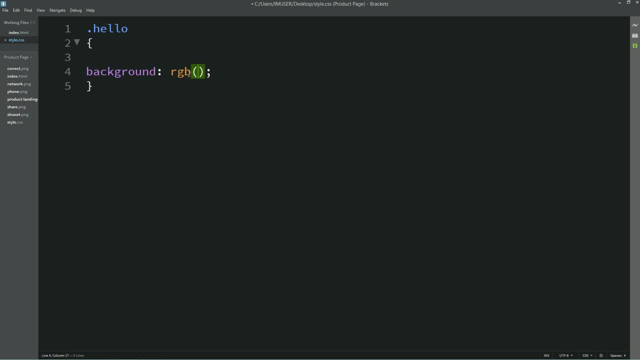 So its value start from the 0 to 255.. If I will write 0, 0 and 0 for everything, it will be black, And if I will write 255, 255 and 255 for everyone, It will be white color. 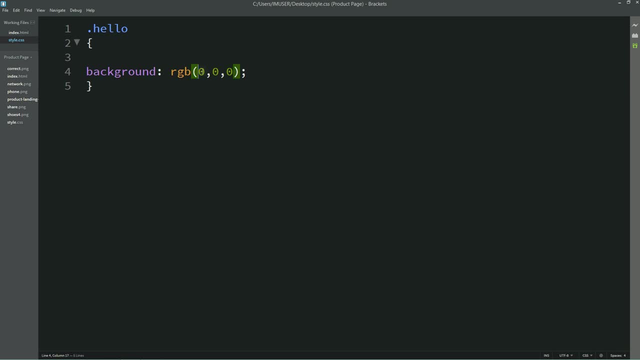 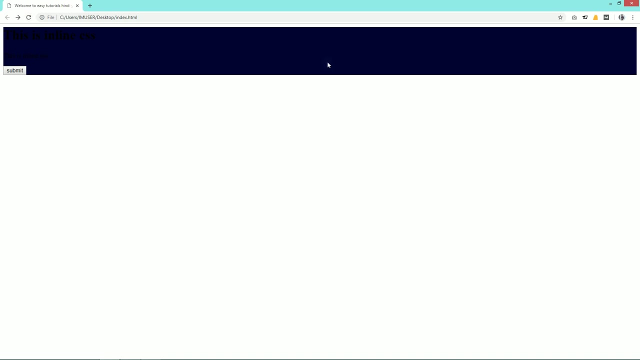 So, like that, you can increase the value from 0 to 255.. Let me increase any value. Suppose the red is 0, green is 0 and the third one I will increase. I will write it 50 and refresh the web page and you can see this different color. 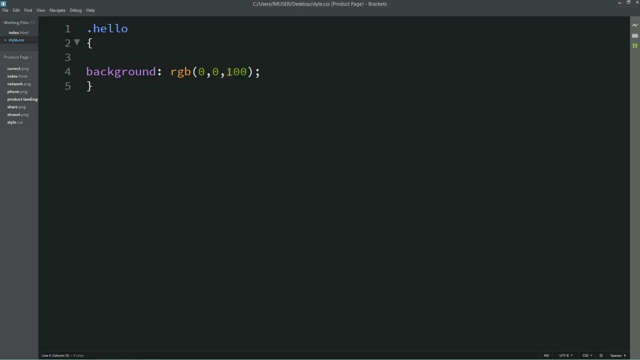 Let me increase it. I will change it to 100, and again you can see some different color for this background. Let's come back, And if I will increase the value in this green G For the middle one, I will change it to 100.. 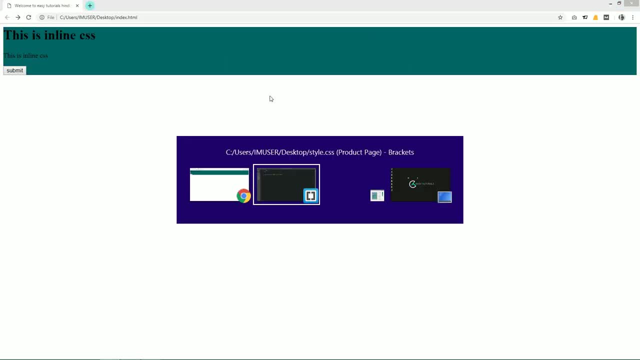 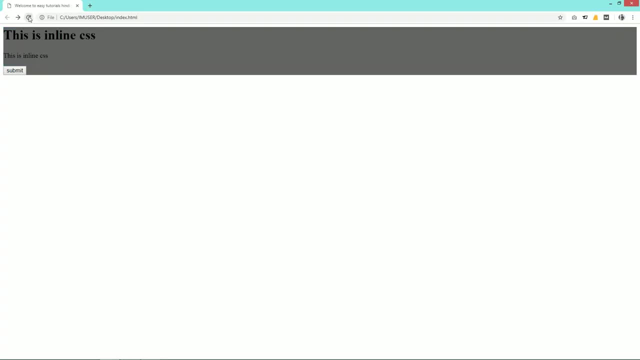 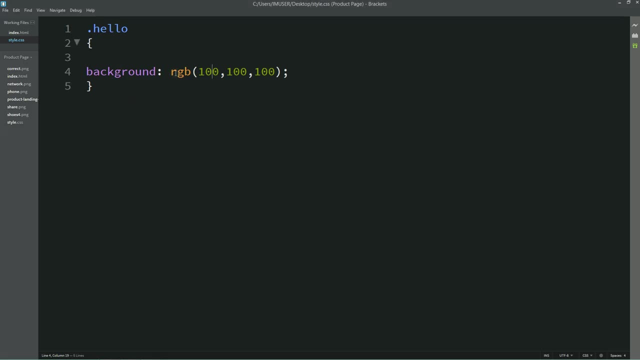 So now it is mixed color again. Let's come back. If I will change it red one, Refresh the web page and now you can see this is the mixture of all three color And we got a new color. This is one more option. with this RGB, we can add one more thing, which is A. 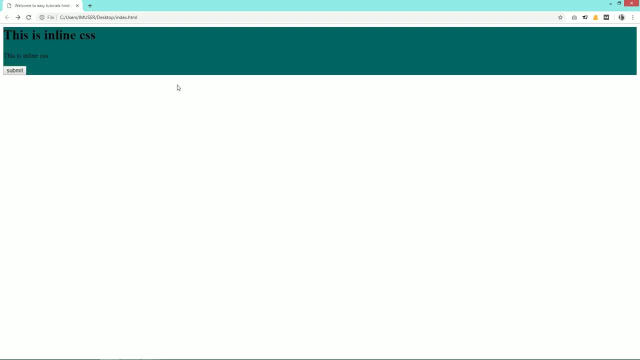 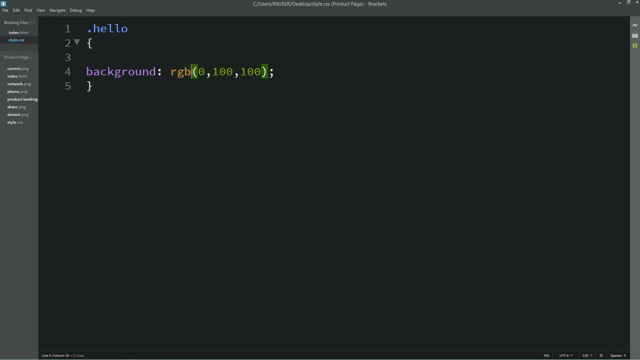 Let me remove this. I will change it to 0 because this is good And with this RGB we will add A, And when we add A we have to add one more value here with comma. So after this 100, I will write comma. 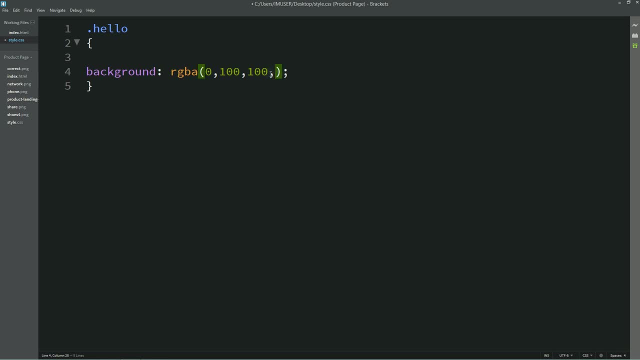 And this value will start from 0 to 1.. It can be 0, it can be 1, or it can be in 0.5, 0.2, 0. something less than 1.. It is actually representing the opacity of the color. 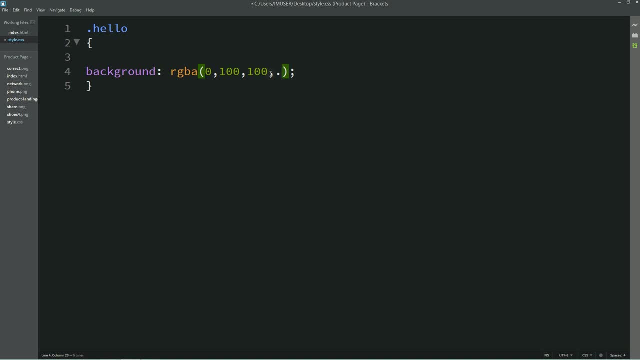 Opacity can be 0, or opacity can be 100%, or it can be 20%, 30%, anything. So let me write the 0.5.. So it will be opacity 50%. Let me refresh the web page And you can see. 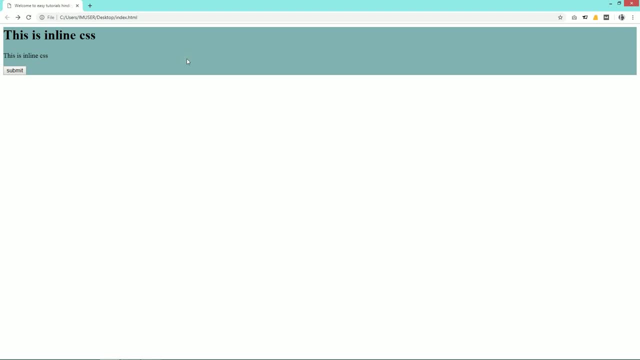 It looks like the color opacity is low because we have added 0.5.. Let me reduce it again. I will write 0.2.. It means 20%. refresh the web page again. even more light color here. So this was the third option, to add the color. 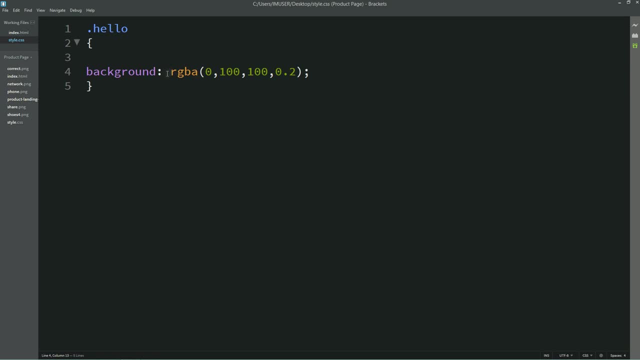 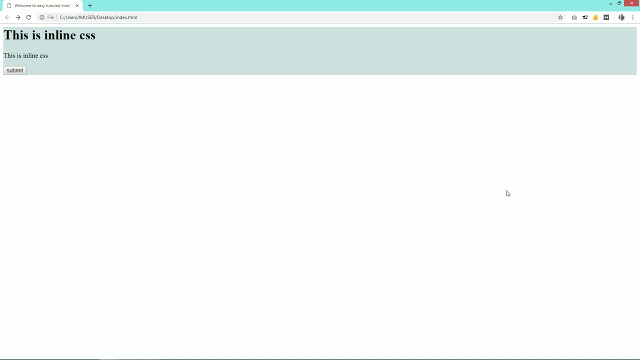 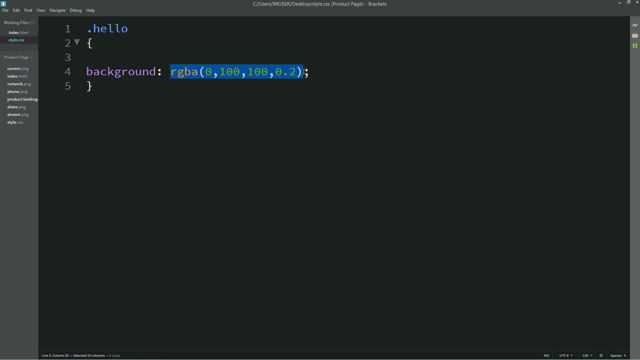 This value also, you can select from the web page, right click and inspect, and then you can select the value From the color box, As we did for the color code. So now you know about the colors code, Let me remove it and we will see what we can use in the background. 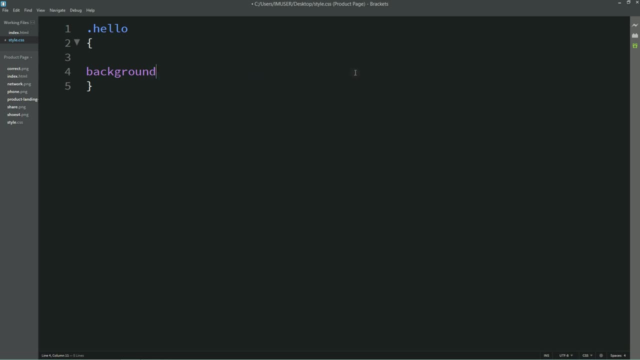 So with this background we can add background color, And this time you can use the color. We are getting lots of color name here. You can select this one to add background color, So let me use this one. So earlier we used background. 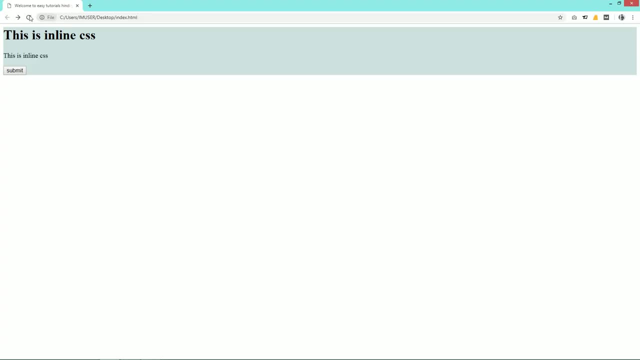 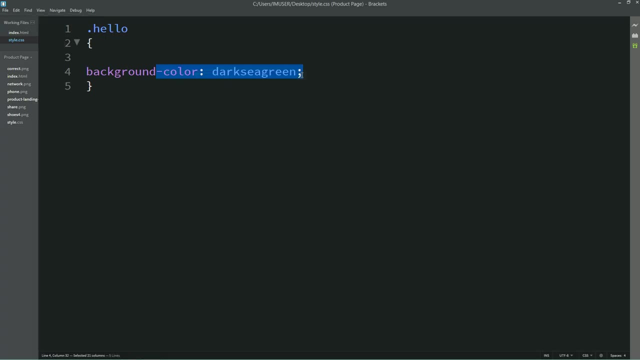 This time I am using background color, So it also works. Next let's see what we can use. We can write background image. Mostly, we will use this tag to add background image on our web page, or we can also use it to create gradient color in background. 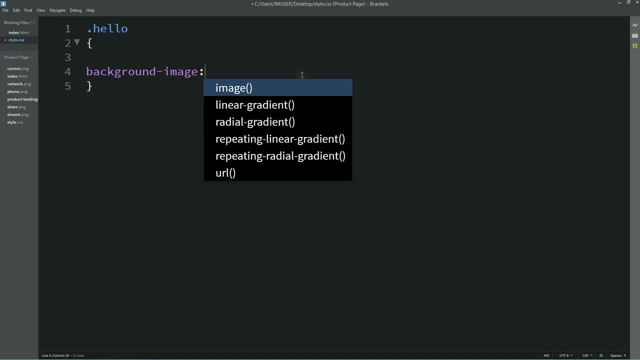 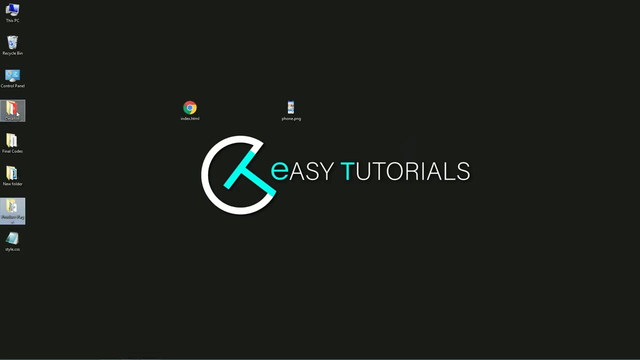 So let me add one image first. For that I will write url, And in this url we will write the path of the image. Suppose your image is available in this same file where you have css file, then you can simply write the image file name. 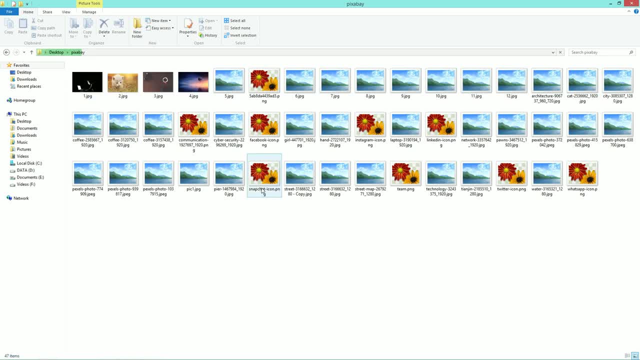 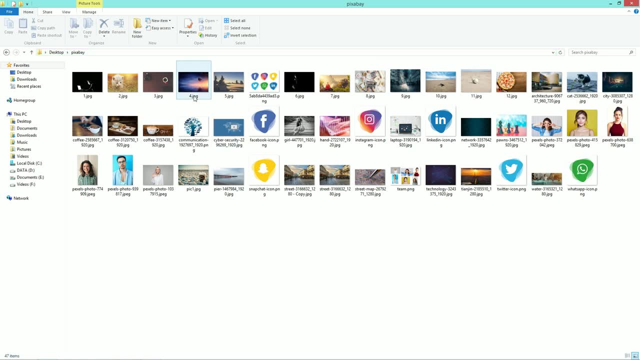 But let me search where is my image. So in this folder I have so many images, So I will connect the image from this folder itself. Let me think which one I will use. I will use this one, 3.jpg, And it is available in the folder after desktop, and then one other folder called pixaway. 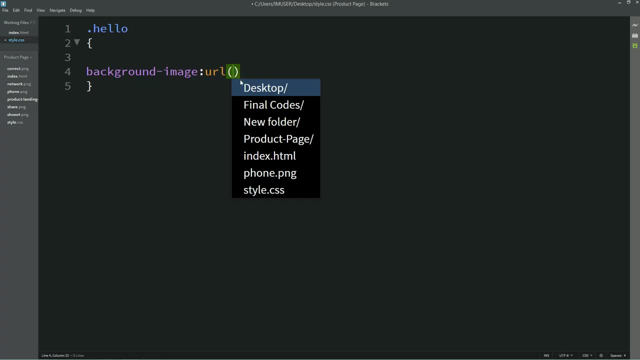 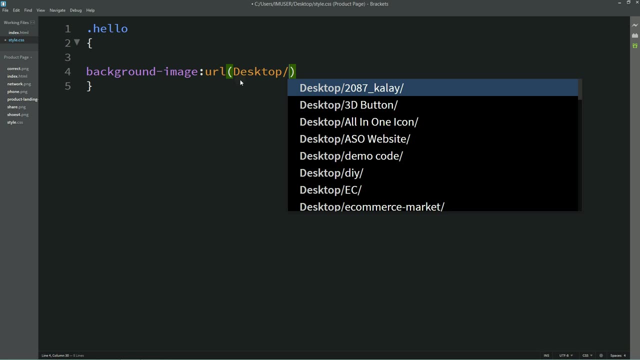 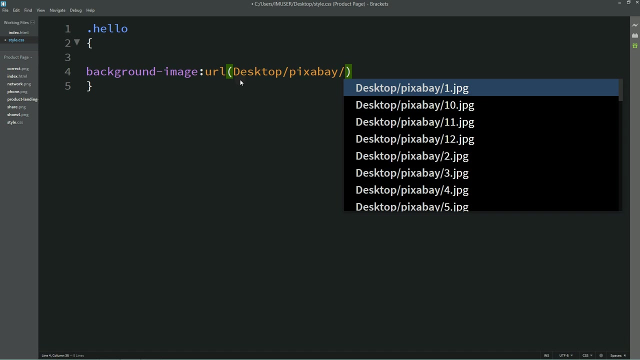 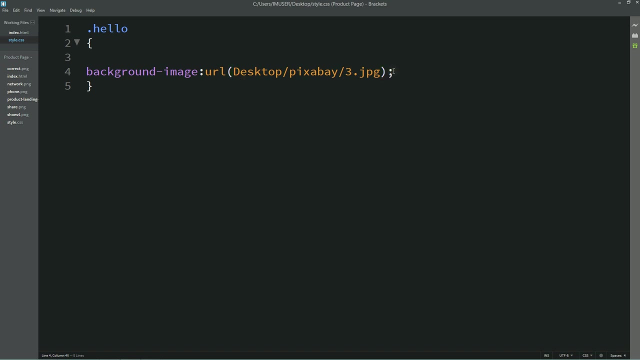 So let me come back in the css file. Here I will write the folder name, which is desktop, And after that I have one more folder called pixaway, And in this folder I have this image 3.jpg. So we are using this image. 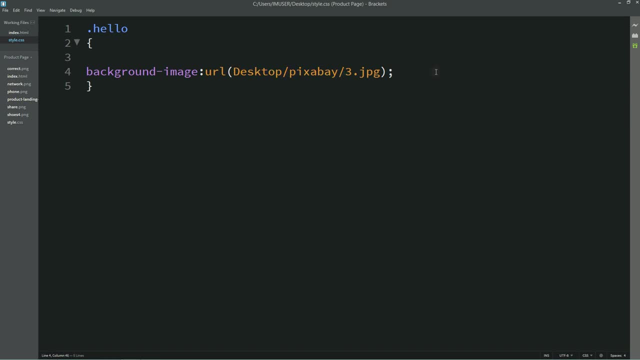 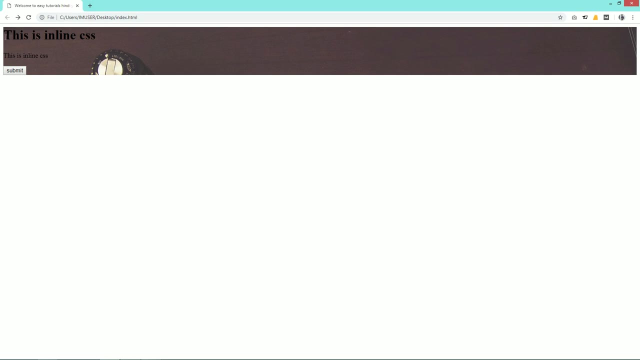 Suppose this image is available in the same file, then you can remove the initial part. Simply you can write the file name. That's it. Let me refresh the web page and you can see this image on this web page, But it is not visible clearly because its height is very low. 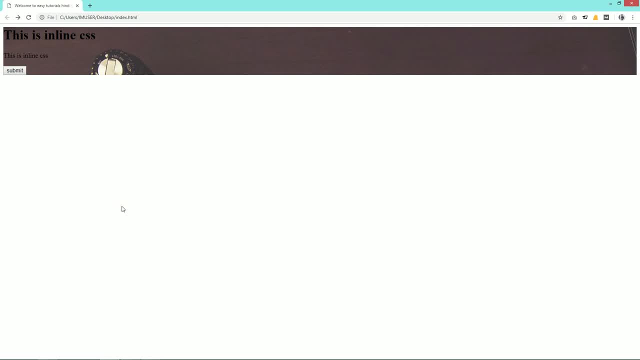 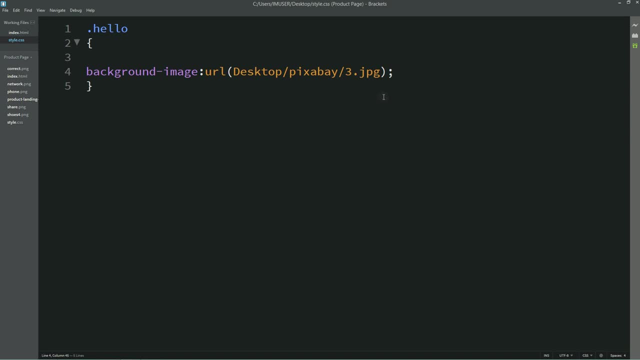 We have not defined the height of the content, So let's come back. We will increase the height first, so that we can see the image full screen. I will tell you more about the height, but let me write it here, because the background is not clearly visible. 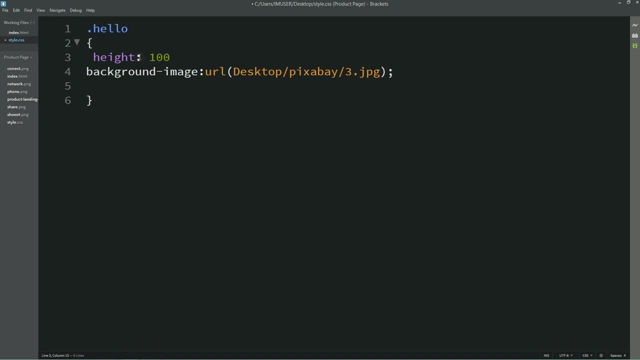 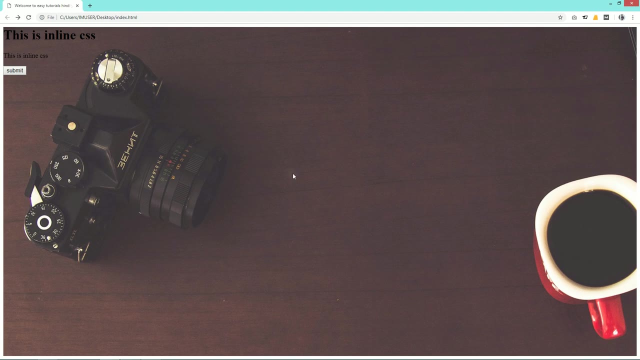 It is very small, So let me write it here: Height 100 percent And refresh the web page and you can see the image on this complete web page. So This Is How you can add an image using CSS property background image. 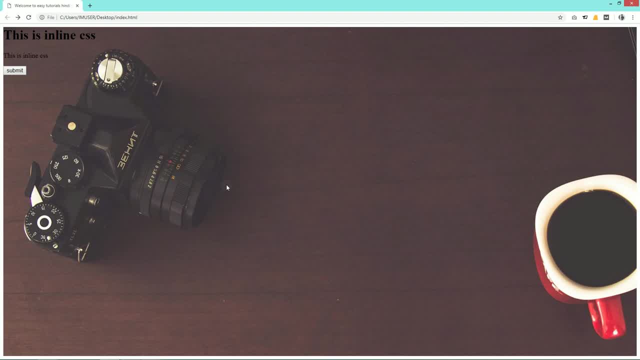 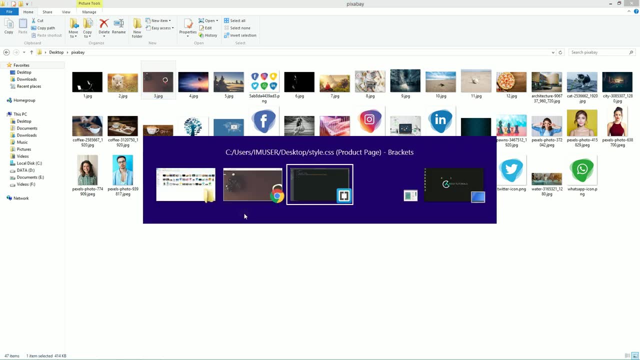 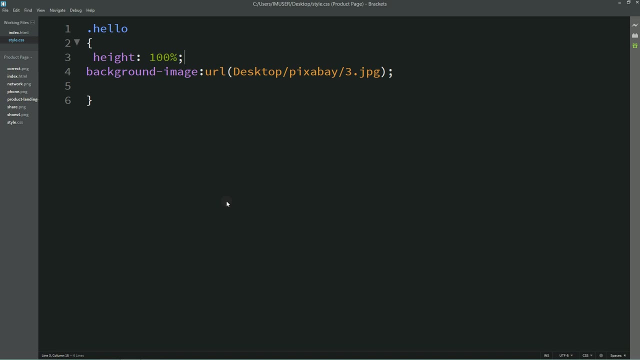 Since we are using an image which is fit to this screen. that's why it is coming like this. But suppose if we have an image on different size, if it is in very big or very small, You can find some issue like this image can be repeated and sometimes it will be small. 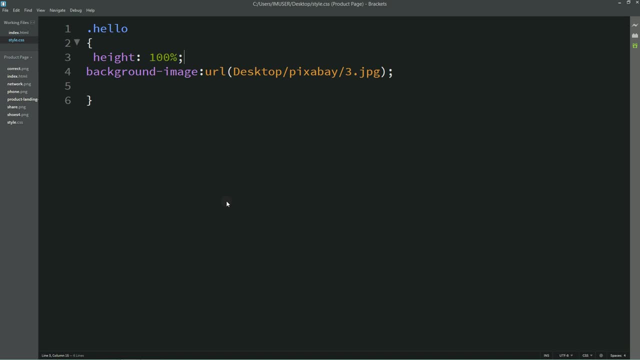 It will not cover the entire page, So I will recommend you to use 1920 x 1080 pixel of image for full screen image. Let me come here in the CSS file and here I will write Background repeat And it will be none, so that our image file will not repeat in background. 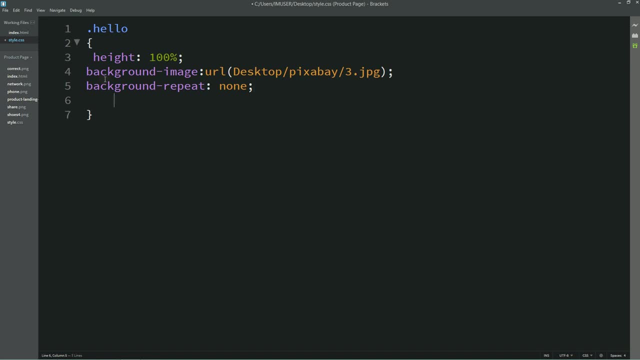 As I told you, if you have a small image, then it will repeat. Next we can add a background position And it can be bottom, center, left, right, top, anything. So here I will write the center, because we want this image in the center. So 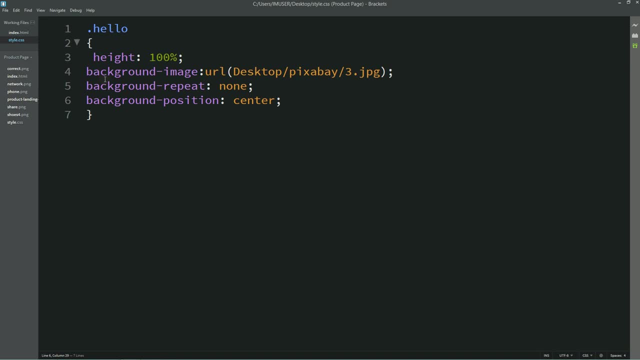 Let's see what else we can write in background. We can write the bottom, center, left, right and top. Let me select the center right here. Next you can write the background size And in the background size you can select auto content and cover. 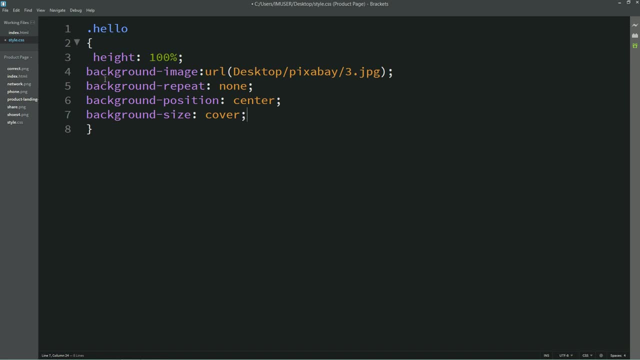 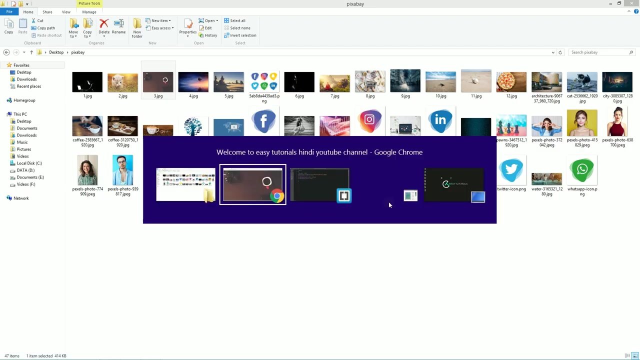 Here I will write Cover So that the image will come in full screen. So these are the background properties. There is one more option called background attachment. Let me refresh this first. Right now it is looking like this. Next we will see background attachment. 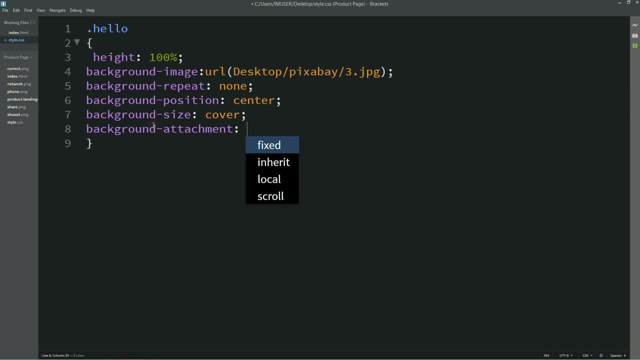 It can be fixed Inheaded: Local Scroll Anything. So these are the options that you can use in background attachment. Suppose you have to create a parallax effect, Then you can use the background attachment as a fixed. So when you will scroll the web page and it looks like a second content is overlapping. 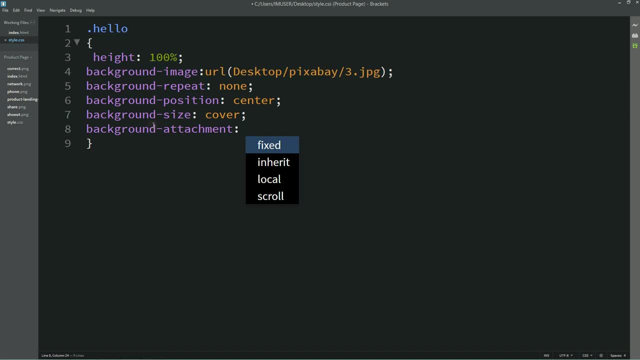 the above background image Because we don't have any long content on this web page so that I cannot scroll this. But we will teach you how to do it When we will create a full template. Now I will teach you some other content. 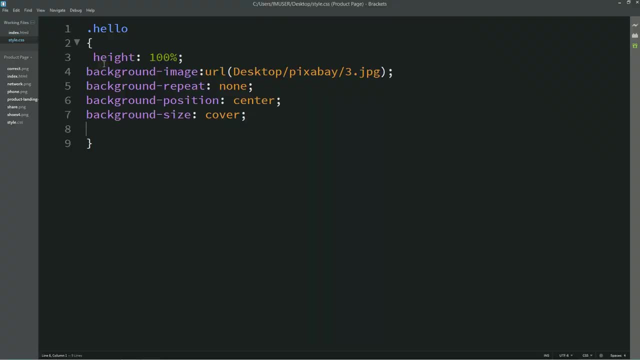 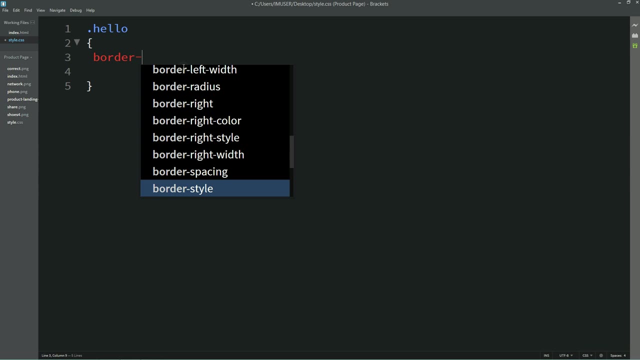 I mean some other property of CSS. So let me tell you Border. So how to use the border. I will tell you Here. I will write border First. let's see the property border style. So border style can be dashed, dotted, double, and these are all option that you can use. 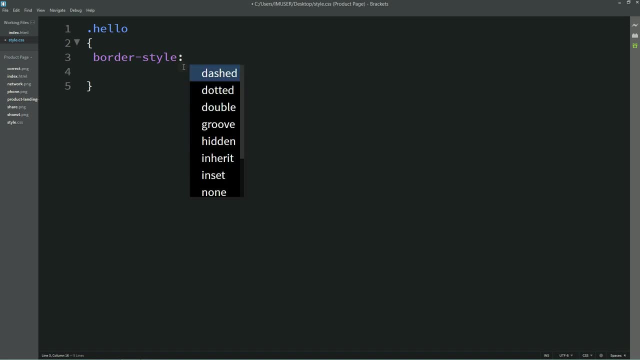 in border style. So let me select one option. one option: solid border style will be solid. next we will write another property, which is border width. so here we will define the width of the border. so let me write 2 pixel. next we'll write border color and we can write any color. 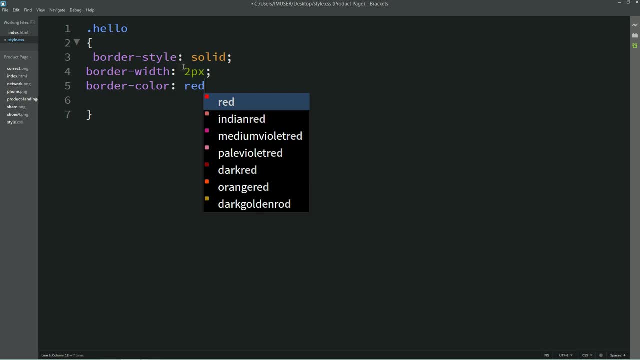 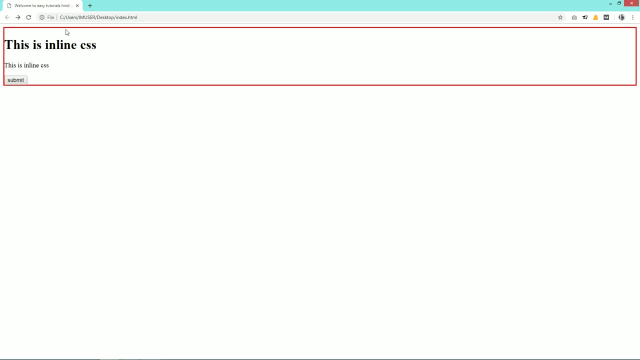 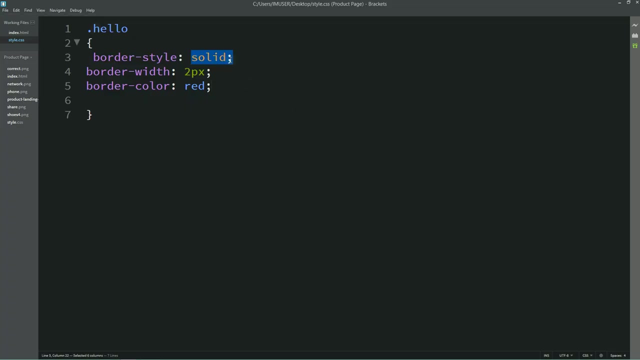 here. let me write red. let me refresh the web page and you can see one red color of border around this text and its width is 2 pixel and it is in red. let me change some style. so for this border style, let me select a dashed. let's. 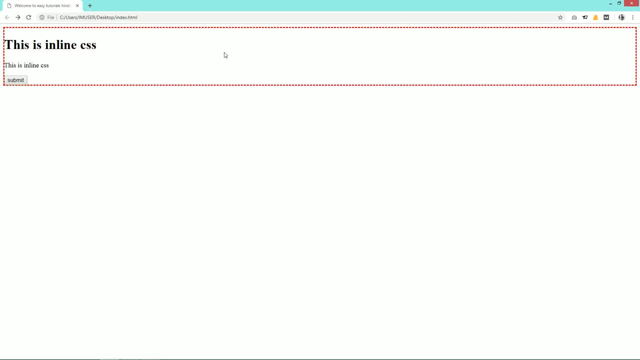 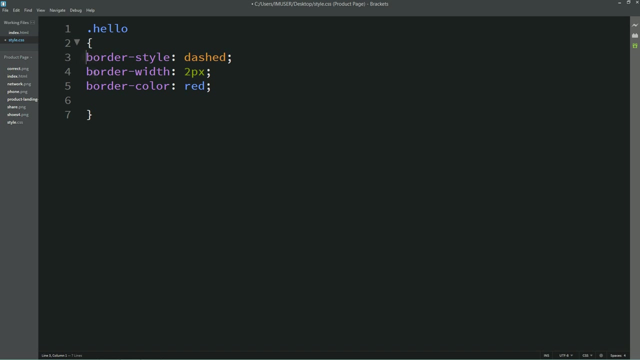 refresh the web page again and you can see the border is in dashed style. now we have another option also: we can write everything in one line. instead of writing this three line, we can merge all the three lines in one line. so here I'll write border, and first we will write the width of this border. it will be 2 pixel. 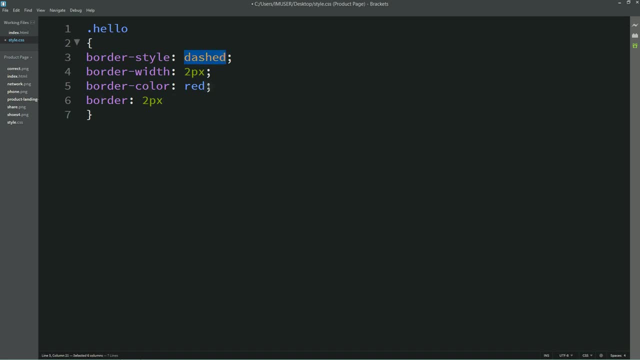 then we will write the style. so style: we are writing dashed and at the end we will write its color. let me write red. we have added all the three options in one line. let me remove the above three line. that's it. save these changes. we are writing only one. 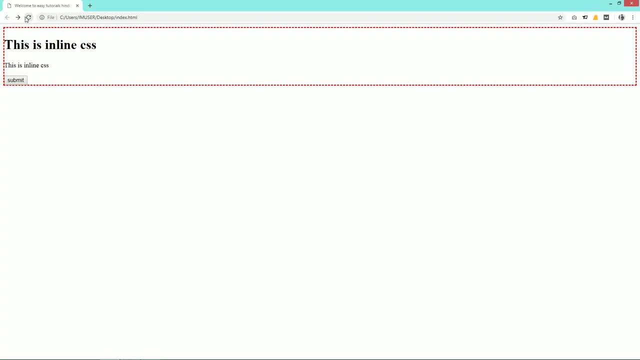 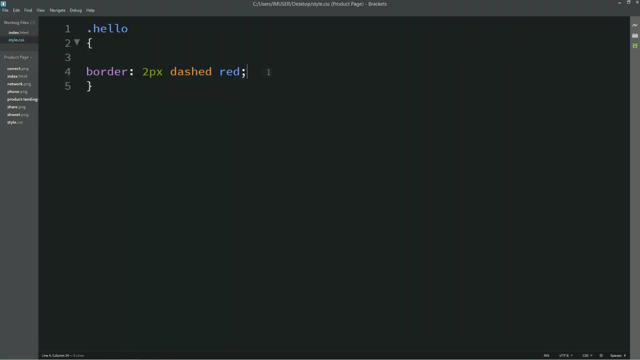 line. so after reloading the web page, you can see we are getting the same style for this border: the 2 pixel of border width, dashed and red color in writing one code only. this is the option to add border. now we have other option also. like this, border is going around all sides, so we 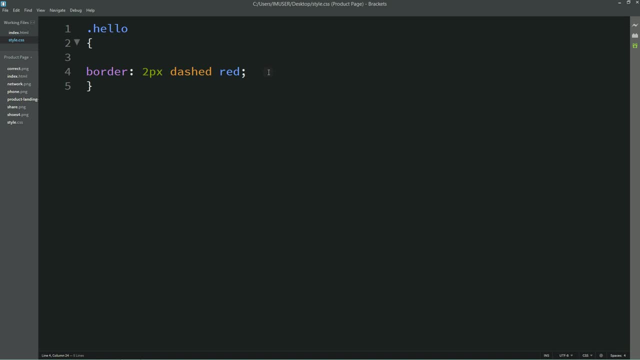 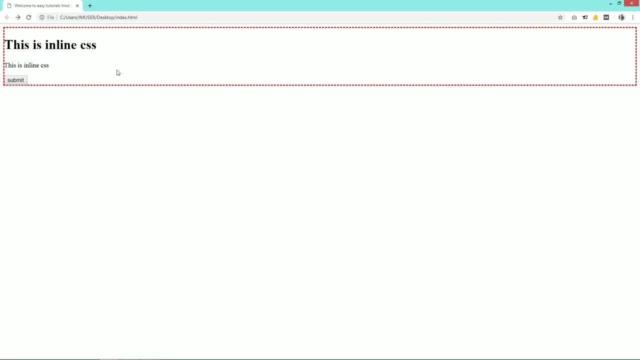 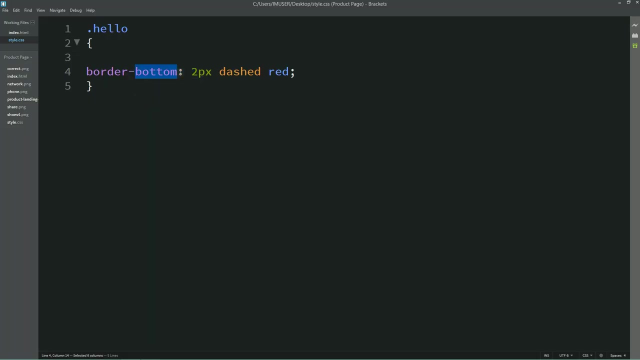 can define the border from any left side or right side, or top or bottom, so let me change it here. I will write border top. refresh the web page and you can see this border only in the top. next I will change it to border bottom. now you can see this border line at the bottom only. there is no border from top, left or right. 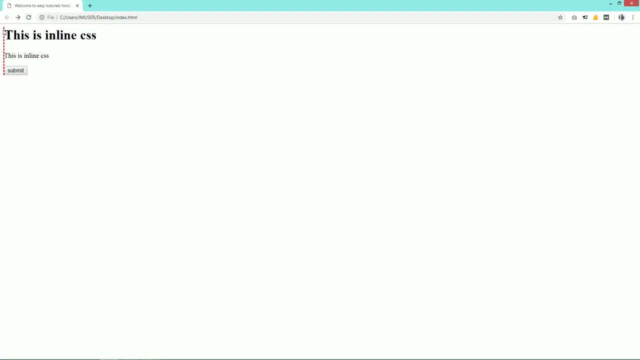 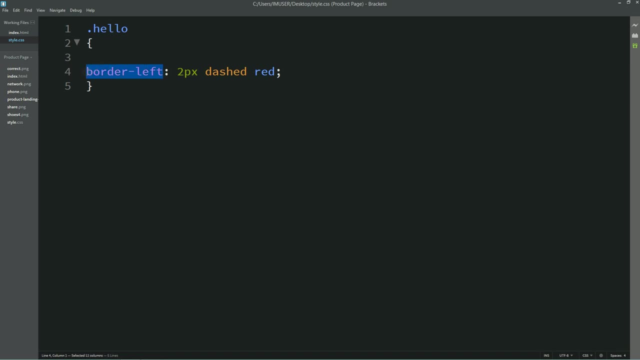 let me write border left now you can see this border in left side only. similarly, you can write border right also. let's see some other property. there are so many property about the border that we will learn while making the complete web page. first let me write one. 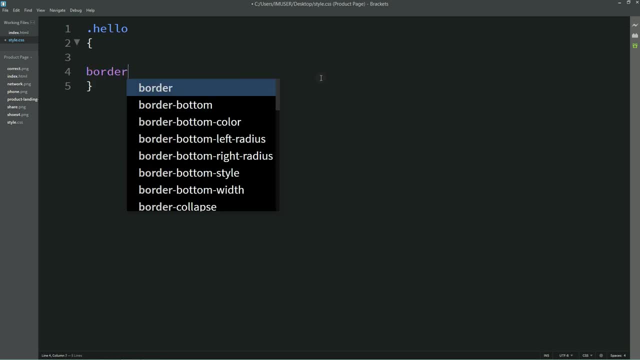 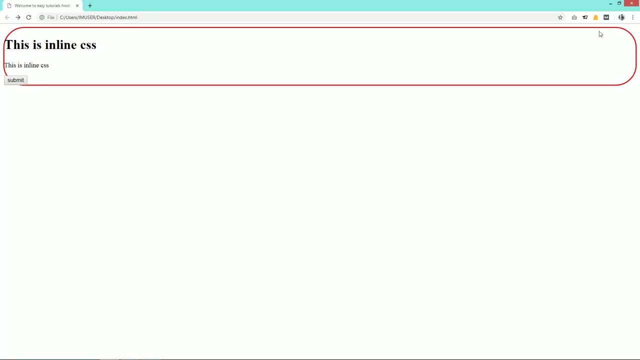 border here 2 pixel solid, and here I will write red as we did earlier. here we will define the radius of the border. so let me write border radius and let me write 50 pixel and reload the web page and you can see some radius at all corners. so this is. 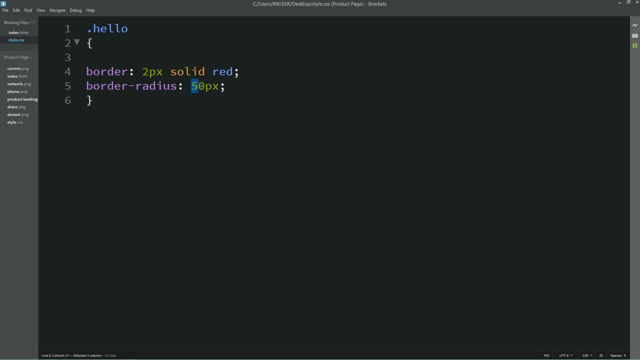 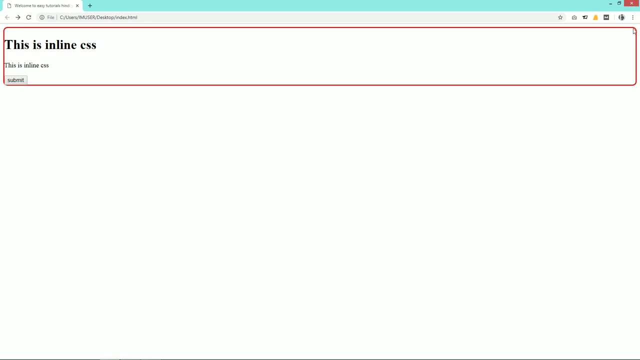 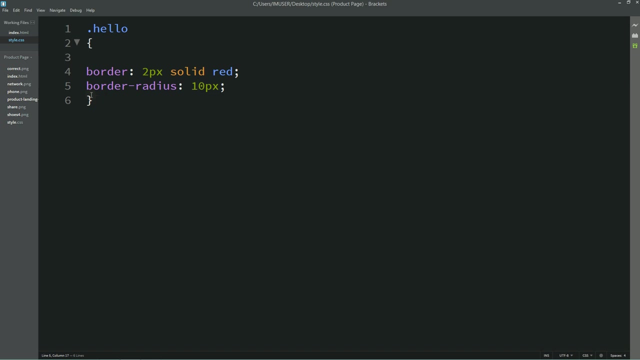 the radius 50 pixel. let me reduce this and you can see a small radius for each corner. so this is how you can add border radius, as we did this radius in every side, at every corner, so we can define the radius for a particular corner also. so let me write border top left radius. 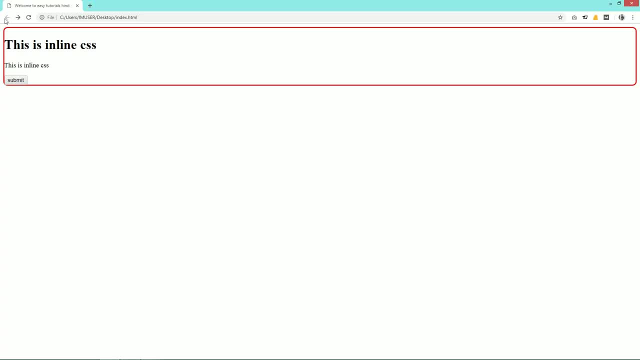 here I will write 30 pixel. reload the web page and you can see the top left corner is round, because the radius is applying for the top left corner, its only, and the other corner are a square. there is no radius. so this is how you can add the border radius in different. 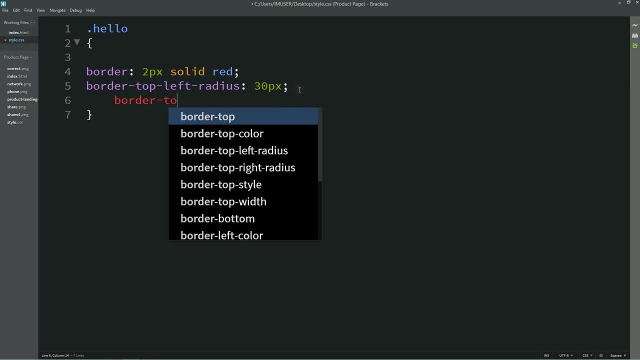 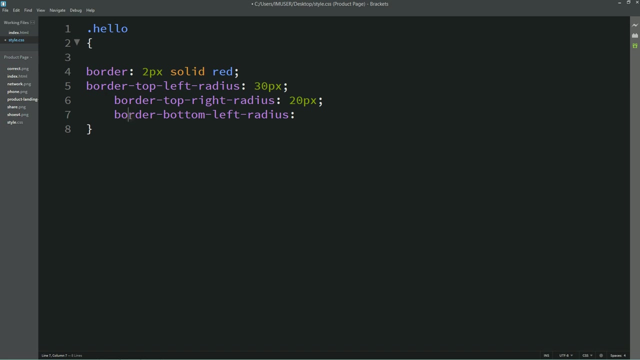 corners. let me write border top right radius, so you can apply the border radius in the top right corner. here I'll write border bottom left radius, then we can add border bottom right radius. so this is how you can add a different radius in different corner. now we will move on to different property of css. let me remove these codes. 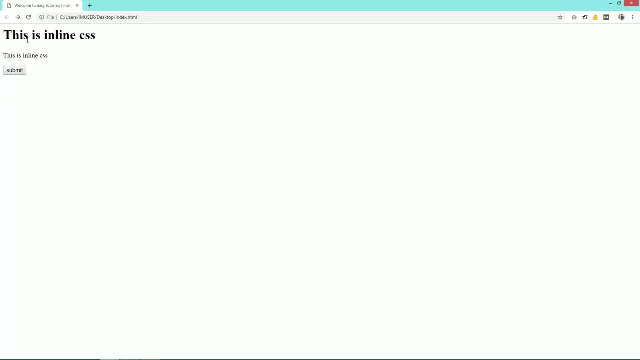 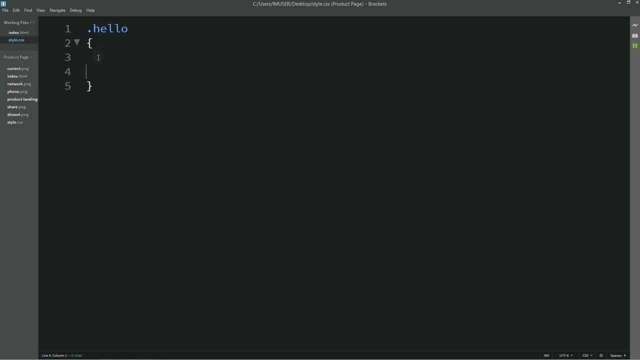 refresh the webpage and now you can see there is no css property here. and now I will tell you about cursor. let me write it here. here I'm adding cursor and you can see there are so many options. you can go and try each of it. let me select one of it, which is pointer. 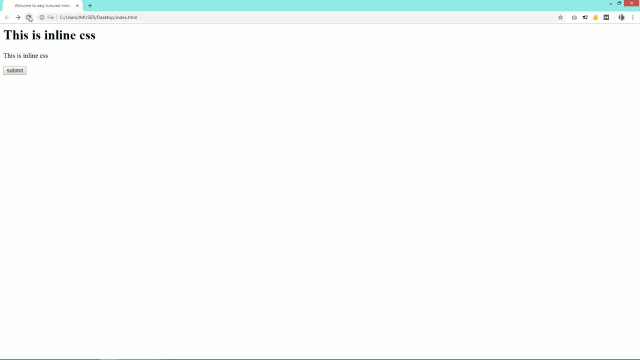 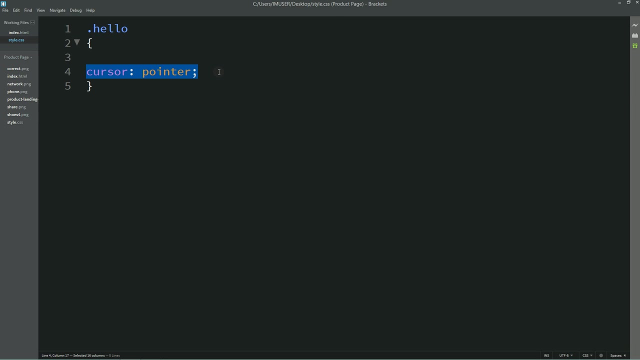 then let's me refresh the web page and you can see if our cursor is somewhere else. it is like this: when I take our mouse on this div, it becomes a hand icon. so this is how you can change the icon of the mouse pointer. let me remove this and let's check other property we can add. we can add float. 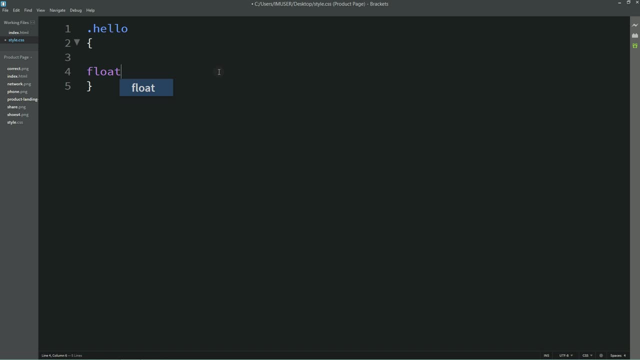 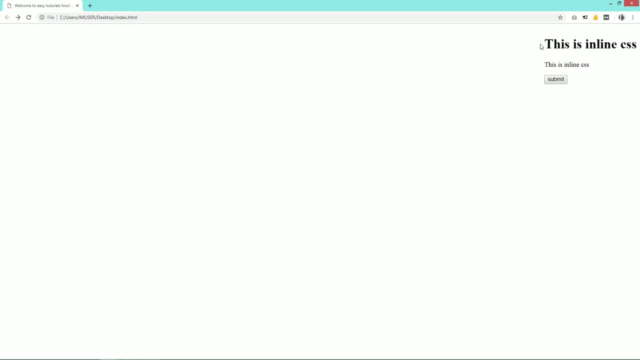 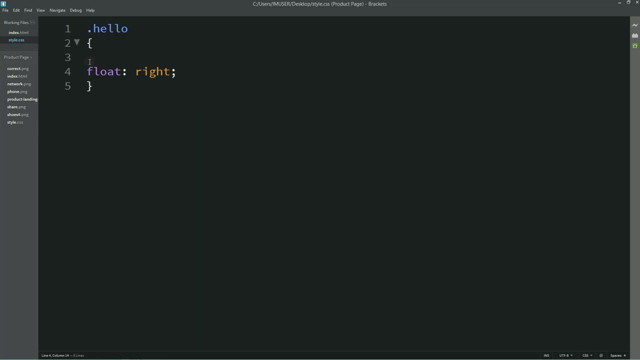 also in this float you can write inherit left, none right. so let me write this one float right. save these changes and you can see all the contents in the right side. so this is how you can align the content on your web page using the float property. let's remove it and we'll see other property which is display. 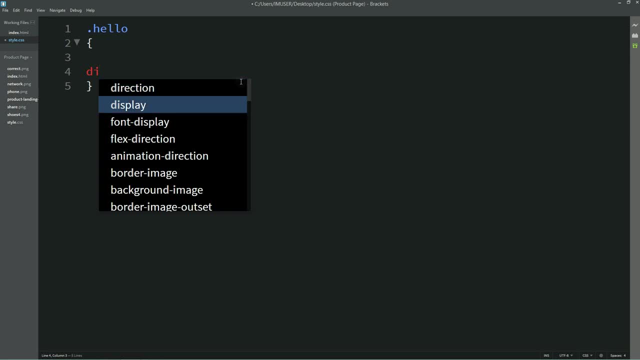 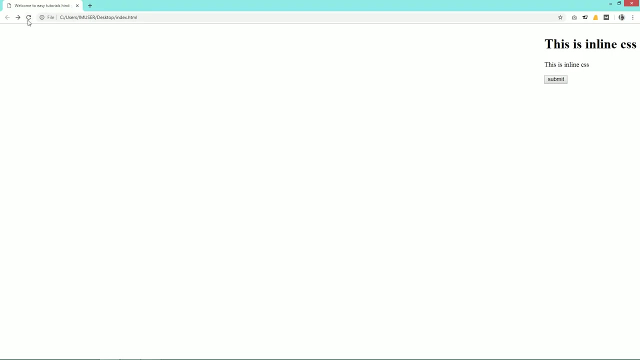 display property which is display. in display you can see there are so many options: block content, flex and inline, inline block- and i will show you more examples of this. for now, let me select one property. i will select display none. let me refresh the web page and you can see. 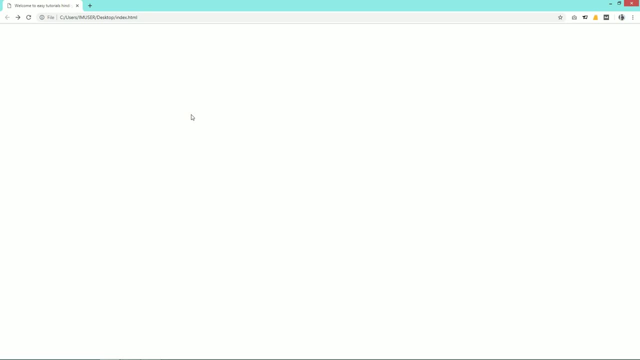 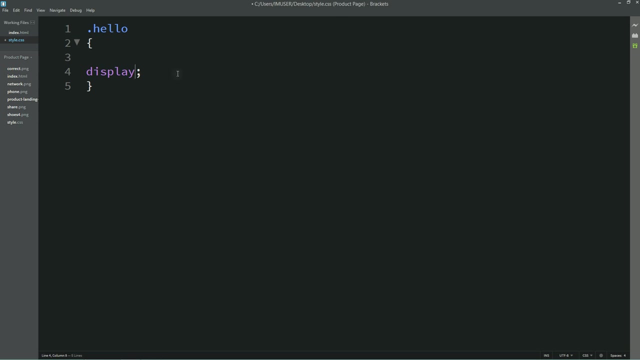 this content is invisible because we have written display none. so this is one property of display and later i will explain all property of display when we will create multiple divs. after display, we can write visibility. it is also very simple. we can write collapse, hidden, inherit, visible. so mostly you can use it to hide any content and again you can display. 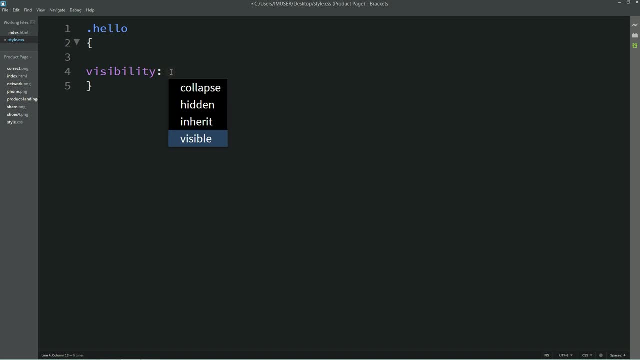 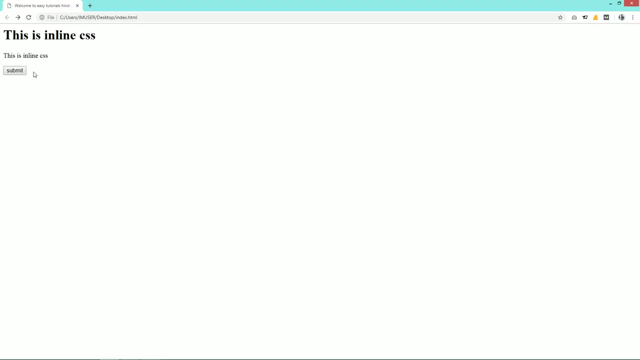 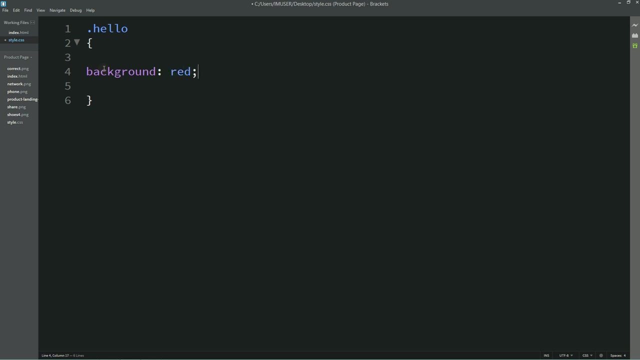 the same content and and and. let's learn about dimensions. so dimensions can be height, width, max width, min width and some other things. so let me refresh the web page and you can see we have written like this. so let me write one background here so that you can see the height. i'll write background. 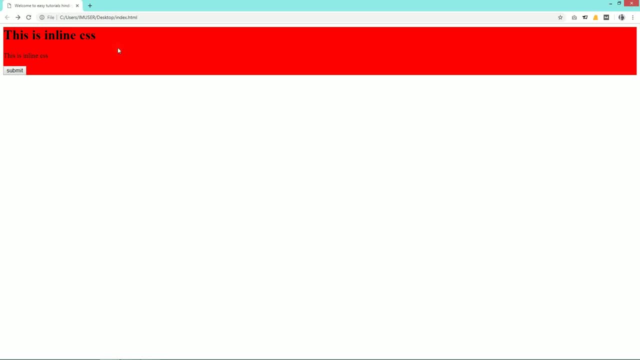 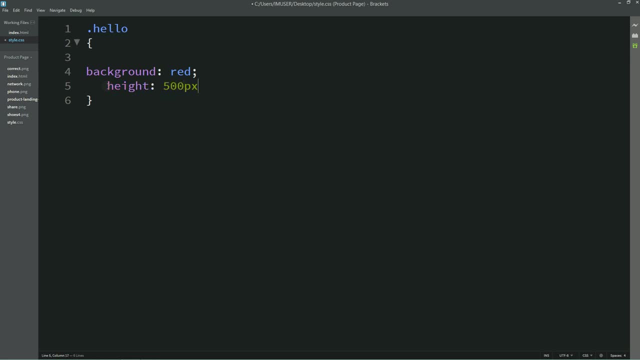 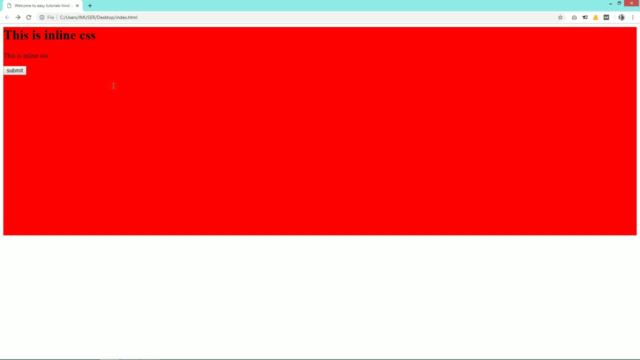 red and reload the web page and you can see its height is very small and if i want to increase the height, as we did earlier. so here i am writing: height 500 pixel. reload the web page and you can see the height has been increased up to 500 pixel. 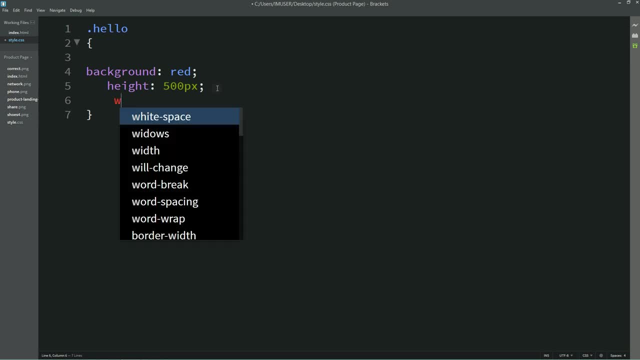 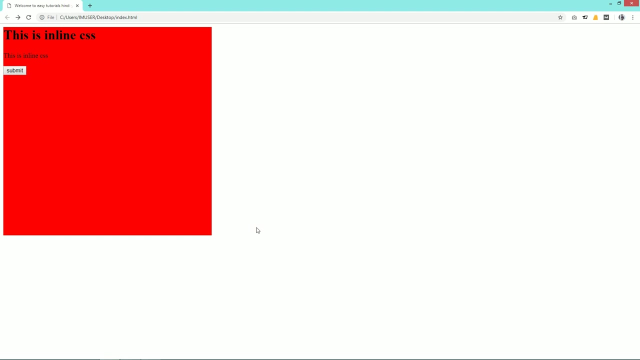 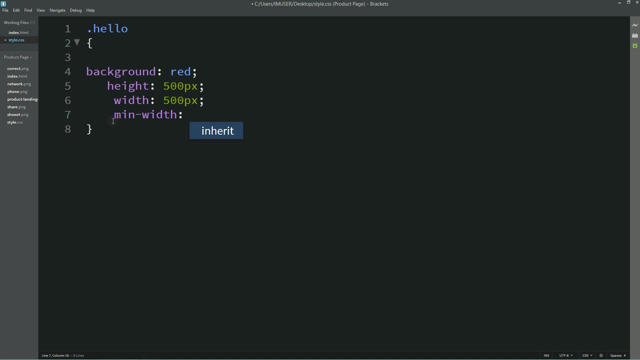 similarly, we can add one more property, which is width. let me write width. i'll write the same width, 500 pixel. and now you can see width is also 500 pixel and height also 500 pixel. so this is how dimension properties works. next i will write min width. in min width, what 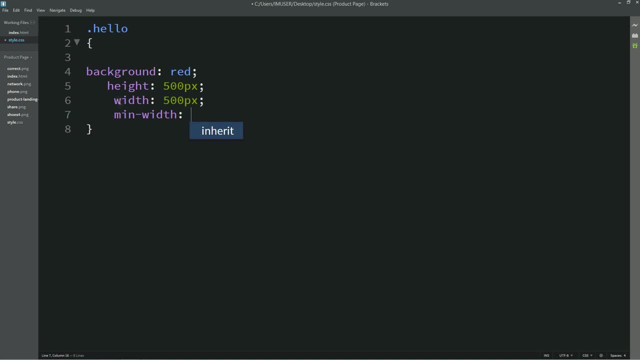 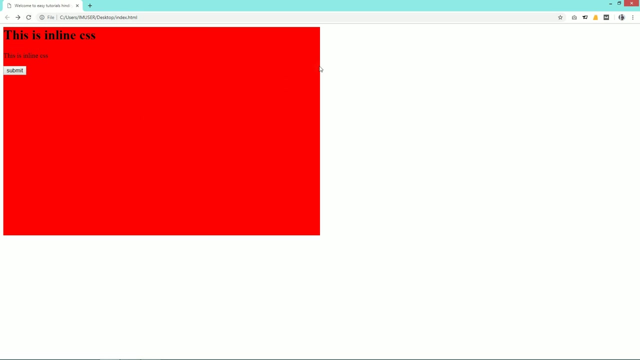 happens if we will set the min width at some value like 200. the content width will not go below that. so let me write this width in 50 percent and let me remove this min width and save these changes. reload the web page and you can see this: div width is 50 percent. 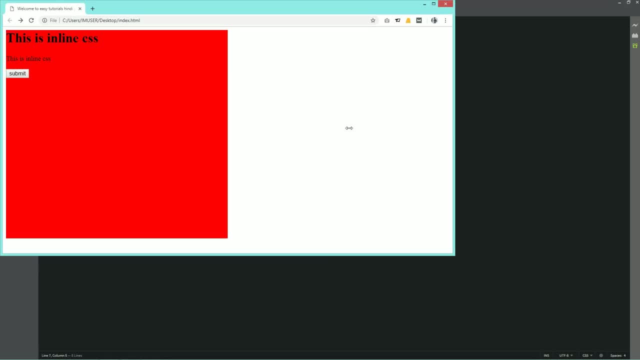 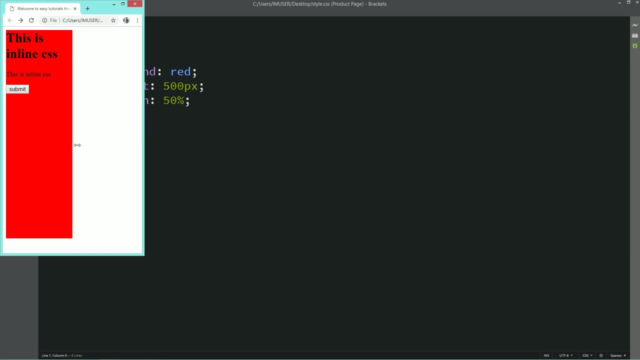 and as i will change the size of this browser, you can see its width is getting decreased, so it is 50 percent of the entire web page width right now, but it is very small, right, and suppose if we want this div to be a fixed size for a small device, then you can use the. 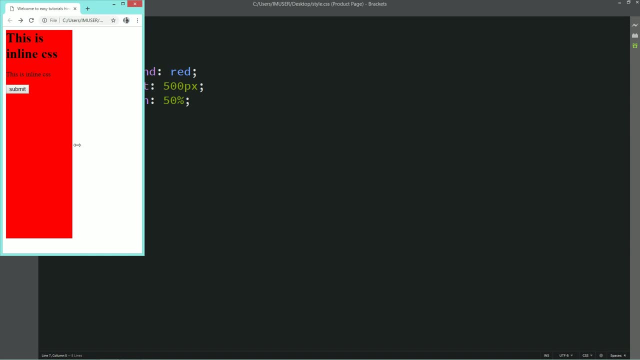 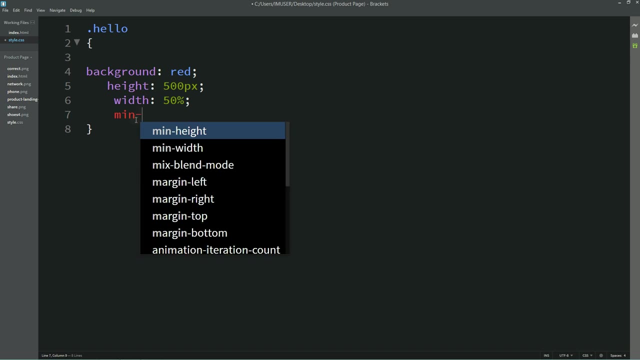 min width. so let me come back in the css file and here i will write min width. let me change the size of this browser to 300 pixel, so it will be 50 percent, but it won't go below the 300 pixel. let me refresh the web page and you can see its width is minimum 300 pixel. it can go above 300, but 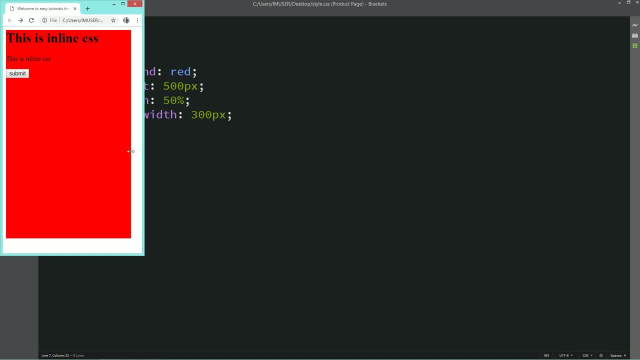 it cannot go below 300. this is how you can use the min width also and max width also. when i'm talking about dimension, we'll see some other dimensions also. we can use the line height also. in line height we use to add some space vertically for a text or paragraph. so for this text you can. 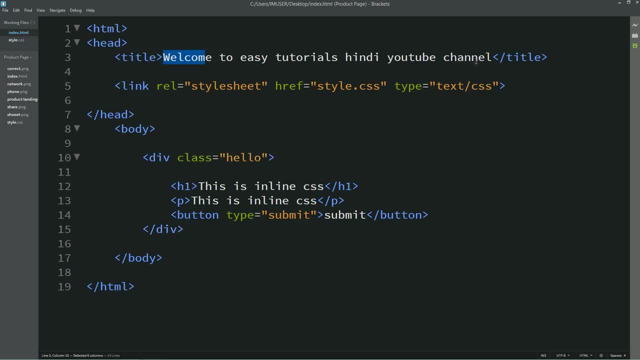 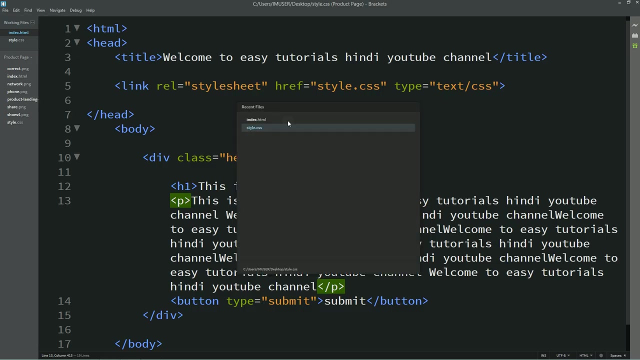 see i will add more text. let me copy here. i will add some more text in this p tag. let me refresh the web page and you can see these text. it is in two lines and how line height works. let me show you. come back to the css file. 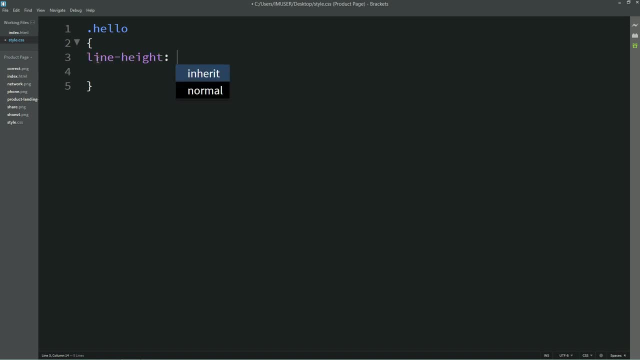 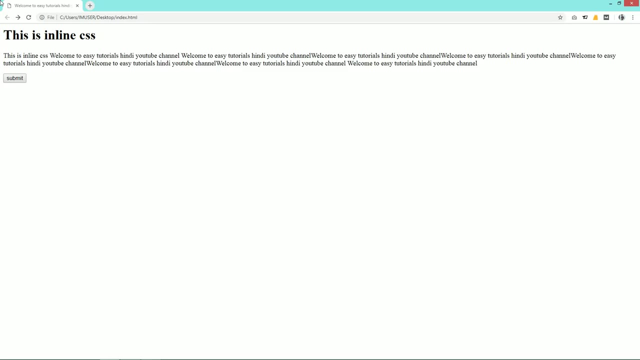 for this one. i will write line height. i'll write one value: 30 pixel. reload the web page and you can see, as i reload the web page, the vertical space between these two lines got increased. you can see the blue space. this is the line height. so this is how you can add a line height for a text to add some extra space from. 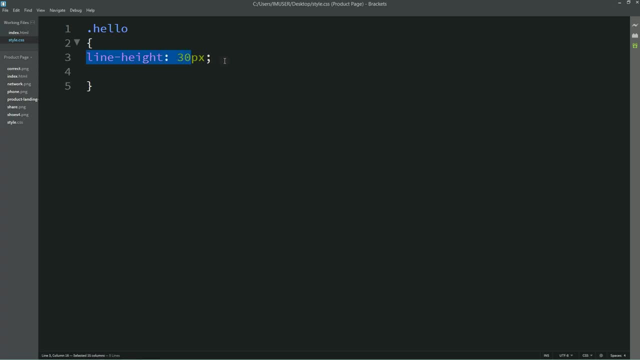 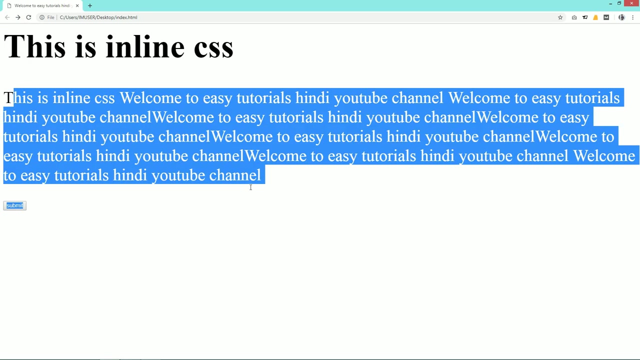 vertical. let me remove this and we will talk about fonts. for font, let me use font size. font size, as i did earlier. we can write any value here. i will write 40 pixel so that its font got increased for this p tag. let's come back and 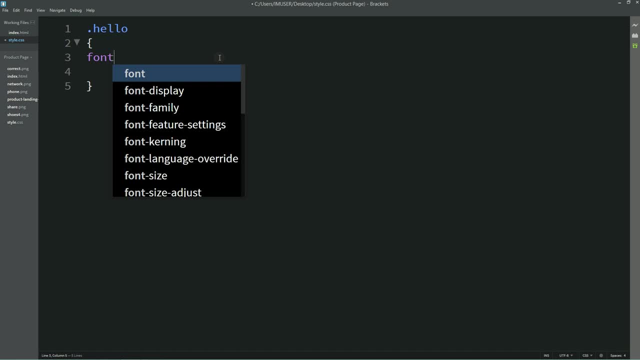 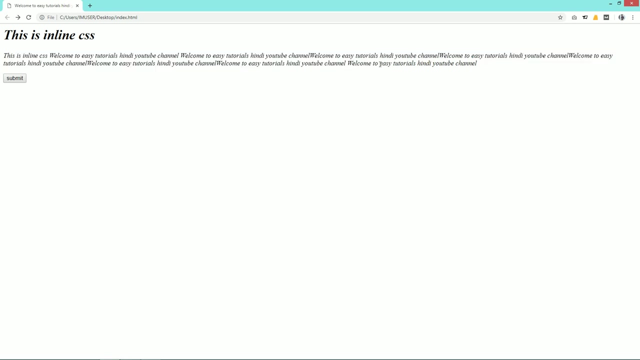 we will remove this and see what we can add else. we can add a font style, and in font style you can select italic, oblique, normal. so let me select italic. reload the web page and you can see the entire text in italic font style. so this is how you can add a font style. next, we can add font family. 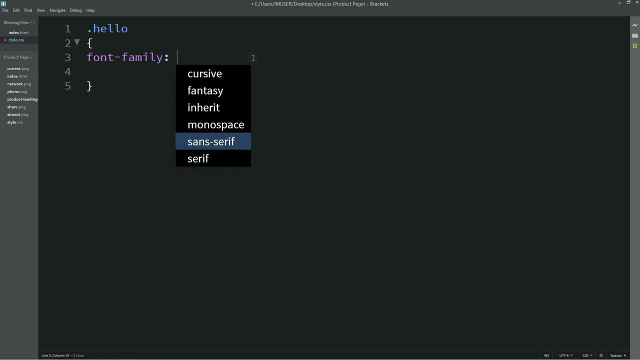 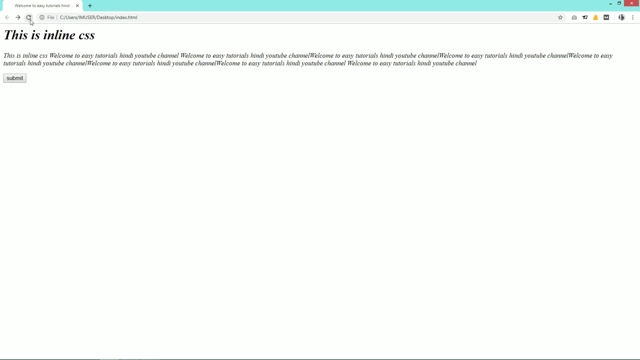 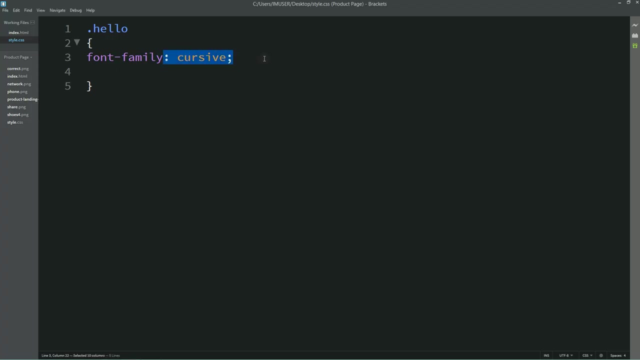 and in the font family, by default you can add these font family. let me select this one cursive, reload the web page and now you can see different font family on this web page and let me change it again. i will write some other font family. i'll write fantasy. 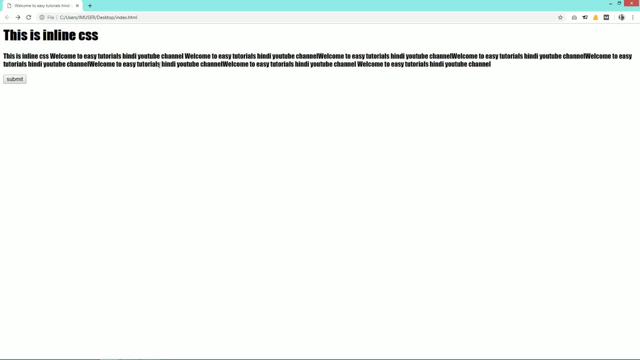 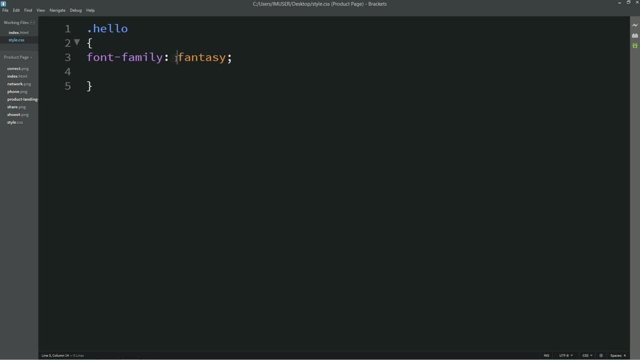 reload the web page. now you can see again different font style on this web page. i mean font family. so we have limited font family in default. if you want to use a more font style, then you can go for the google font. and how to use the google font: i will create a separate video for that. 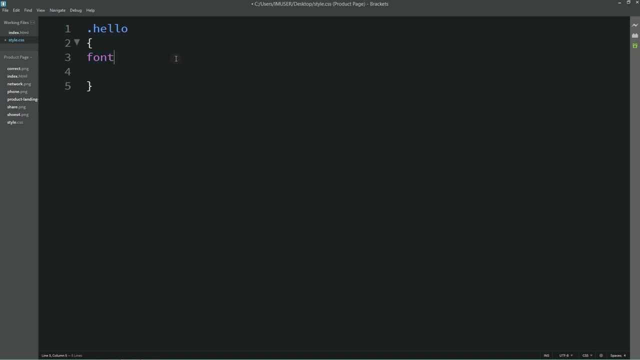 in further videos. let me remove it. after understanding this font, we will see how we can style the list, as we did earlier. we created some list, so let me come back in the html file and here we will create some list. let me remove this and here i will write one ul tag and this ul i will. 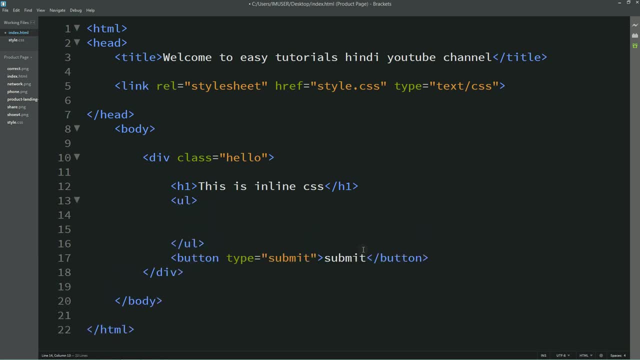 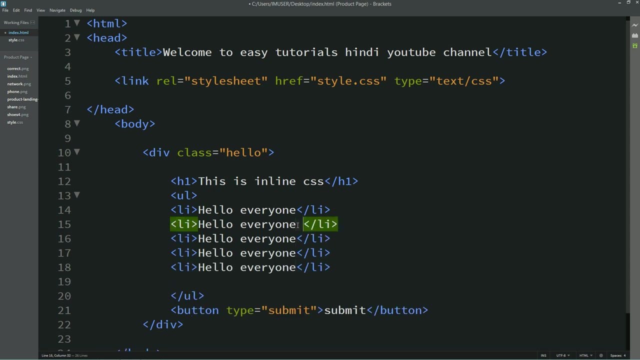 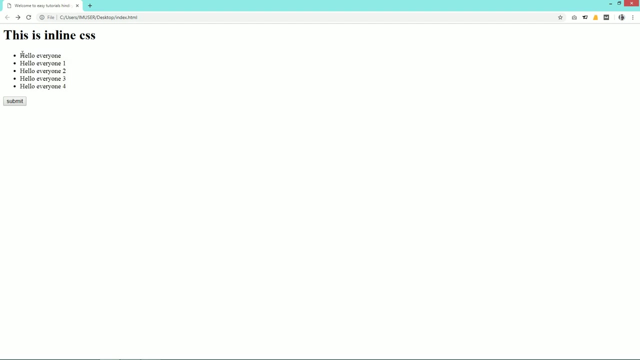 write one list item and some message here: hello everyone. let me duplicate it and we'll write different title. so let me just write one value: hello everyone. one, two, three and four. so this is one unordered list. reload the web page and you can see these lists on this web page. 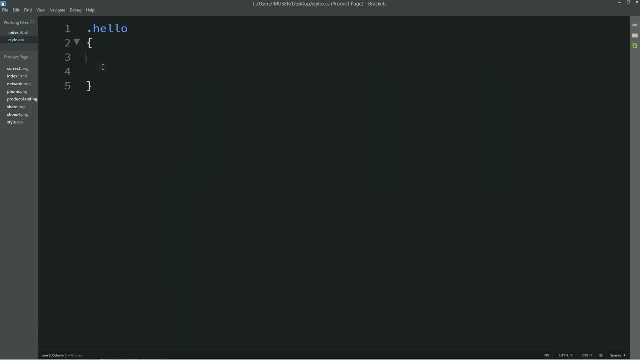 now let's see how we can style this list. so come back in the css file. here we will add another one. let me remove this rom- and simply we will write ul, because we are applying the css code on ul. so here we will write ul: list style. 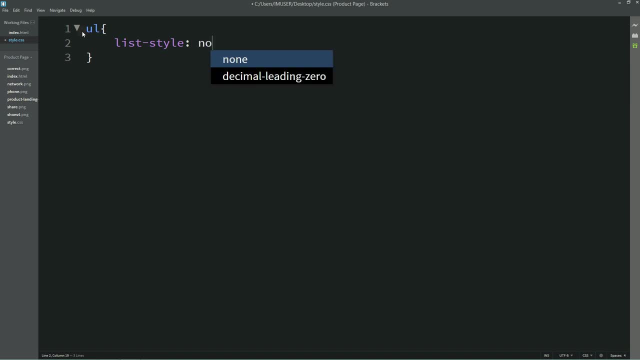 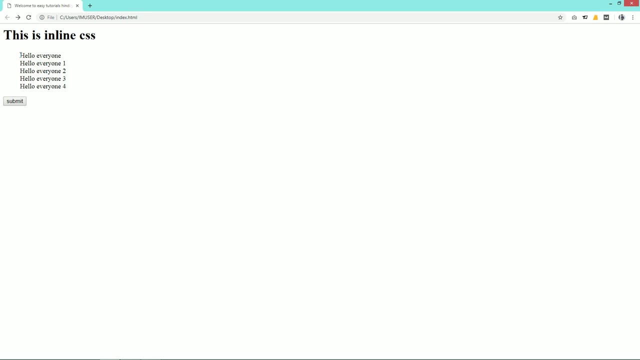 and in list style you can see we have a more option. so let me write none and reload the web page and you can see the bullet points has gone. this is how you can remove the bullet points, and even you can replace the bullet points with some other icons. so let me come back in the CSS file and instead 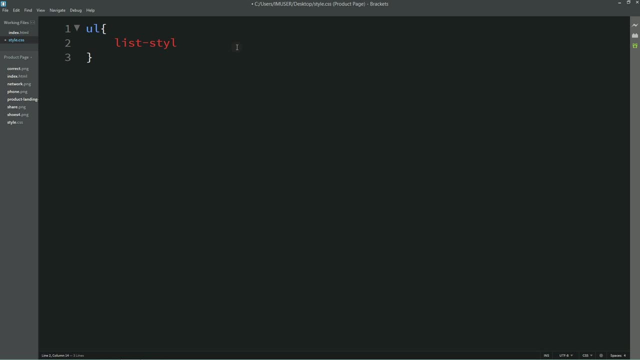 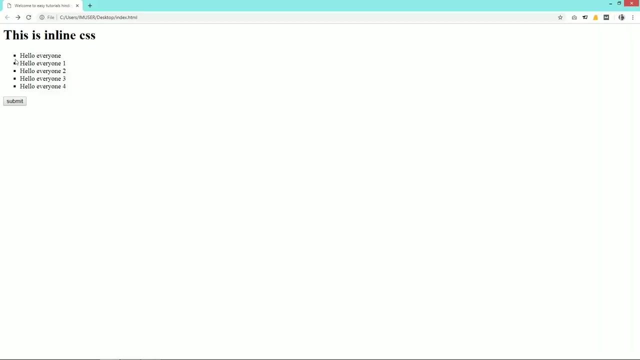 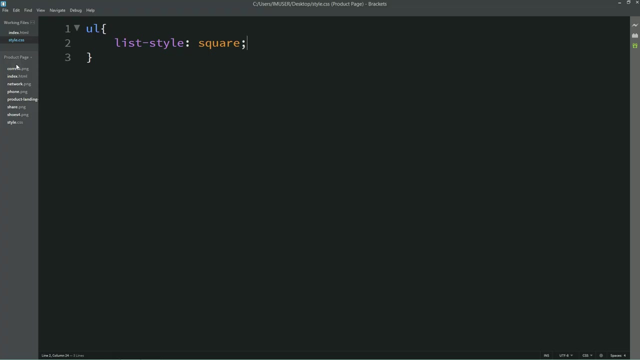 of none. let me write list style and if you can select from this one, I will select a square, save these changes and reload the web page. now you can see square icon before each list item. so this is how you can add style in your list. now we'll talk about margins. for that, let me use this class name. 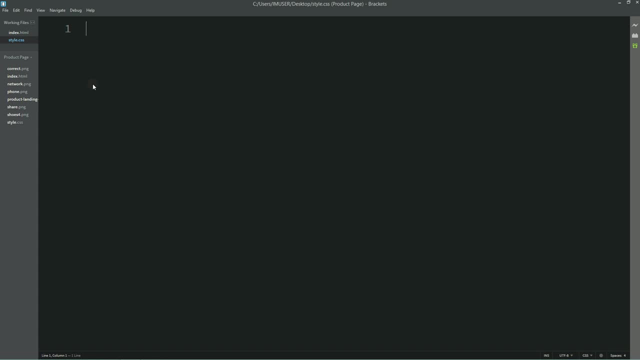 hello. I will write it here in this CSS file: dot. hello. and let me add one border here so that you can see the spacing clearly. so let me add one border. I will add border for two pixels. so let me add one border. I will add border for two pixels. 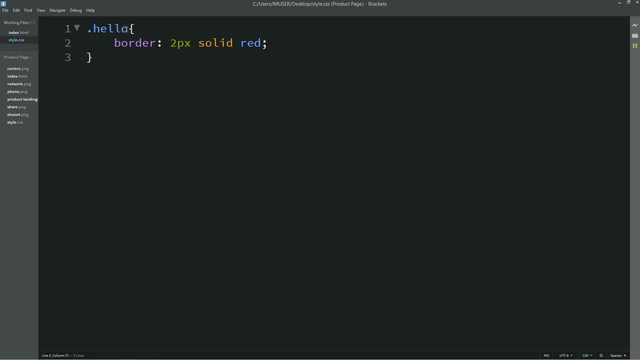 so let me add one border. I will add border for two pixels, solid and red color, as I did earlier. reload the web page now. you can see one border around this text. now we'll see how the margin and padding works. so here we will write margin: 40 pixel. write this text and reload the web page and you can see. 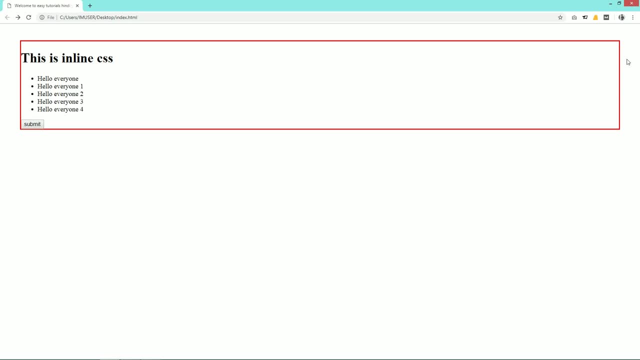 it will add 40 percent space from each side. it will add 40 pixel from top, left, right and bottom right and this margin is adding these space outside of this division. and this is the difference. when we will use padding instead of margin, let me write the padding. also, in the padding I will write 40. 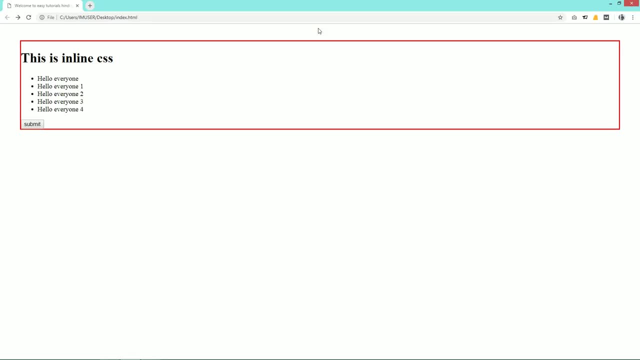 pixel and save these changes. reload the web page and you can see, as I will refresh the web page, you can see 40 pixel space between these division between this border. so the margin is adding a space outside of this div and padding is adding a space inside of this div and this padding is. 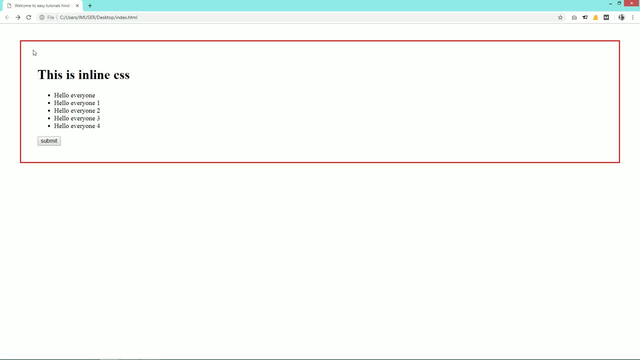 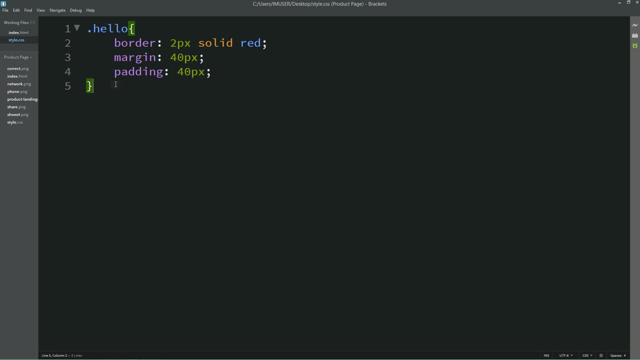 also adding 40 pixel space from all sides. it means from top, bottom and left right. let me tell you how you can write the margin in other way, so let me remove the padding, because the process will be same for both of it. for this margin, we have added 40 pixels, so let 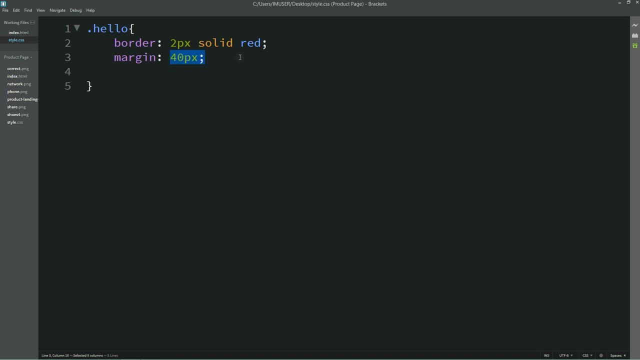 me remove it and here we will write the margin one by one. instead of margin, here we will write margin left. in this left we'll write margin left- 40 pixel. then we'll write margin top. let me write 100 pixel. you can write different if you want. like this: you can add margin from left, right, top or bottom. 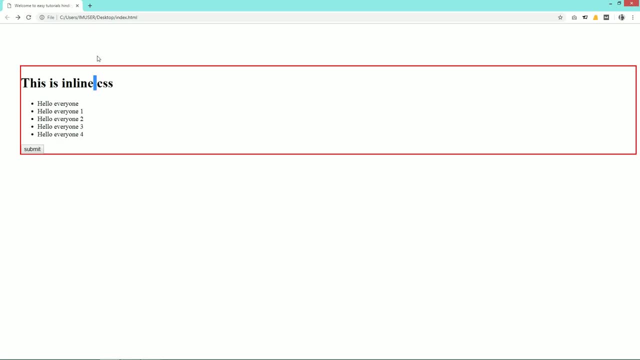 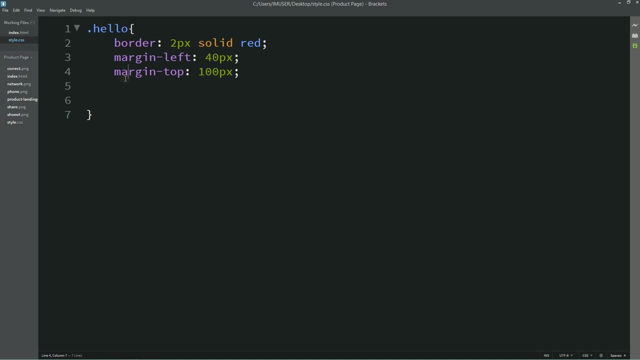 as you see, from above it is motor space because we have added 100 pixel, and from left side it is 40 pixel and there is no margin. from the right side, you can add different value for each side, and now I will tell you another option in which you can add all the margin in single line, as I 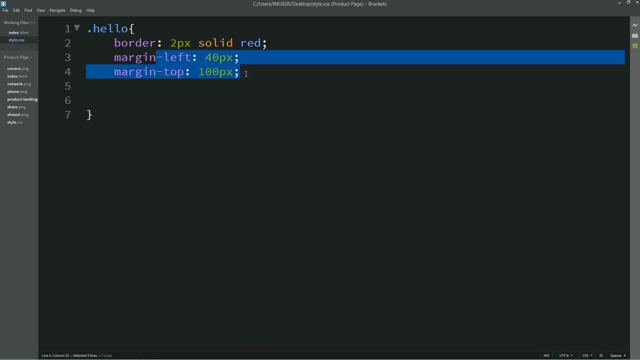 did for border. we wrote all the things in one line so we can do the same thing in margin. so in the right side we will write the value for value in clockwise direction. so first value I am writing 100 pixel. it will be for top. if we will rotate again clockwise then it will be right side. so 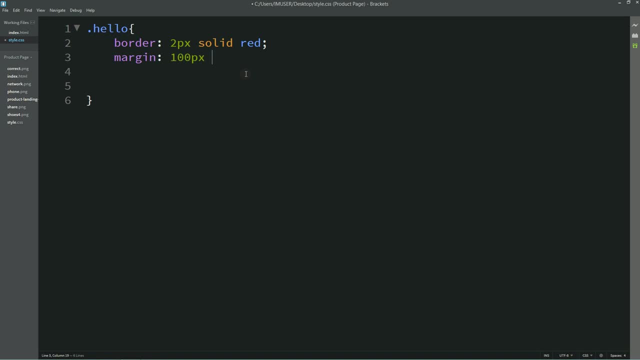 in the right side we can write another value. so let me write a 200 pixel from the right side and again rotate in clockwise so we will come to the bottom. so here we will write the value for bottom. so let me write 10 pixel in the bottom, then we will come to the left side. so if we want, 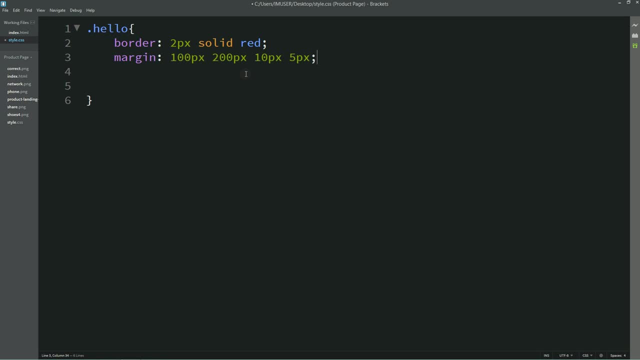 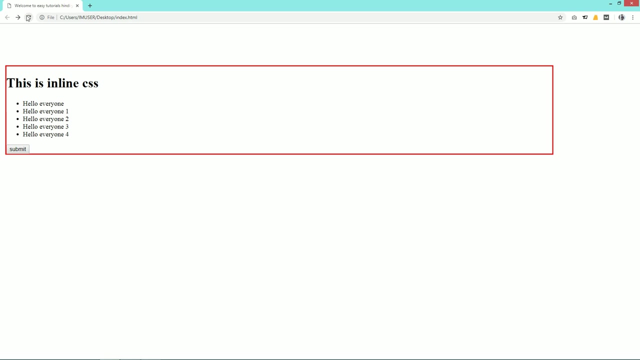 5 pixel from left. I'll write 5 pixel. so this is how you can add a different margin in one line itself and we are adding different margin. let me refresh the web page and you can see different margin from top and right and left and bottom margin is not visible because we have lots of a space in the bottom. 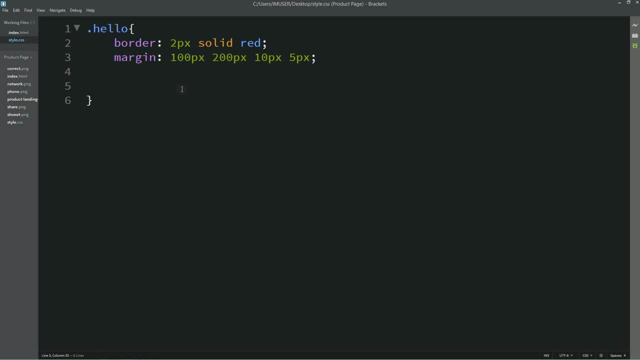 so this is how you can add four value here. next, we have more options also suppose: uh, we, we want the equal value for top and bottom and equal from left and right. so instead of four value, we can write two value only. so let me remove the two value and what it will does. so it will add. 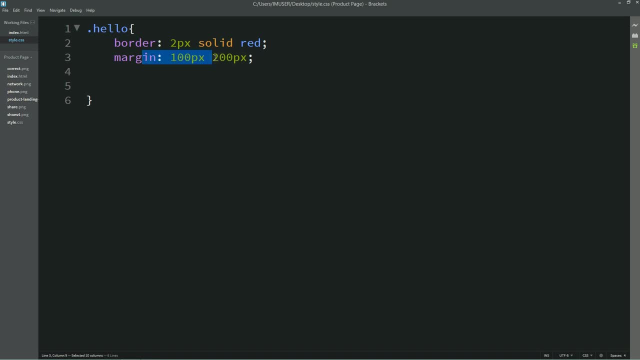 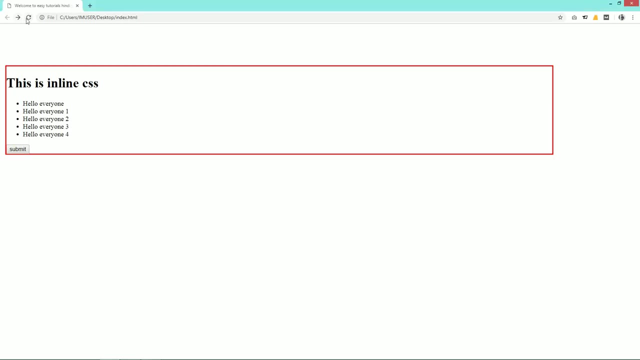 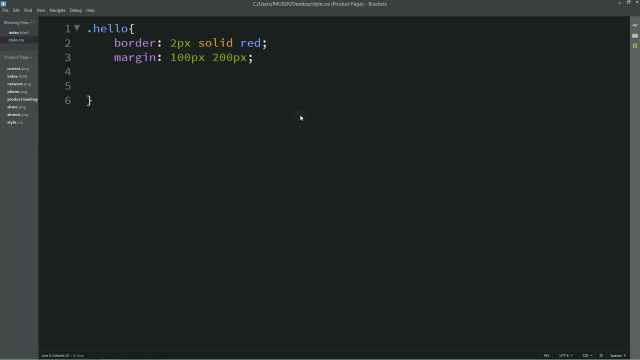 100 pixel a space from top and bottom and 200 pixel a space from left and right side. so, using these two value, let me refresh the web page and you can see we have margin from top- 100 pixel, and from the left side and right side it is 200 pixel. so this is how you can apply top and. 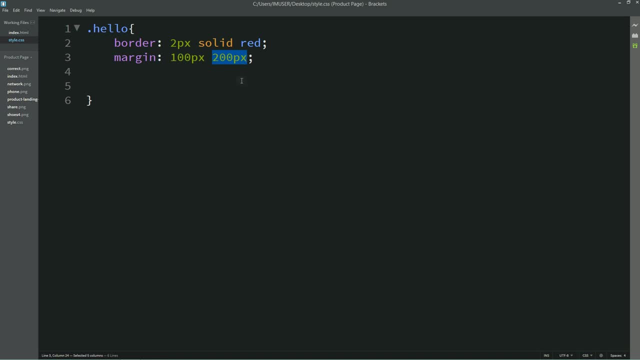 bottom and left and right. suppose we want a different margin from the bottom and we want the the left, right same. so here we can write three value. so the first value will be for the top, second value will be for left and right side and the third value will be for bottom. so let 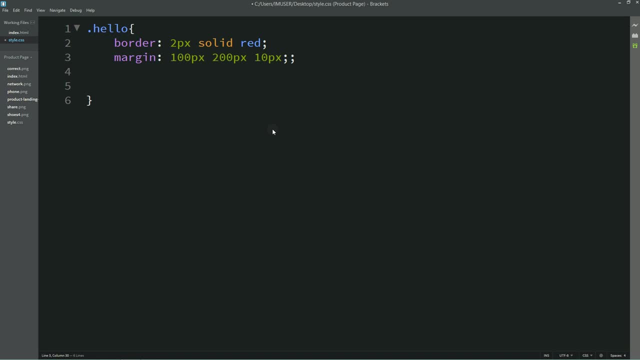 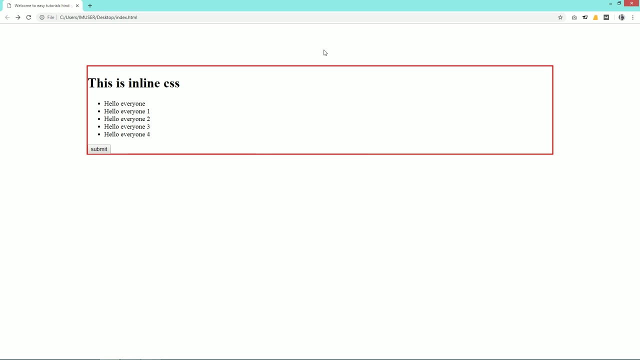 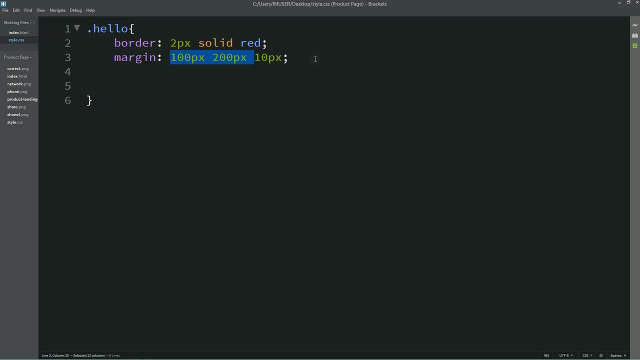 me write bottom 10 pixels. so this is how we can write three value. reload the web page and you can see the same value, because top is same, left, right is same and we have added 10 pixel at bottom, which is not visual because we have lots of space at the bottom. and this is how you can add margin. 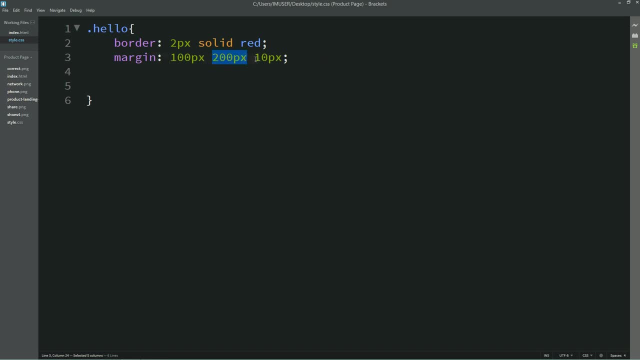 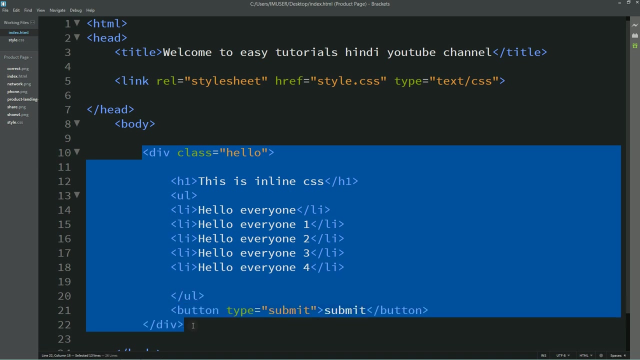 the same way, you can add padding also in one line, but the difference is that the margin will add a space outside of the box and padding will add a space inside of the box. next we will see the property for outline. let me remove this and come back to the HTML file. let me remove everything from the HTML also, and here. 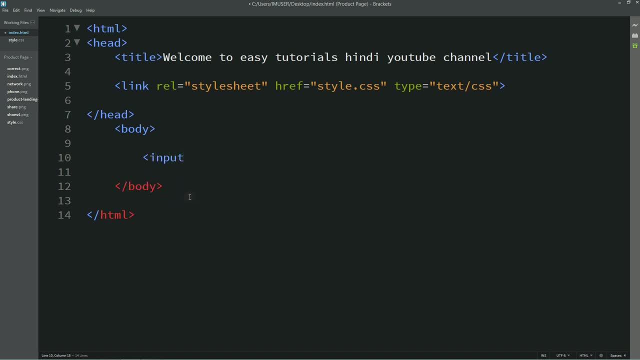 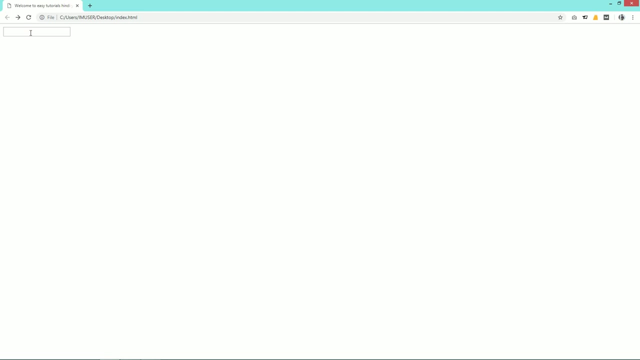 I will add one input box. I am adding input type and type will be text. that's it. reload the web page and you can see this input field here, and when I click here it's loading again and then I am going to add any text that I want to add. 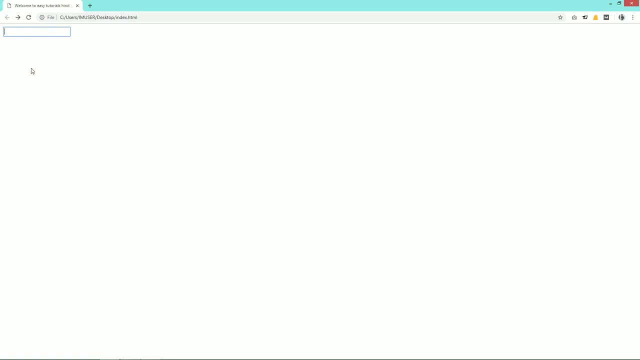 or I can filter them and tolerate it. if I want to edit anything, then you can see it's loading again and then I am going to add any text that I want to edit here. you can see one color at border, which is outline, so we can change this outline. we. 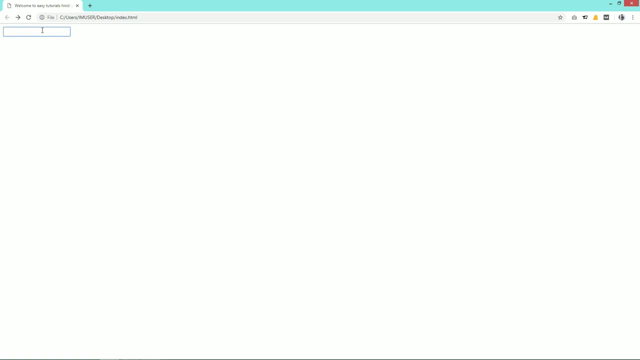 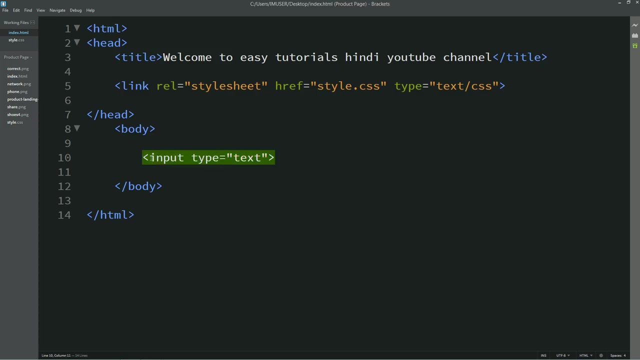 can hide this outline, which is right now in blue color. for that we will just come back here. in HTML file, copy this tag input and we will add this tag here because it is HTML tag, so we don't need any dot. simply write it here and here we. 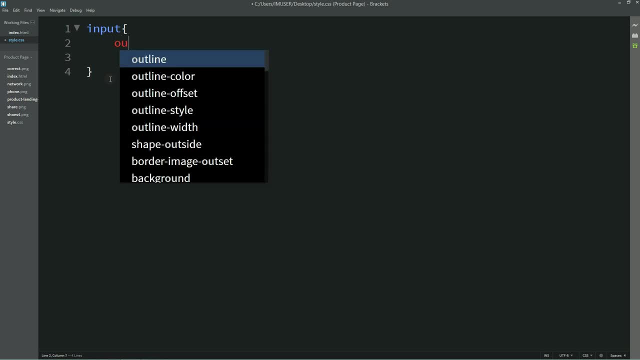 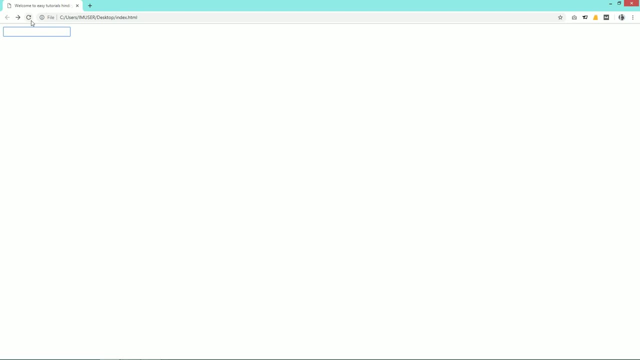 will write outline and we can write the outline none refresh the web page and if I click here, there is no outline coming correct because we have set outline none. so this is how you can hide the outline if you don't want and if you want to change the color here, you can change it to outline color. 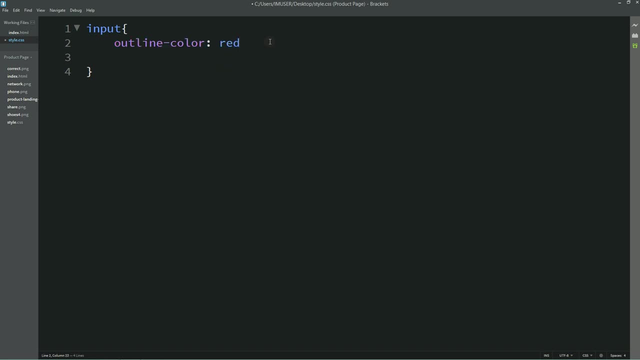 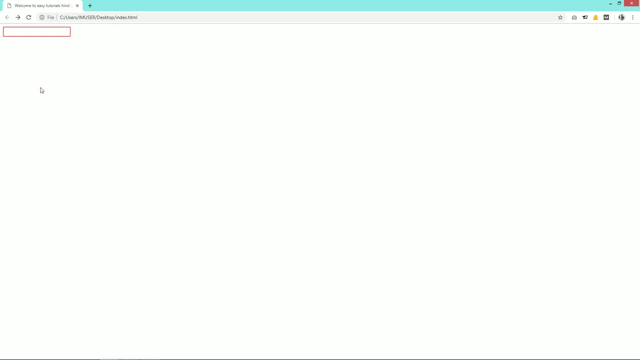 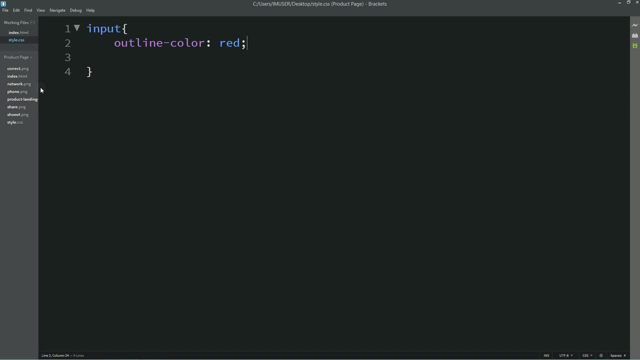 and select any color that you want. let me write red below the web page and if I click here, you can see red border which is red outline. so this is how you can set the color of outline. now we'll tell you some text property. so we, if we have, 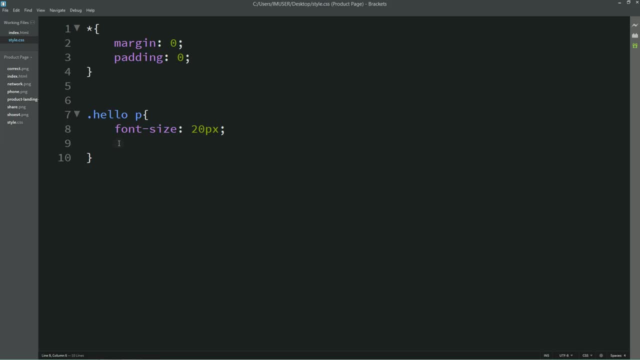 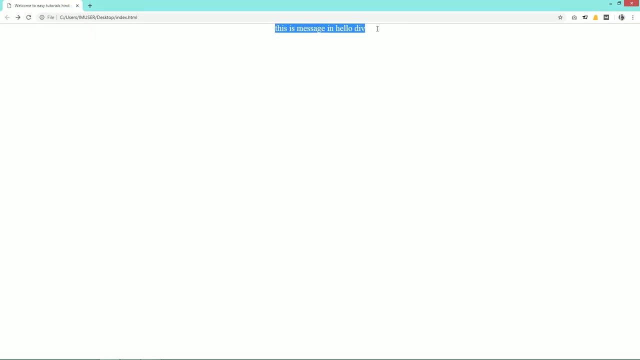 a text in one div. here we have applied a font size 20 pixel. let me write text align Center. you can write the text align left, right. also justify: let me select text align center. reload the web page and you can see this text in this center. let me. 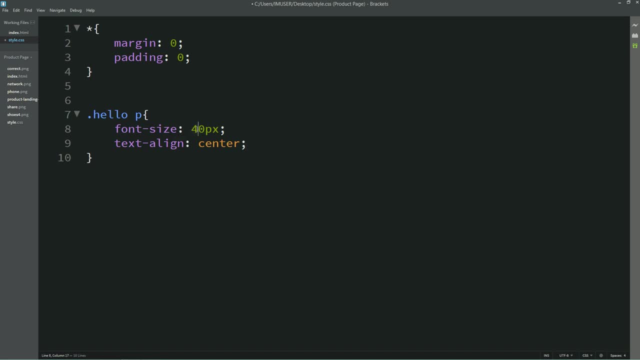 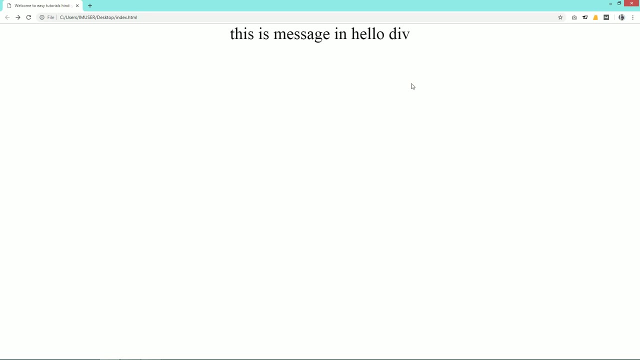 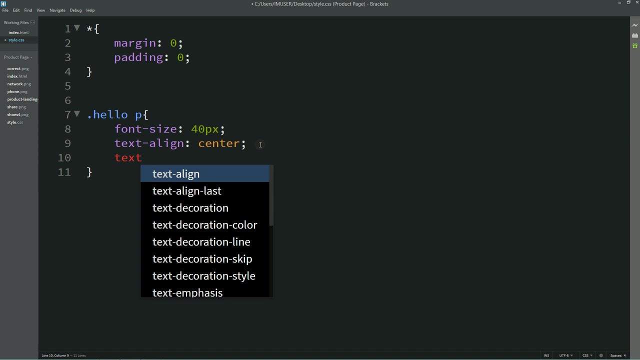 increase its font size. now it is clearly visible. so this is how you can add text: align for the text. next to: let's see what we can add, and- And we have already talked about line height- we can add text decoration And text decoration. you can see. you can add inherit none and other things. 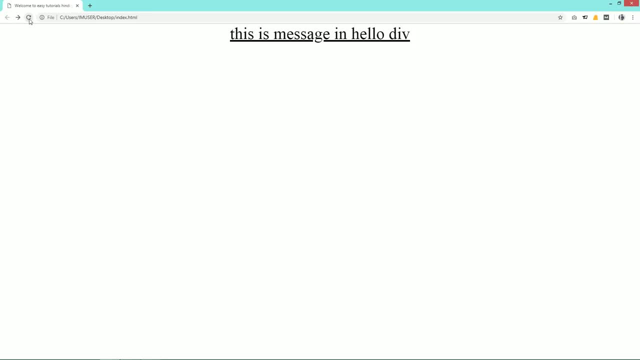 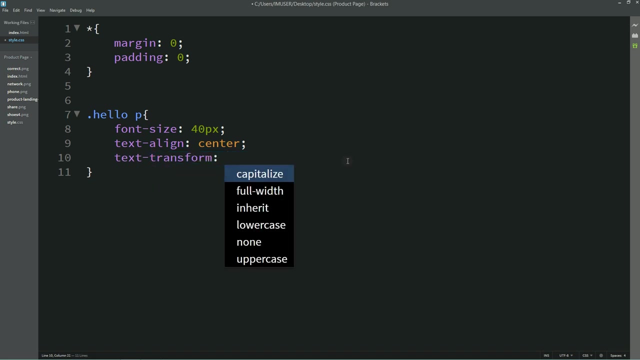 So let me select this one underline, reload the web page And you can see one bottom line below this text. So this is how text decoration works. Let me remove this, and here I will write text transform. In text transform you can write capitalized: uppercase, lowercase. 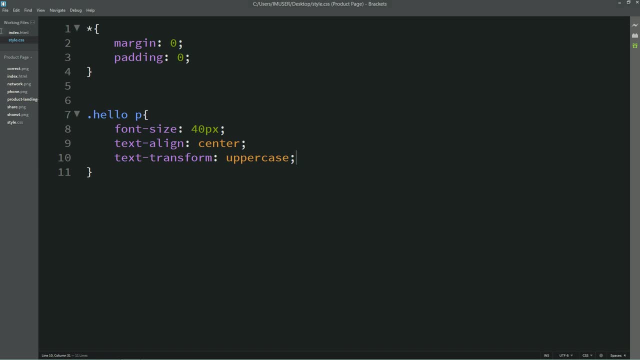 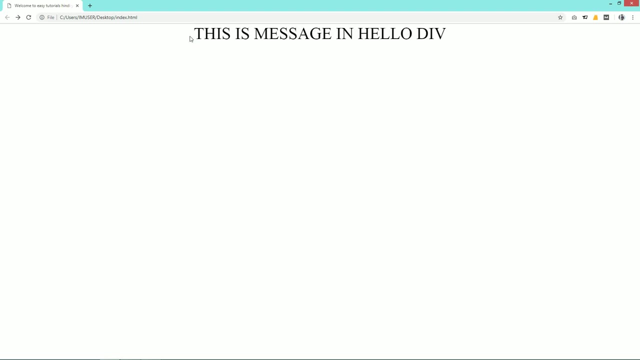 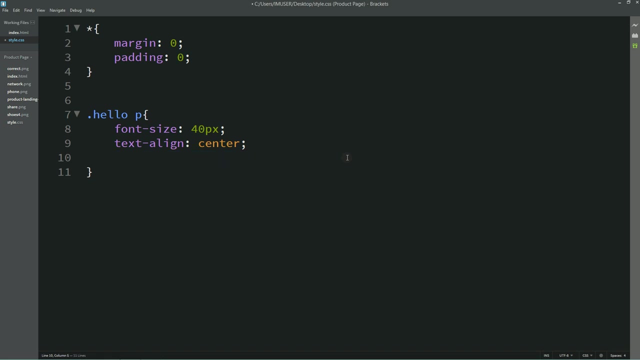 Let me select this one uppercase and save these changes, And now you can see all text in uppercase. So this is how text transform works. Let's see what we can add in text. So let me remove this one, And here we will add letter spacing. 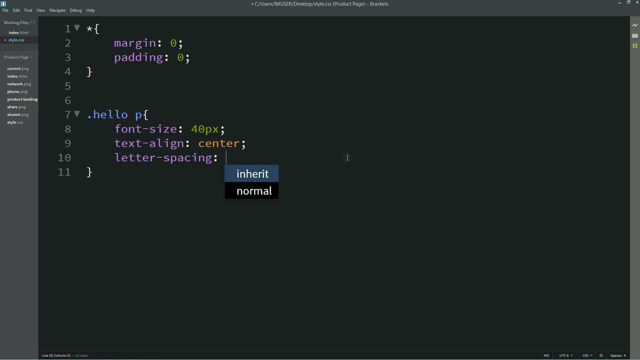 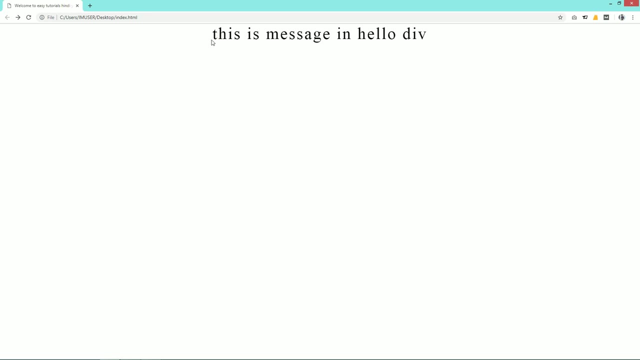 In the letter spacing I will write one value. I'm writing three pixel. Reload the web page and you can see a small space between each letters. DIV. you can see a small space between D and I, a small space between I and V. 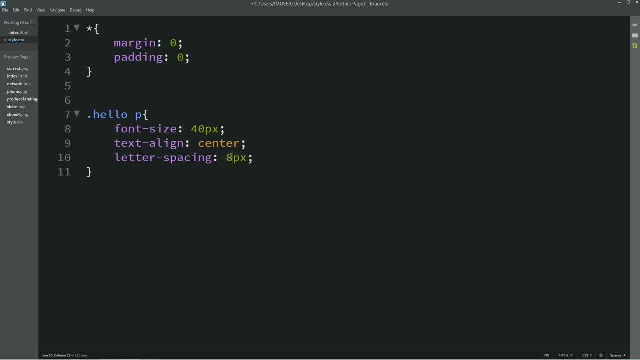 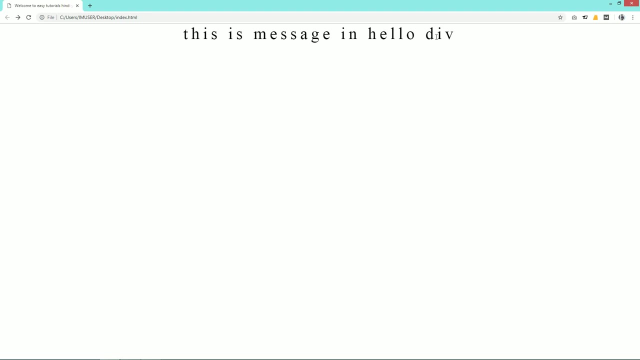 Let me increase it. I will change it to 8 pixel. Reload the web page and you can see the spacing got increased Between this D and I. let me increase it 18 pixel And again you can see this space is increasing because we are increasing the letter spacing. 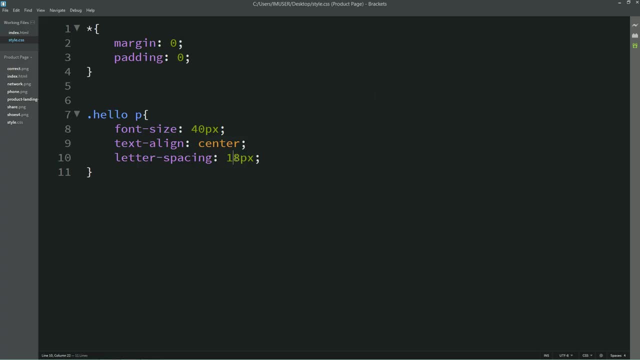 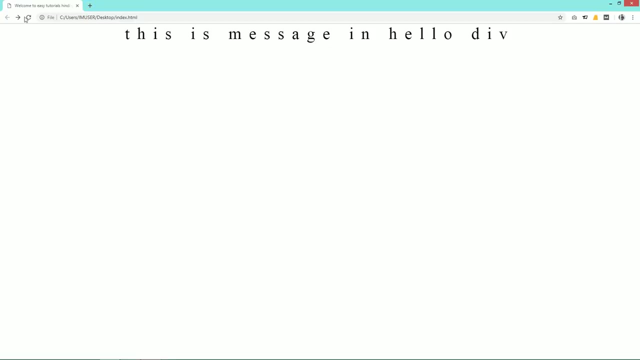 This is how letter spacing works. Remove it And instead of letter spacing, let me add word spacing, And I will add word spacing 30 pixel And reload the web page. Now you can see the space between each words. You can see this and is: 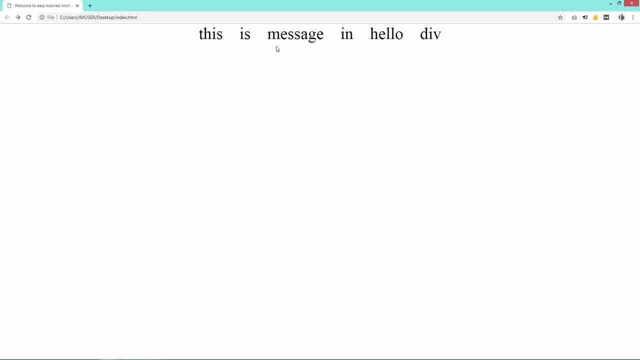 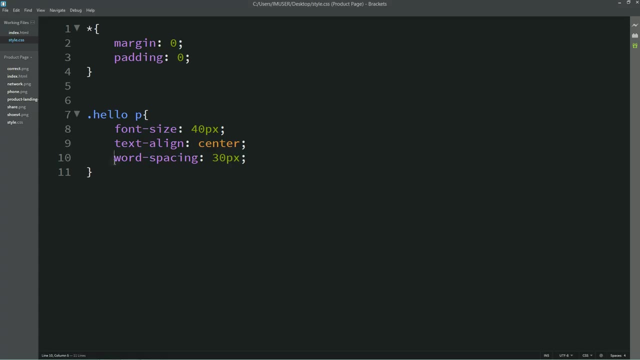 There is some space between this and is, So all words are far from each other because of word spacing. Now we'll see the next option In the text: what we can add. We can add text shadow. Let's remove it, And here we will add text shadow. 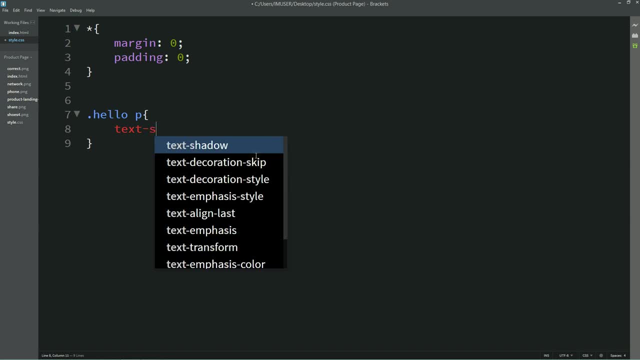 And if you will create a div, we can add box shadow also similarly. So let me add text shadow here And here. we will write three value. Let me write 20 pixel. I will teach you how to get these value. Then we'll write 10 pixel, 5 pixel. 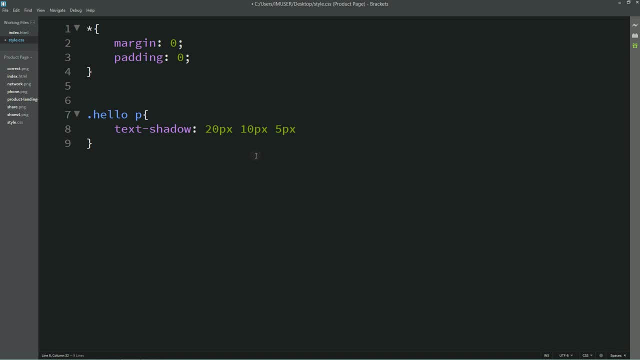 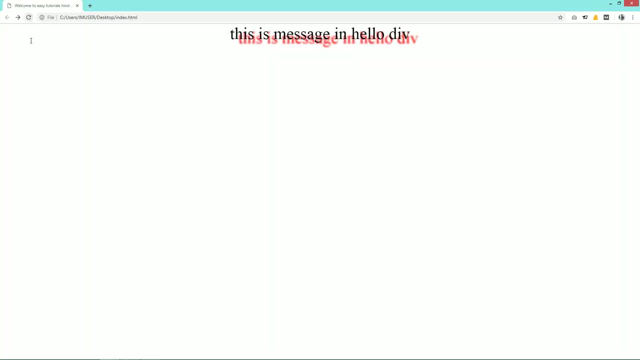 Then we have to write color. So color- I'll write red. Reload the web page. This text is very small So let me increase it again. Font size: 40 pixel and text align center So that you can see it clearly in the center. 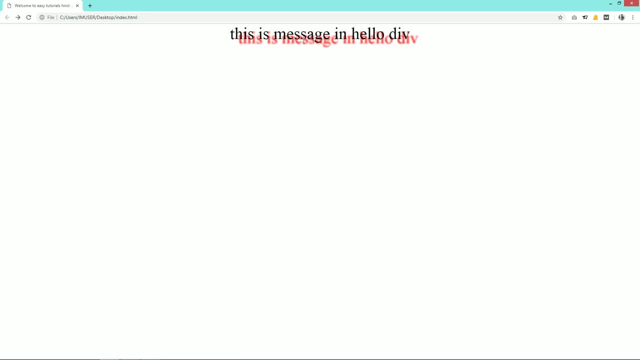 So right now you can see this text in black color and there is shadow in red color, But it is not looking that good. You can change this shadow easily, So right click here And select inspect. Here you can see we have font size text align. 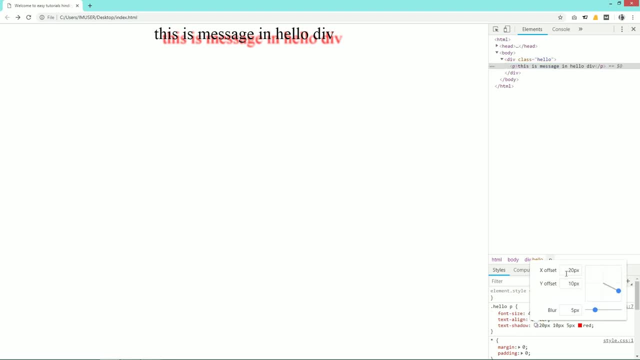 Then we have text shadow. In text shadow you can click on this icon and you can see it is X offset, which is 20 pixel. So if you don't want the X offset, you can change it to zero and you can increase or 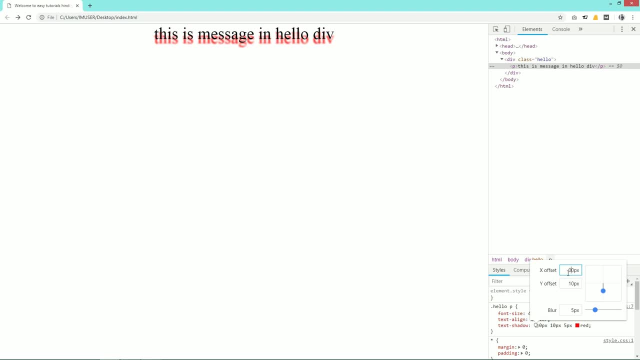 decrease it. Now we have the Y offset, 10 pixel. Let me write different value here. I will write 10 pixel for X offset. You can write the minus also, So the shadow will come in the left side. Text is in the right side and shadow is in the left side. 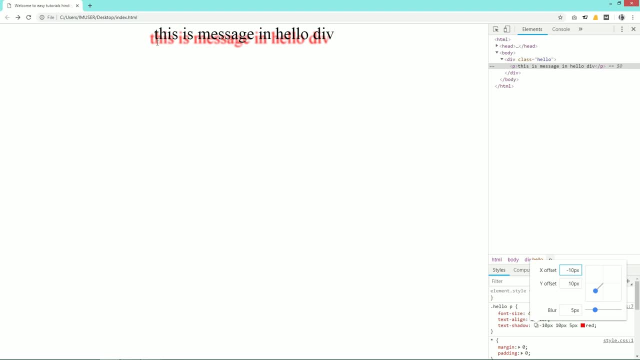 You can change its value according to you, And let me write minus 2 pixel for the Y offset. Let me remove it, And here we will write 2 pixel. So now it is even better than earlier And this is the blur option. 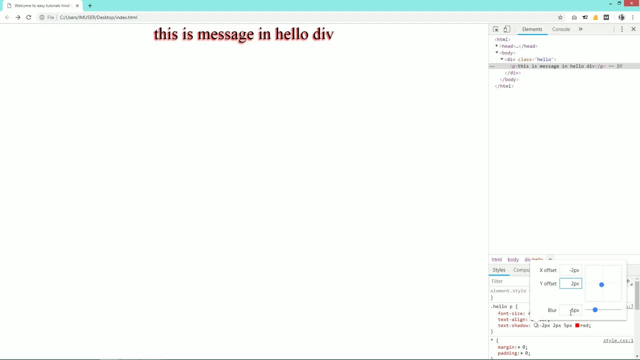 So in this blur option I can increase this one, So you can change the value of this blur. You can adjust this one. I will decrease it to 3.. That's it. So this is how you can get all the three values. 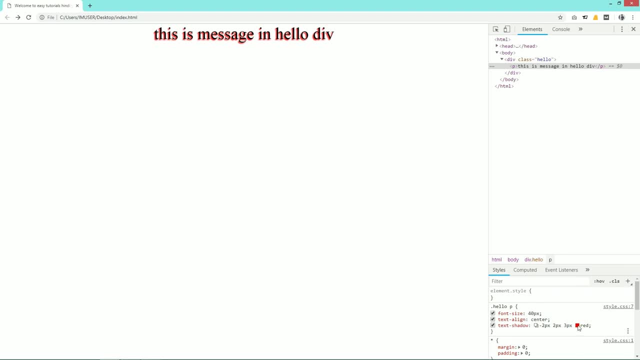 Then click on this color, And on this color you can change the color from this color box. I will change it to light blue. This is how you can add the text shadow. Which one is good for you? Just copy the value and come back in the CSS file and paste it here. 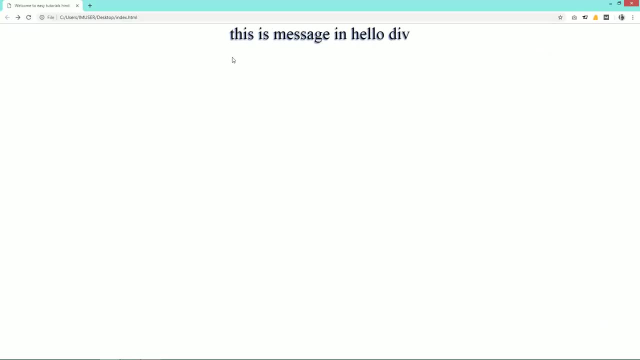 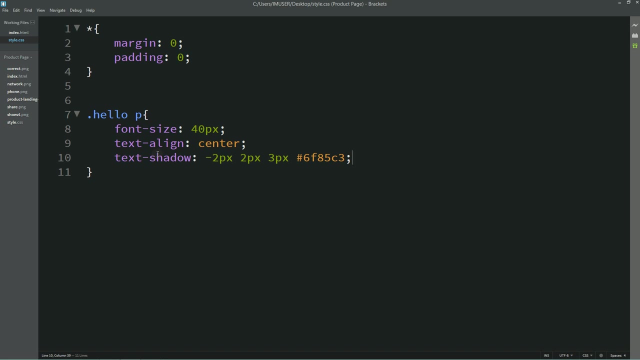 And reload the web page, The same text shadow will be there on your web page. So mostly you will use this type of shadow using the inspect code. So this is how we learned everything about the text decoration and text properties. Now we'll talk about some classes. 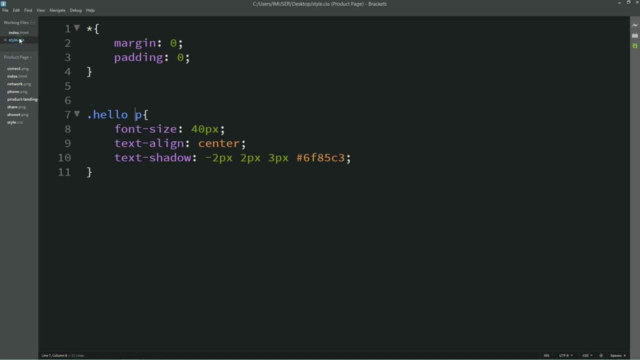 See, as we did here, one class name, then P. So Let's come back and we'll see if we have more divs. So just come back in the HTML file and we have this div here, Class name hero. And let me create one more div. 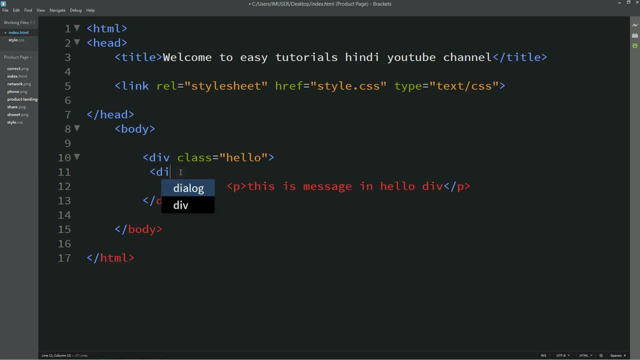 I will add one space and here I'm adding one div And let me write one class name here. The class name is in a hello. You can write any class name And I will close this div here. So suppose we have this type of structure: one div and one another div in the parent div. 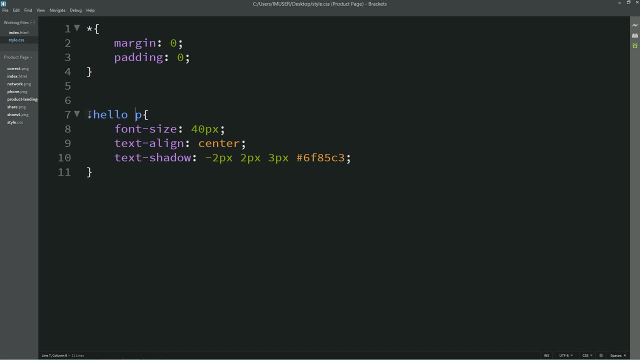 So let's see how we can use this one. We have written the class name of parent div, And after that we can write the second class name, which is inner hello. Then we are writing the P. So this is the class name. 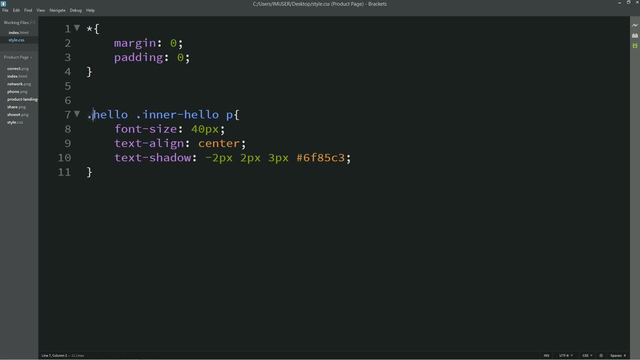 We have written the class name of parent div. This is how you can refer different class name from the parent class to the child class. Apart from that, we have some pseudo class like active, The other one is focus And we have hover. 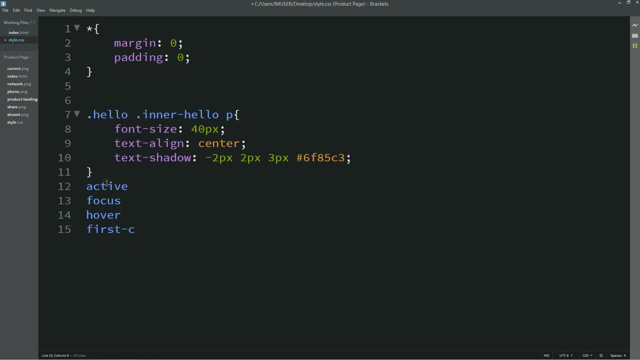 There is a first child and next is last child, And we can also write nth child and value. So these are the different pseudo class. So for the active condition we can add some CSS using this one Suppose one button is already active. 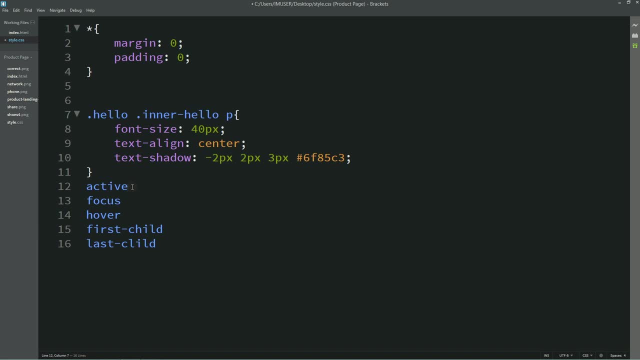 We can change the style. Suppose something is focused. we can change the style Suppose we will take cursor over any element. we can take cursor over any div. We can change the CSS property by hover First and last child. We can change the style. 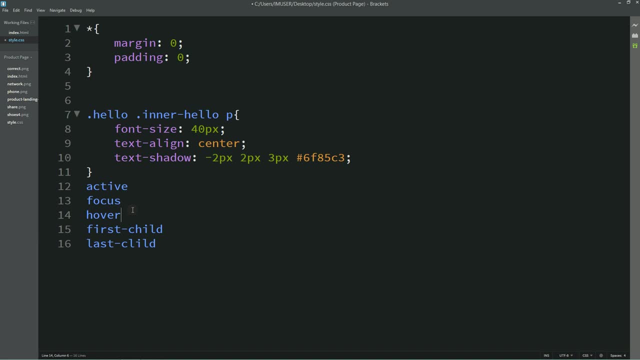 I will tell you like if you have multiple things list, multiple list, and if you want to select the first one or last one, then you can use this first child or last child And if you want to use any other child between those lists, you can use nth child and value. 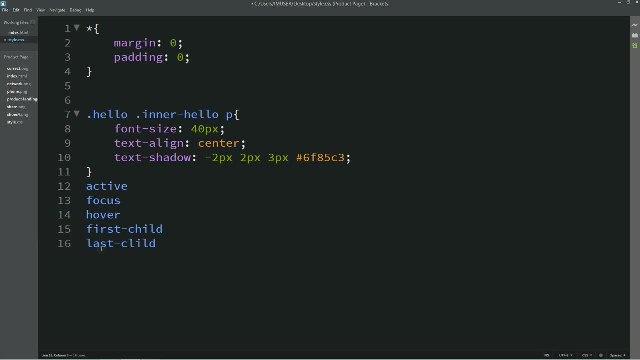 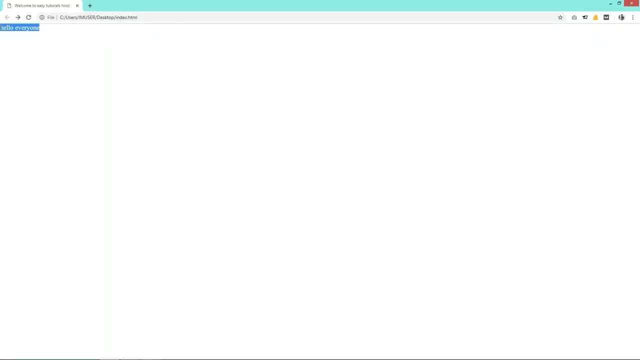 Let me show you one example of hover. So just come back in the HTML file and here I will write one text And the text I am using in the p tag. So the text is: hello everyone. So this is the text on the web page. 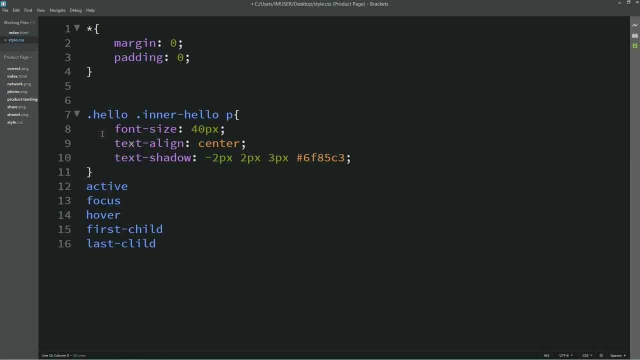 Let's copy this p and come back in the CSS file. Let me remove it. Here. we will write p And after that I'll write this colon And I'll write hover. Let's remove it from here. And when we will hover this p here, we will change the color. 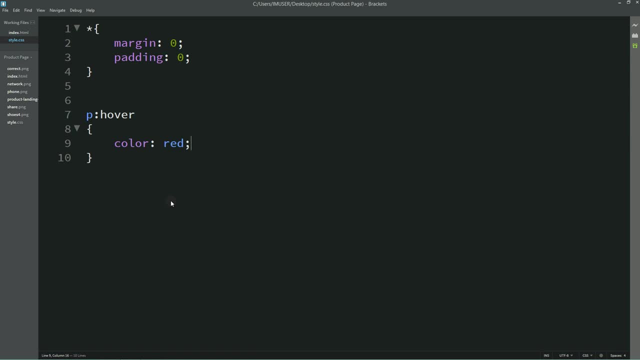 Red. Reload the web page And you can see it is black right now by default. Better I will increase the font size. So I'll write this p again. And here I will write font size: 40 pixel. Then text align center. 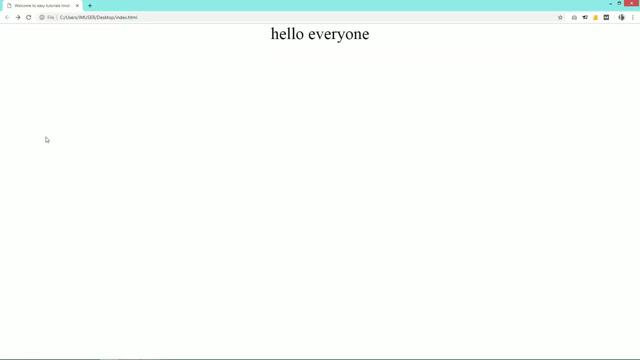 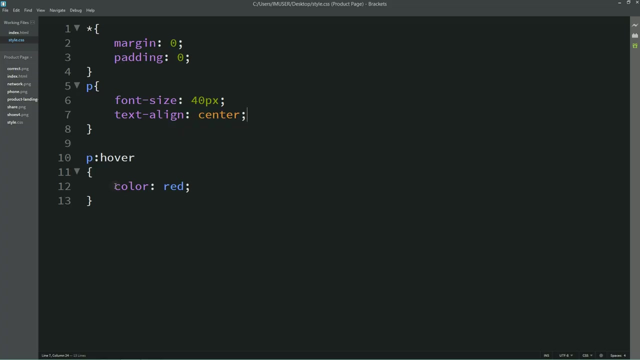 So right now you can see this text is in black color by default, And when I will take cursor over this text it will become red. So you can see. this is how hover works. Apart from this pseudo class, we have some pseudo elements also. 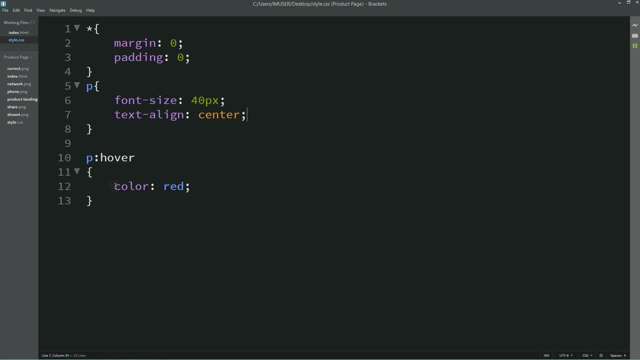 That we will learn after learning the position absolute and relative. Then we will learn about the pseudo elements, like before and after. Next we will learn about position. Let's see where we can use the position relative and absolute. For that we will come back in the HTML file. 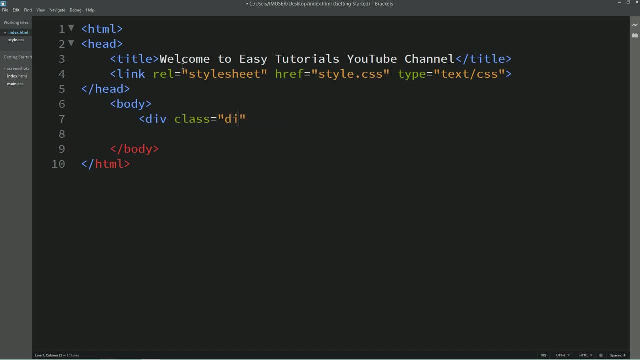 Here we will create one div with the class name demo. I will create one more div And this time I am writing the class name With class name demo inner, And let's add one message in p tag. So I am writing position. 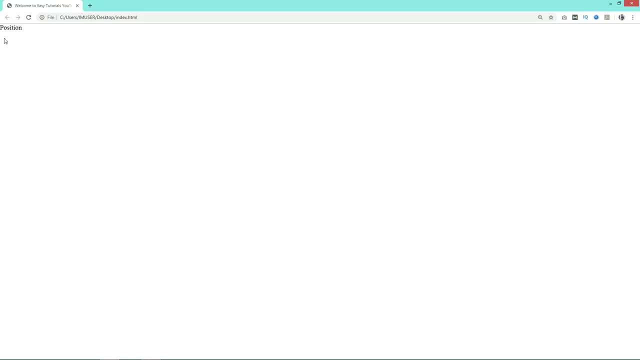 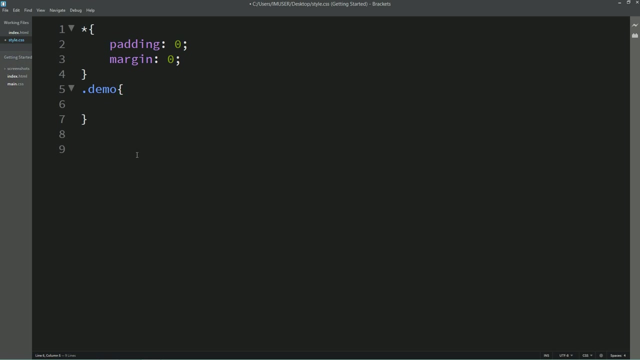 That's it. Let me refresh the web page And you can see this text on this web page. Let's use this class name in this CSS file. Here we will write with dot. For this one, we will set the width And height. 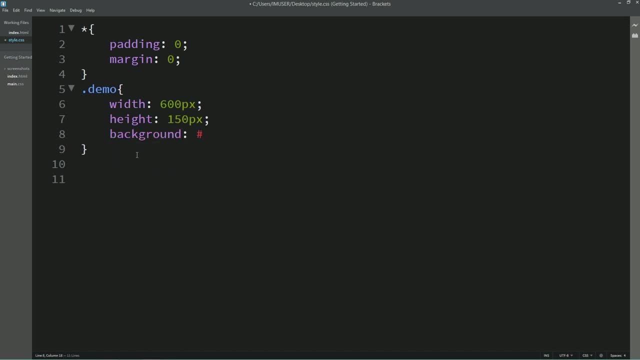 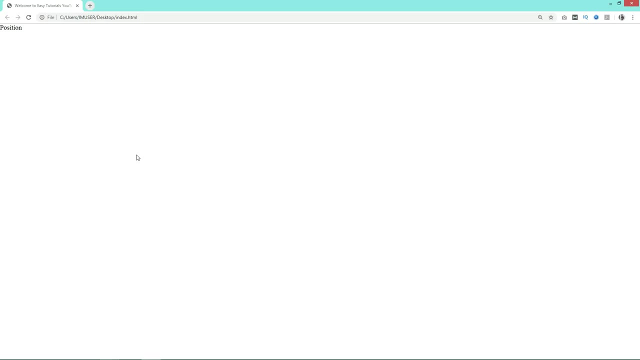 Let's add one background. I am adding this color, Color code, Then I am adding margin: 100px from top and bottom and auto from left and right. Now you can see this div over here with a background color and one text. 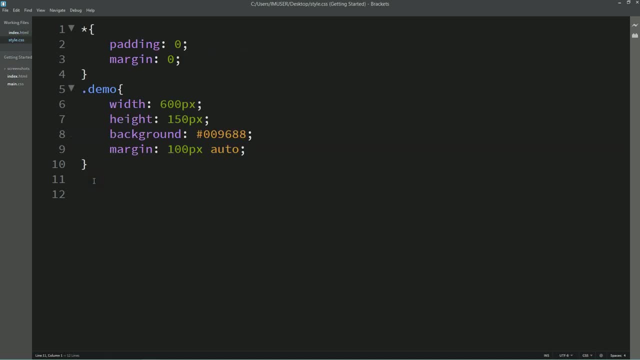 Let's use the second class name, Write it here in the CSS file, And for this one also, we will set the width and height. It will be a small div And here we will write Different background color. So it is red. 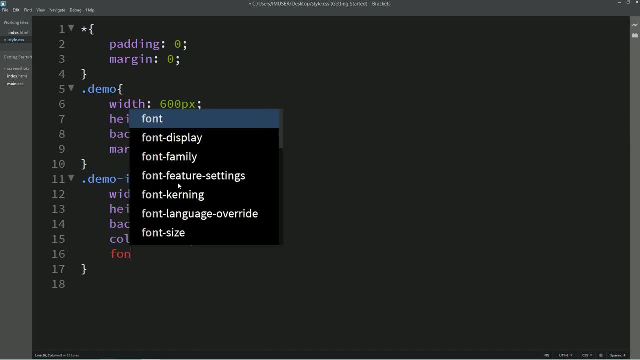 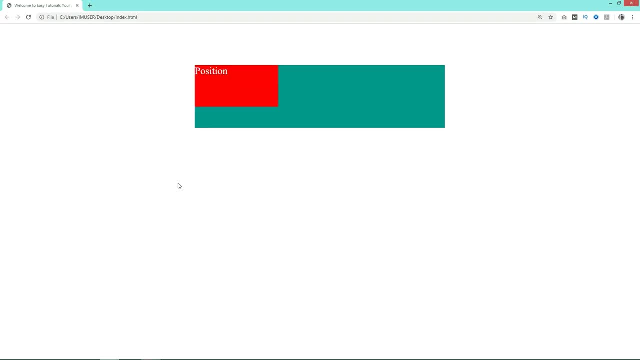 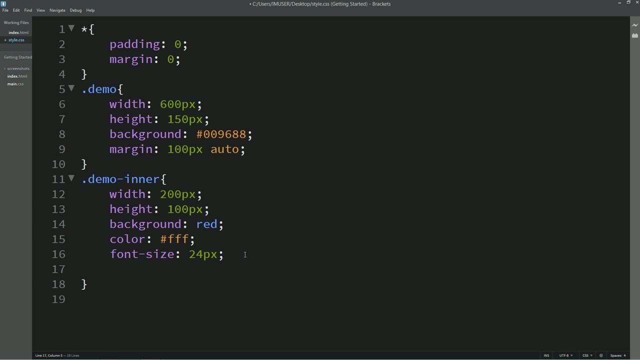 And color will be white So that we can see the text clearly. And let's write the font size So that you can see there is one more div inside the parent div. Now let's see what happens if we add position absolute. When we will set the position, we can use some other things. 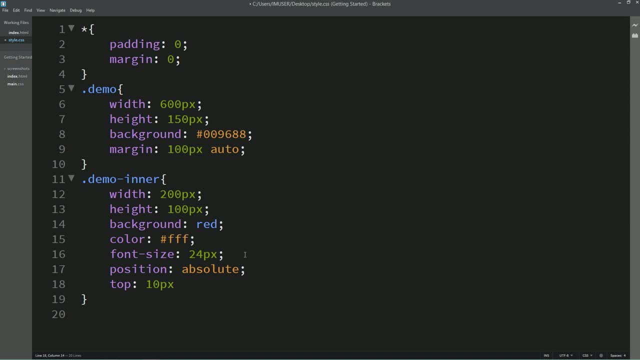 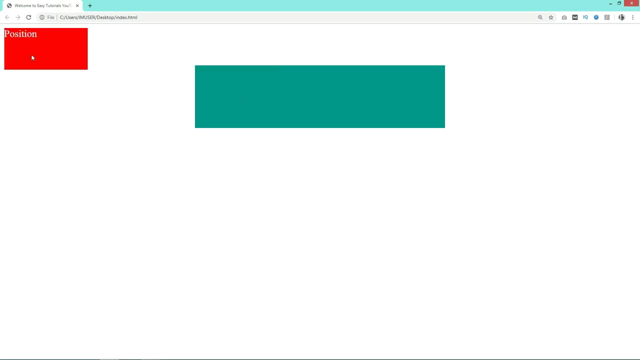 Like Left, bottom or right. So here we will write the top 10px And left 10px. Let's see what happens. After reloading the web page, you can see this small div comes at the top corner, Because right now our small div is in position absolute. 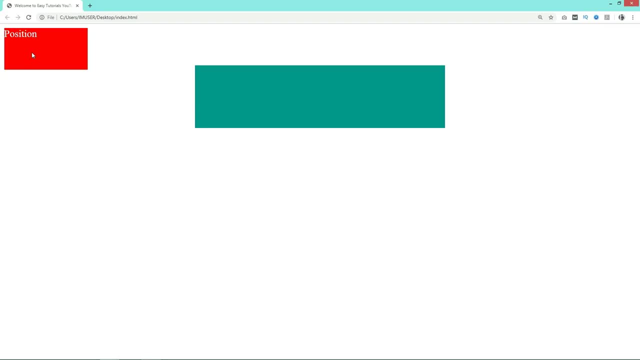 But it is in the absolute position with respect to the entire web page And it is about 10px distance from left side and 10px distance from top. Because we have written top 10px and left 10px, Now we have to set this position absolute in respect to the parent div. 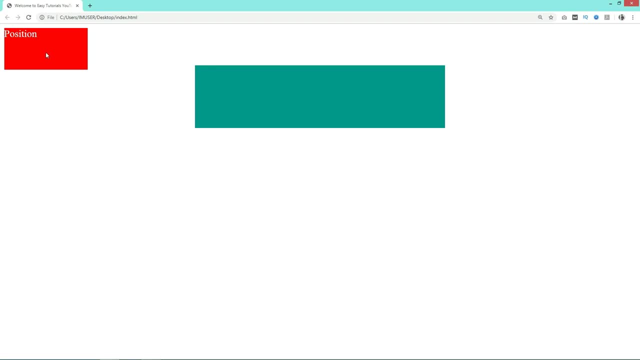 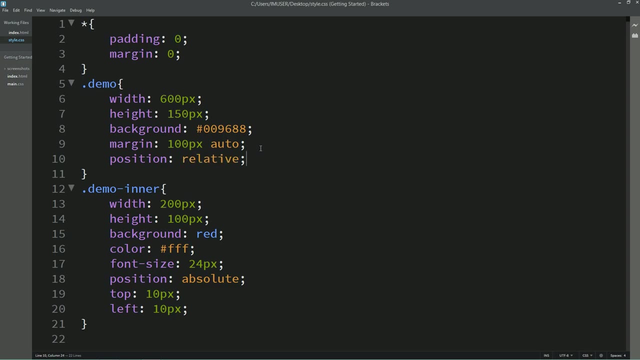 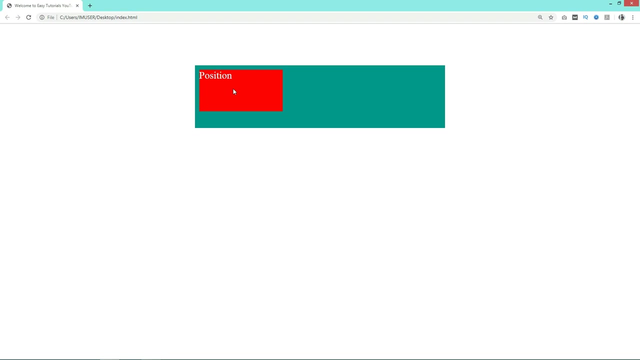 So for that we will come back in this CSS file And in this parent div we will write position relative And now we will refresh the web page again And you can see, now this small div is in position absolute with respect to the parent div. 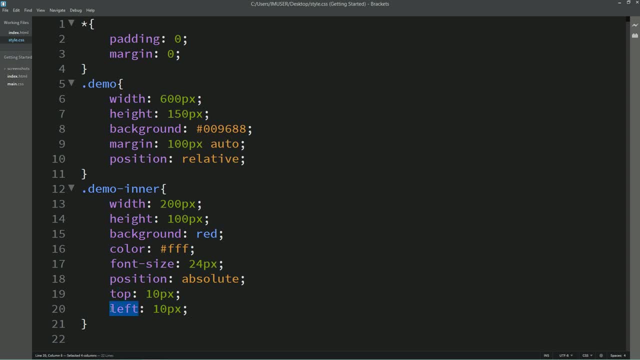 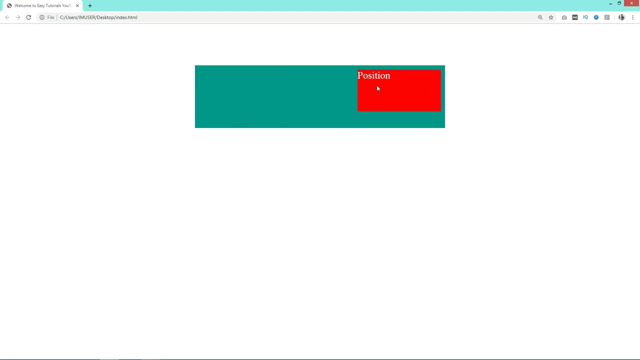 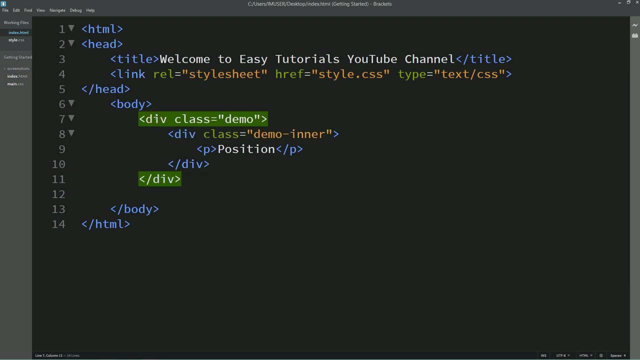 Let me change its position from Left To right. It will be right 10px And reload the web page. Now you can see this one in the right side with respect to the parent div. So this is how position absolute and relative works. 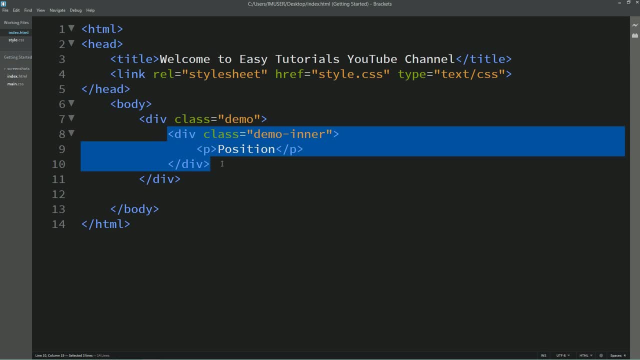 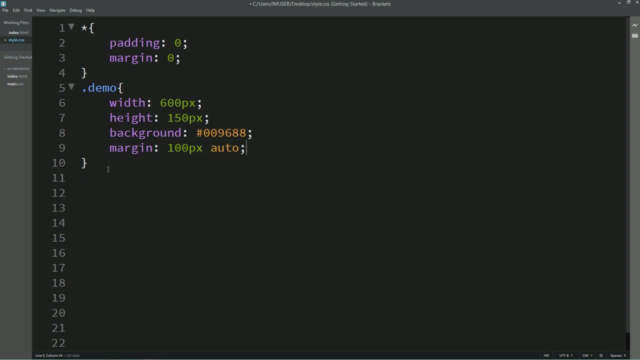 Now let me remove this from HTML file And I will remove it from the CSS also. Next we will learn about the studio elements that I told you. So let me come to the web page. right now You can see only one div, So just come back in the CSS file. 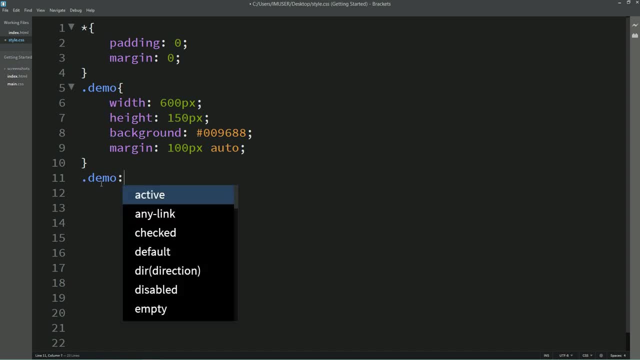 Copy this class name, Write it here And here. we will write double colon And after that I am writing after. It is a pseudo element For this one. let me write content empty. You can write anything in this content field. You can write any message. 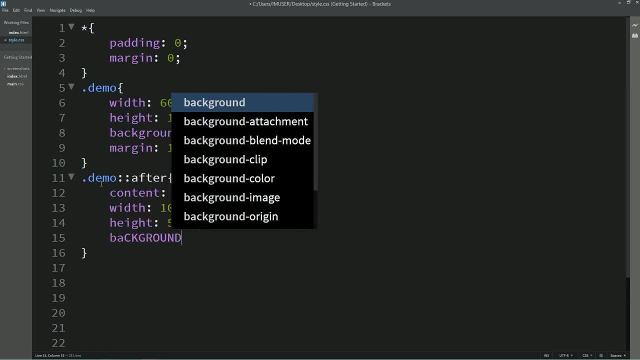 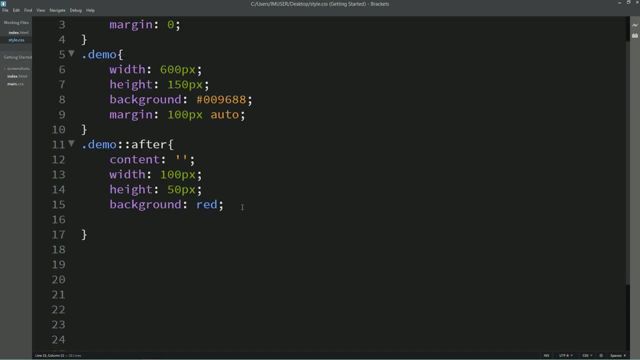 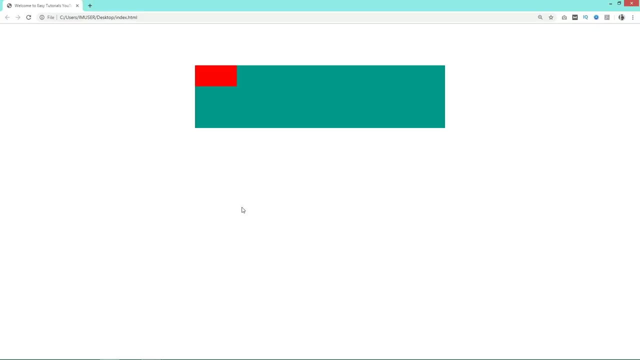 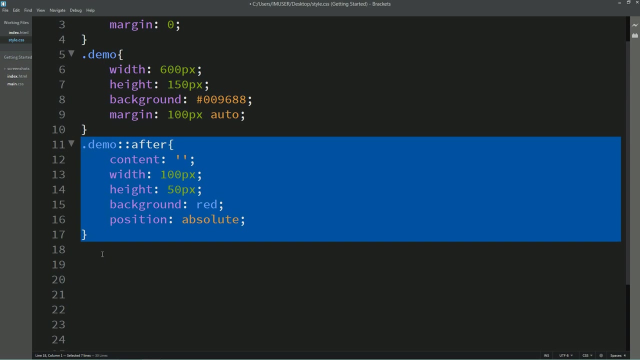 Then I am adding width and height. Ok, Let's set the background red And position absolute. Refresh the web page. You can see a small box over here At the top corner. Now duplicate it And here I will change it to before. 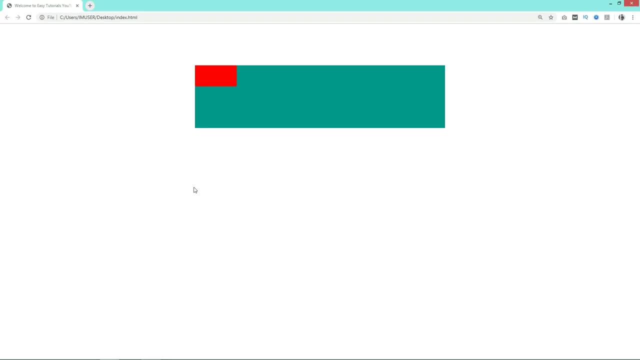 And let's add some message. In the first one I am writing hello. This is hello too. Reload the web page Right now you can see only hello, because the second one is hidden. We had the first one. Let me remove this message. 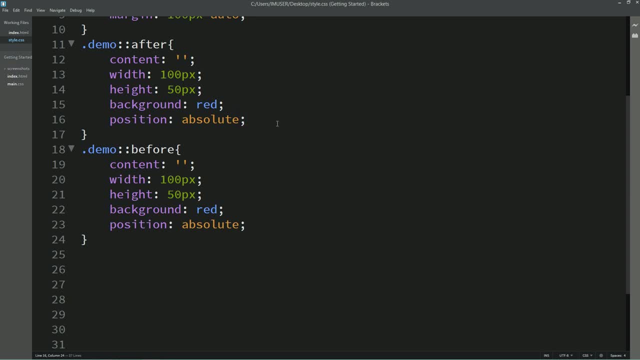 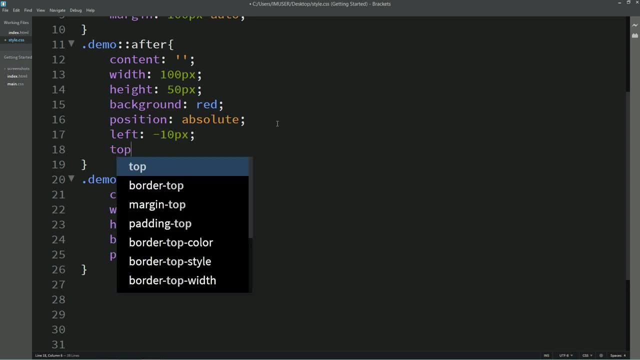 And right now you can see only color. Here I will write left minus 100px And top minus 100px, And we will write this for before also. So here we will change: instead of left it will be right And instead of top it will be bottom. 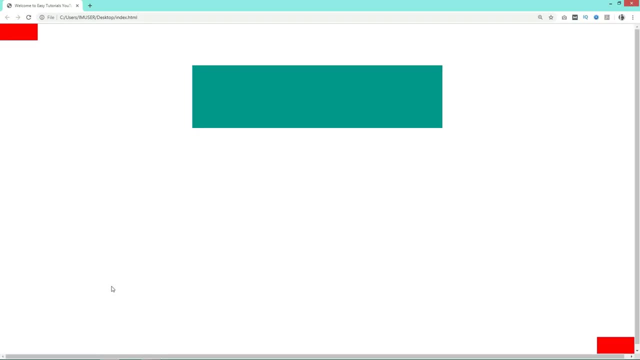 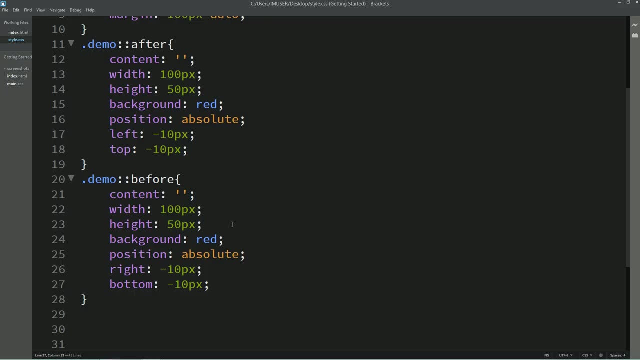 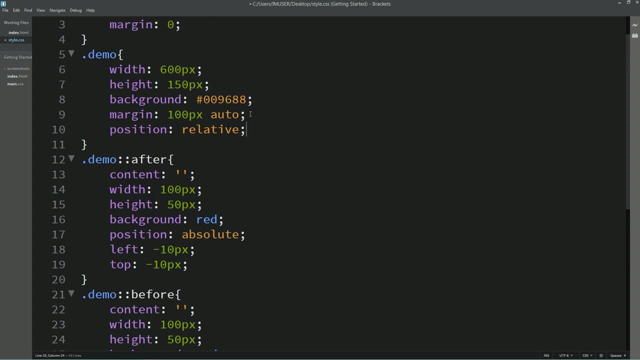 So the position will be different. Right now you can see these both color at the top left corner and bottom right corner, So we have to set its position according to the div. So let's come back In the CSS file, In this class name, I will add position relative. 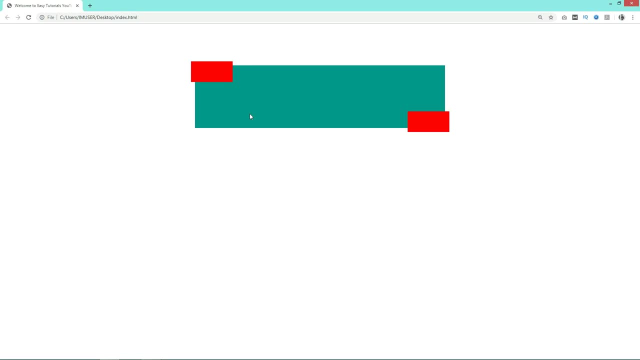 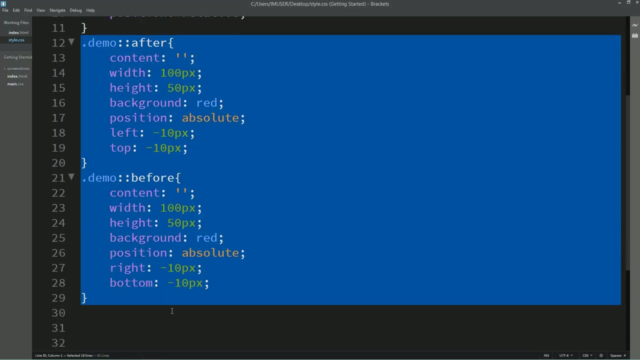 That's it. Reload the web page And you can see Now this small zero elements are fixed at its position with respect to the parent div And it is in the top left corner And the second one is left bottom corner. Again, let me remove this. 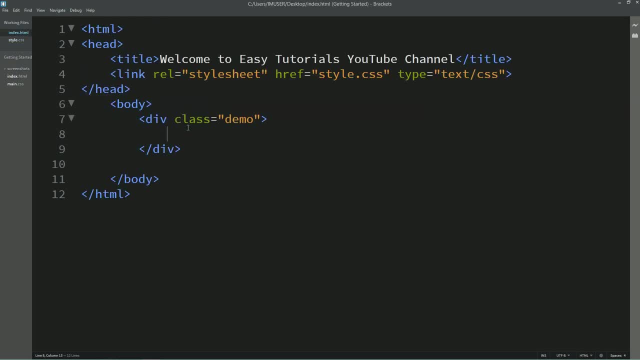 And next we will learn about display flex. We will use display flex to create columns and rows on our web page. So let's come back in the HTML file. Here we will create one more div And let me add one class name. It will be demo inner. 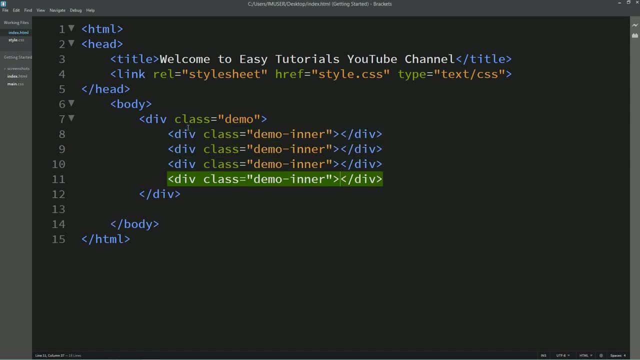 Let's duplicate it Because we need more div here To create different columns. So in the first one I will write 1 in p tag. Let's add it in the other also, It will be 2,, 3 and 4.. 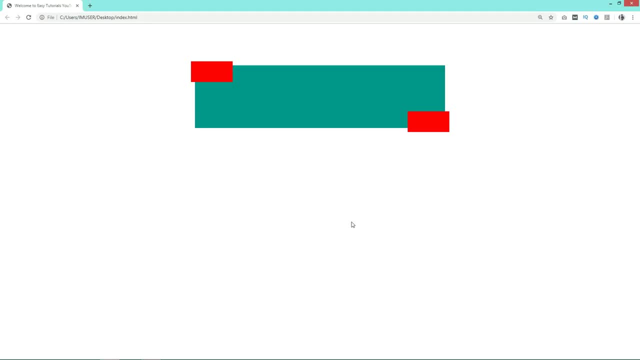 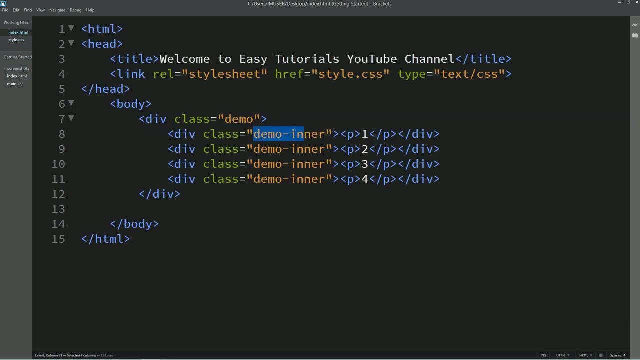 That's it. Save these changes And let's reload the web page. You can see 1,, 2,, 3, 4.. It is coming like this vertically. Now we will copy the class name Demo inner. We will write it here. 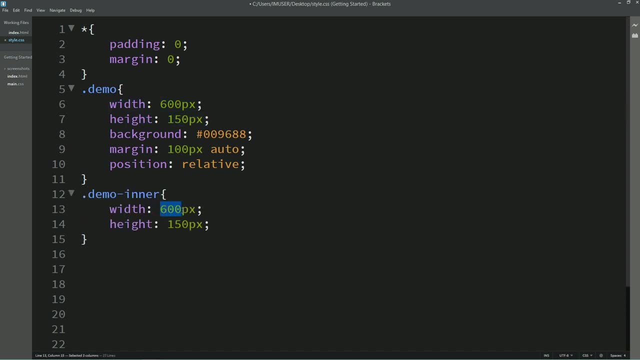 And for this one we will write height and width. It will be a small div of 150 pixel. Let me change it to 600 for the parent div. Now, for this small div, we will add a background color, So it will be red. 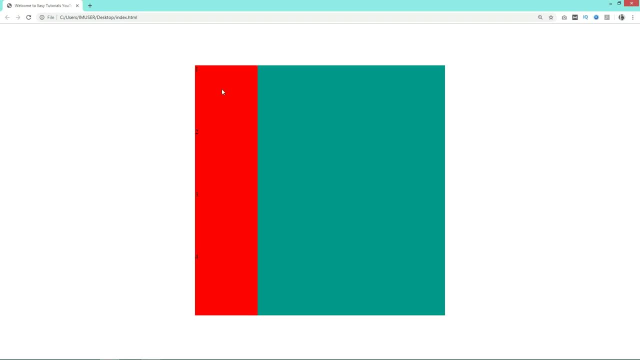 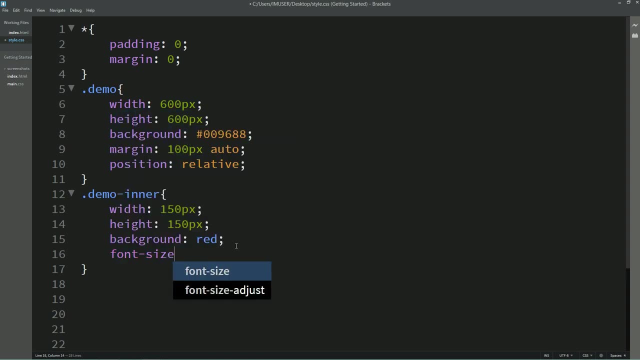 Reload the web page. Now you can see the same background color for all the four small div. So we will change the background color for each div. So let's come back, And First We will change the font size. It will be 24 pixel. 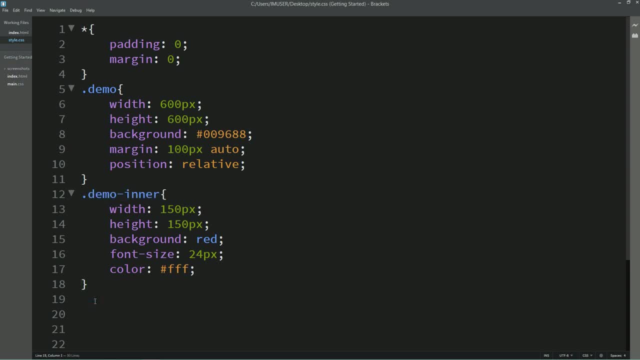 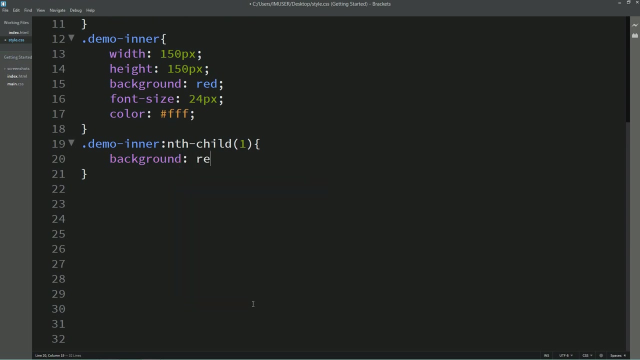 And color white. Let's copy this class name here And here we will write Net, child 1.. So it will select the first div with the class name demo inner. Here I will write the background red And remove it from here. 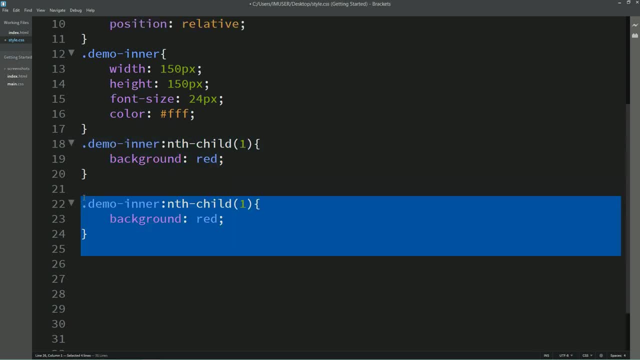 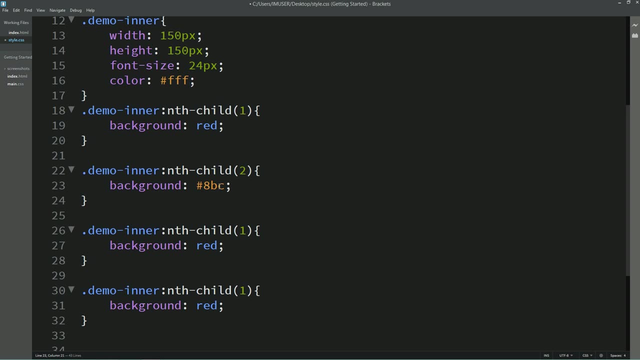 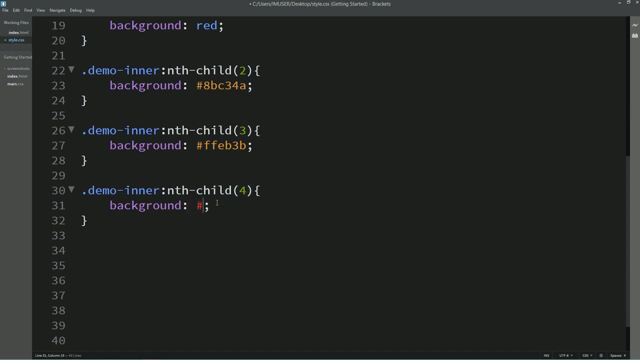 Because we are adding different color for individual. Now duplicate it And change it to 2. And different background. This is for third one, Again different color, And this is 4.. Here also, we will write different color code. Now refresh the web page. 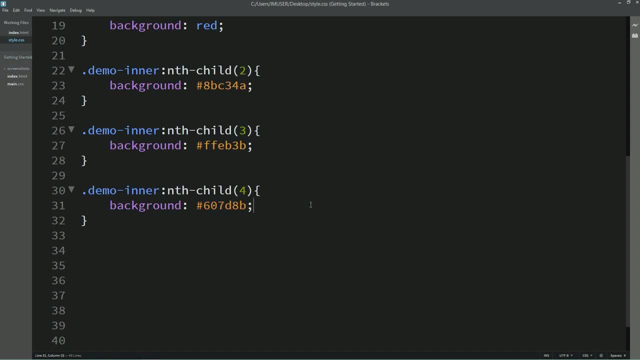 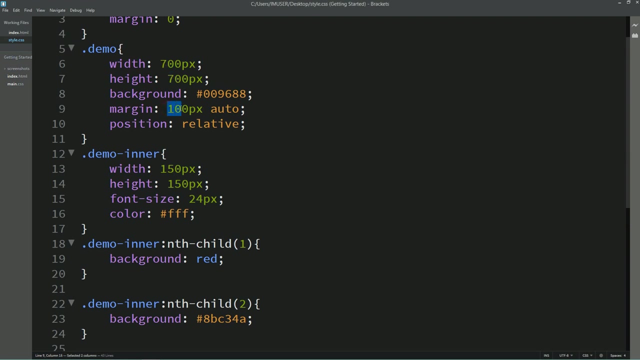 And Let's copy this, And Here you can see different color for each small div. So right now it is coming vertically. First let me increase its width. I will change it to 700.. That's it. And margin: I will reduce 50 pixel. 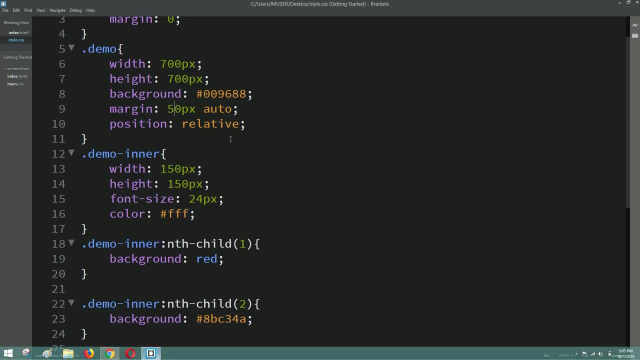 So it is coming like this: We have some extra space at the bottom. We don't need this position here. Let me remove it Now. here we will write display flex. So We have display flex. Let's see what happens. Reload the web page. 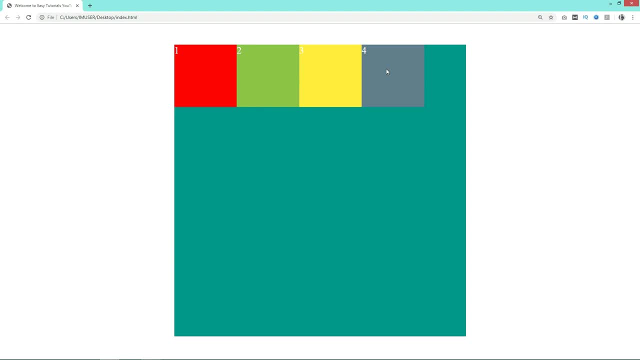 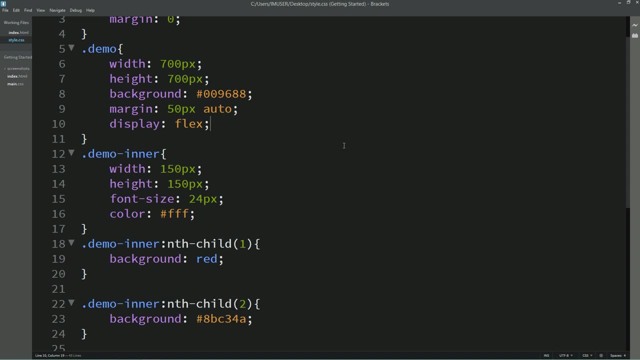 Now you can see everything is coming in one row. We have 4 columns And we have different content, like 1,2,3 and 4. And each columns have different background color. Now you can see what else we can do with the flex. 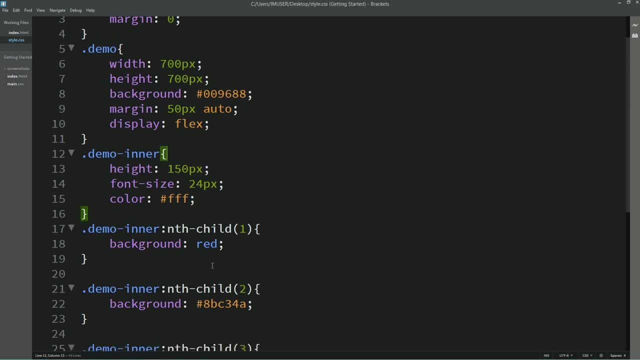 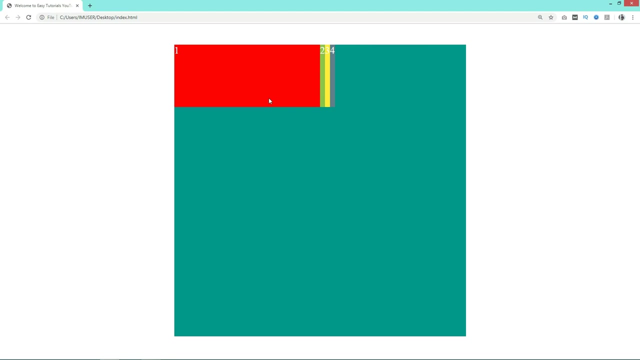 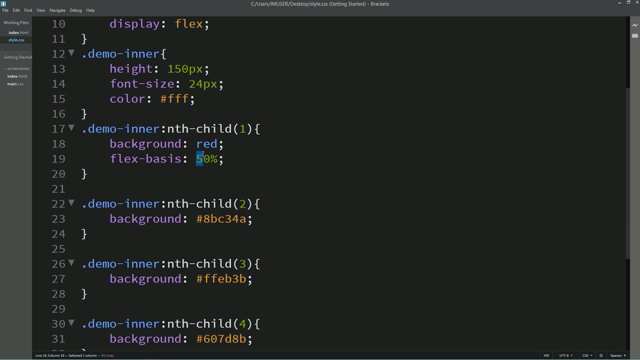 So instead of width here we can add different thing, like we will add flex basis, It will be 50%. Now Let's see reload the web page and you can see we have added flex bases in only first div and the other three divs have no fixed width or any flex bases. let's come back. 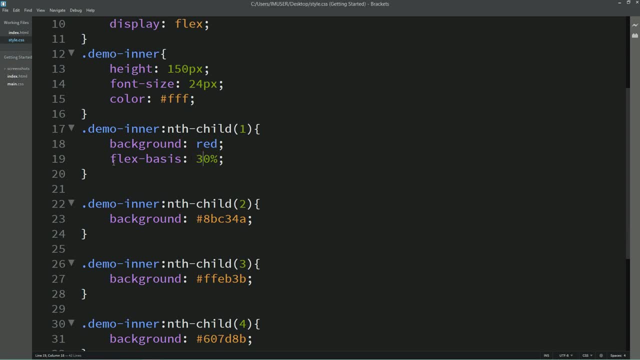 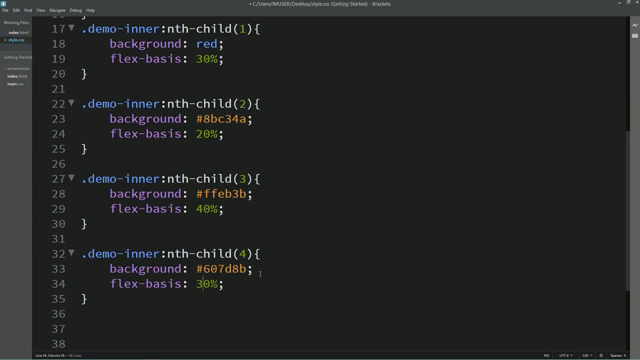 and I will reduce it. I will make it 30%. just copy and paste it in the second one, let's say 20% for this one. paste it in the third one, it will be 40%. and now for the fourth one, it will be 10%. let's reload the web page and you. 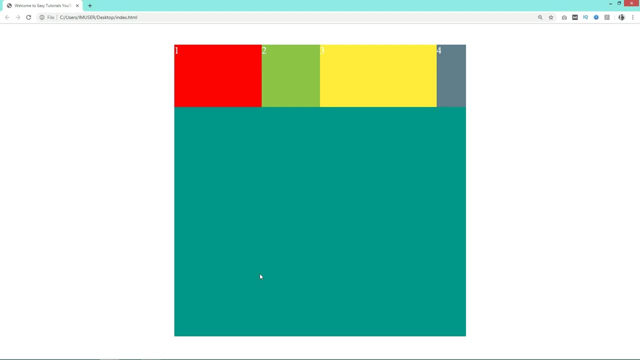 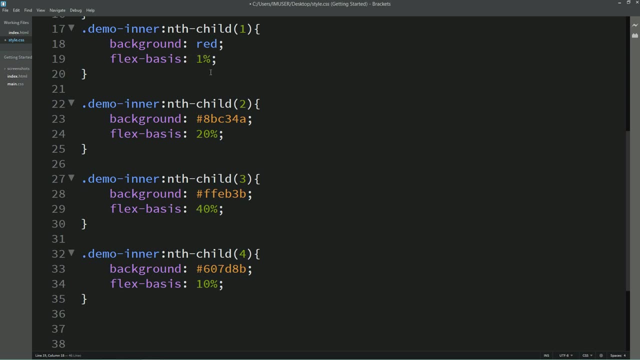 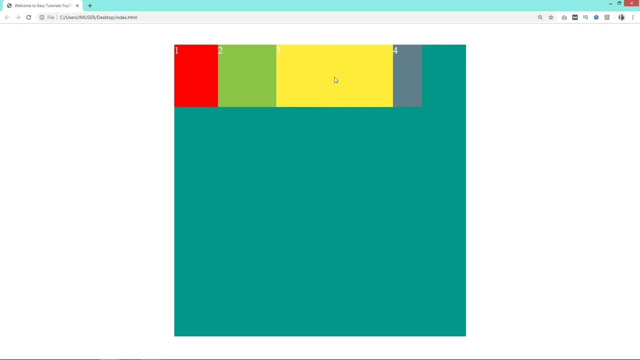 can see different width for each columns because we are adding different flex bases. let me change it: 15%, so it is less than 100%, so we have some extra space at the end. You can see we have this extra space that we want to. 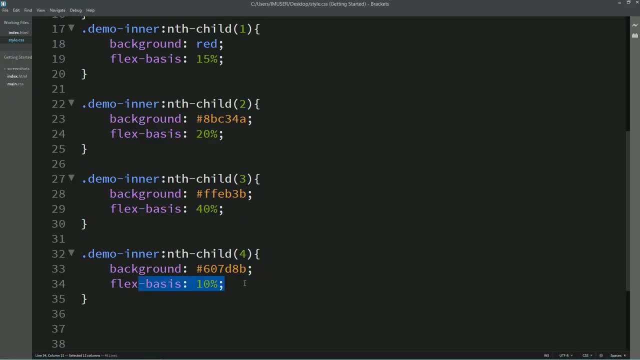 cover. so in the last one even you can do this in any column. so So let me do it. in the last column, I will write flex1.. So what happens? if I will write flex1 in any column, it will occupy all the space available. 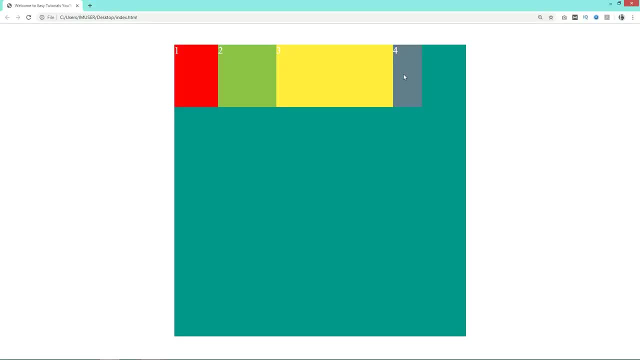 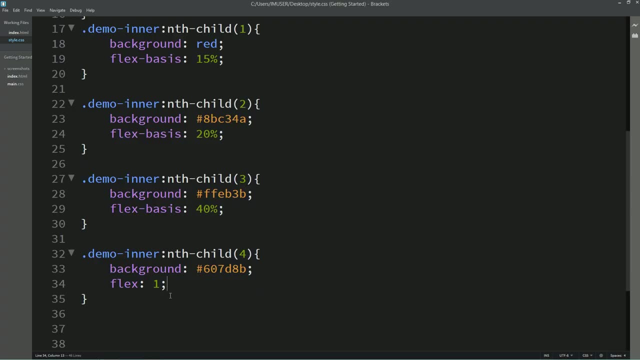 in the row. So let's see the web page again And you can see the last one is covering all the empty space, So it is not fixed. you can use this flex1 in any column. Now I will remove all the flex spaces from here. 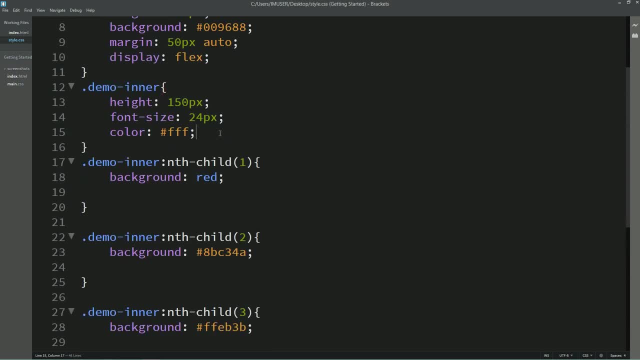 In this demo inner I will write flexbases 15%, So this 15% will be applicable for all 4 columns. Reload the web page and you can see equal width for all 4 columns and we have some space at the end. 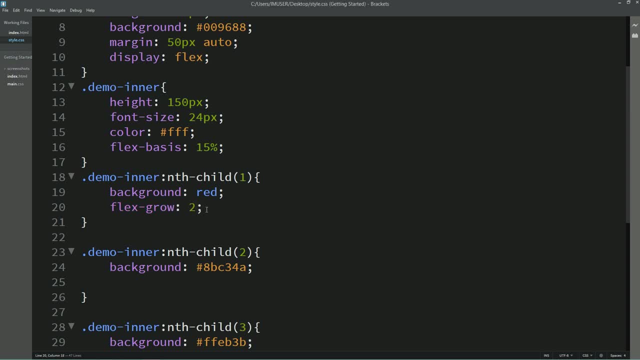 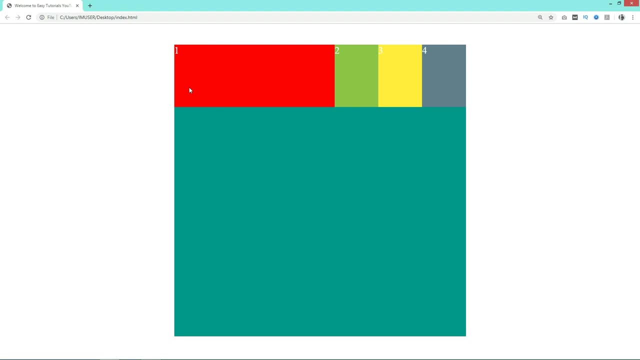 Next, in the first column, I will write flexgrow 2.. Now refresh the web page and you can see the first column is bigger than other one And it is using flex, Using the entire space available in the row. Now let's come back in the CSS file. 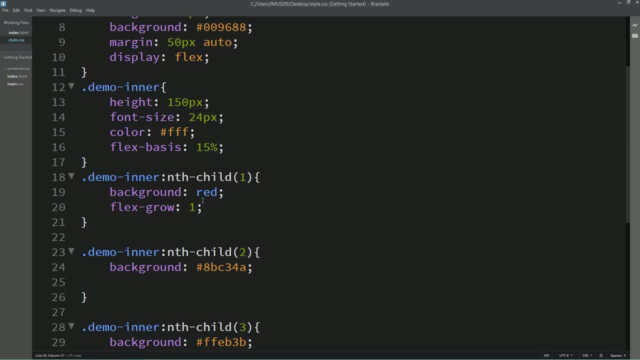 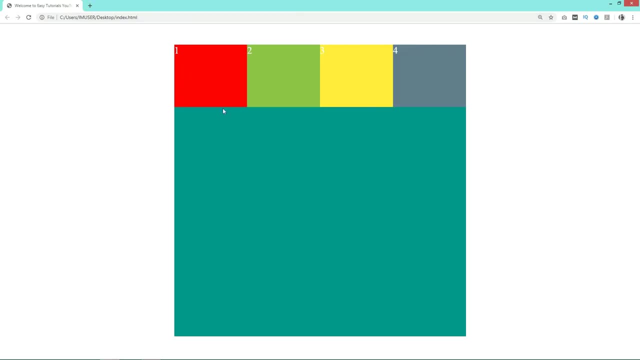 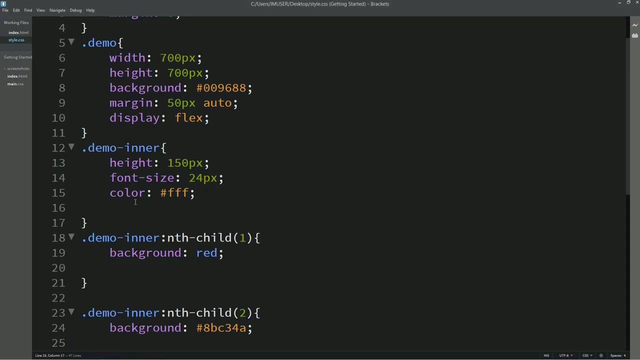 If I will use flexgrow 1 also, it will be same, And if we will set the flexbases 25%, it will occupy all the space and all blocks will have same width. Let me remove this flexbases and now it is looking like this: 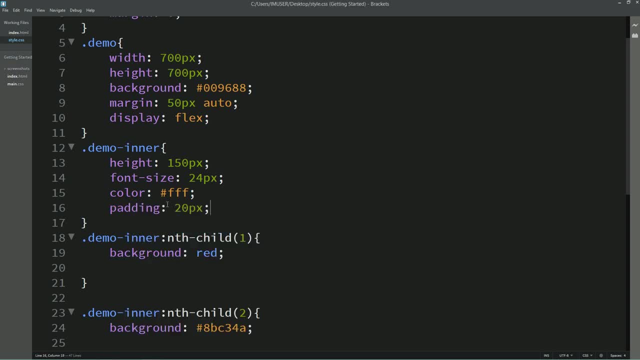 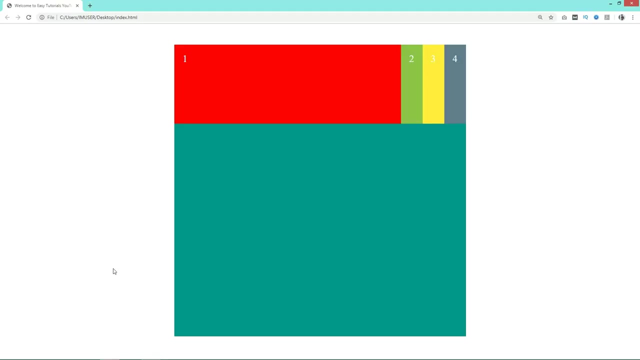 So let's come back, and here I will add padding to add some space: 20px. So right now it is looking like this: All blocks are equal. Next, in the first one, I will write flexgrow 2.. So you can see the first one is big compared to the other. 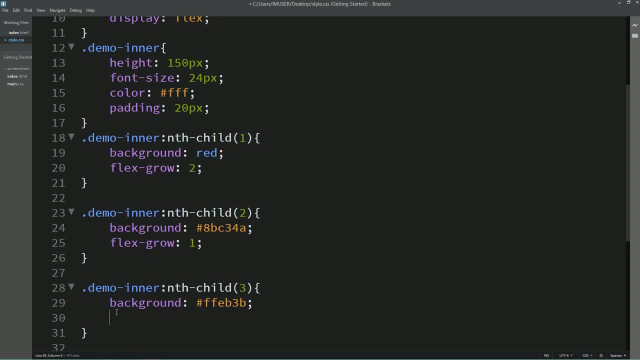 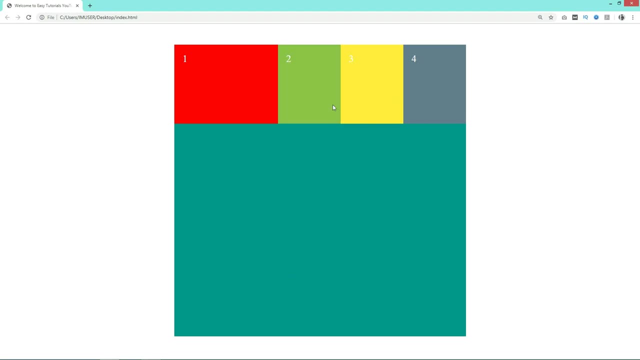 Let's copy it and add it into the second one. Here I will write flexgrow 1.. In the third one, also flexgrow 1 and the last one, also flexgrow 1.. Now refresh the webpage and you can see 2, 3 and 4th block are equal and the first column 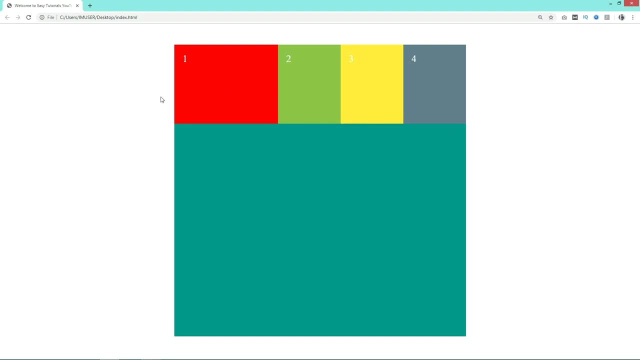 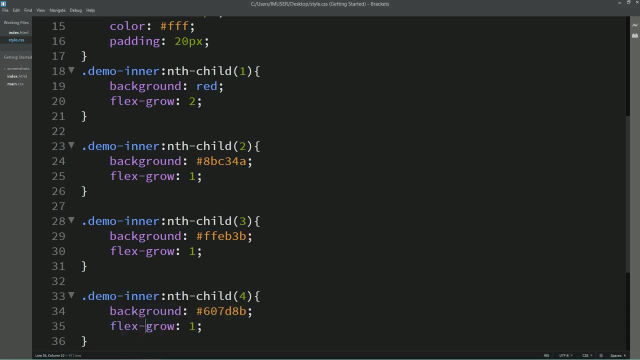 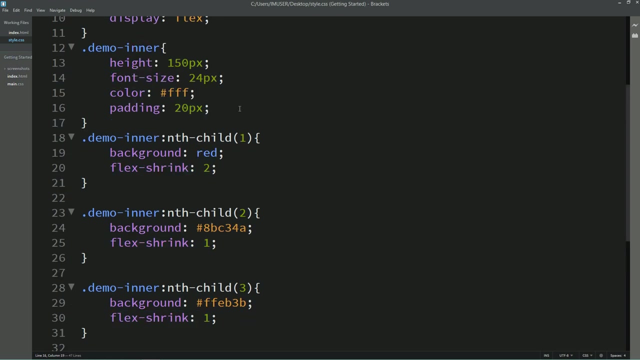 is bigger than other. Next, I will change this flexgrow to the flex shrink. Let me select all of it And here I will write flex shrink. So first one is flex shrink 2, then 1,, 1 and 1.. 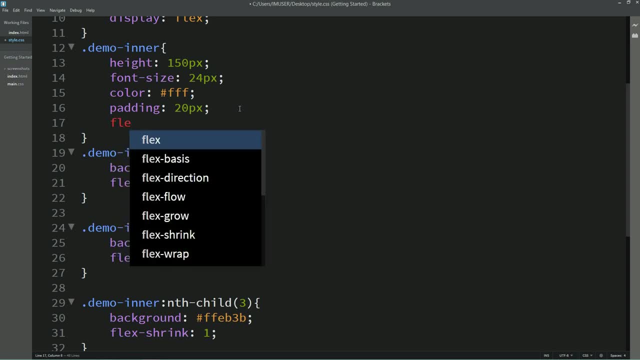 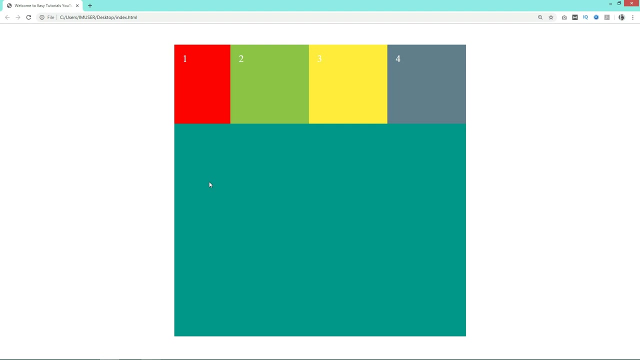 And here we will set the flexbases: 25%. It will be applicable for all the column because we are writing it into the class name, which is common class name. Let me increase it. flex shrink: 3.. Reload the webpage. Let me increase it to 4.. 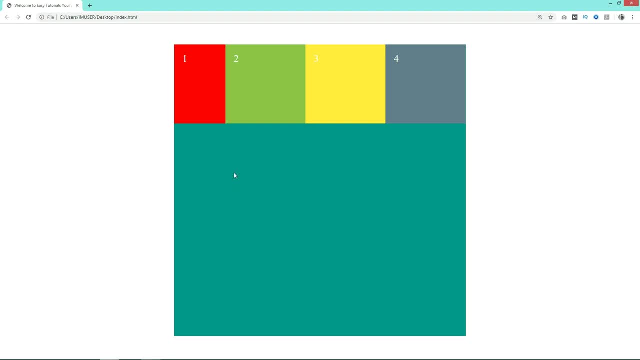 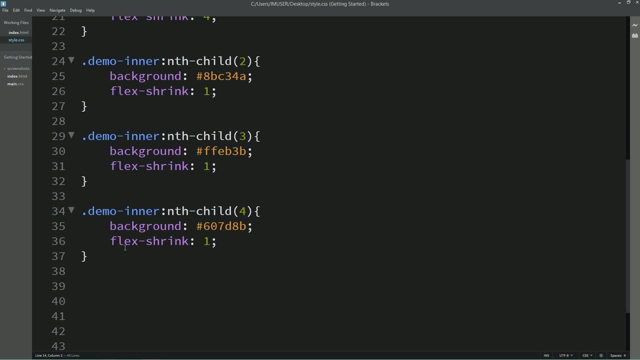 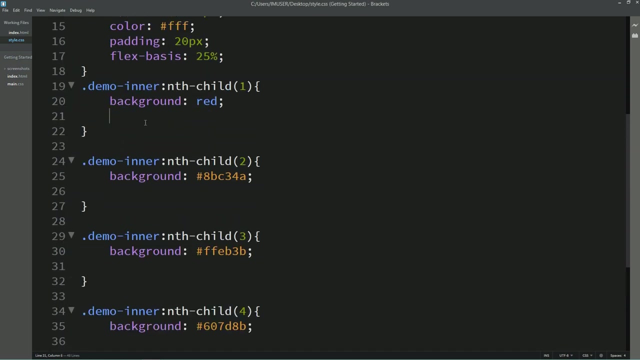 And now you can see: second, third and fourth column have equal width and the first column have a small width. Compare to the first one And compare to the other. Now let's see what else we can do with the flex. So let me remove it. 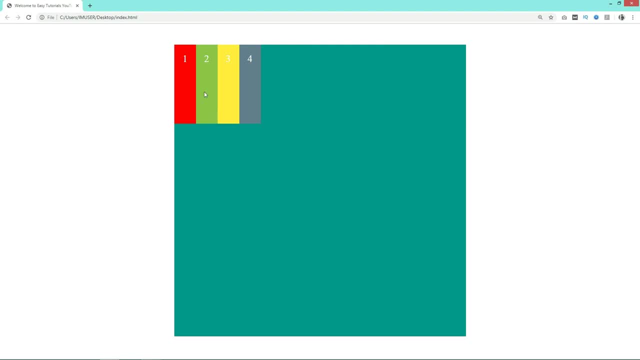 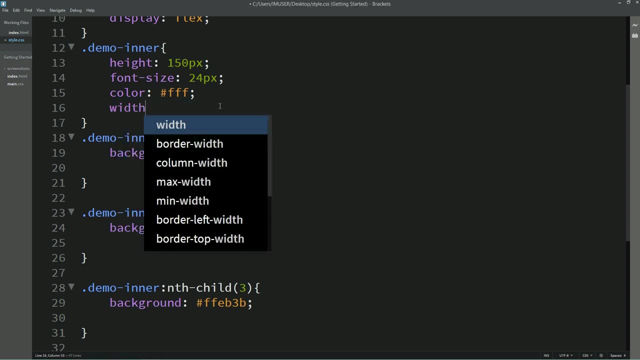 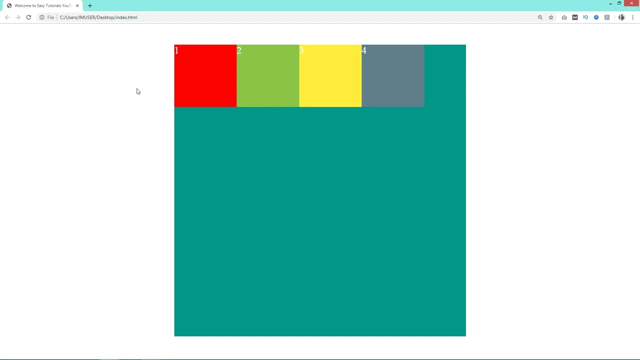 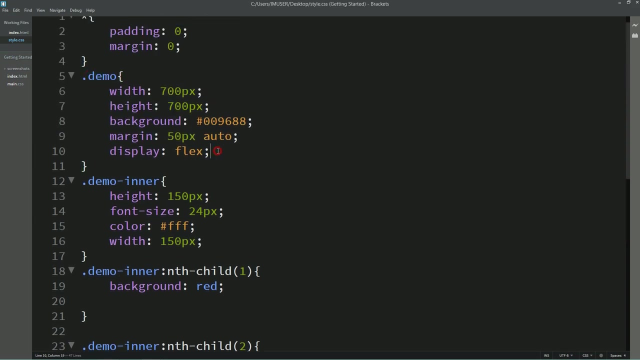 It is like this. I will remove the padding also And here we will write width 150px. So right now it is looking like this: All blocks are equal, Suppose we want to align it vertically center. So for that we will come back here in the parent div. 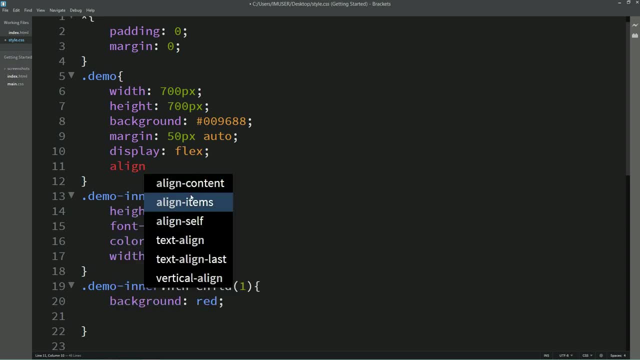 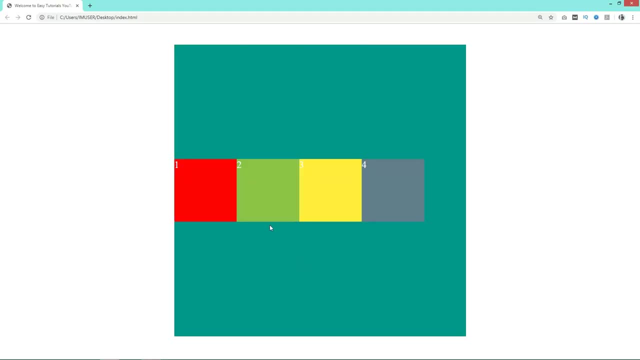 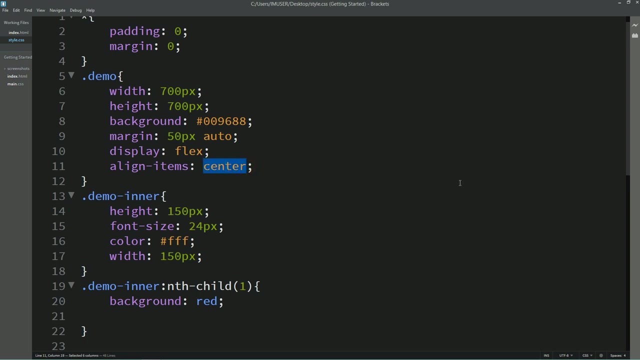 In this parent div where we have written display flex. After that I will write align items center. After adding this, refresh the webpage and you can see this content is vertically centered. If I want to shift it on top, That was already by default. 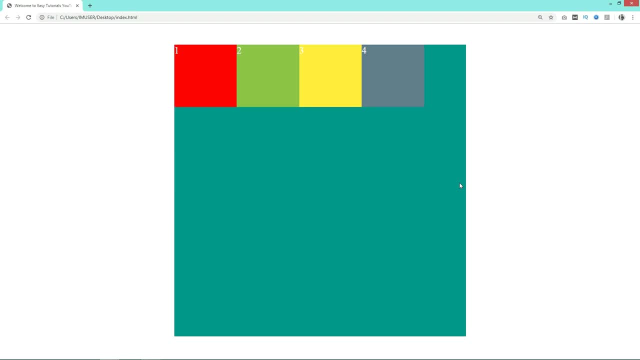 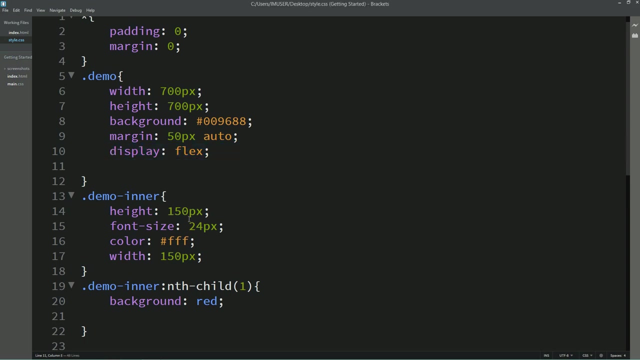 So for that we need to write flex start. So it is on the top, And if you want this at the bottom, then we will write flex end And you can see this content at the bottom Now. let me remove it Now. if you want to align the content horizontally, then you can write: justify content. 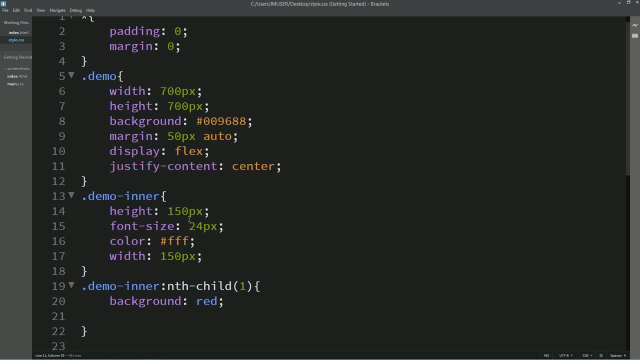 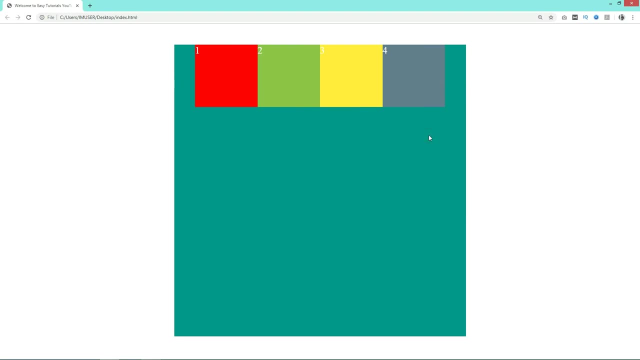 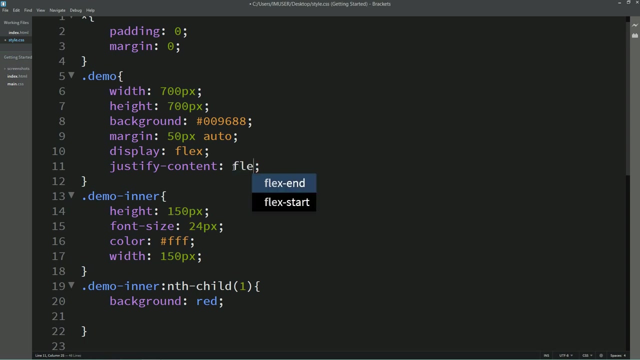 And in this justify content. let me write center, And right now you can see this content is center from horizontal, So it is on the top And there is some space from left and right side. Instead of this center, let me write flex: start. 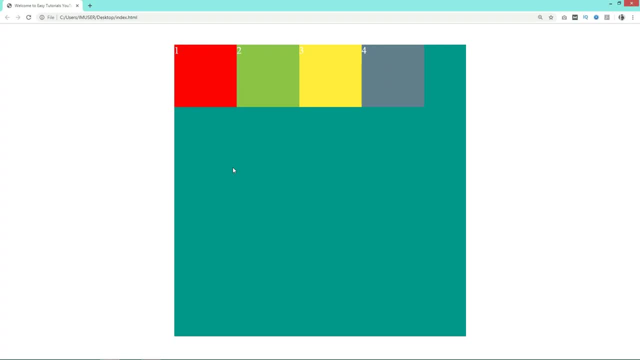 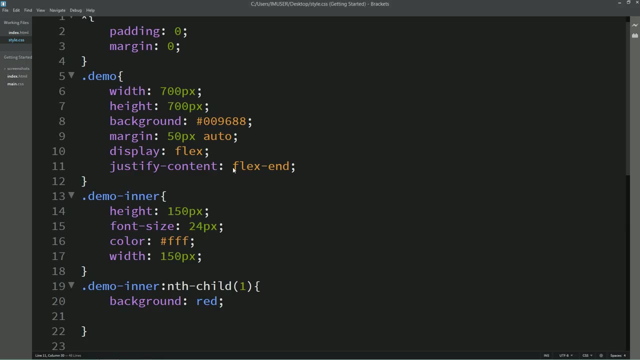 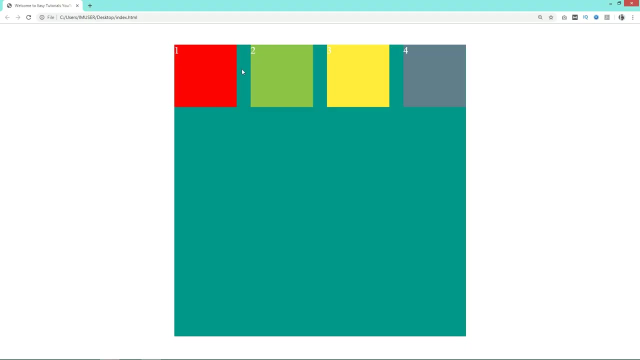 So it is the default one. It will start from the left side And if I will write flex end, it will start from the right side. Let me remove it and here I will write a space between When we will write justify content. a space between you can see, equal space between all. 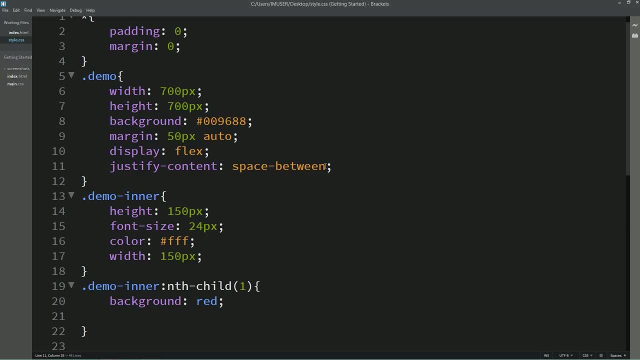 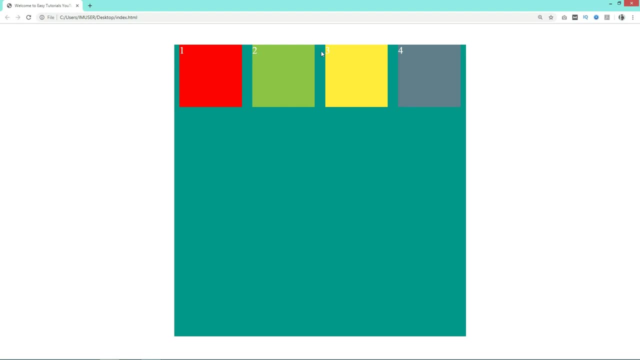 the columns. Now we have one more option here. I will write a space around. So when we are using a space around, so the equal space will be divided between the column and at the end of these columns also, So you can see some space at the beginning also at the end also. 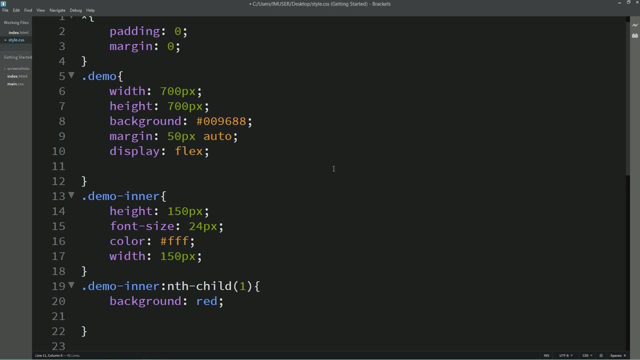 Now you know how to align columns vertically and horizontally. Next I will write flex direction. By default, the flex direction is row. Let me write it here, row and reload the web page. you can see it is showing like this by default And if I will change it to column and refresh the web page. now you can see all the divs. 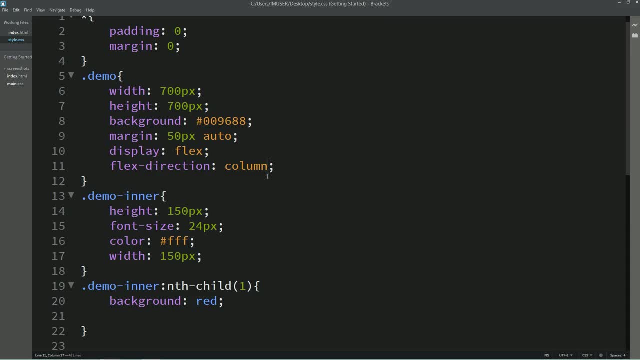 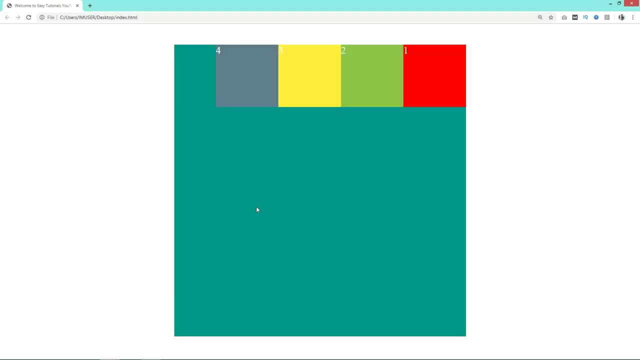 are coming vertically as it is in column. Now, here we can write row reverse. reload the web page and you can see the fourth is coming here. then four, three, two and one. It is in reverse order. Similarly we can do it for the column reverse. 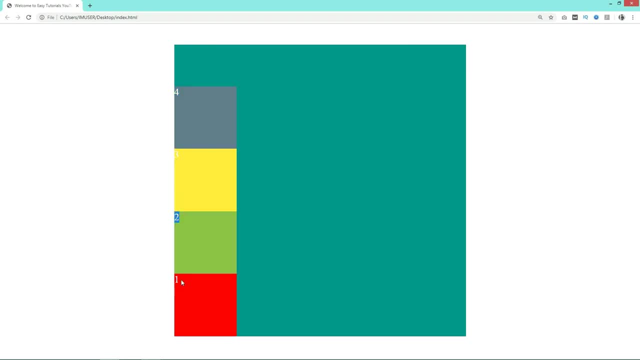 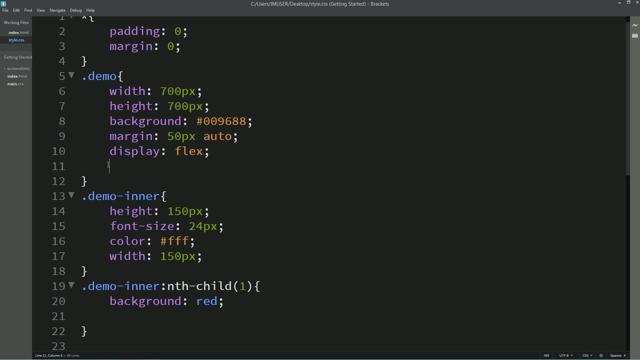 And now the all divs will come in single column and reverse order: four, three, two and one. So let me remove it and we will learn other thing in flex. So let's come back in the HTML file and we will duplicate it, because we need even more. 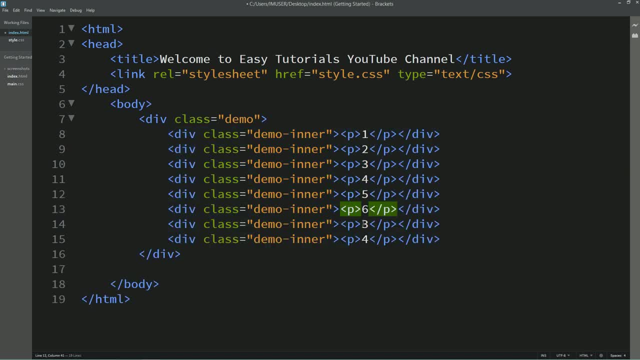 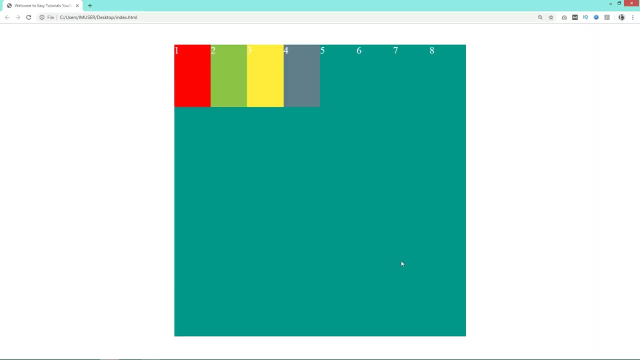 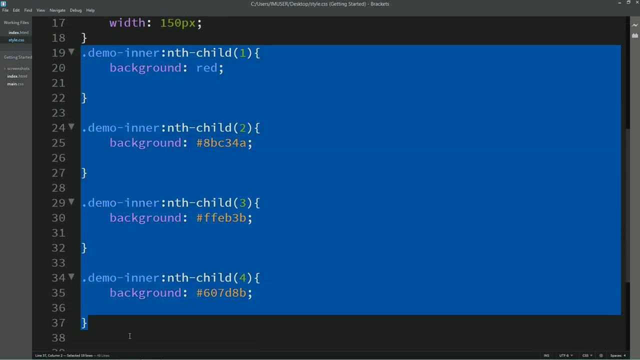 columns here. So total, we have eight small div. Reload the web page and you can see color for only four div. I will add colors in other also. Let's duplicate it in the CSS file. I will increase the order five, six, seven and eight. 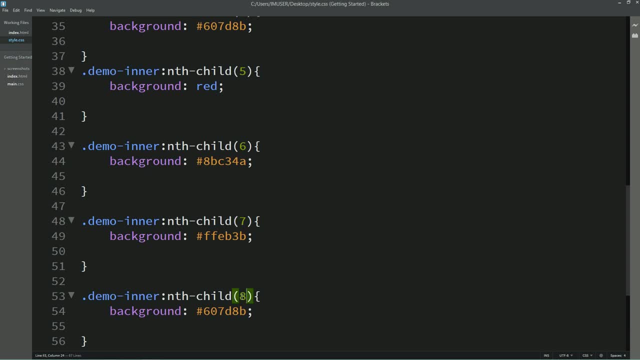 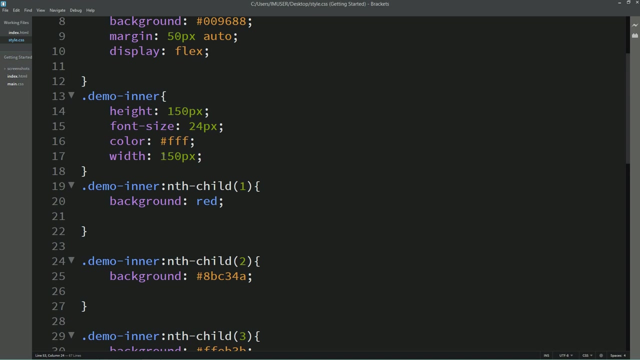 So now we have color in all the small div. Right now you can see we have the width set here, 150 pixel, but it is not showing on web page Because All the small divs Are coming in the same horizontal row. That's why there is no such a space to adjust the width of 150 pixel. 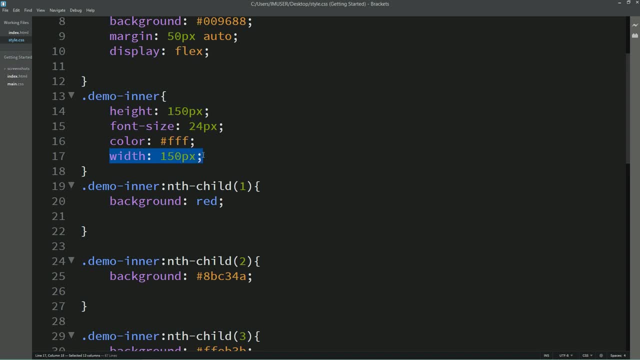 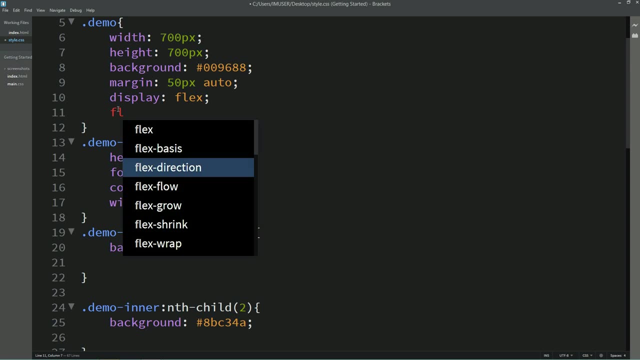 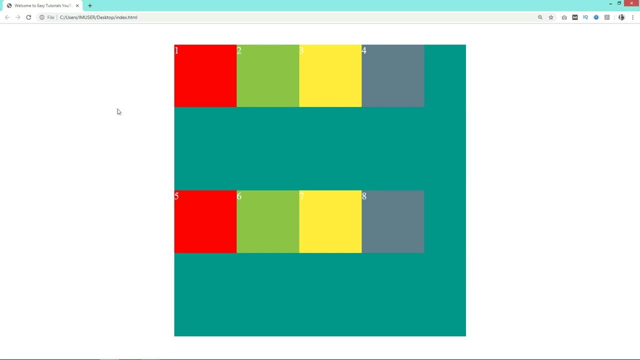 That's why all the small divs are compressed. For that we have one option: We will come back in the parent class name And here we will write flex wrap And it will be wrap. Reload the web page and now you can see all the small div have 150 pixel of width and 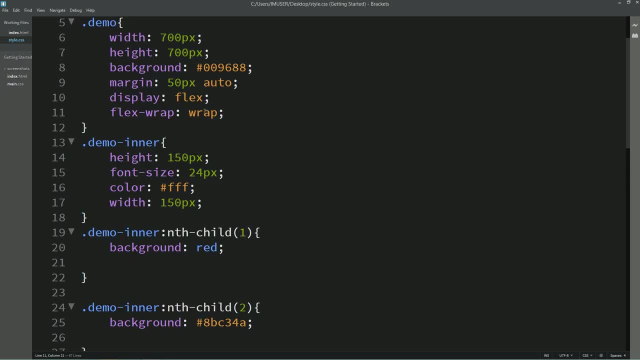 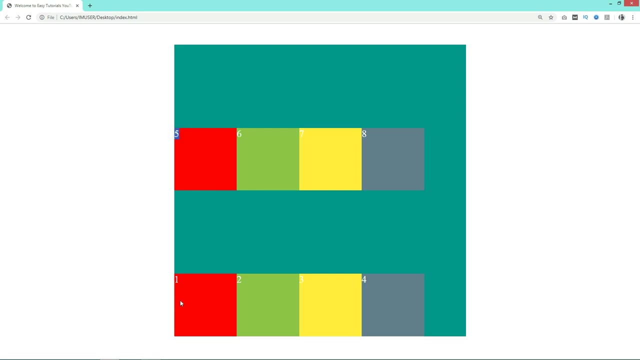 it is coming in two lines. Next, we can add one more thing here: instead of this wrap we will write wrap reverse. So everything will be same, but the order will be different. eight, seven, six, five And four, three, two, one, like this, That's it. 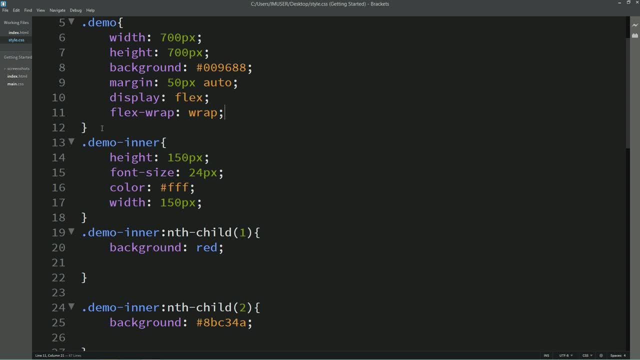 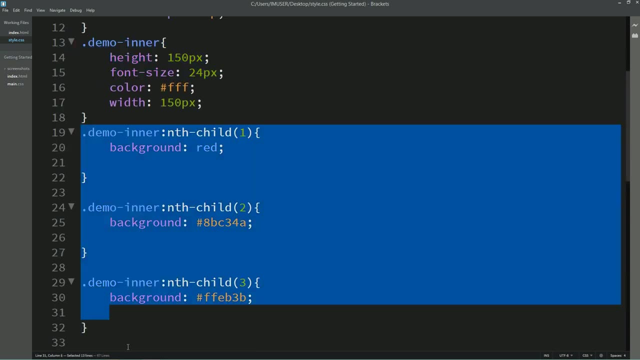 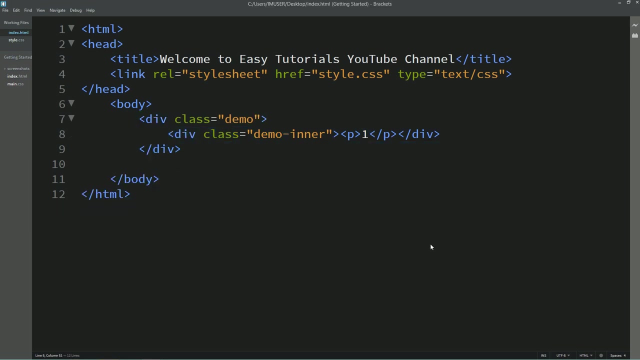 Let it be wrap itself. So this is all I wanted to teach you about the display flex. Now I will remove it. Let it be Wrap itself, And I will remove it from the html file also. we will need only one small div. 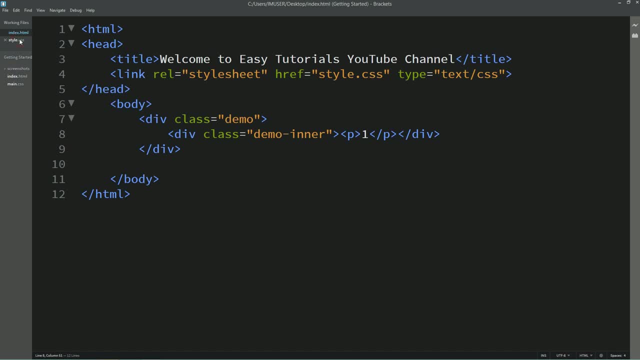 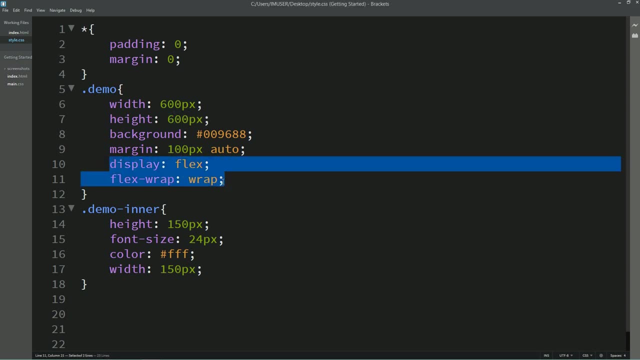 Reload the web page. we have only one div here. Let me add one color And I will reduce the height, width and margin. I will change, I will remove this display. flex that you already learned. And, And, And, And. here I will write background red. 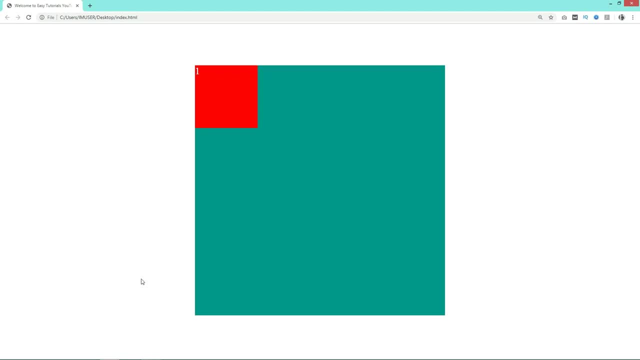 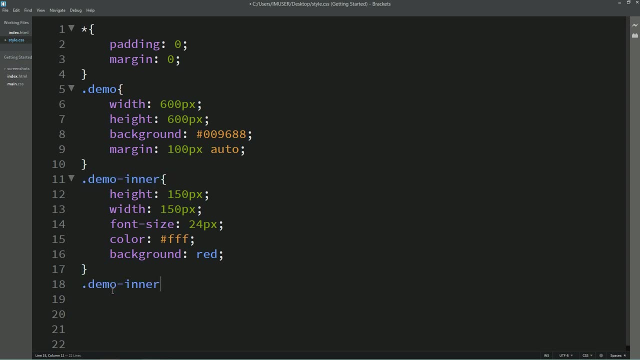 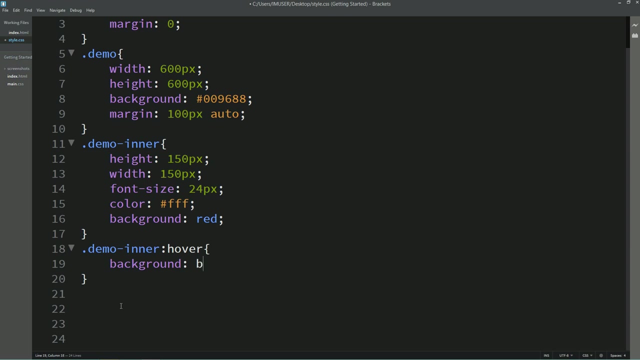 Reload the web page and now you can see one big div and one small div inside the parent div. So let me copy it here And after that I will write colon hover And when we will hover this div we will add background blue. So reload the web page and you can see, when I take cursor over this small div, the background. 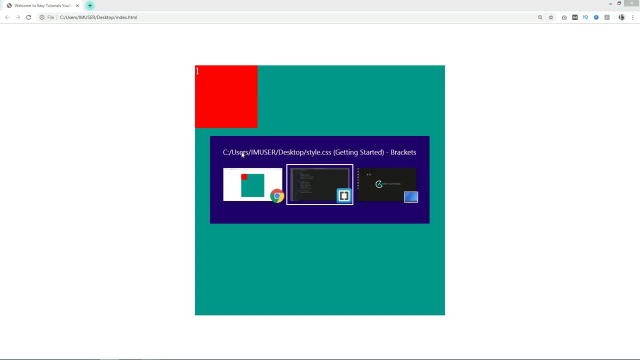 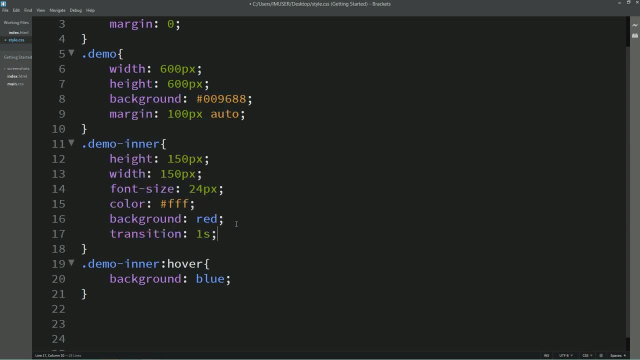 color is changing Right now. It is changing very frequently, So we need to add some transition For that. we will come back and in this div here I will add transition once again. Reload the web page and you can see when I take cursor over this small div, it takes one. 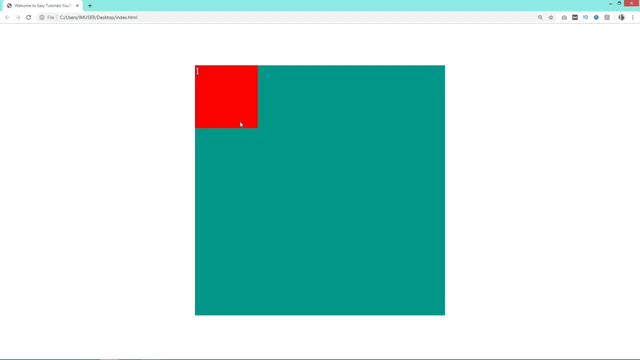 second to change the color from red to blue. So this is how transition works. Next, I will tell you very small example of animation. For that I will add a little bit of color. So this is how transition works. Next, I will tell you very small example of animation. 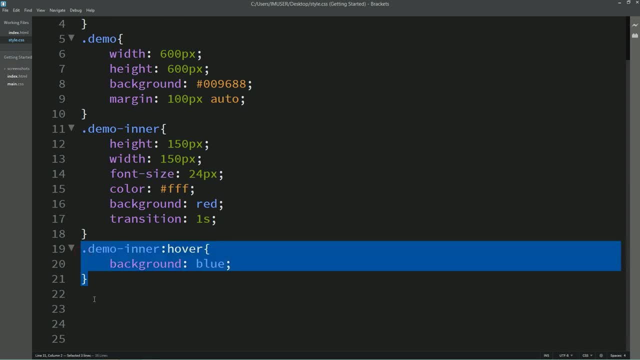 For that, I will add a little bit of color. Next, I will add a little bit of color. So this is how transition works. Next, I will add a little bit of color. So this is how transition works. For that I will remove this hover. 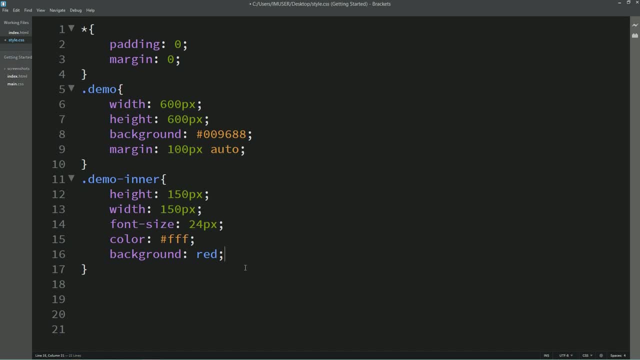 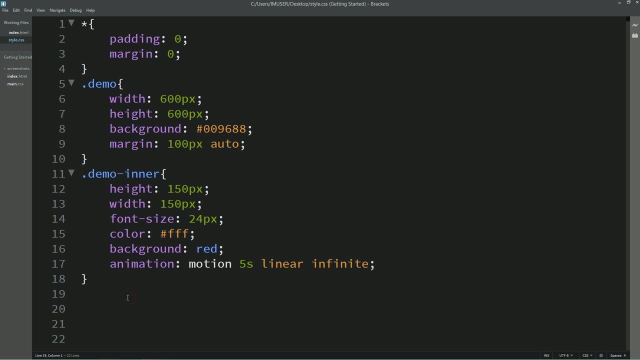 And I don't want this transition. also, And here I will add animation- We will write any name for this animation, So let me write motion. It will be for 5 second linear and it will run infinite time, And for this motion we have to set the keyframes. 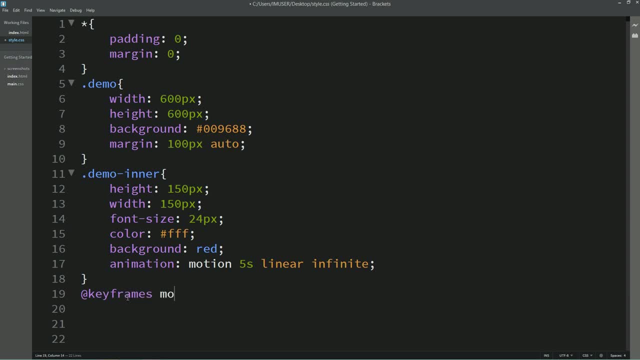 So here we will write at the rate keyframes And for this motion we have to set the keyframes. So here we will write at the rate keyframes And the name of the animation which is motion, And here we will write 100%. 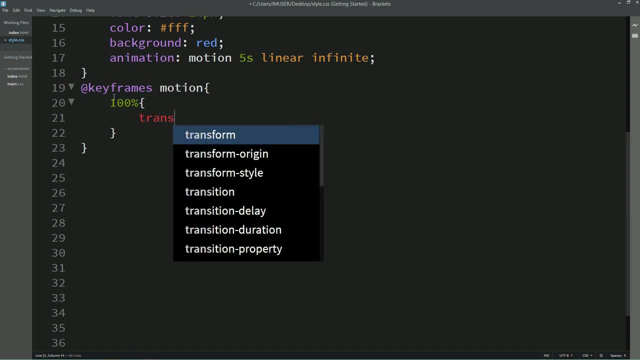 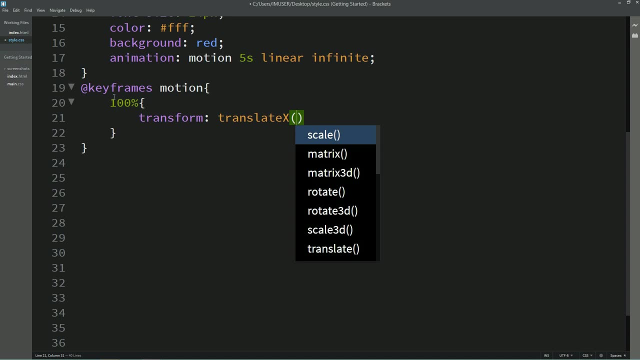 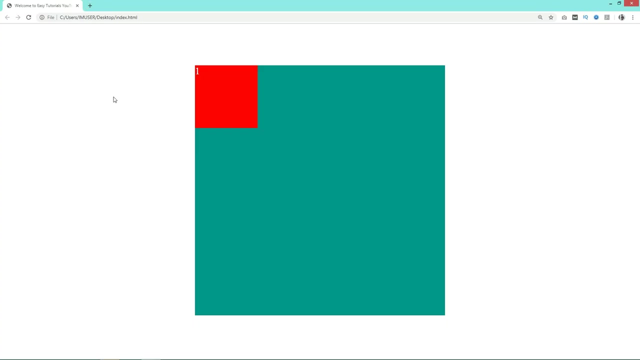 So when it is 100%, we will write transform, translate x. Basically, translate x will move the content in x direction. So we will move it by 400 pixels. Save these changes, Reload the web page And now you can see it is moving horizontally by 400 pixels in x direction. 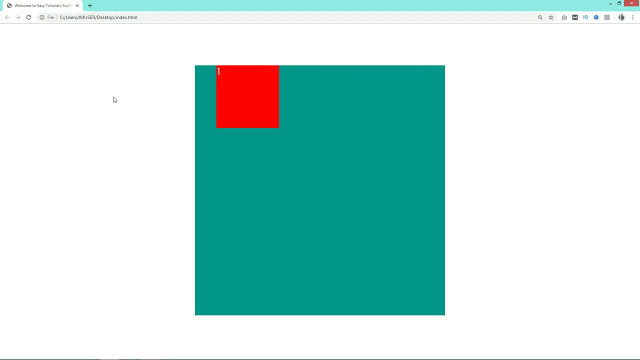 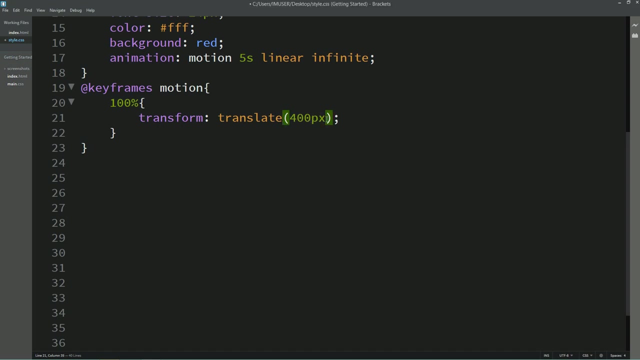 Save these changes, Reload the web page And now you can see it is moving diagonally by 400 pixels in x direction, If you want to move it in the y direction also. So let's come back in the css file And instead of translate x, we will write, simply translate. 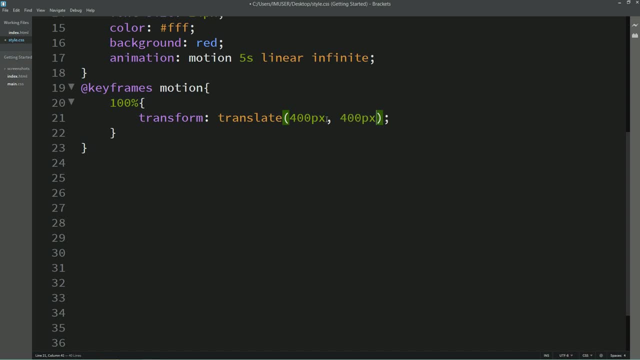 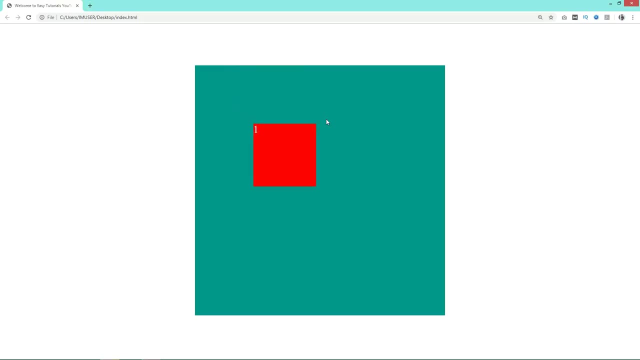 And here we will write 2 value, which is for x value and y value- 400 pixels. Reload the web page And now you can see it is moving diagonally. So we will move it by 400 pixels And here we will write 2 values. 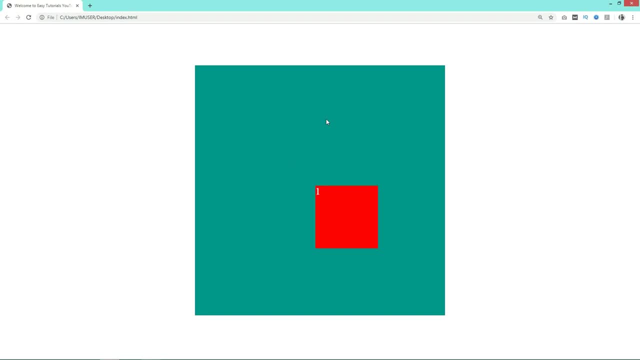 So this was very small example of css animation. You will learn more about the animation- different type of animation- when we will create a complete template using html css.